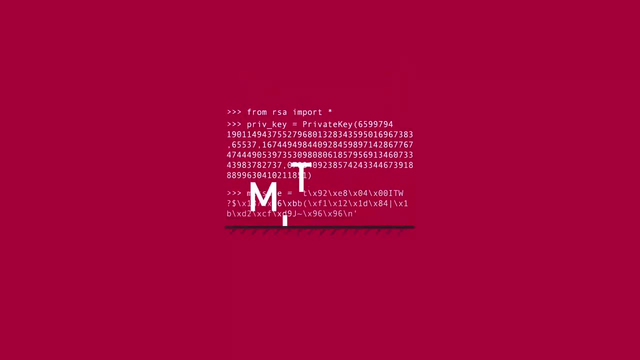 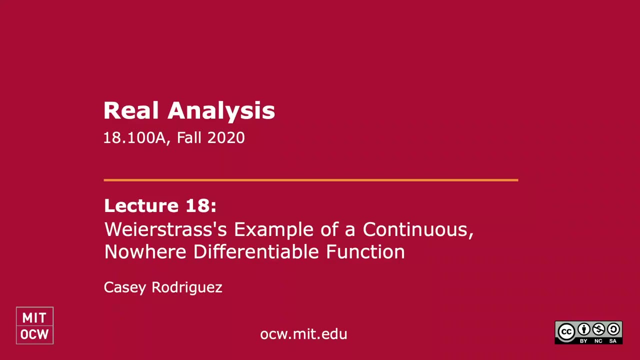 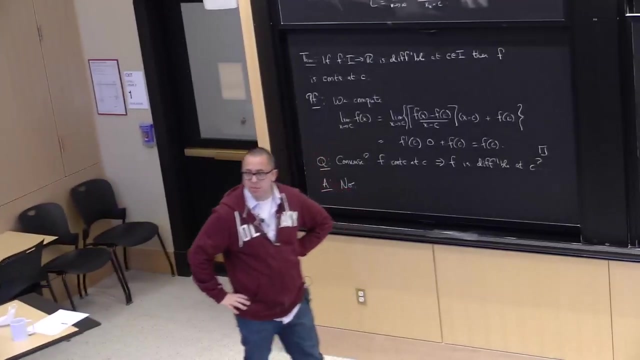 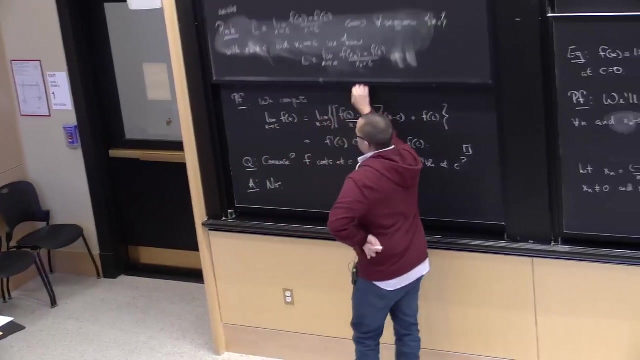 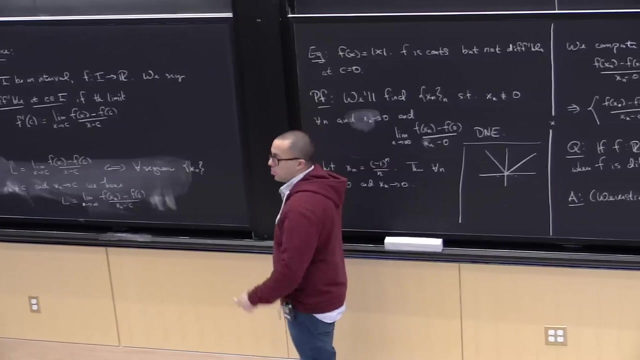 Okay, so we're going to continue with our discussion of the derivative. So now let me recall the definition we introduced at the end of last time of the derivative. So let i be an interval, meaning it could be open, closed, it could go out to plus infinity. 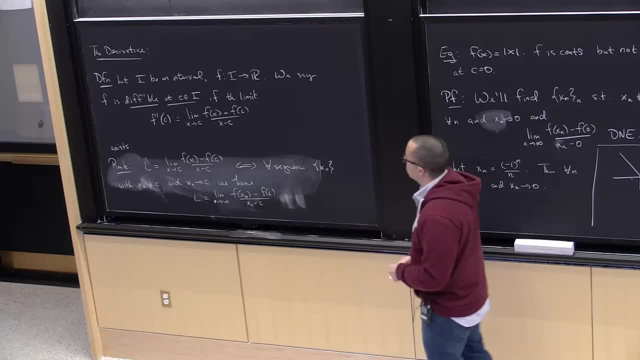 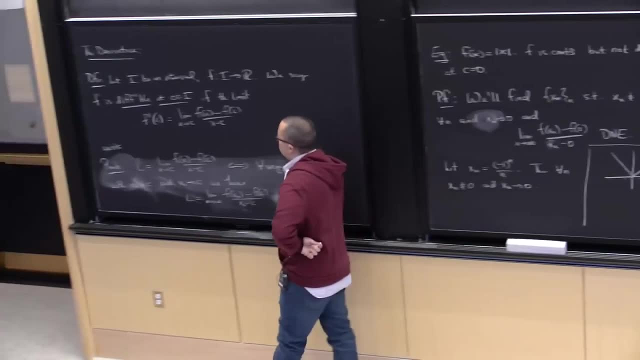 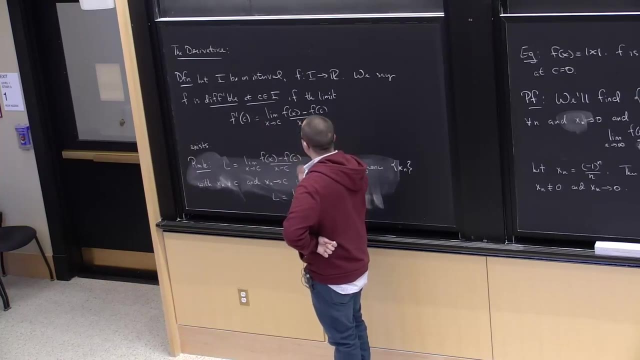 it could go out to minus infinity. but you know what an interval is, And let's take a function from that interval to r. So we say f is differentiable at a point c in i. If this limit of f of x minus f of c over x minus c, this difference quotient, if this limit 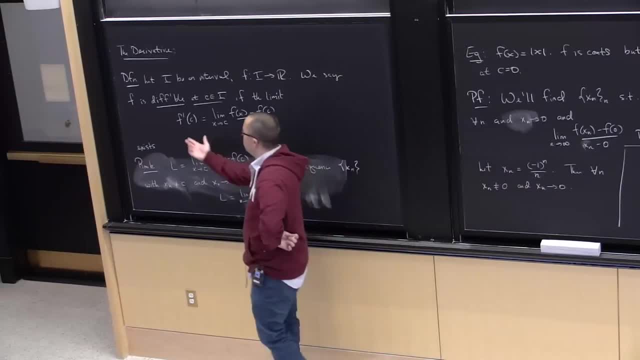 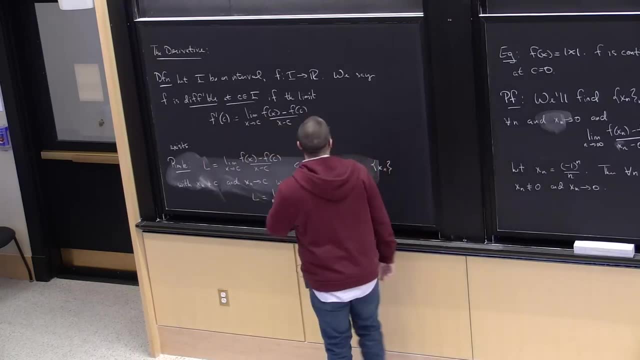 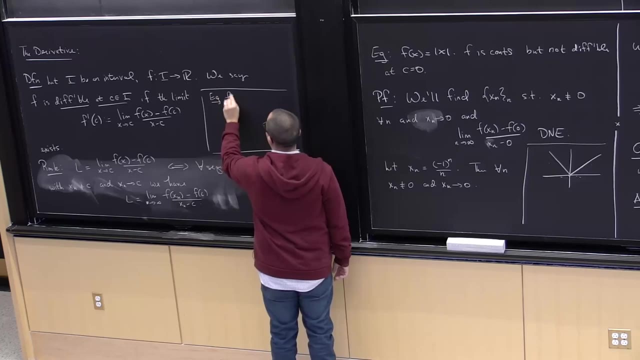 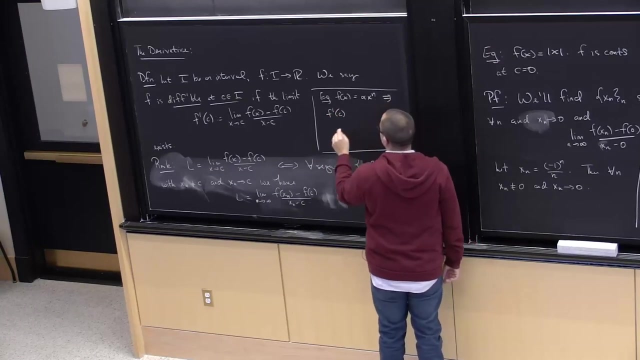 exists. if this limit exists, we also denote it by f prime of c. And last time we showed that. we gave a simple example that from last time- that if f of x equals alpha times x to the n, then this function is differentiable at every c and its derivative is equal to n times alpha. 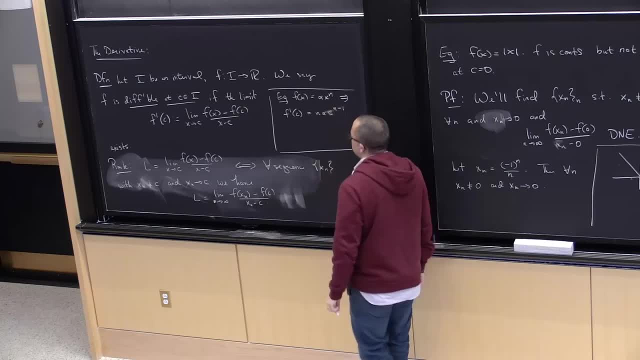 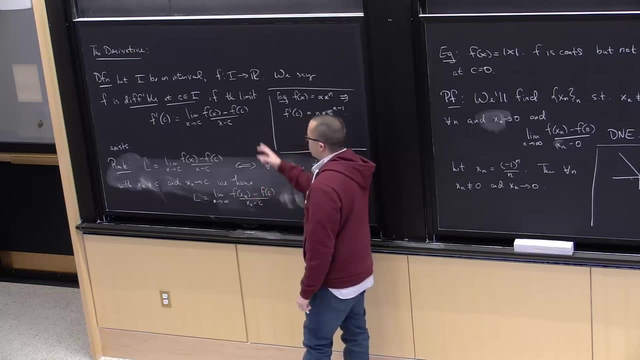 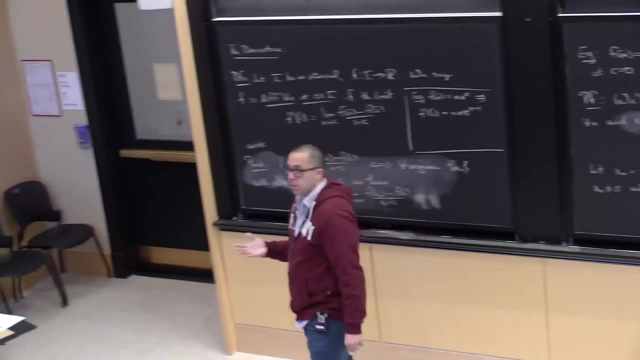 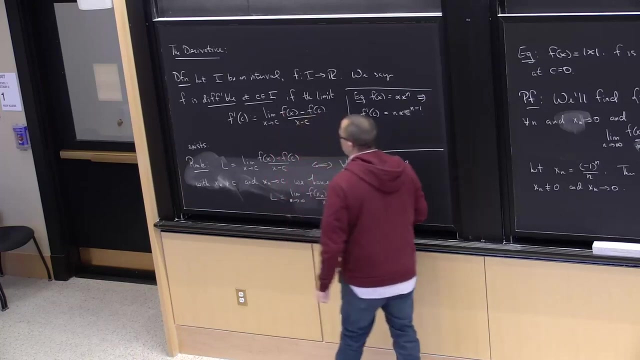 x c to the n minus 1.. All right, now let's state this in an equivalent way, using sequences. Remember, we had this characterization of limits of functions And you know, the function we're kind of looking at is f of x minus f of c, over x minus c. we had this equivalence between limits and limits. 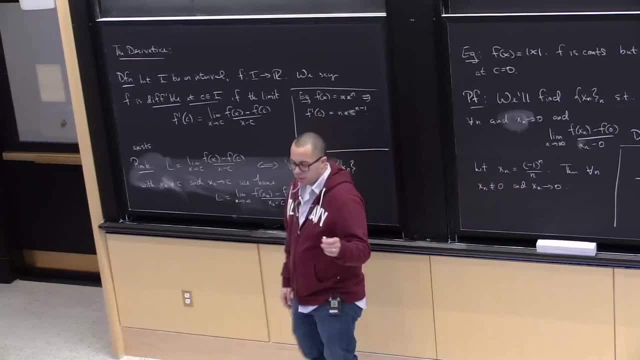 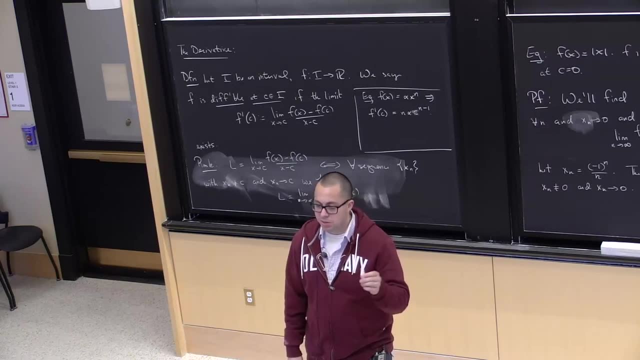 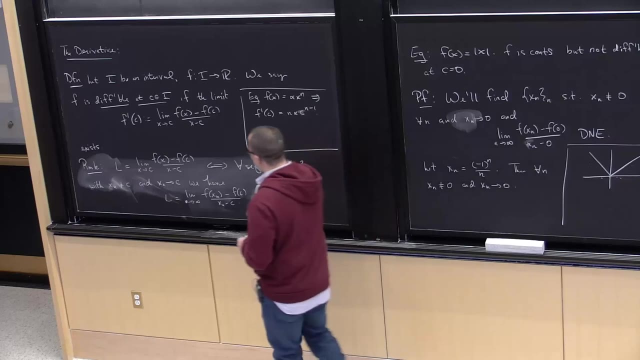 of sequences from last time, that the limit, as let's say, g of x as x goes to c equals l if, and only if, for every sequence x of n converging to c, g of x of n converges to l as n goes to infinity. So we can restate what it means for a function to be differentiable. 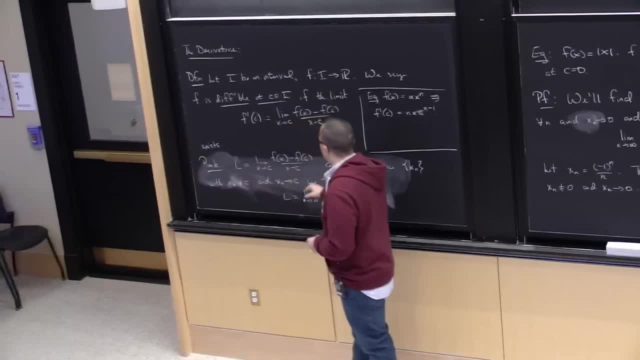 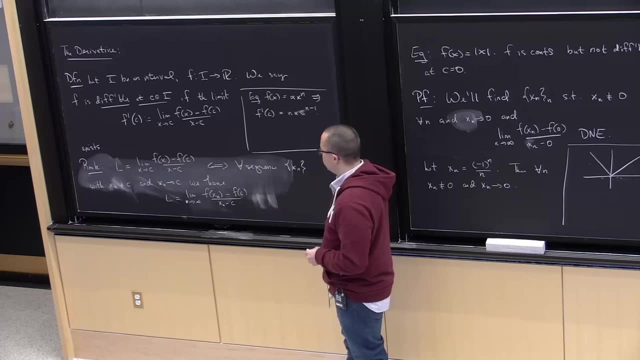 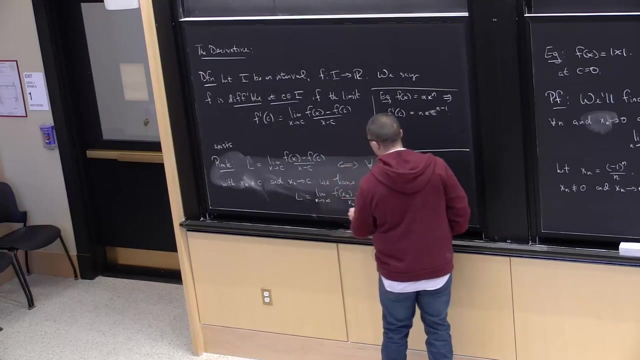 at a point and its derivative to be l. say if and only if, for every sequence x of n, with x of n not equal to c, for all n and converging to c, we have that l is equal to this limit as n goes to infinity of now this sequence of numbers f of x of n converging. 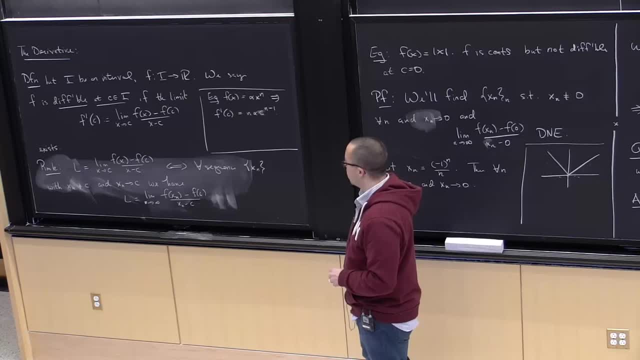 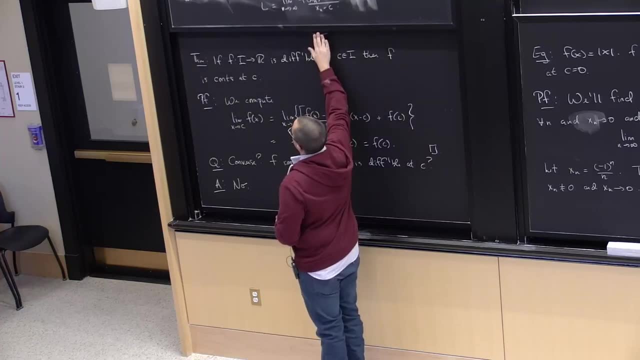 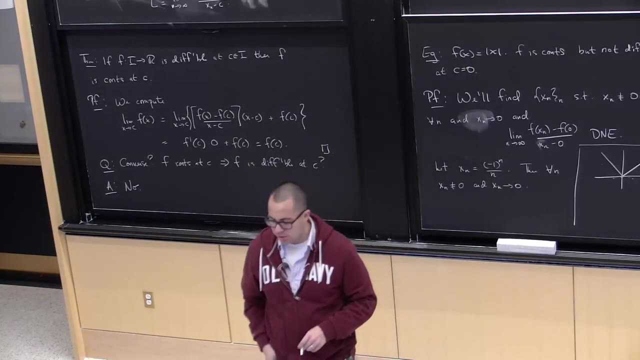 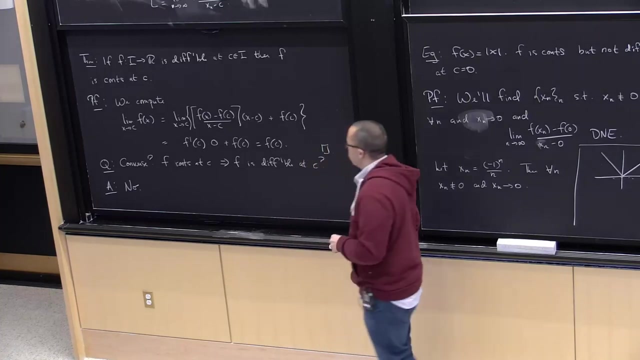 to c, x of n minus f of c over x of n minus c. okay, All right, so today, the theme of today is the connection between differentiability and continuity. okay, And we have kind of a very easy implication, which is that if x of n converges to c over x of n converging, 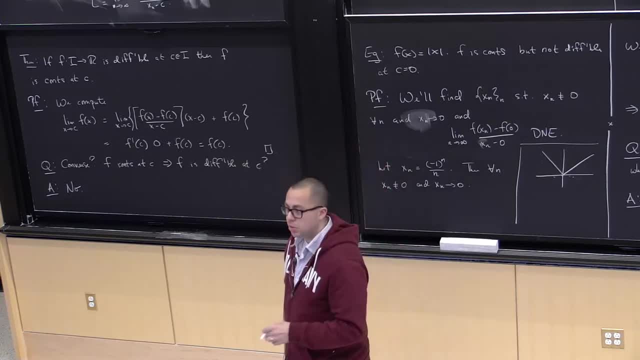 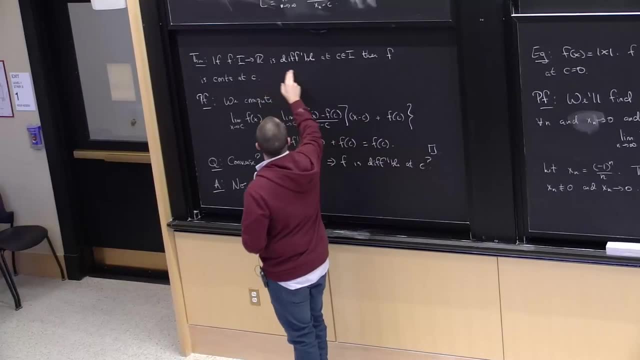 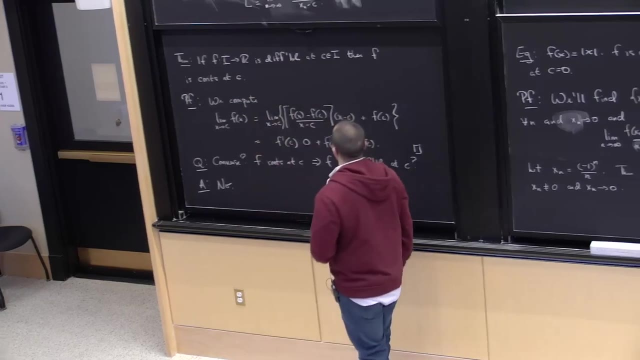 to c. if a function is differentiable at a point, then it must be continuous at that point, okay? So that's a statement of this theorem. If f going from an interval to r is differentiable at c, then f is also continuous at c, okay. 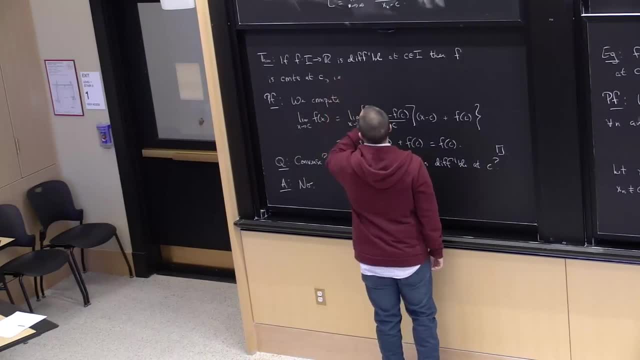 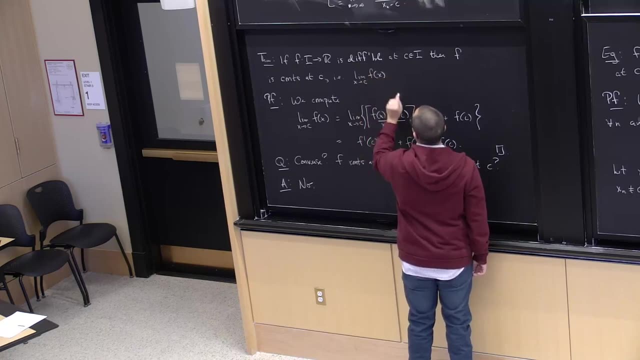 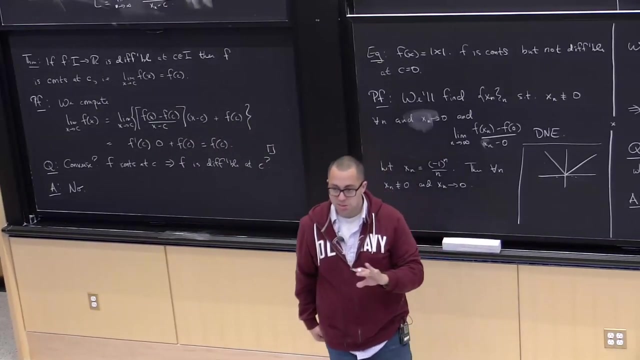 So let me also add in here that continuity at the point c in an interval is equivalent to saying that the limit of a function is differentiable at a point. okay, So let me add in here that at all this, as x goes to c of f of x equals f of c. okay, Now this: 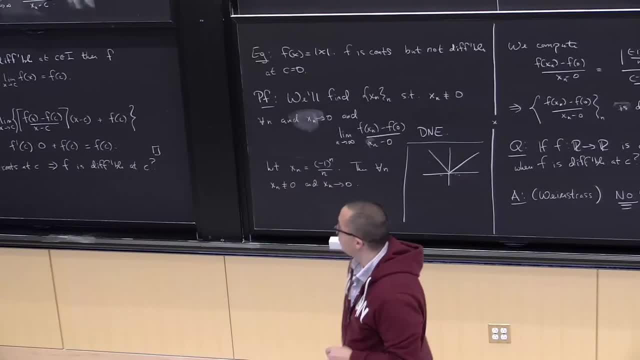 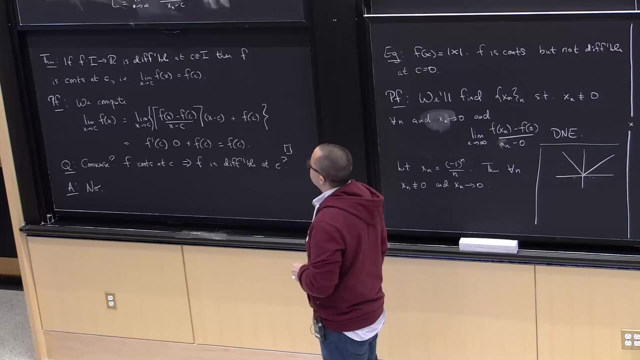 is just a subtle point that I want to make is that for an interval, open, closed, half open, half closed, whatever- any point in that interval is a cluster point of that interval And therefore this definition I made up there is actually meaningful and for continuity. 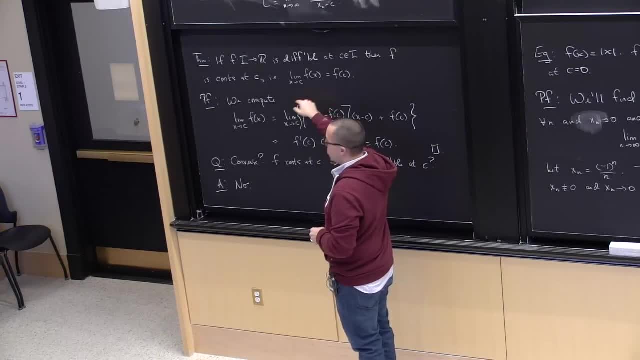 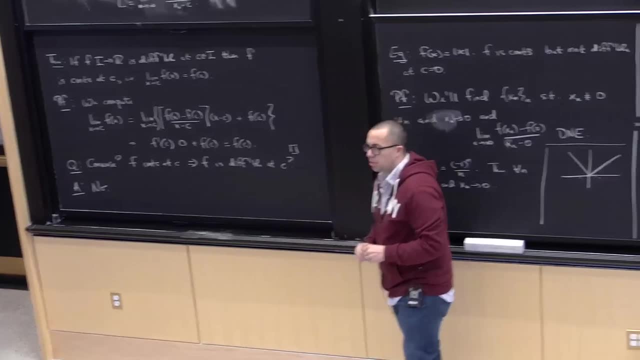 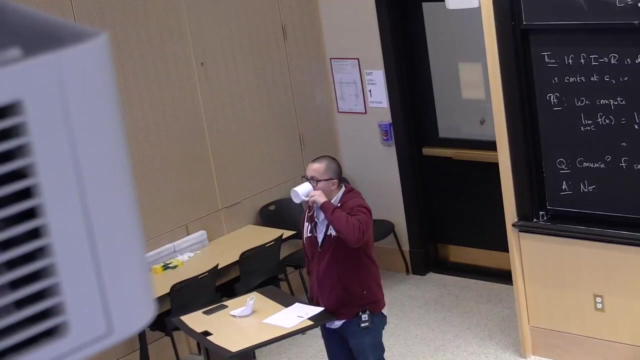 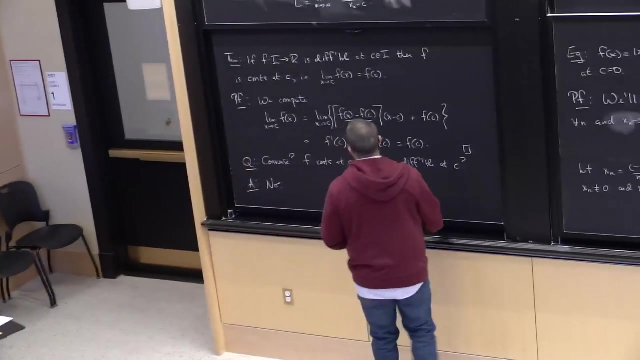 something being continuous at C is equivalent to. if C is a cluster point- which I just said it is, it always is. this limit equals the function evaluated at the point. So that's just kind of a subtle comment I want to make. 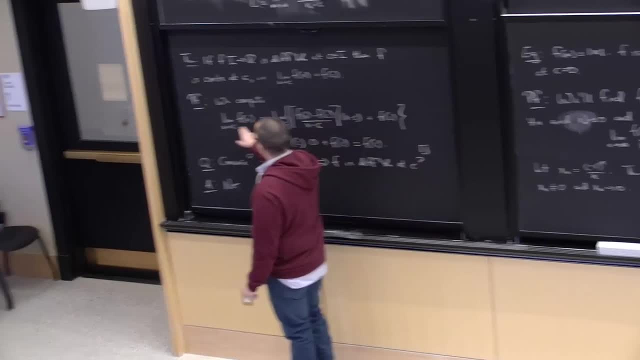 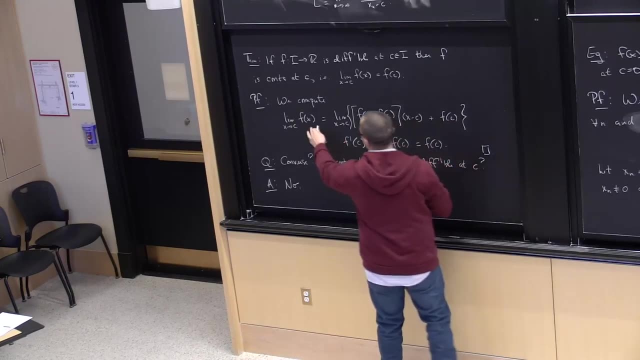 So how do we prove this? We write the limit as X goes to C of F of X, as in this way. So essentially, what I do is I add and subtract F of C, and then the part that is F of X minus F of C, I multiply by X minus C and divide by X minus C, which is perfectly fine because 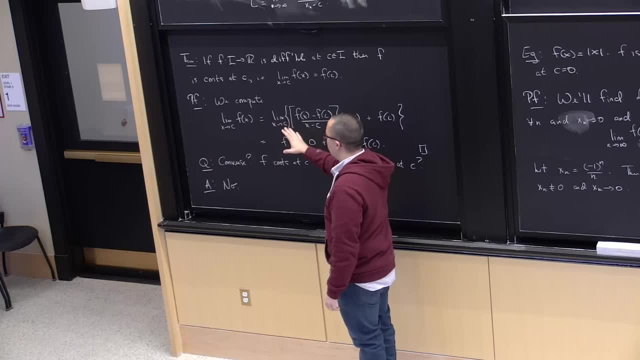 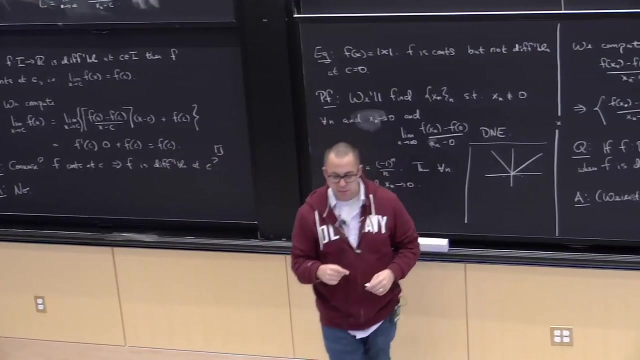 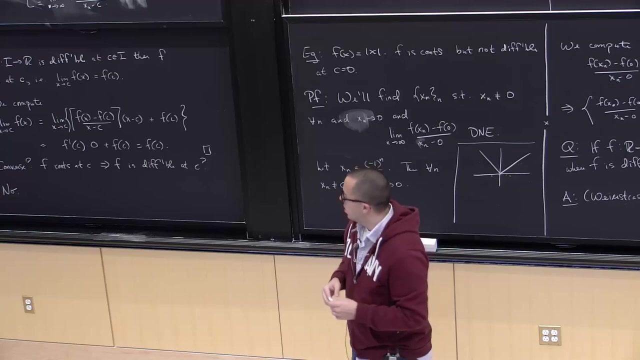 remember, for a limit. I'm never actually looking at points where X equals C, So that's fine, And so I get this expression here. Now, what we know about limits is that the limit of the sum is the sum of the limits, as long as all these limits exist, and the limit of the product is the product of the. 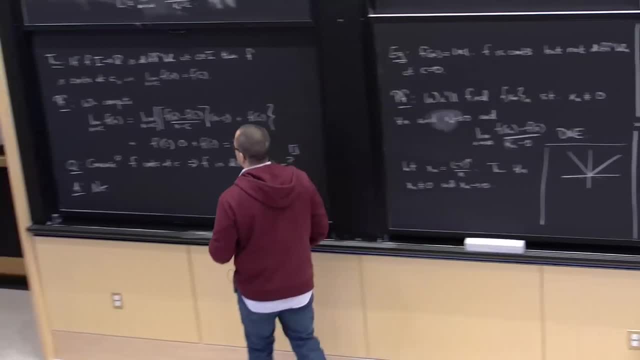 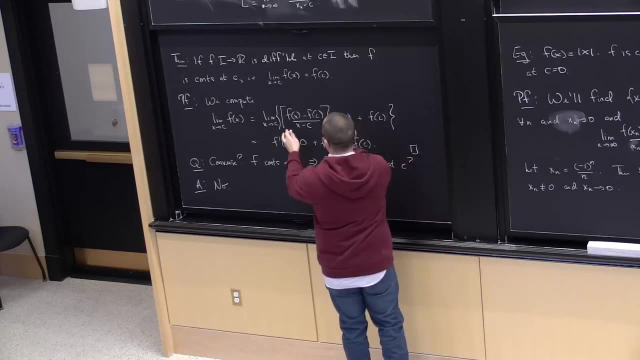 limits, Again, assuming all of these limits exist And the limit as X goes to C of everything you see here do exist. So, as X goes to C, this thing in brackets or in the? I guess these are brackets, I don't know what those are called. 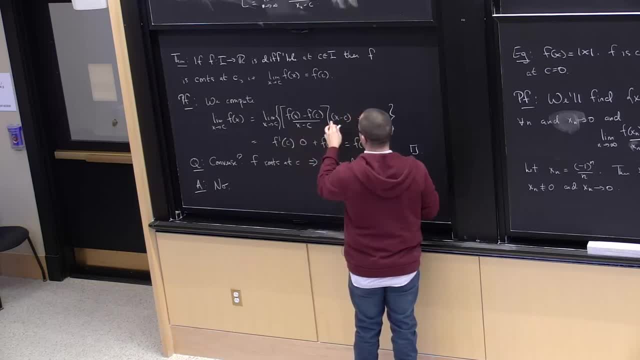 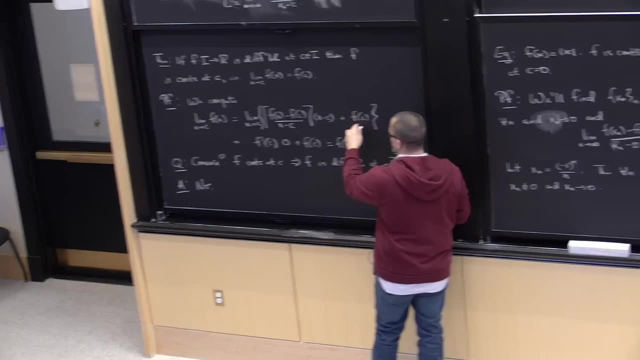 This limit here is F prime of C. As X goes to C. of X minus C, that's just 0. And F of C is just a constant. There's nothing changing with X. So the limit of a constant is that constant. 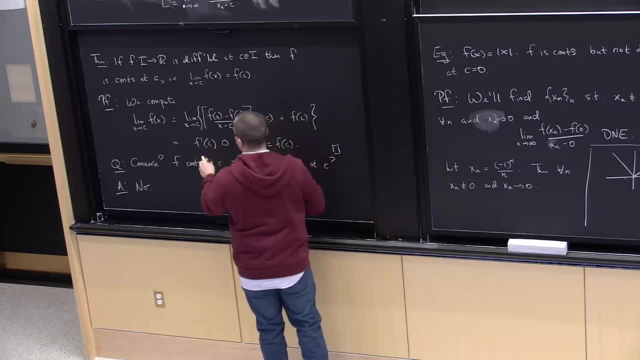 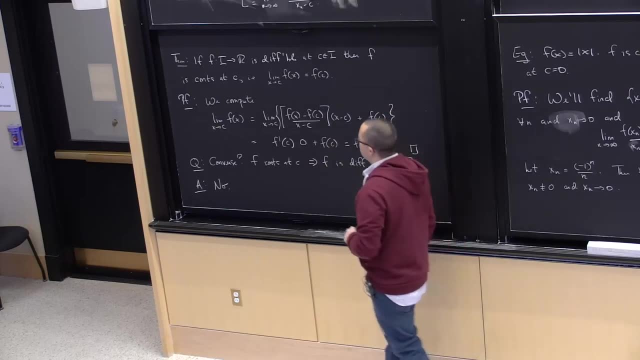 So I just get F of C. So the limit of this whole expression is F prime of C times 0 plus F of C, which equals F of C. So we've just proven that the limit, as X goes to C of F of X, is equal to F of C, which is: 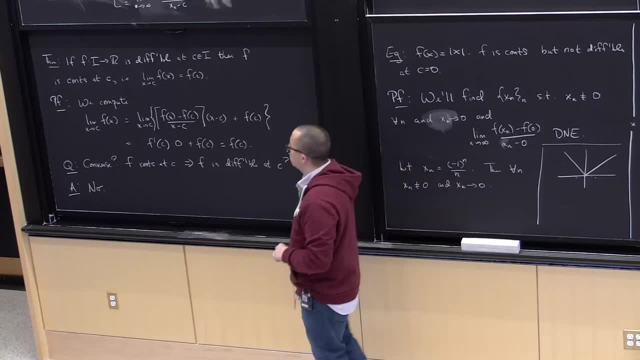 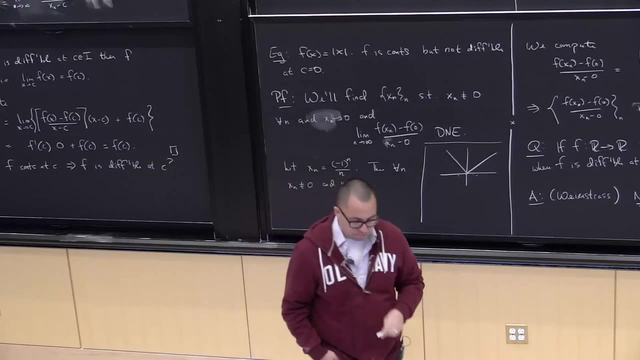 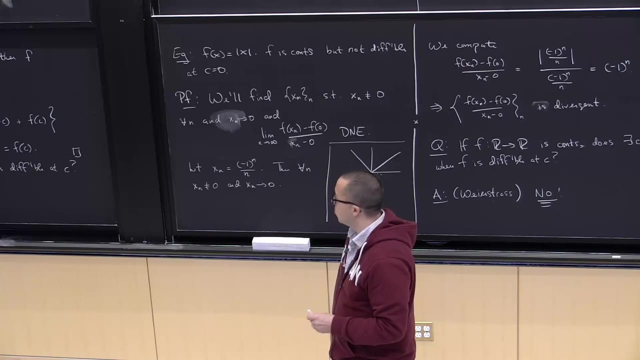 what we wish to prove, And therefore a function which is differentiable at a point must be continuous at that point. So, as beginning math students, we're learning proofs, but we're also learning questions. What types of questions to ask, And whenever you come across this? 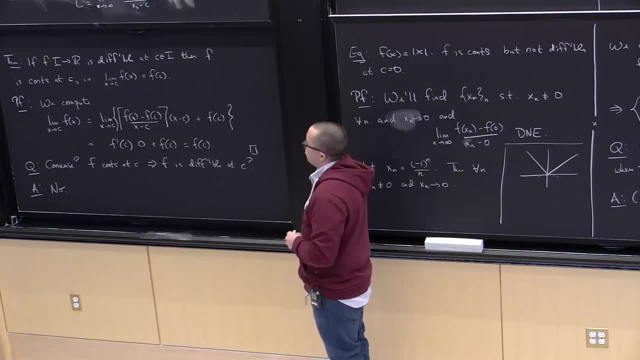 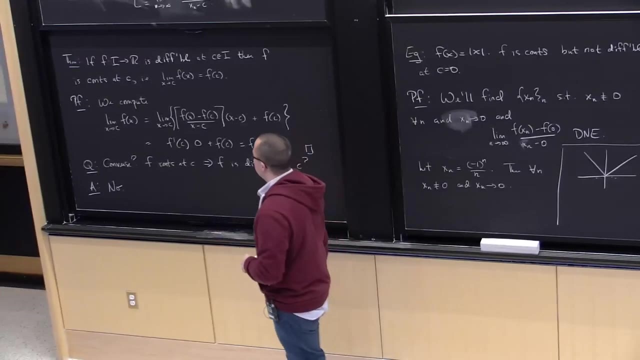 a new theorem that has one implication, one hypothesis, one conclusion. then you should ask yourself: does the converse hold? Does the conclusion also imply the hypothesis? So we've shown that F, differentiable at C, implies F is continuous at C. So does the 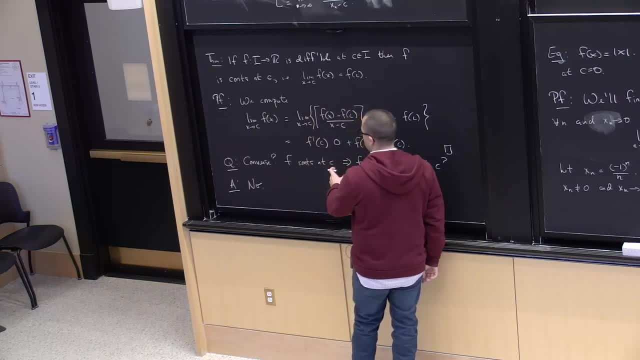 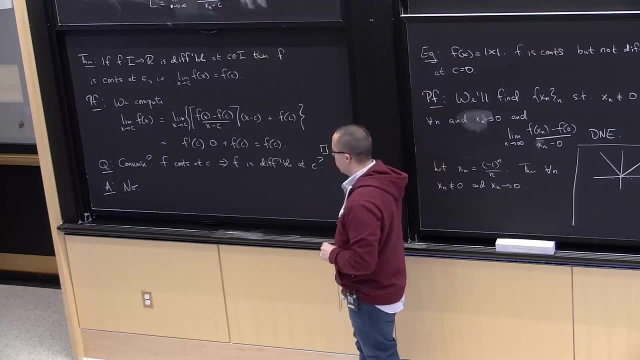 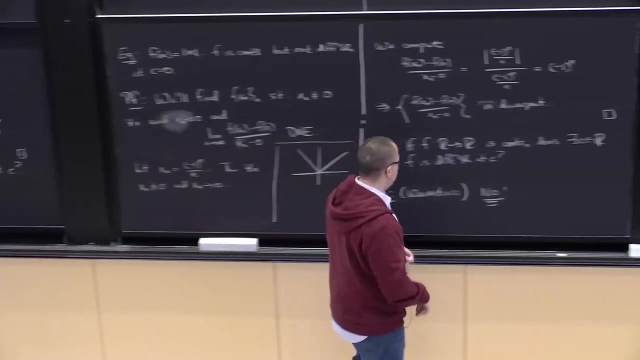 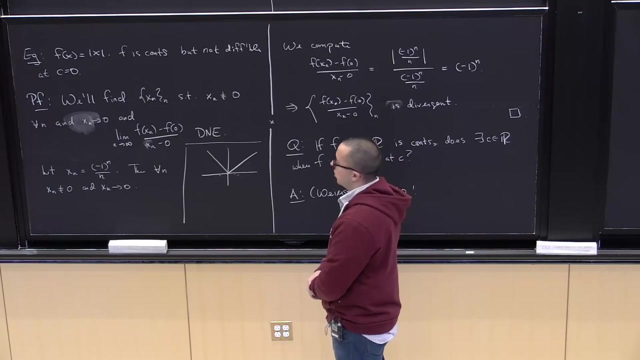 converse hold, Namely if F is continuous at a point, does this imply that F is differentiable at that point? And as you can see already there, the answer is no. I think you've probably covered this in calculus. But what's the function that gives this counterexample that is continuous at C but not differentiable? 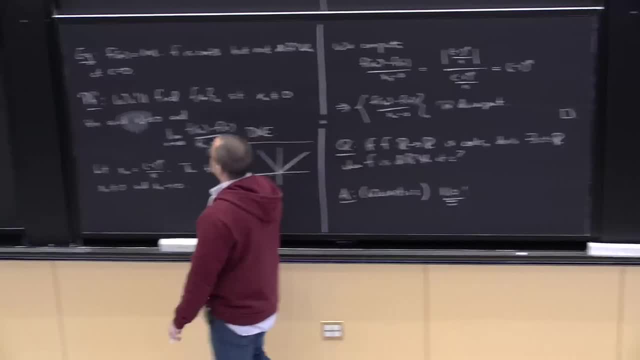 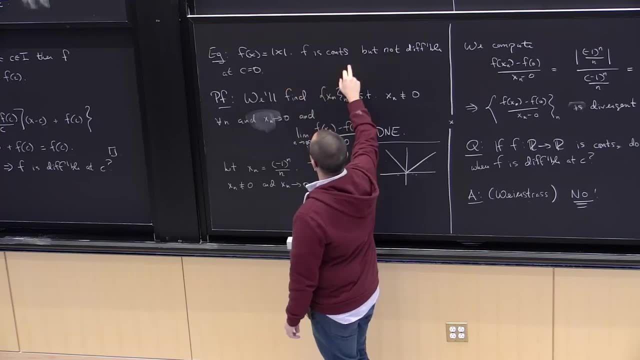 at C. Well, let's take for example, C equals 0.. And let's look at the function F of X equals the absolute value of X In this function. here, this is continuous at every point. So, in particular, this is continuous at every point. 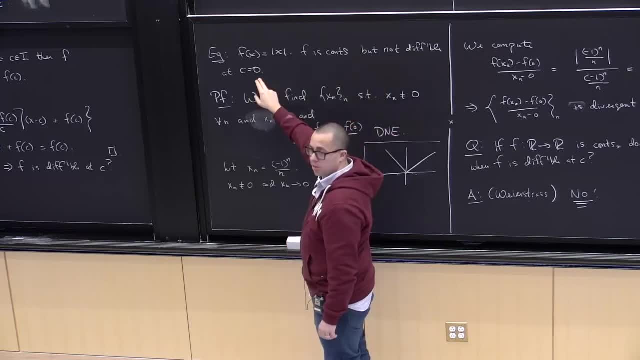 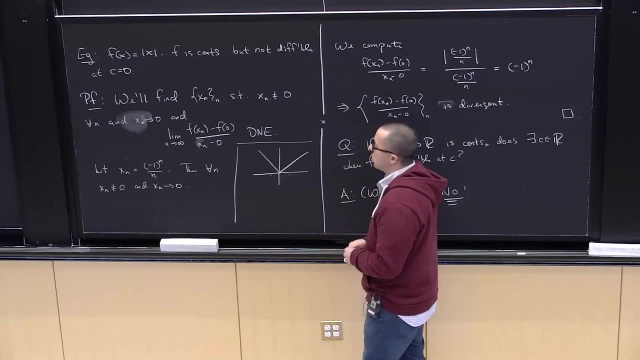 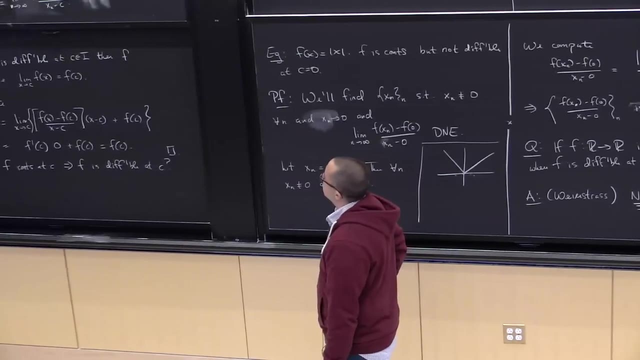 So, in particular, at C equals 0. But it's not differentiable. at C equals 0. And how do you come up with and how do you do that? How do you show something's not differentiable? The simplest way is to use this remark up here by finding a sequence converging to C. 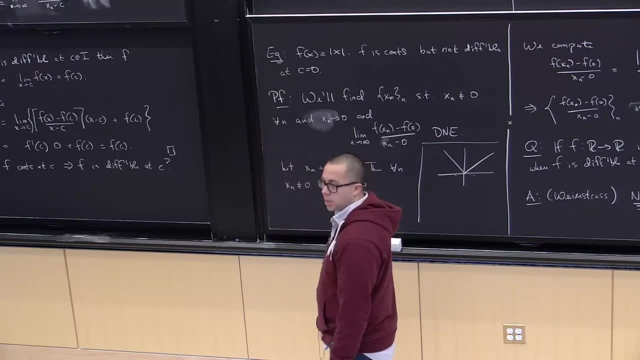 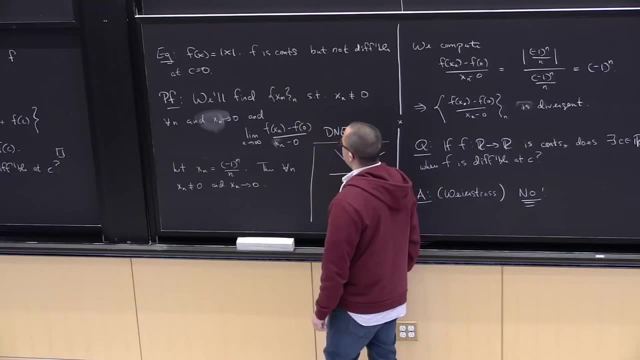 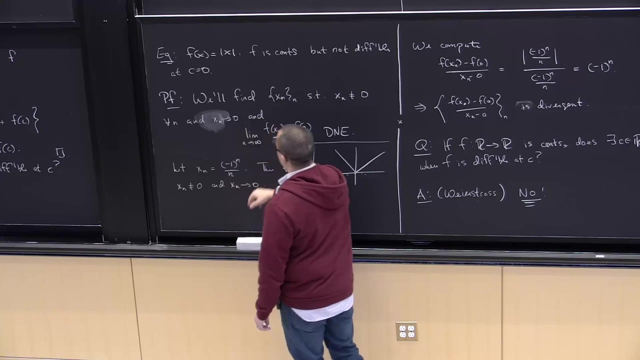 so that the difference quotient does not have a limit as N goes to infinity. So that's what we'll do here, is we'll find a sequence X sub N, With X sub N not equal to 0, for all N converging to 0, such that this limit does not exist. 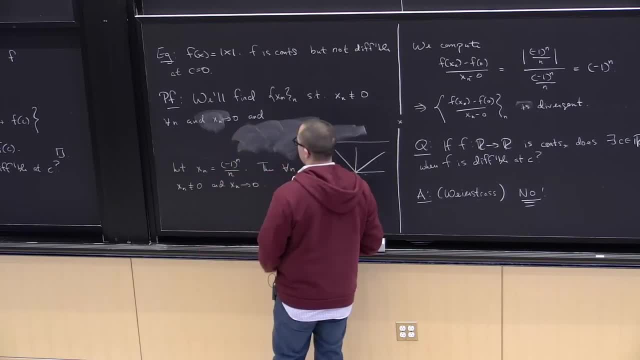 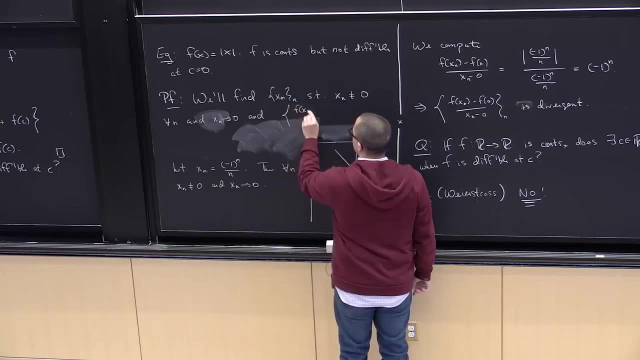 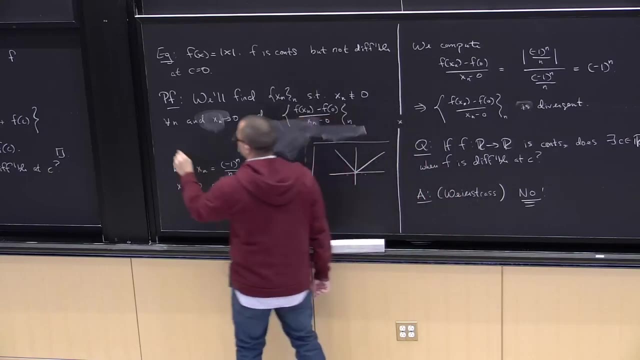 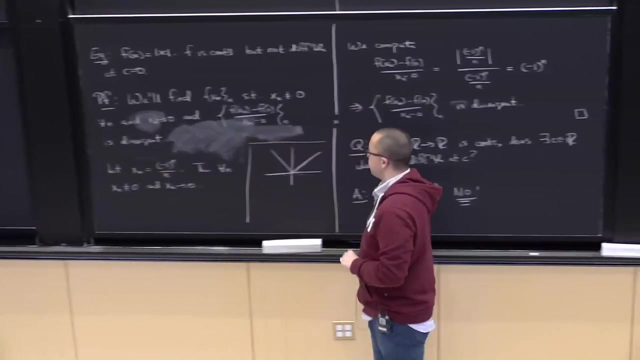 And rather than write that because the limit does not exist, it doesn't make really sense for me to even write that- let me write this as saying: as the sequence is divergent, OK, So OK. Now how are we going to come up with a sequence X sub N, so that the difference quotient does? 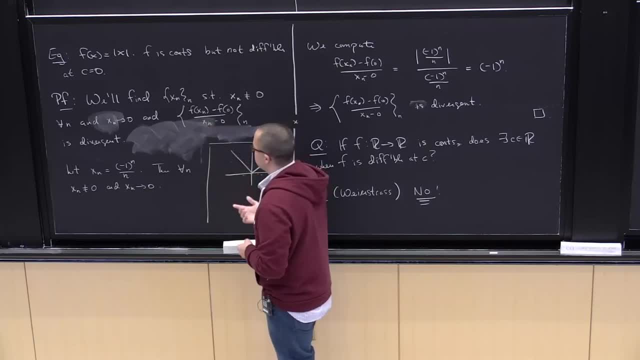 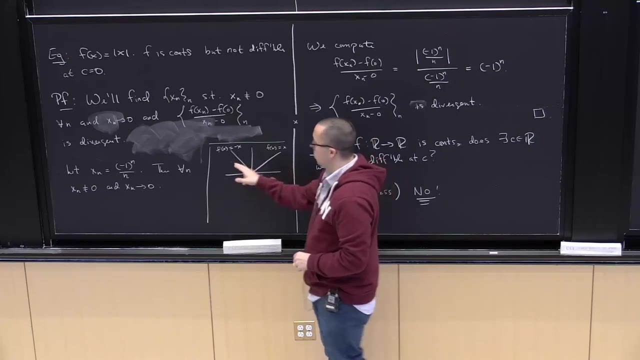 not converge. Well, what's the logic? So, for, F of X equals the absolute value of X. it looks like this. it looks like X, it's equal to X over here minus X over here. OK, So if you were to formally differentiate, well, I mean you could actually differentiate. 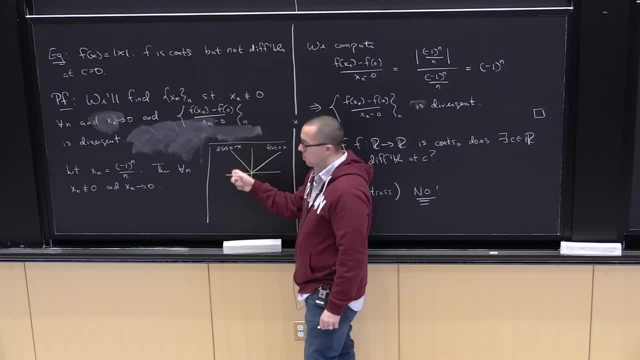 to the left of 0, you get the derivative is equal to minus 1.. To the right, the derivative is 1.. So that kind of suggests maybe there's some funny business going on at 0.. So let's look at a sequence which alternates between being negative and positive, but is 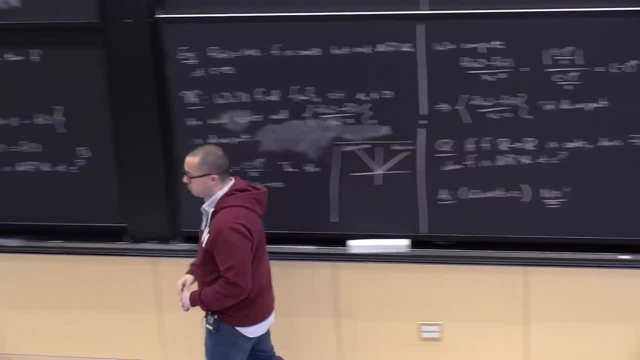 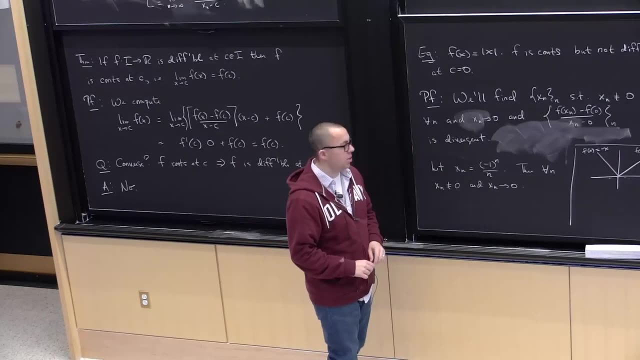 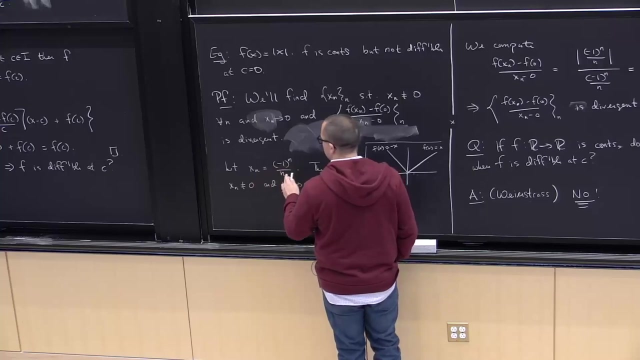 converging to 0.. Let's see if that sequence will provide us with this desired sequence, which results in the difference quotient being divergent. So let's just take a guess: Let XN be minus 1 to the N over N. It doesn't have to be this one, just something that alternates. 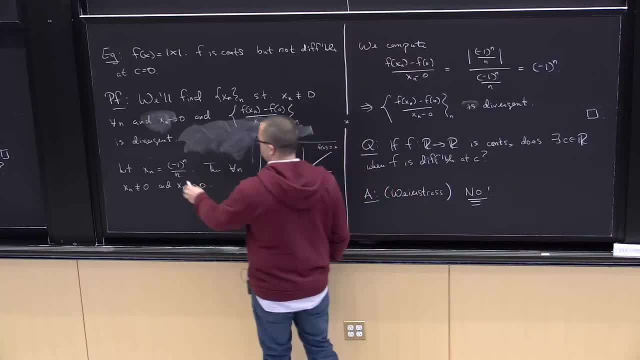 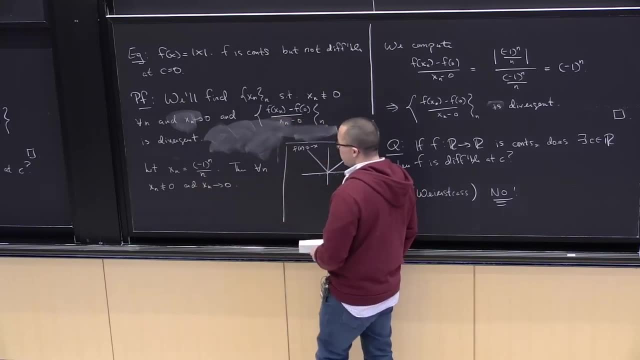 back and forth would be enough. So this could be N squared here, or 2N, or N to the 20,, 20, whatever you like. Then this is clearly always non-zero And it converges to 0.. OK. 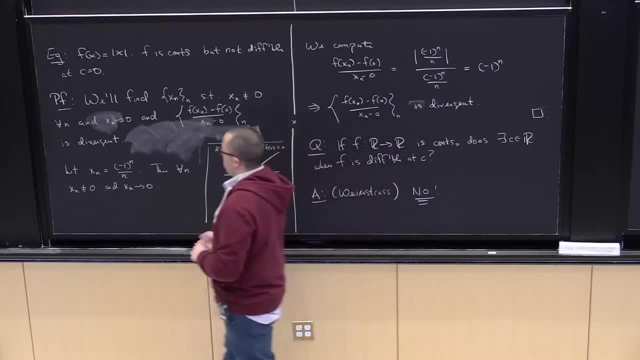 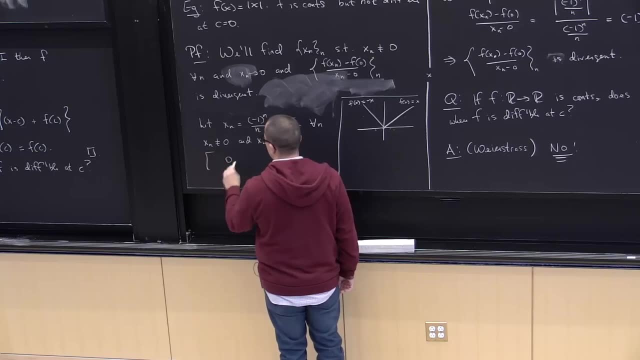 And, of course, why it converges to 0, I mean, you could prove this by epsilon M definition. but also if I take the absolute value, that's less than or equal to 1 over N, and this one, we know, converges to 0. 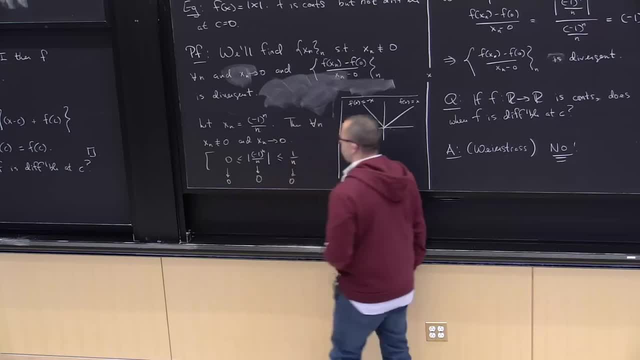 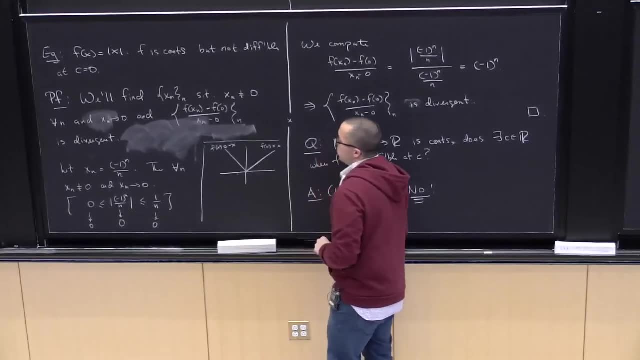 OK, 0.. So by squeeze theorem, the thing in the middle must converge to 0, and we're done, OK. So we have this sequence: X sub N equals minus 1 to the N over N which is alternating back. 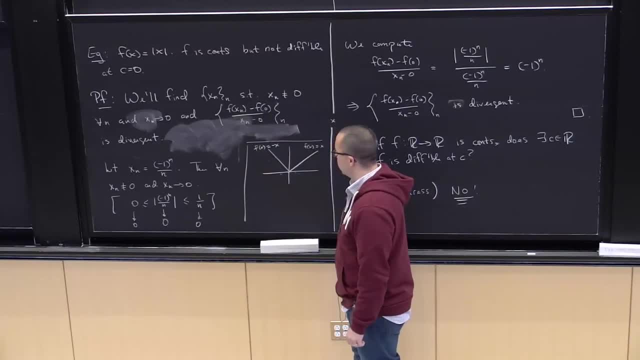 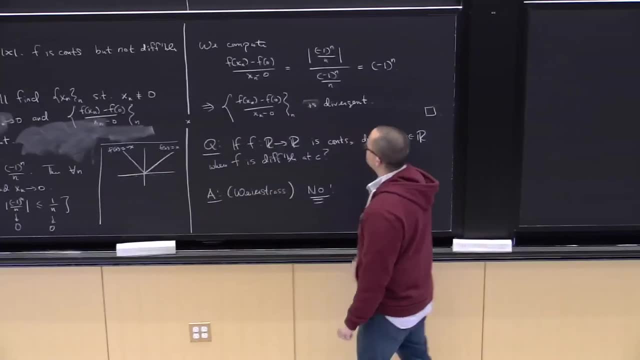 and forth, And we hope it's going to result in this difference quotient being divergent as N goes to infinity, And so we compute that. Let's look at the difference quotient F of X of N minus F of N, So we have F of 0.. 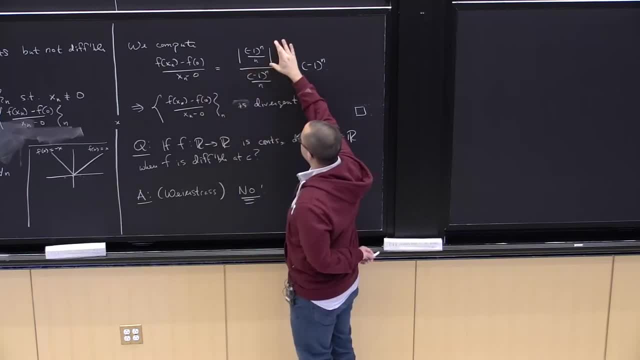 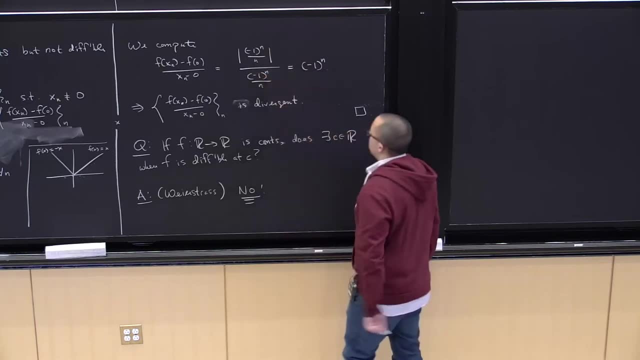 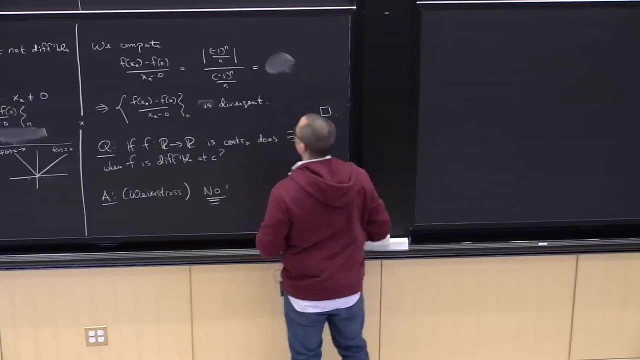 F of 0 is just 0. So I just get F of X of n, which is the absolute value of minus 1 to the N over N, over X of n, which is minus 1 to the N over N. This is just equal to 1 over N over, minus 1 to the N over N, which equals minus 1 to the. 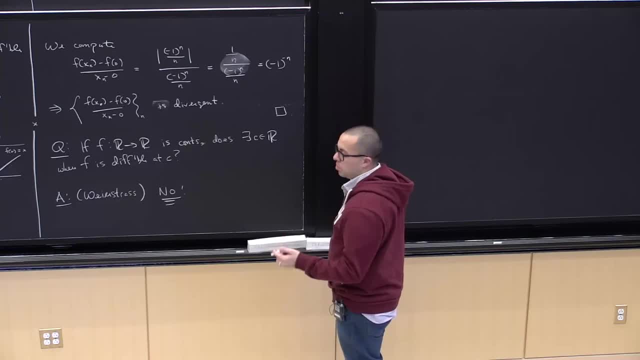 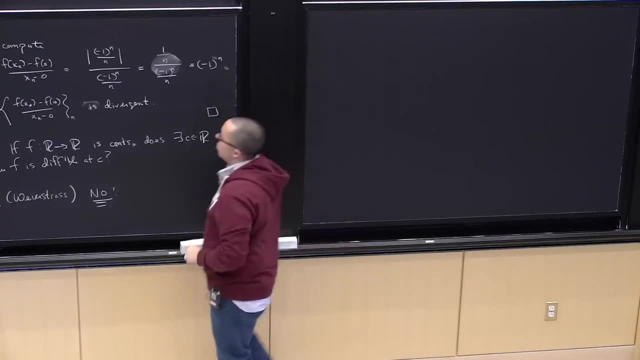 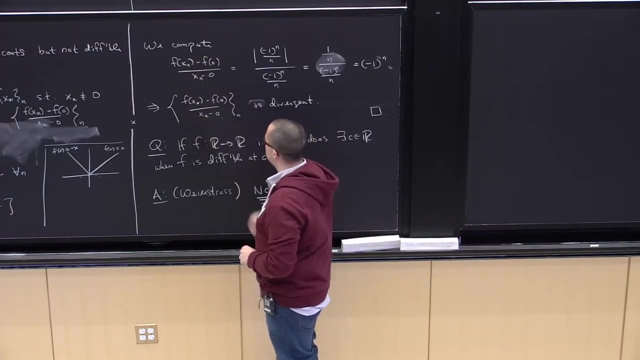 minus n, but minus 1 to the minus n. this is equal to the same thing as minus 1 to the n right. So this sequence here of difference quotients, so f of xn minus f of 0, over xn minus 0,. 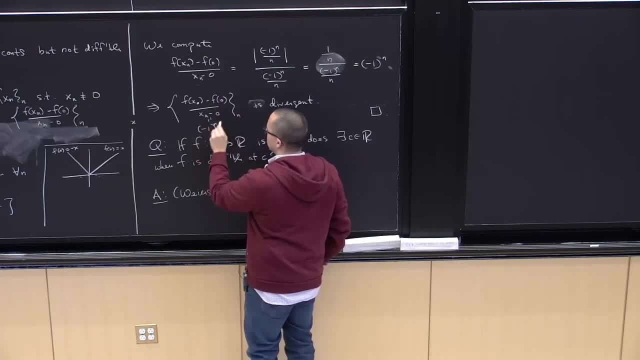 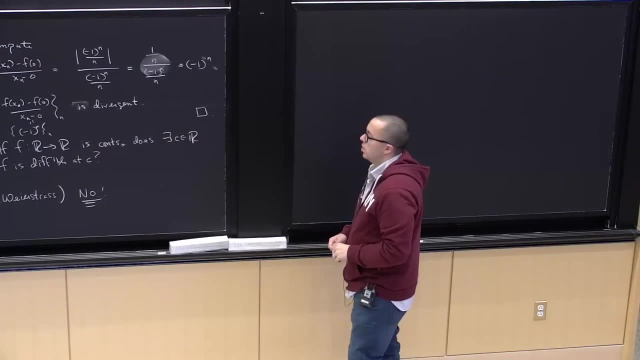 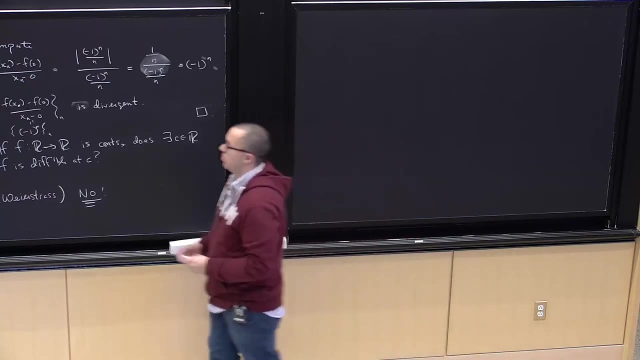 this is just equal to the sequence minus 1 to the n, which we know is divergent, doesn't have a limit. That's one of the first examples of a sequence we prove does not converge. OK, So, in summary, this function f of x. 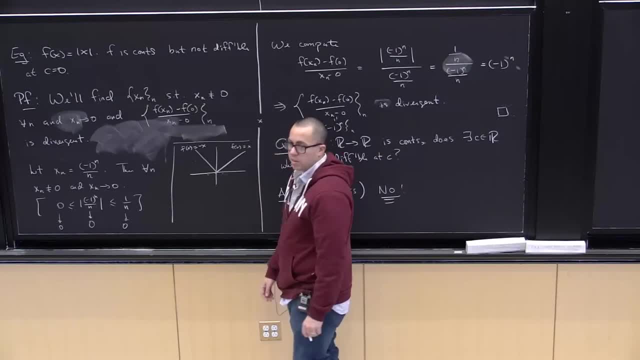 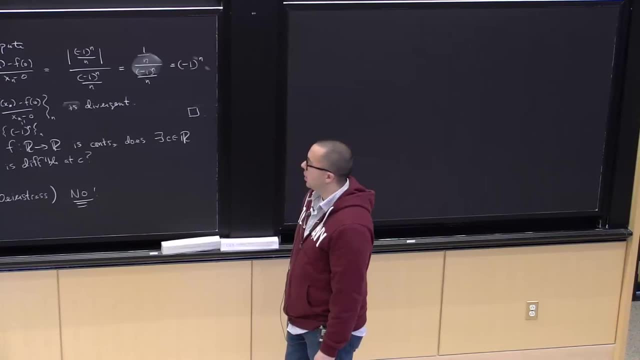 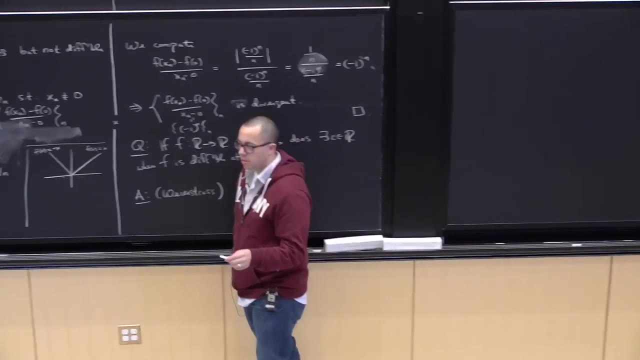 equals the absolute value of x is continuous at c equals 0,, but not differentiable at c equals 0.. So now a natural question that people ask is: OK, so a function being continuous at a point does not necessarily imply, But let's take a function which is continuous. 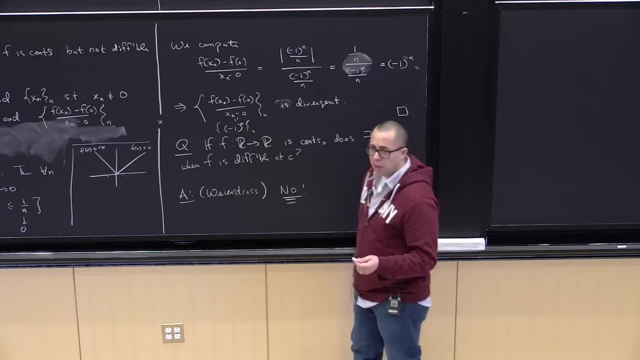 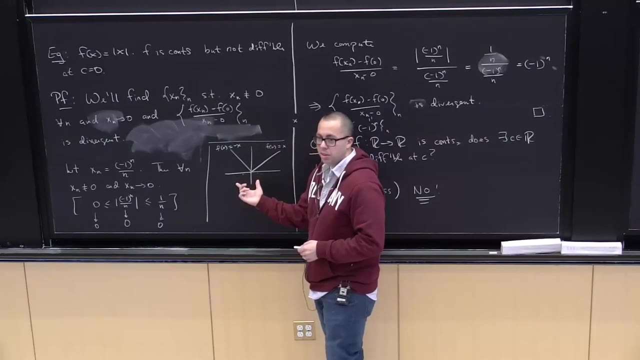 on the real number line. Is there a point where it's differentiable? So it's already on the board, but this is not completely a crazy question to ask. For example, let's go back to f of x equals the absolute value of x, right? 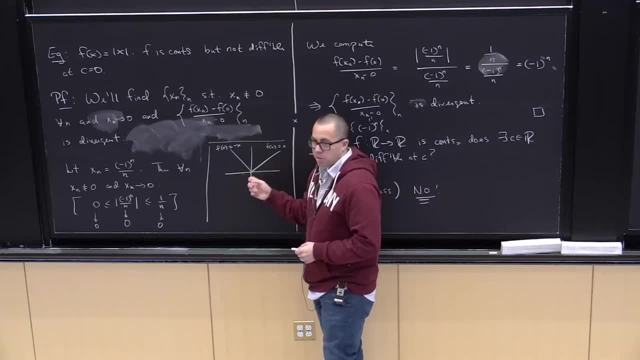 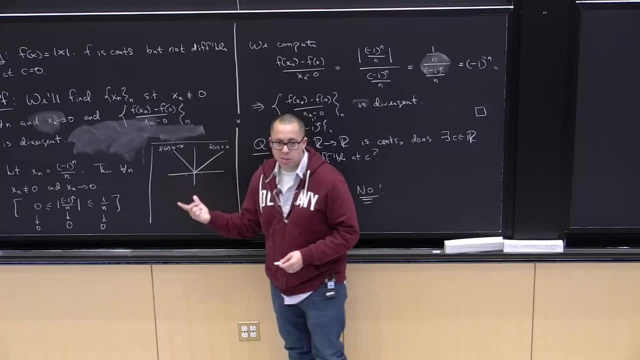 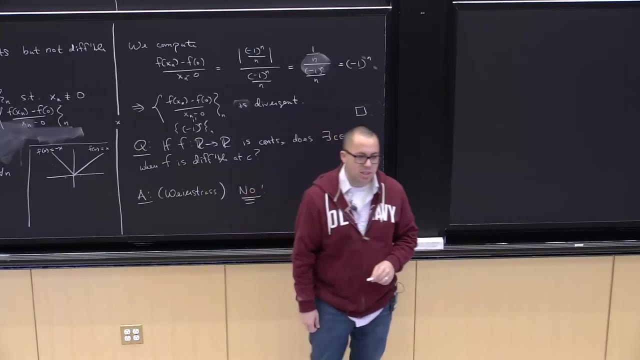 This function is differentiable everywhere except 0. So there's lots of points where this function is differentiable. It's differentiable for c positive and c negative. So for this continuous function there does exist points where it's differentiable, And you can imagine trying to draw any kind of curve. 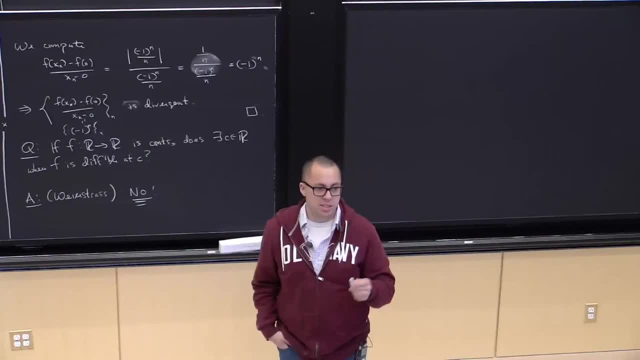 that you can on a piece of paper and you can probably find a point on that curve that has a tangent. all right, I mean, if you sit there with pencil and then try to draw something very jagged, I mean there's still. 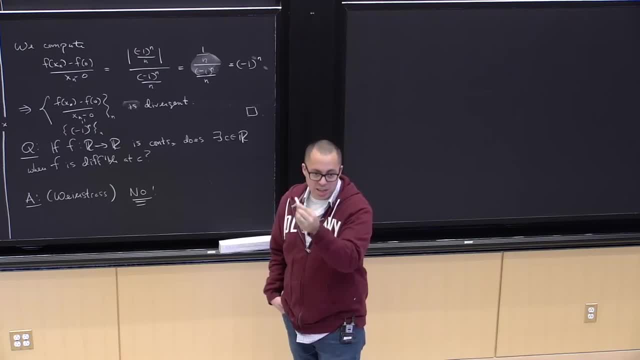 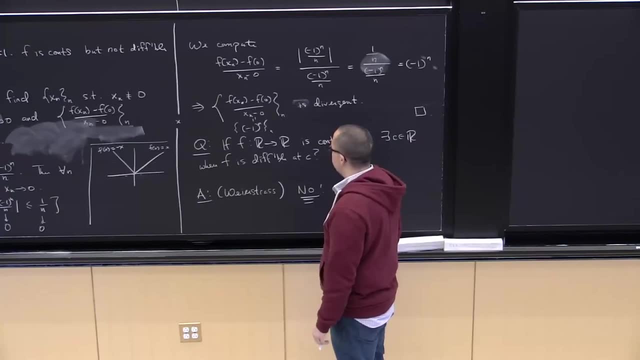 going to be little sections of your jagged curve where it has a tangent. So I imagine this is why people are going to think that it's differentiable Thought this was the case that a continuous function has to have at least one point where it's differentiable. 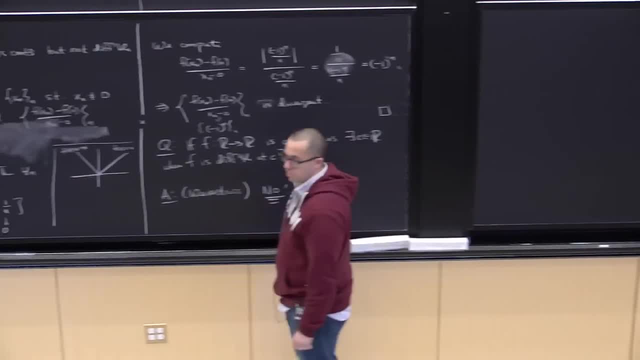 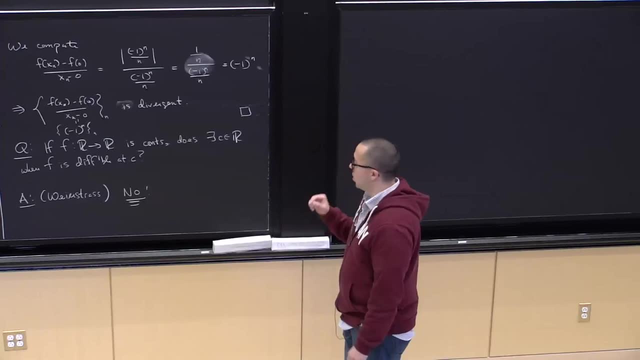 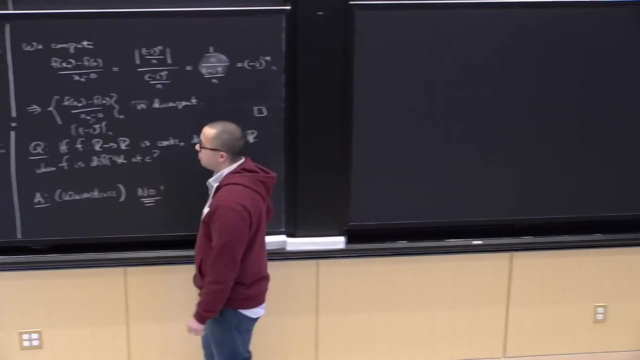 And Weierstrass, the godfather of analysis, said no. He came up with a whole class of examples of functions which are continuous on the real number line but are differentiable nowhere, And this was a really surprising set of examples. 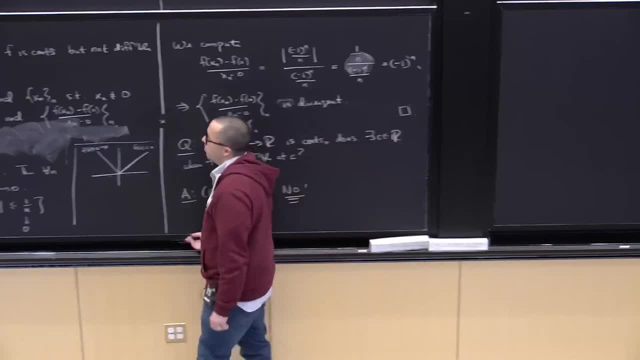 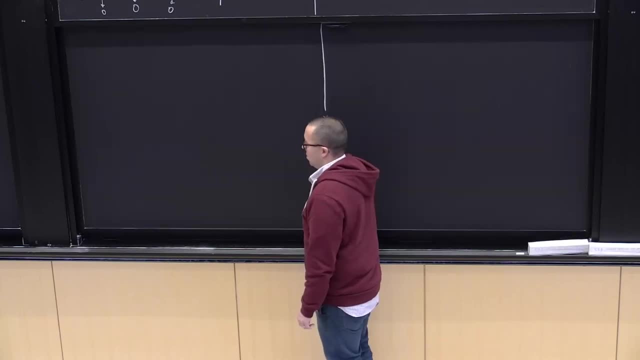 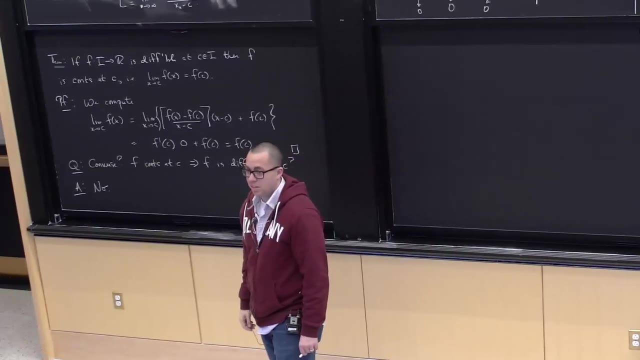 And what I found was that this is a really good example of how a continuous function can be used to generate a result to the community And to me. it's also one of the few results in this class that you really didn't see in your calculus class. 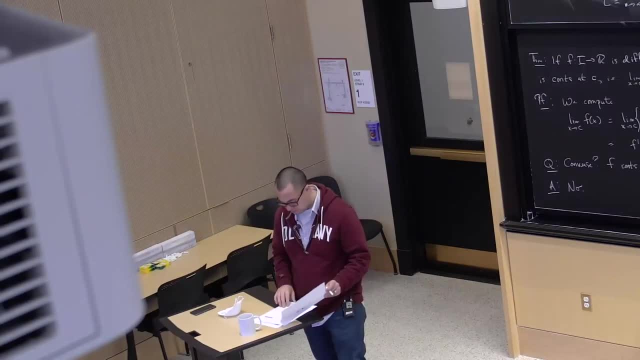 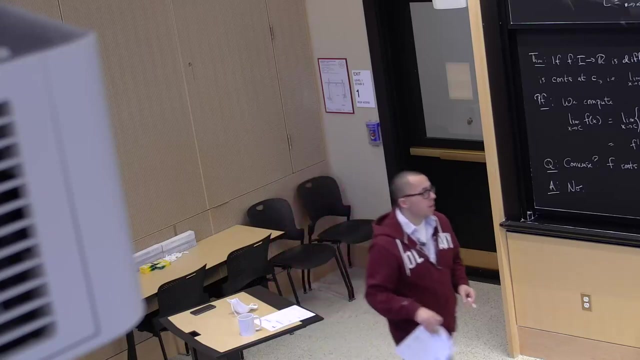 So we're going to go through this example, although in most analysis, classes, it's reserved for later, But I think we can do it now, And so what we're going to prove is: so we're going to construct a function which is continuous everywhere but is differentiable nowhere. 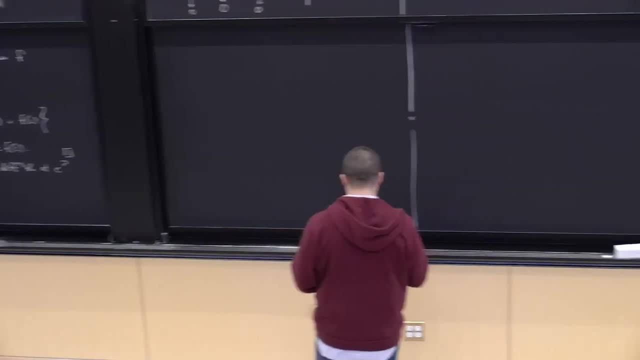 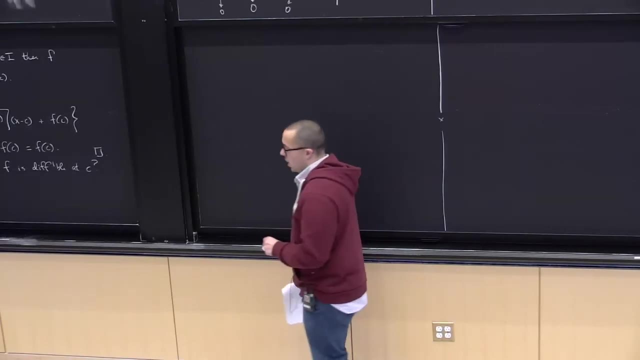 So a continuous, nowhere differentiable function, And I'll even write down. OK, I'm going to write down the function for you. So what's the idea that Weierstrass had? It was, let me, well, I'm not going to write down. 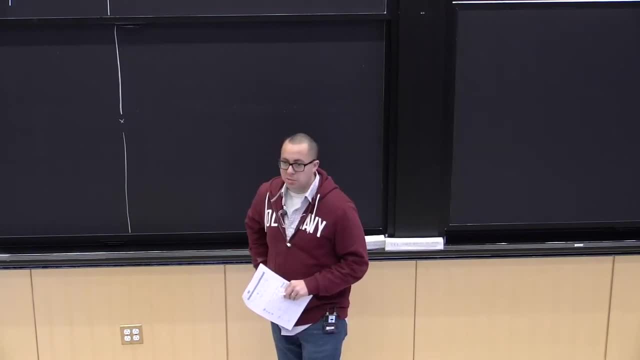 the function just yet. But the idea of constructing such a function is that it should be highly oscillatory. OK, You know. imagine again you're trying to draw a picture of the graph of a function that's nowhere differentiable. You would kind of sit there and break your pencil trying. 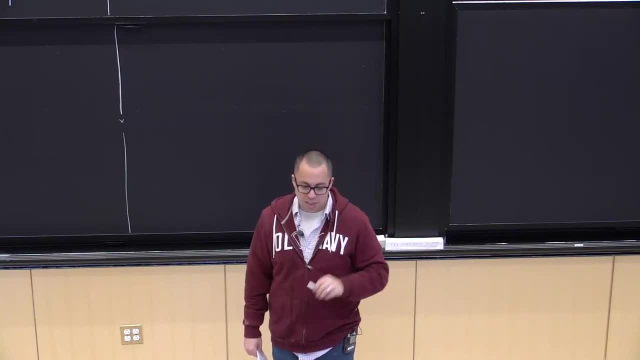 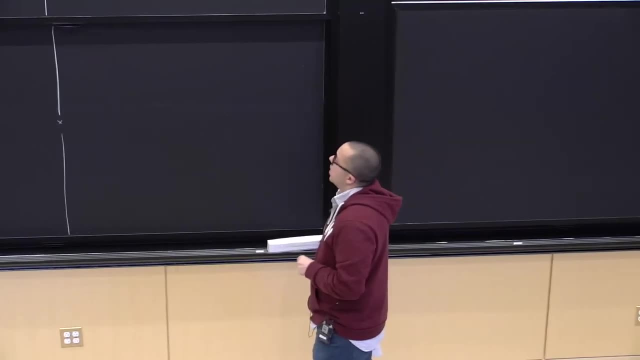 to draw just kind of a highly oscillatory function. OK, I'm not going to write down the function just yet. I'm going to write down the function just so that it never has a tangent. And that's his idea is to build a function which 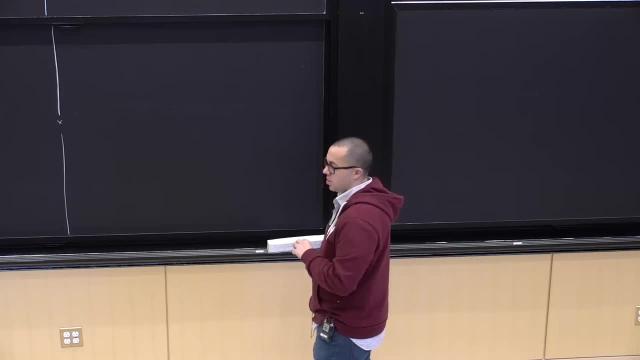 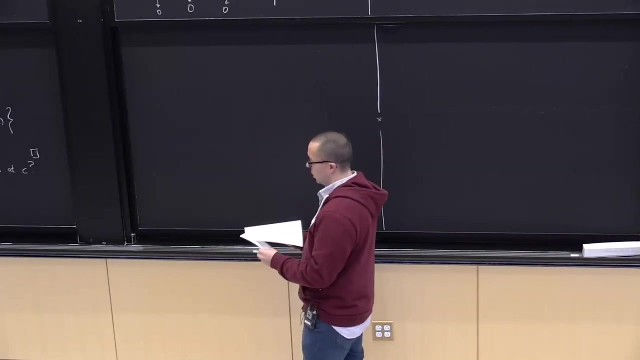 is highly oscillatory, but not too oscillatory, so that it's still continuous at every point. OK, So to start with the construction of this function, which is continuous but nowhere differentiable, we're going to need a few simple facts to start off with. 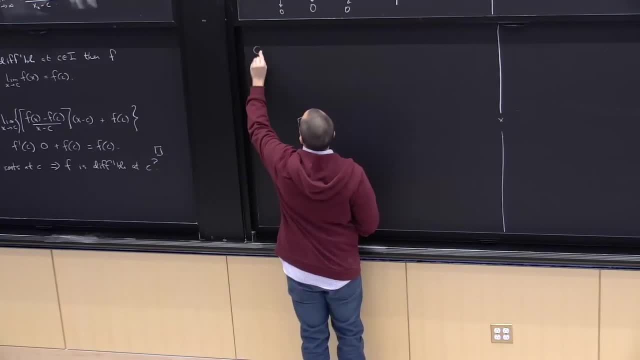 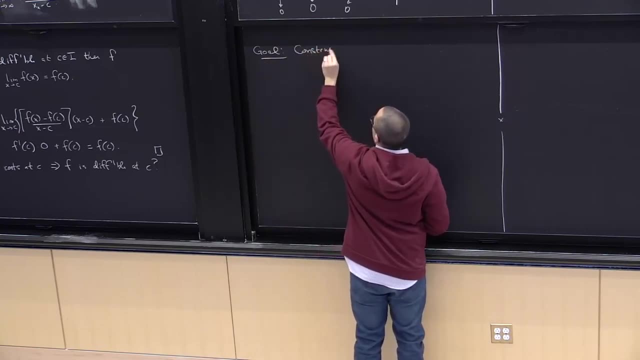 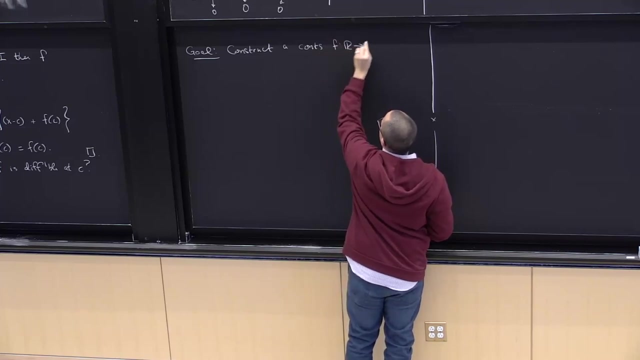 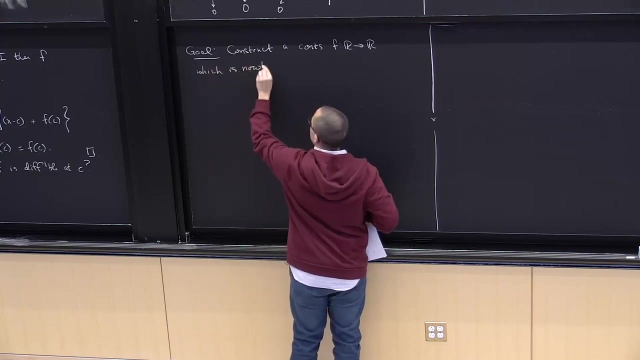 So what is? So? again, we're going to need a few simple facts to start off with. So what is? Again? let me write out and state our goal. We're going to construct a continuous function from r to r, which is nowhere differentiable. 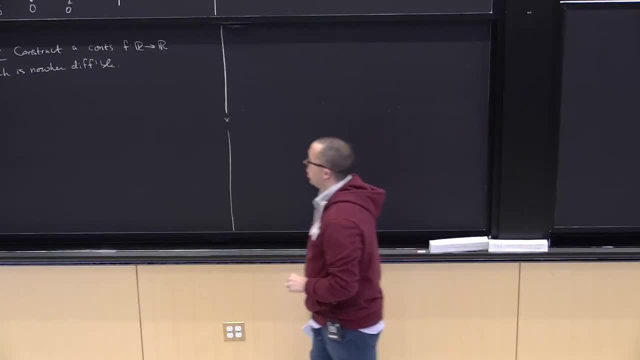 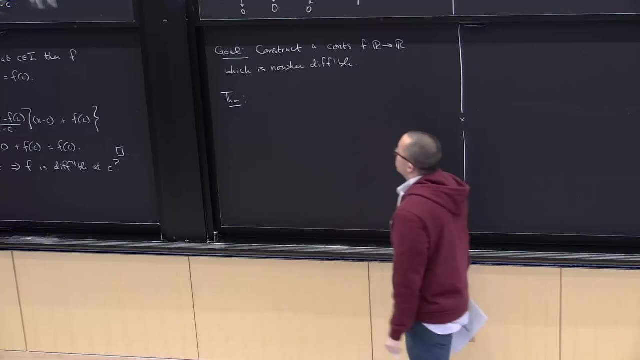 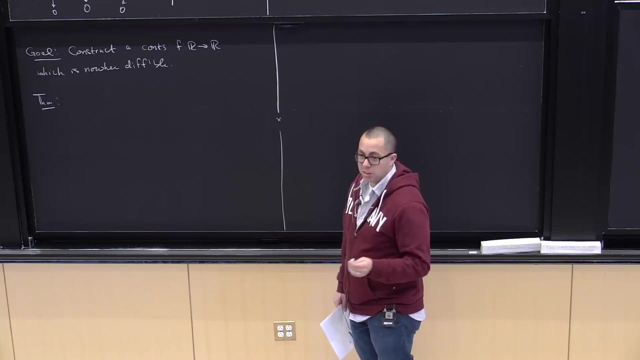 A not differentiable. It's differentiable at no point. OK, So let's start off with a few simple facts about so. I said that we're going to build a function which is oscillating quite a lot. There's two functions, you know that: oscillate cosine and sine. 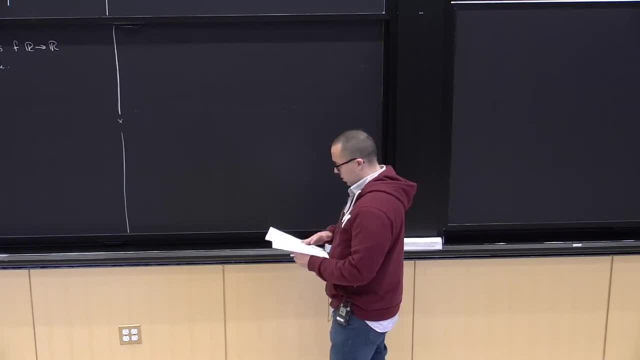 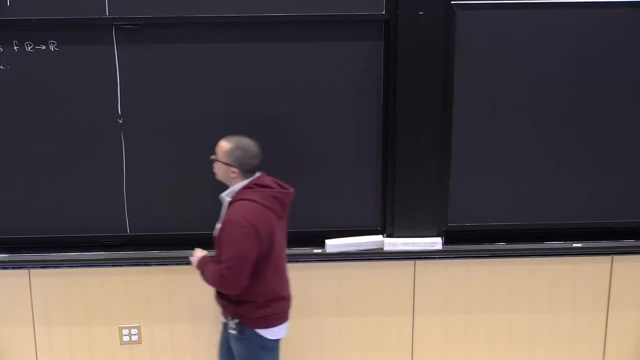 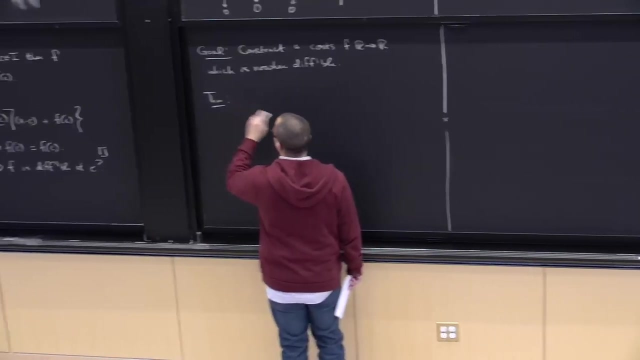 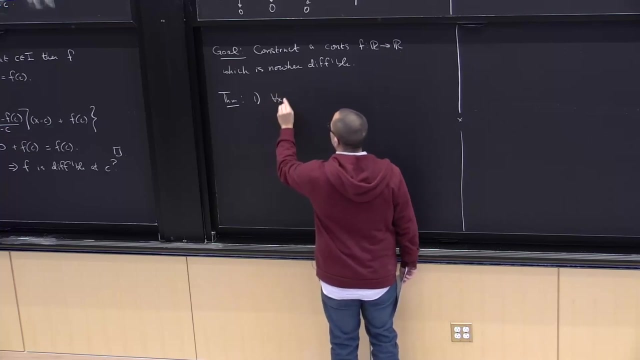 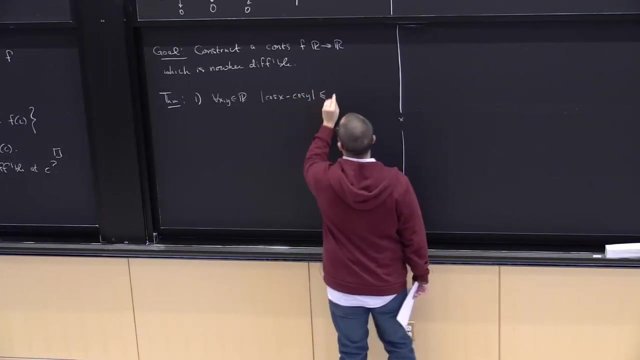 That's Those are going to be our building blocks. We'll choose one of them. Let's choose cosine, say, as to be our building block, But anyway. so let's start off with some elementary facts about cosine. So first is that for all, x, y and r, cosine x minus cosine y. 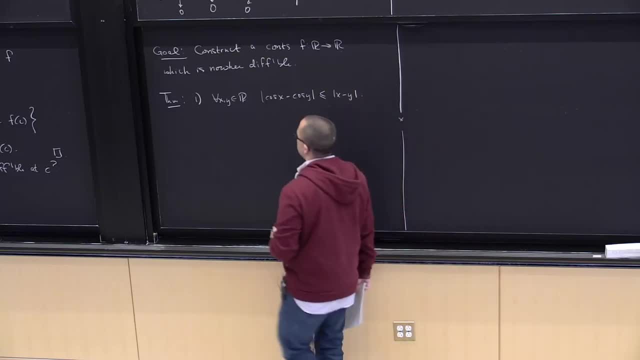 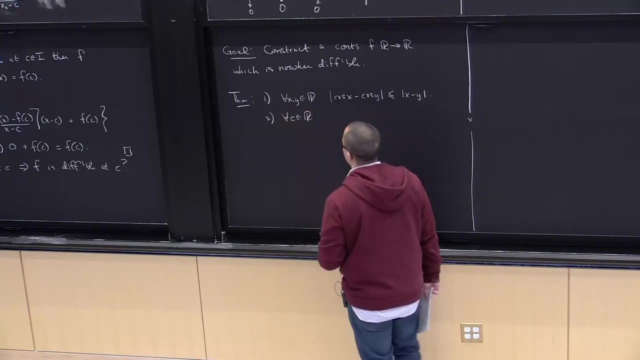 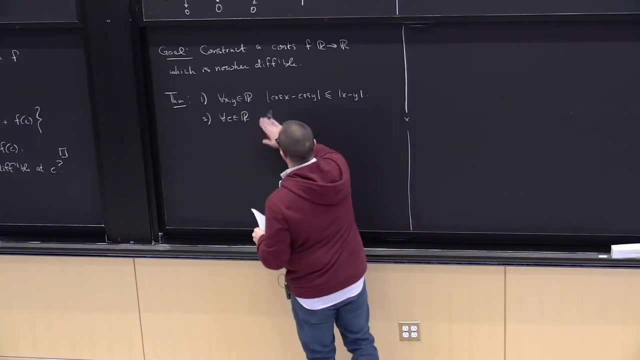 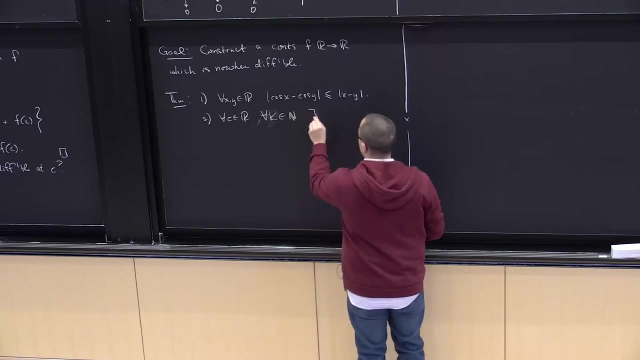 is less than or equal to the absolute value of x times x minus y. OK, And the second is that for every real number, c, and for all k natural number, there exists a y in c plus pi over k c plus 3. 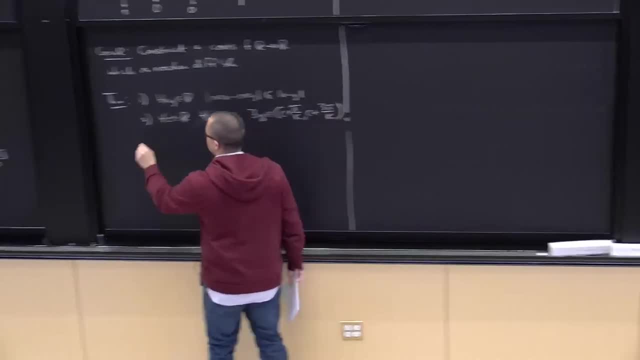 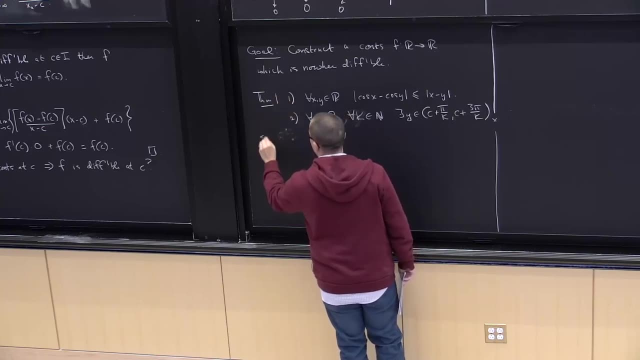 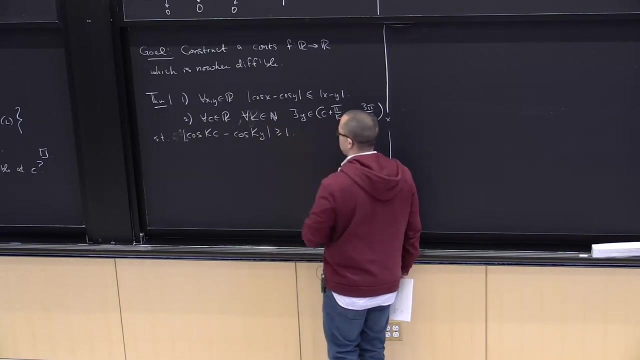 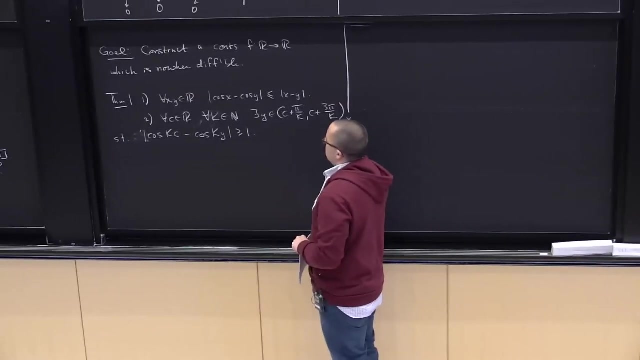 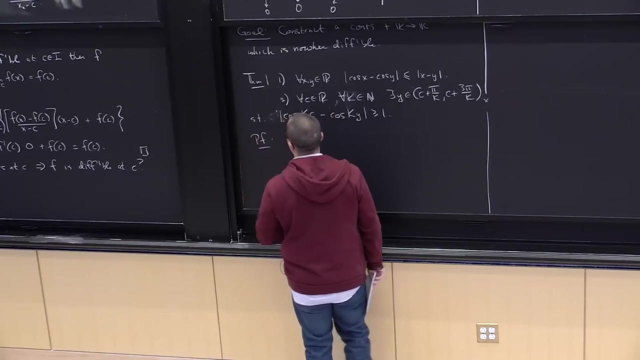 pi over k, Such that- and let me label this as theorem- one such that cosine of kc- that's funny- minus cosine of ky is greater than or equal to 1.. OK, All right, So both of these are simple facts about cosine. 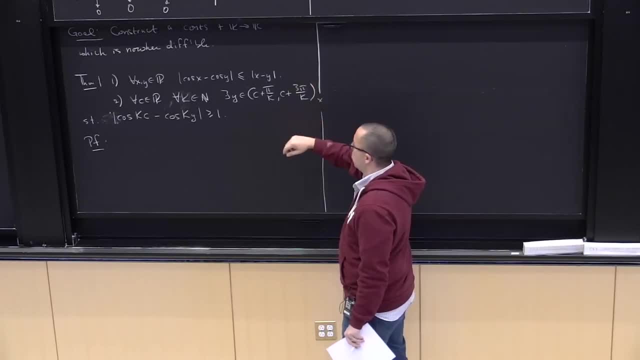 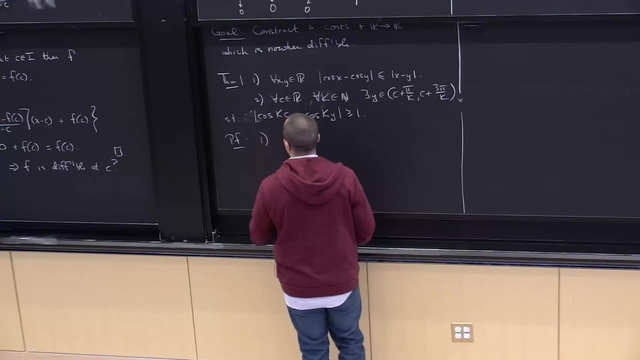 Really, this one just follows from the angle sum formula. This one follows from the periodicity of cosine. So why are these true? So, first off, we did prove, and maybe I should have used sine instead of cosine in all of this. 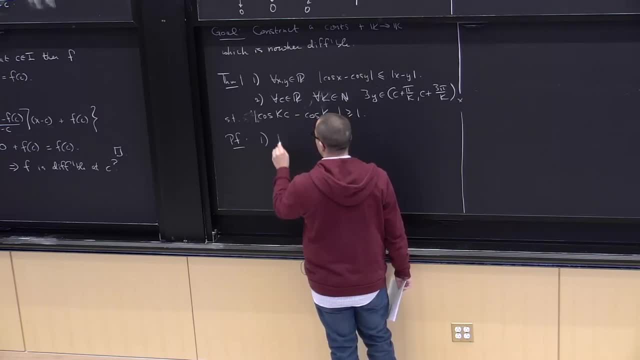 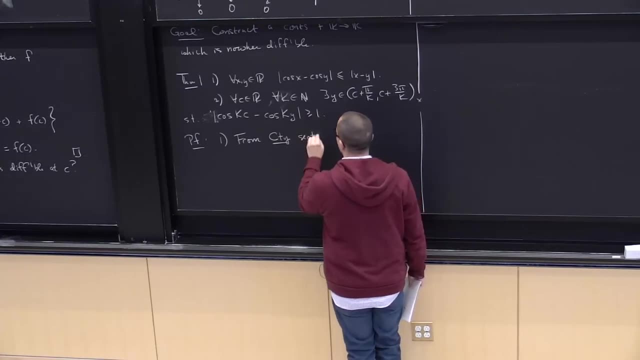 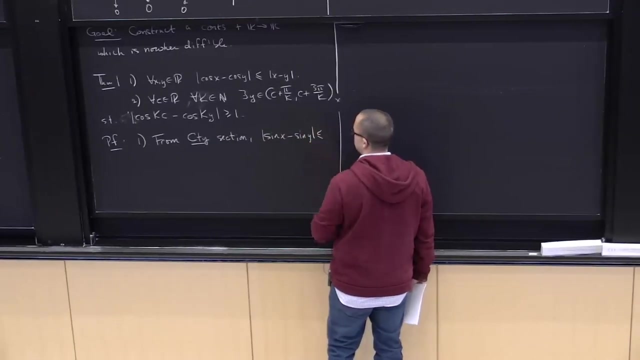 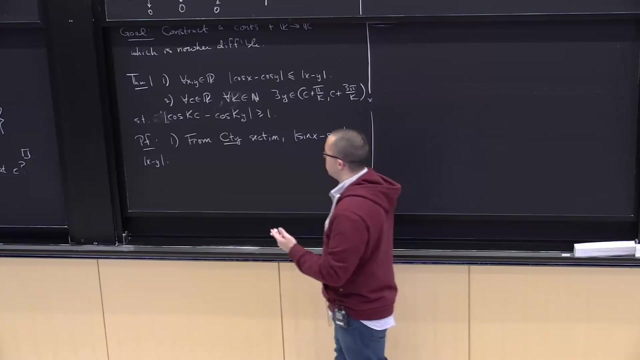 but if you recall From our continuity section, we proved that for all x and y, sine x minus sine y is less than or equal to the absolute value of x minus y For all x and y. OK, And there is a simple relation between cosine x. 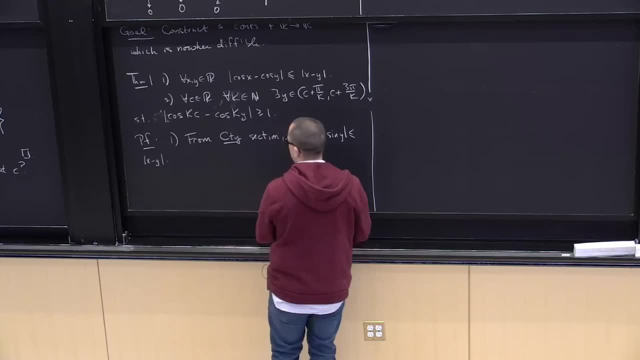 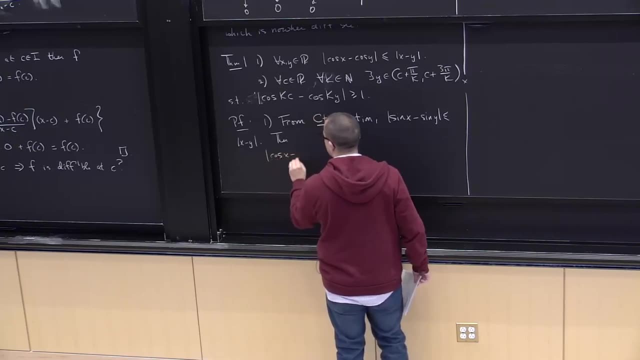 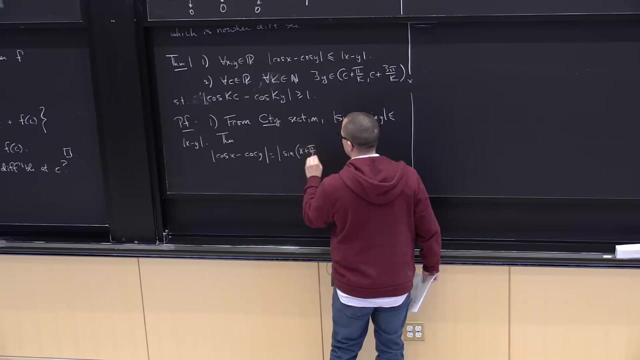 and sine of something, And that's just a shift by pi over 2.. Then, OK, So So Then, cosine of x minus cosine of y, This is equal to sine x plus pi over 2, minus sine y plus pi over 2.. 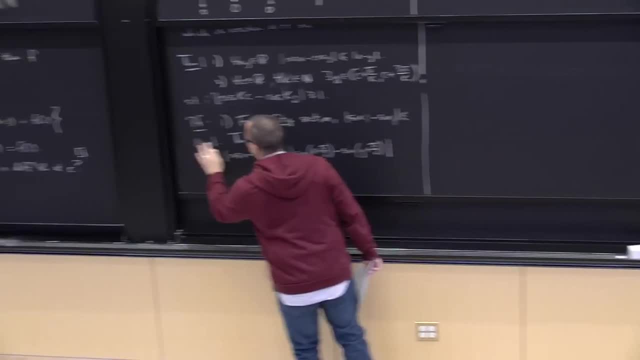 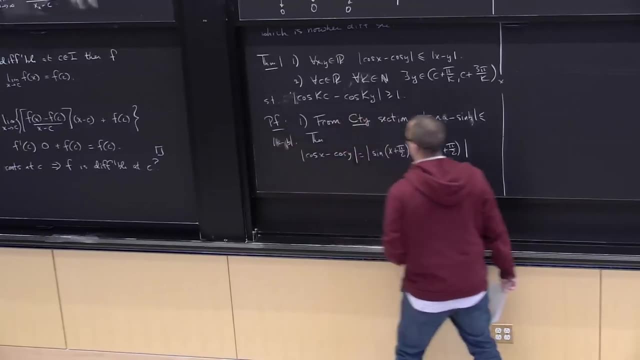 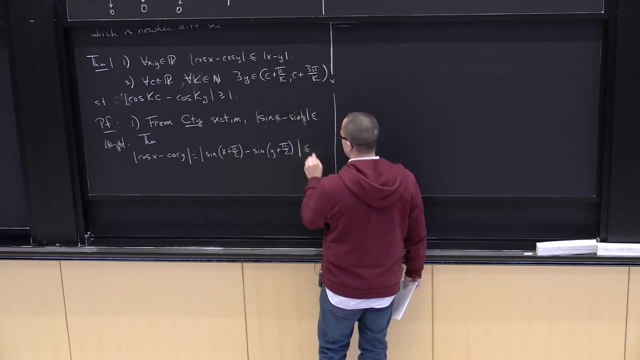 And, if you like, let me, instead of using x and y here, let me use a and b. So then this is less than or equal to. Then this is less than or equal to: x plus pi over 2, minus y plus pi over 2. using this inequality, 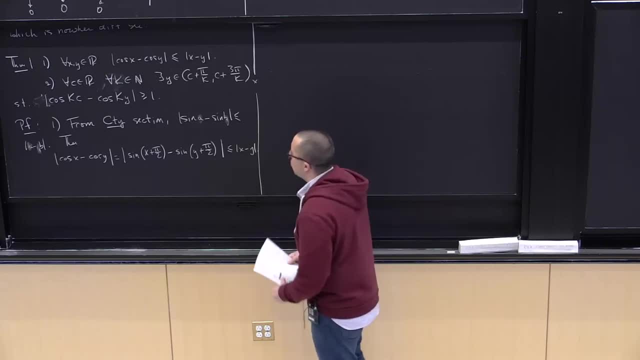 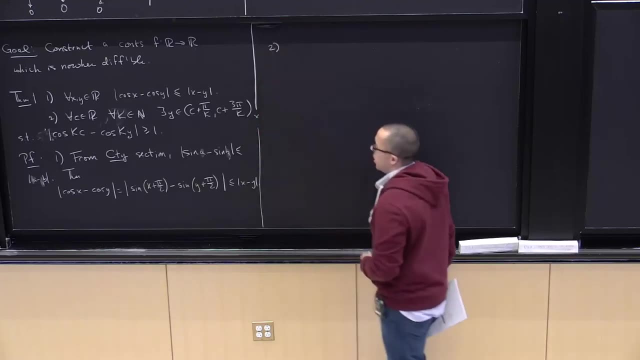 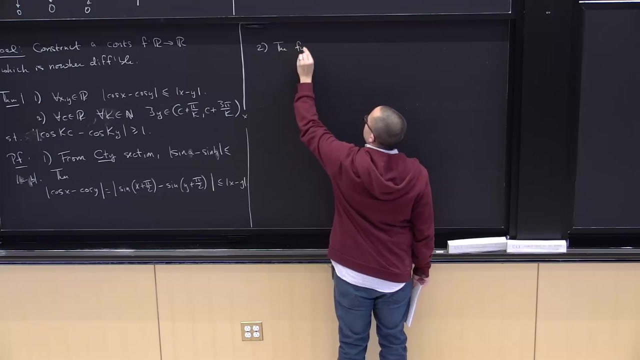 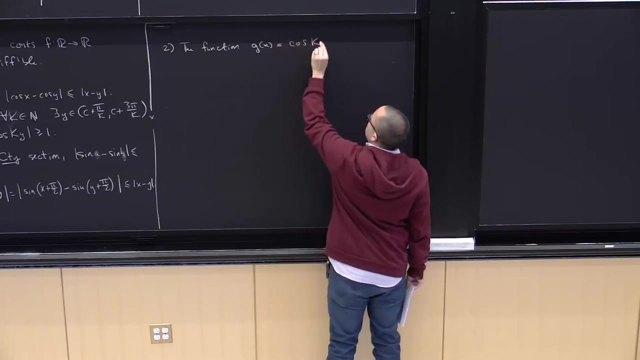 OK, So that proves number one. For number two, it's just a simple fact about cosine being 2, pi periodic. So So Function g of x equals cosine k of x. This is also periodic. But now what's the period? 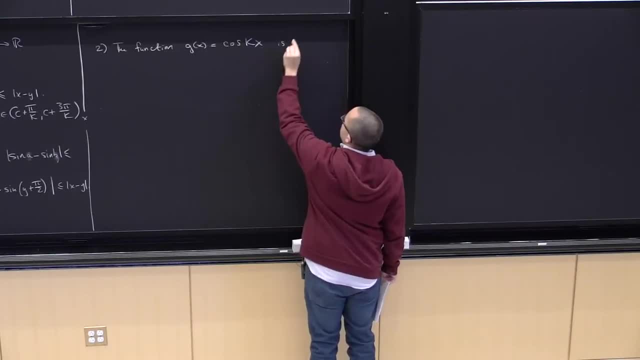 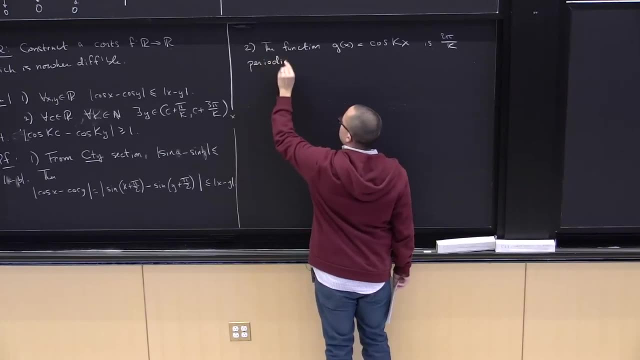 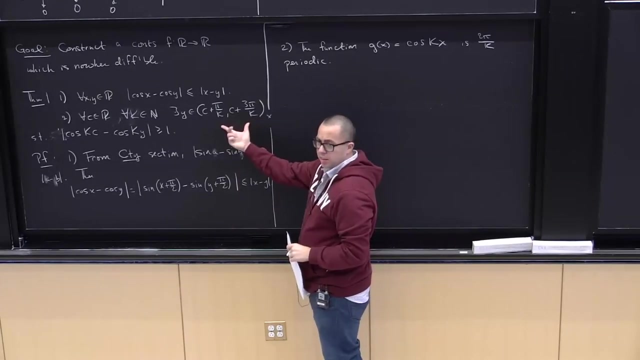 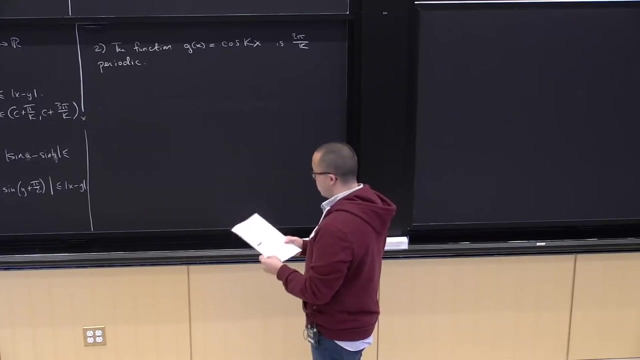 It's 2 pi over k. OK, And now this interval has length: 2 pi, Except it's missing the point c plus pi over 2. And c plus 3 pi over k, All right. Thus, if I look at, 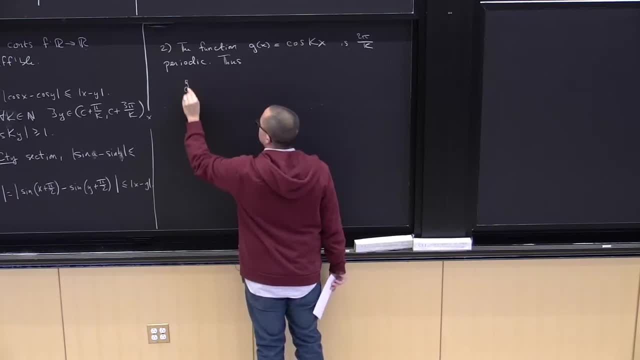 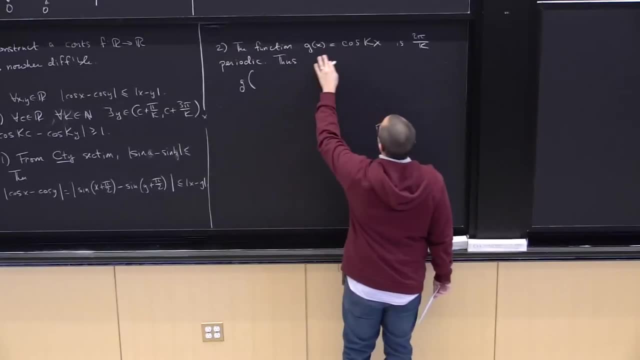 If I look at the image of The interval Of x Between This C, Then so this function g of x equals cosine k of x. if I look at The image of this interval, So this function g of x equals cosine k of x. if I look at: 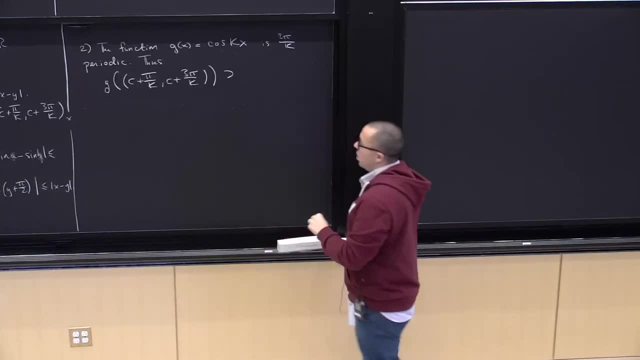 This will contain, You know, All of the real numbers between minus 1 and b. So So This interval, This will contain, You know, 1 and 1, OK, So this is a interval of length, 2 pi over k. 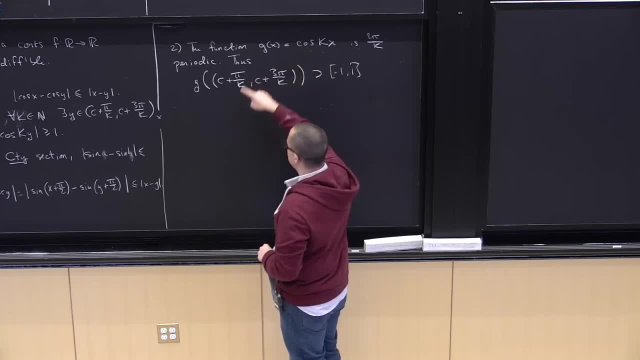 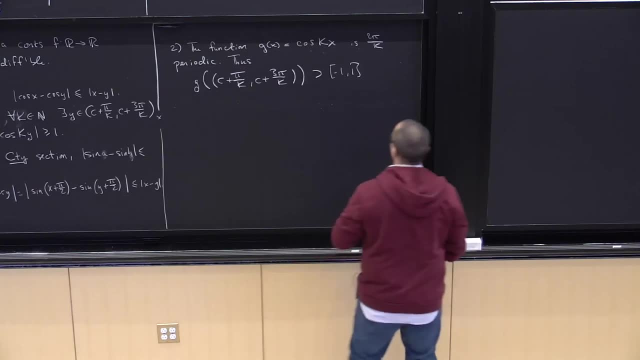 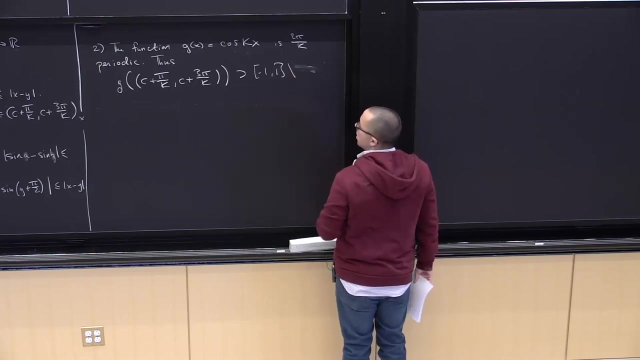 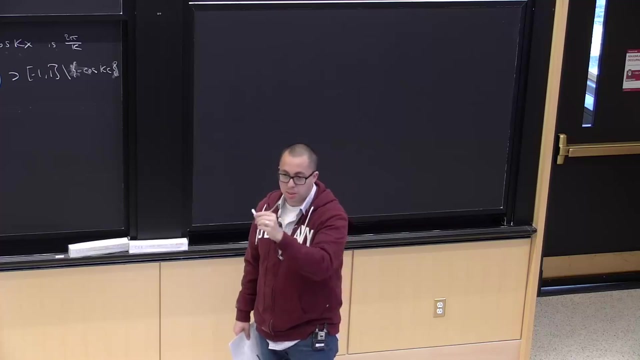 Cosine kx is 2 pi over k periodic, so I should get everything between minus 1 and 1, except possibly the value at the endpoints. So take away, And the value at the endpoints is minus cosine kc. OK, Because cosine of k times c plus pi is equal to pi over k. 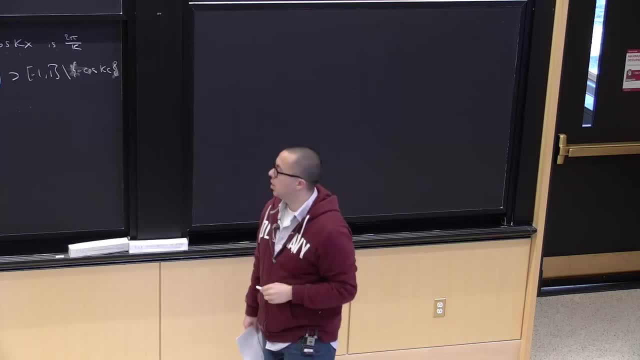 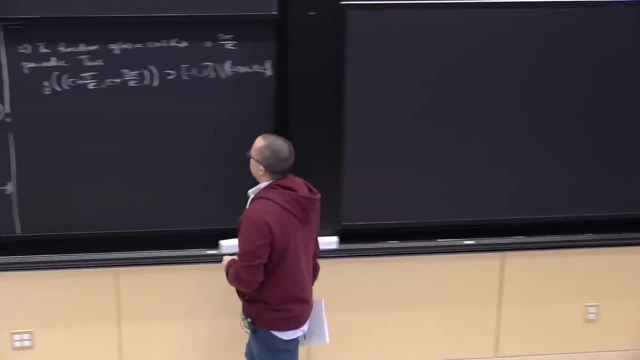 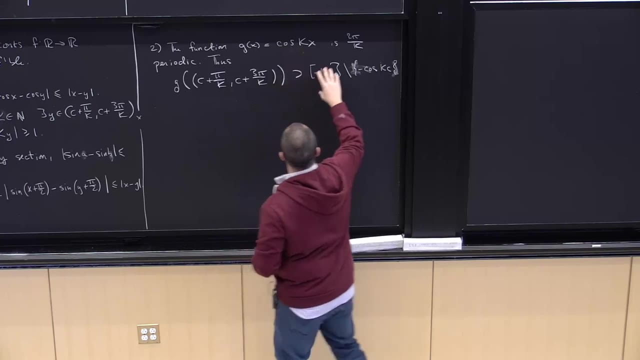 is equal to cosine of kc plus pi, And cosine of something plus pi is equal to minus cosine of that. That's it. That's the thing. OK, All right. so the image of this set by cosine kx contains everything between minus 1 and 1,. 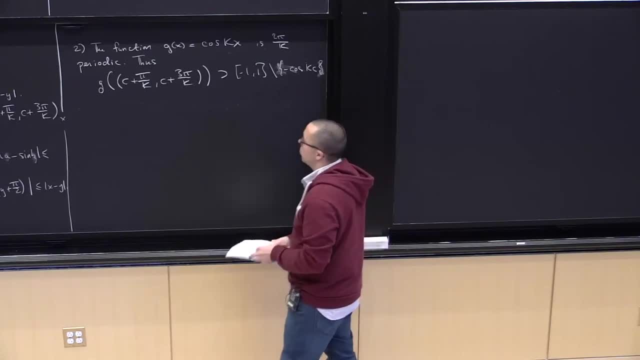 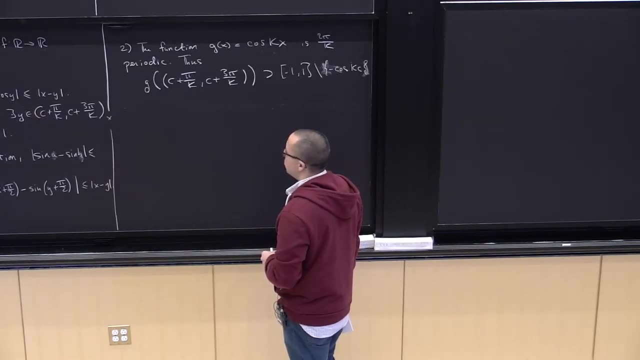 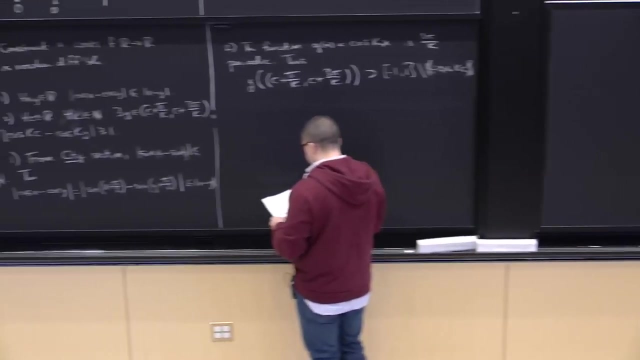 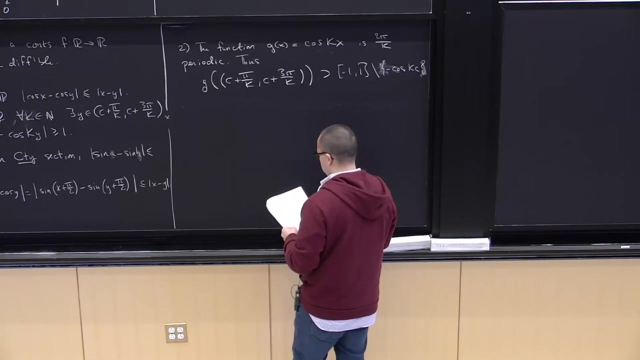 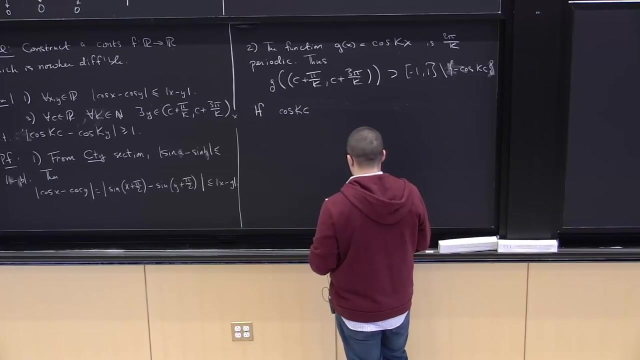 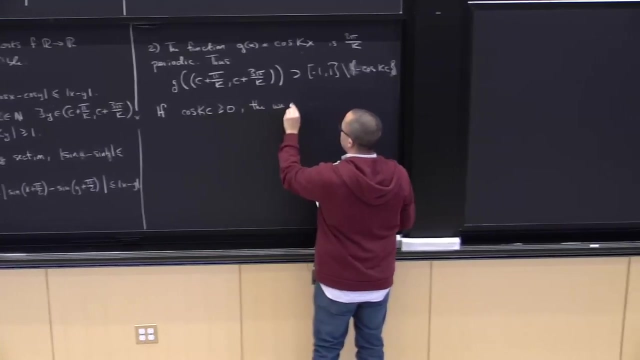 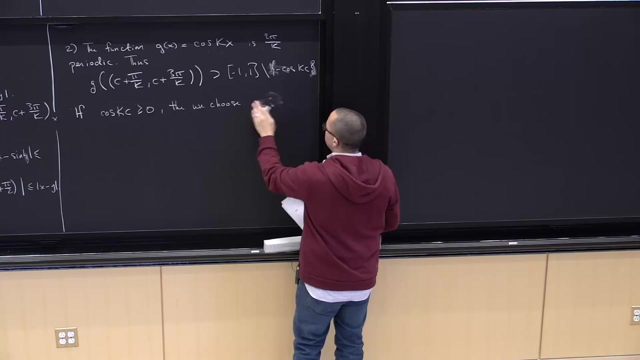 except for, possibly, the endpoint. This really only happens if cosine of k times c equals 1.. So OK then, if cosine of kc is bigger than or equal to 1, or equal to 0,, then we choose y in this interval, c plus pi. 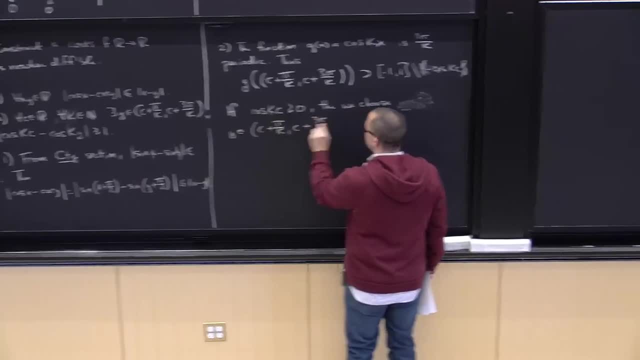 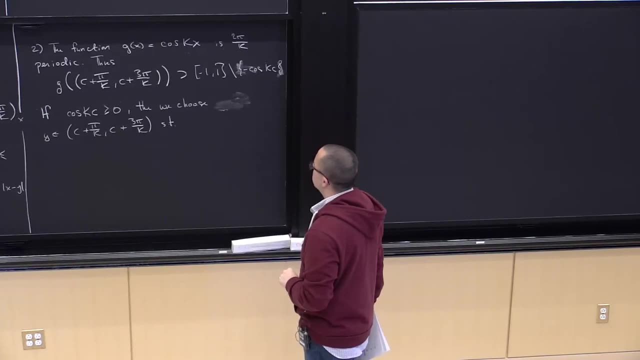 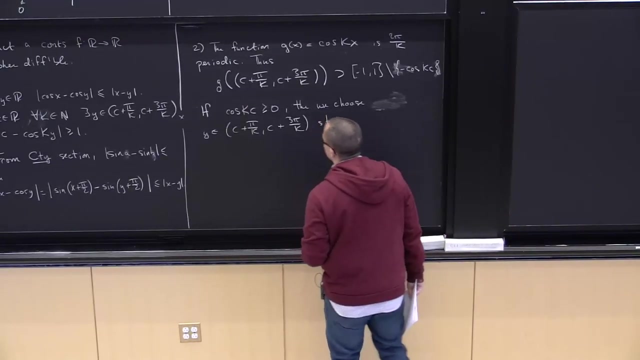 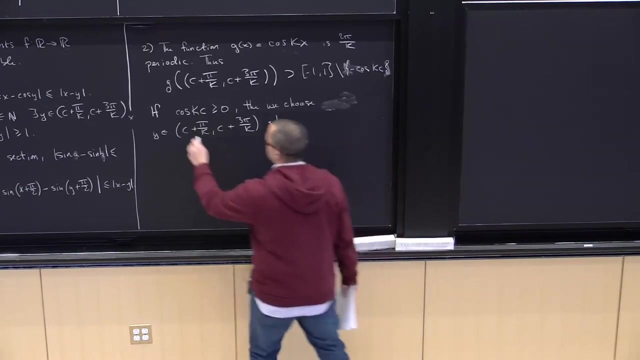 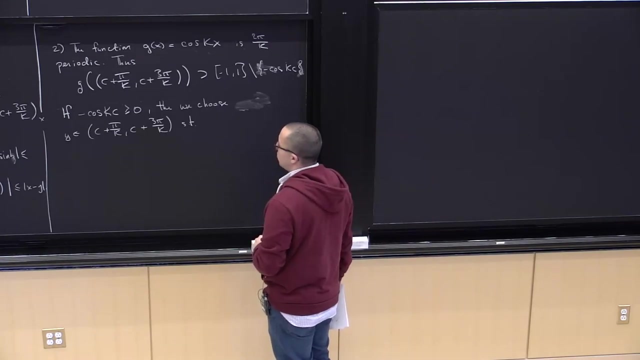 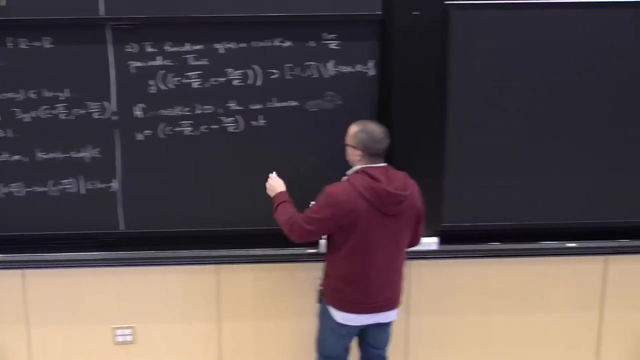 over k, c plus 3 pi over k. OK, Let's write it this way. So if this thing is bigger than or equal to 0, then we choose y. Why am I confusing myself? So this is simple enough. We choose y in this interval, so that cosine of ky E. 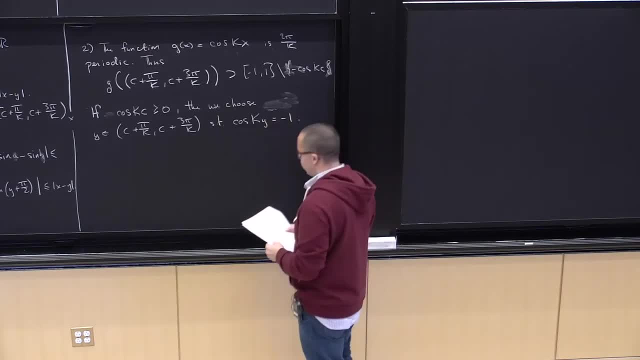 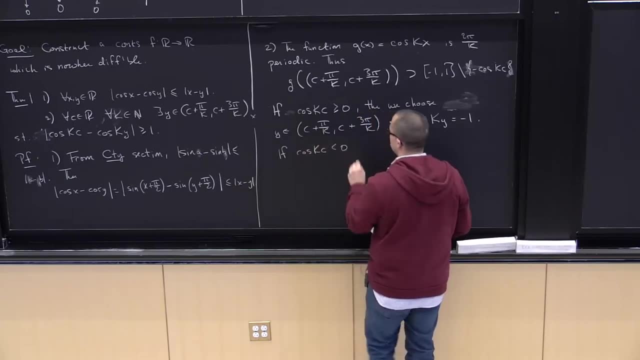 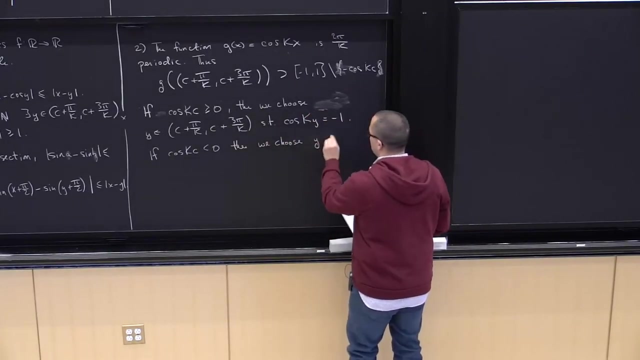 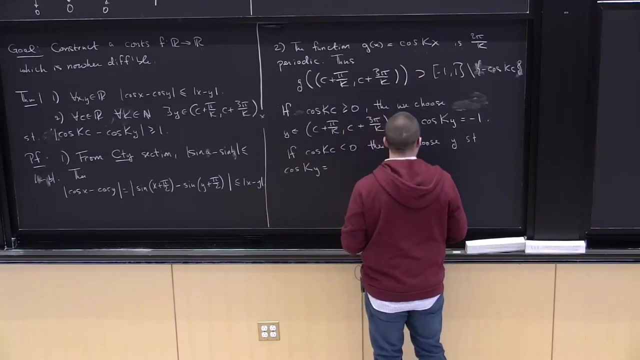 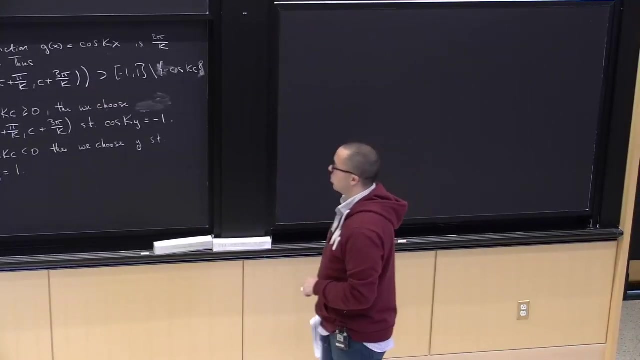 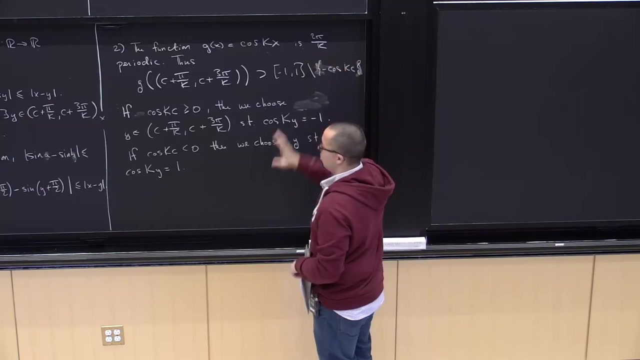 will be positive. OK, equals minus 1, and if cosine kc is less than 0,, then we choose y, so that cosine of ky equals 1.. So again, just to get an idea. so I'm quibbling over a minor point. 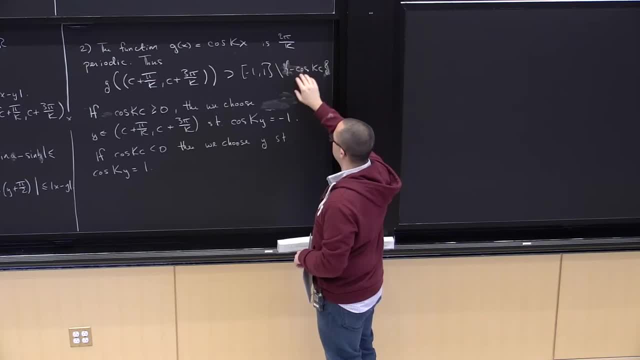 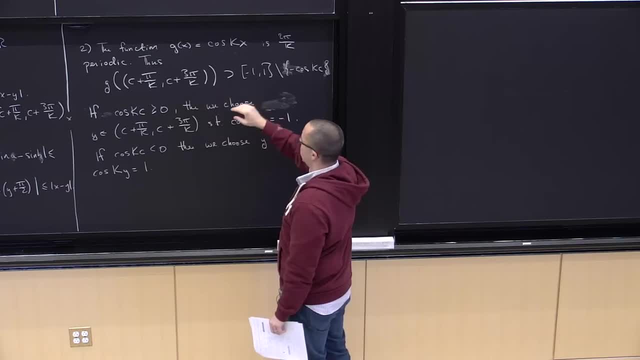 Let's erase this for a minute, and let's imagine that the value of cosine kc is less than 1.. Let's erase this for a minute, and let's imagine that the value of cosine kc is less than 1.. this guy, I mean, it's a 2 pi over k periodic interval, you know so. 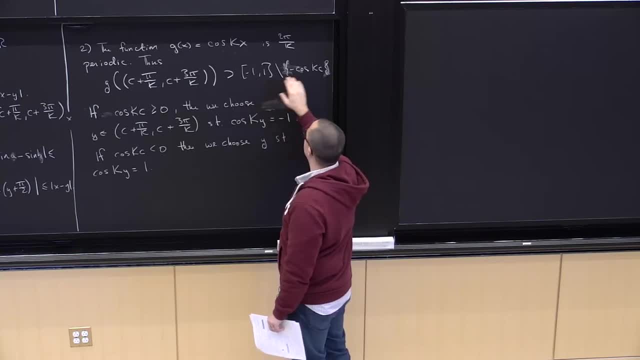 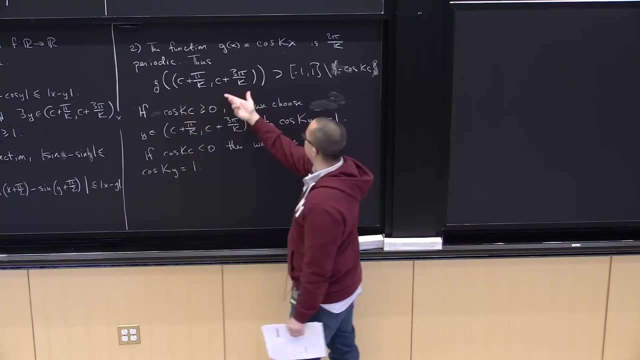 this should basically cover all values between minus 1 and 1.. So cosine of kc will either be plus or minus. so if it's non-negative, then I can find a y in this interval, since it's 2 pi over k periodic. so 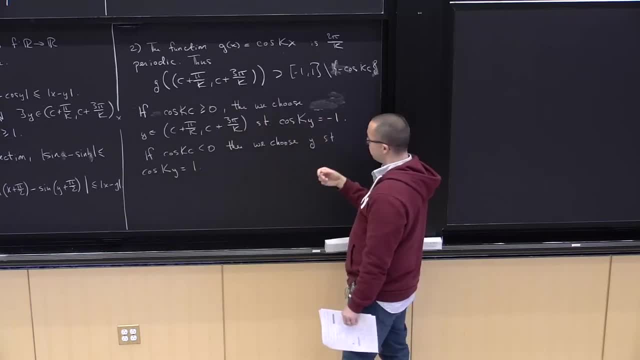 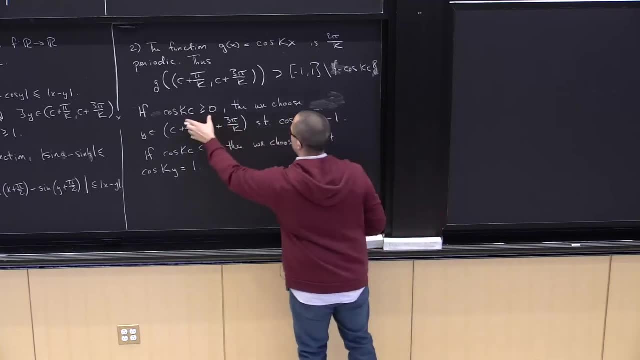 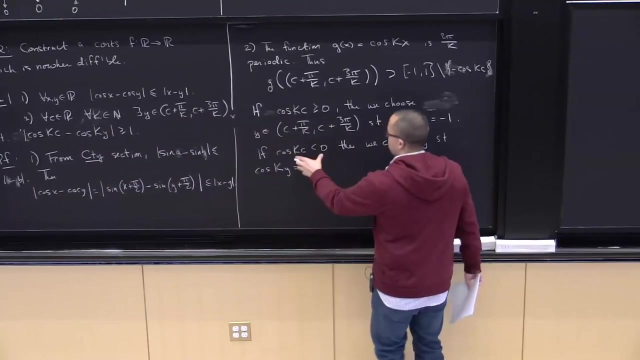 that cosine of ky equals minus 1, okay, And since this is non-negative, and this is equal to minus 1, the difference between these two in absolute value will be greater than or equal to 1, okay. Now, if cosine of kc is less than 0, then again. 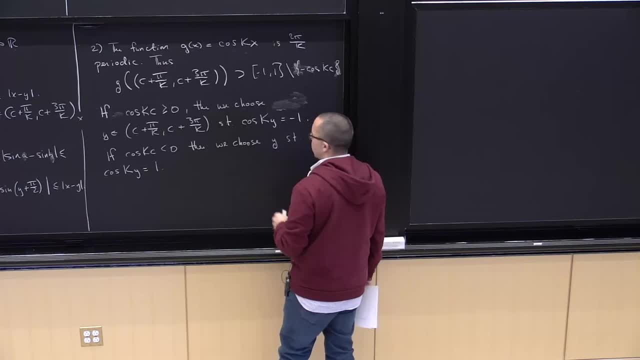 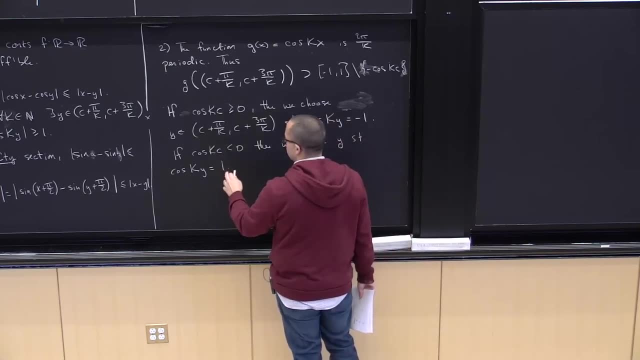 since this interval contains minus 1 to 1, it's 2 pi over k. periodic. we choose a y, so that cosine of ky equals 1.. And then this is negative. this is 1, so the difference between something negative and 1 is greater than or equal to 1,. all right, 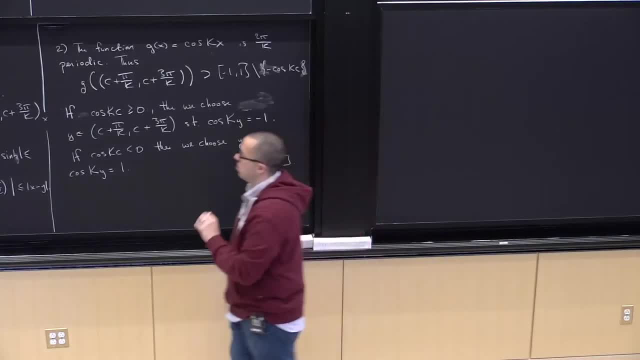 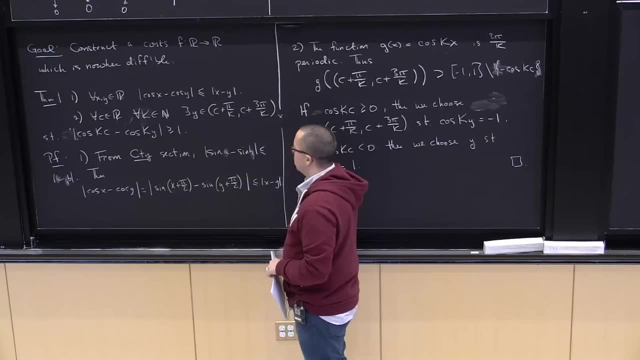 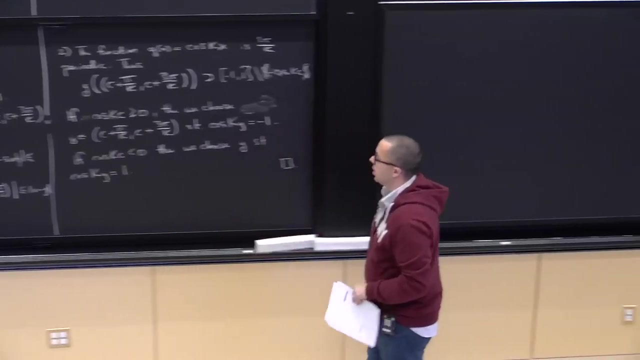 And that's the proof. I made a kind of a mess of it, but this is, you know, very easy to understand if you just, you know, draw a picture, really, okay, All right, so let's take, so let's continue. 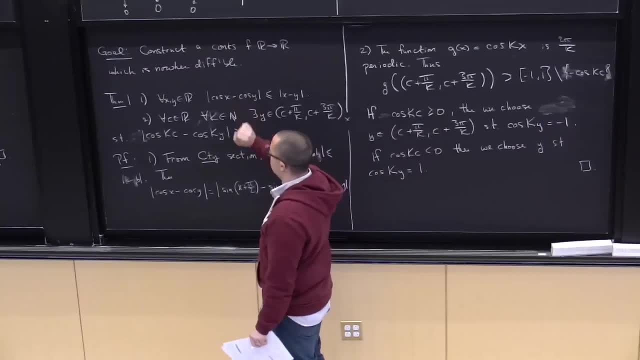 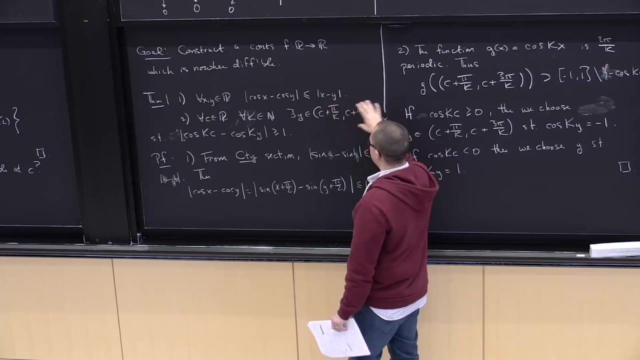 And again, what these two you know parts of this theorem say is that cosine of cosine can be quite oscillatory. if you, you know, insert a k here, right, Because you know the difference between this interval is actually. 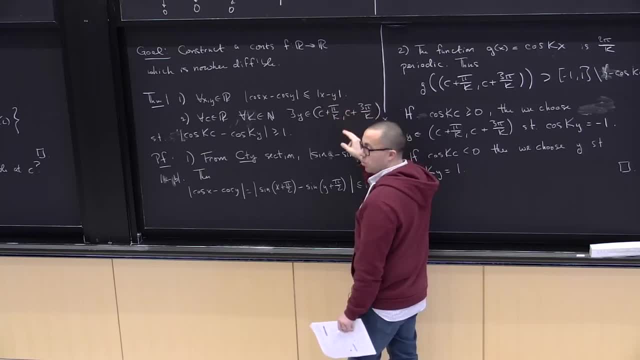 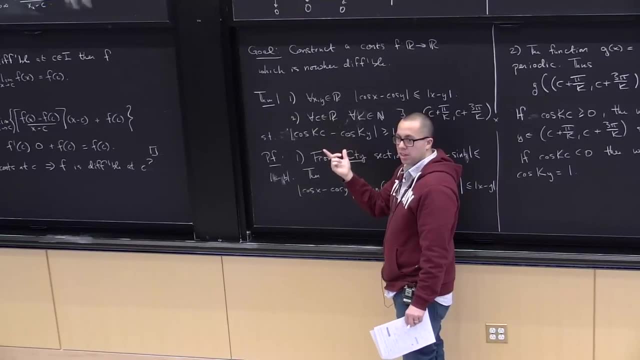 you know quite small right. The length of this interval is 2 pi over k. If k is very large, that's a very small interval. yet somehow we can find two points which differ by at least one in value if we plug them into the function. 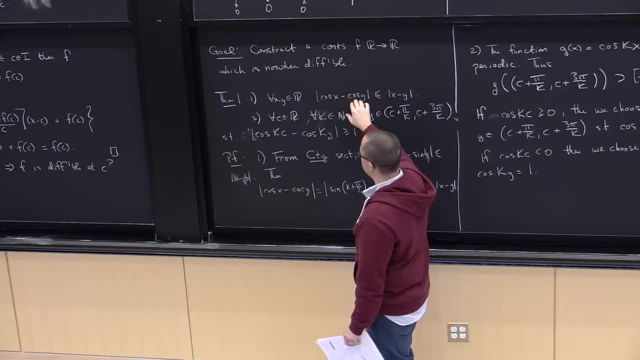 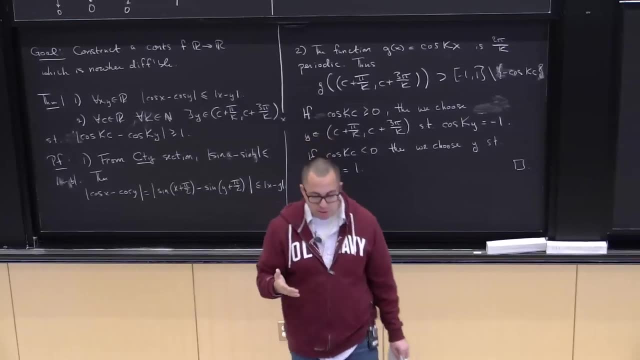 But cosine is not too wild because it satisfies this, this bound. so these two are kind of going to. they're going to be the ingredients in that. you know idea. I said at the start that we're going to build a function which oscillates. 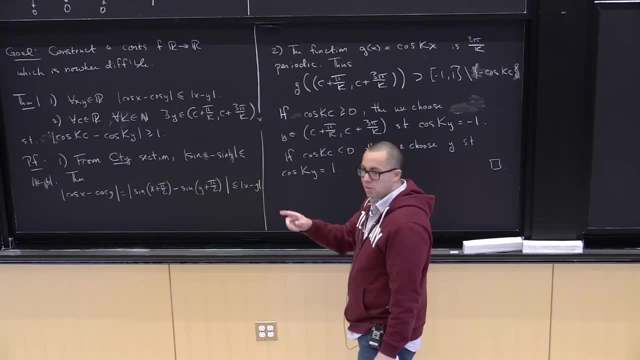 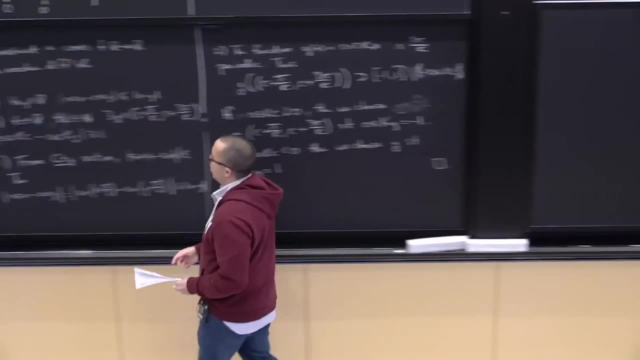 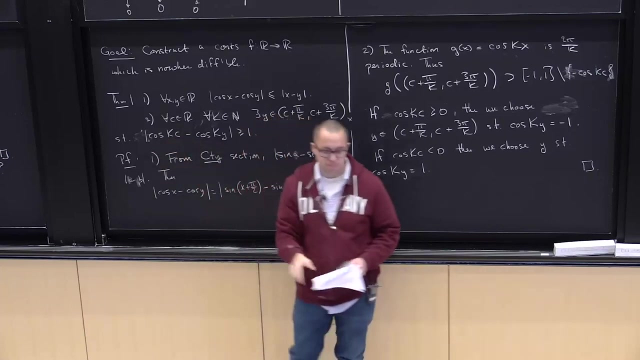 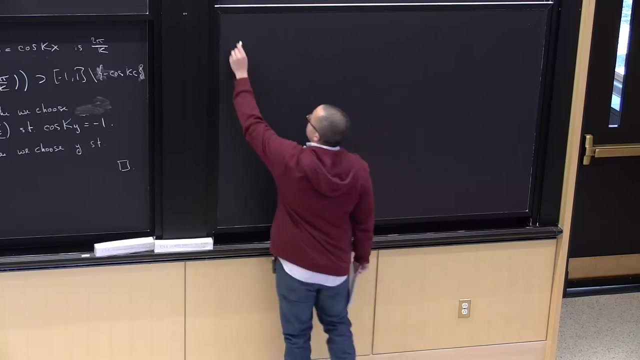 which is quite oscillatory, but it's not too oscillatory that it's still continuous, okay, And we're going to build our function out of cosine kx, where k is going to be changing, okay. So I'm going to need one more very simple fact, so this one, I won't mess up too much. 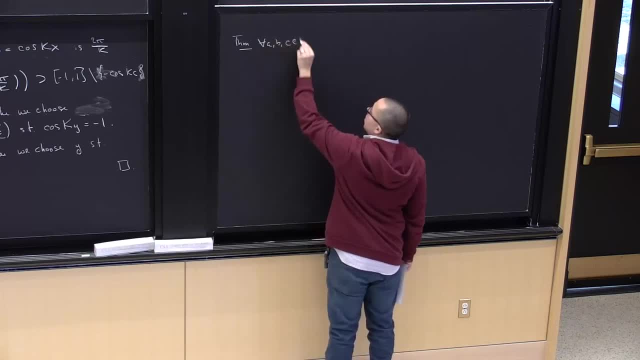 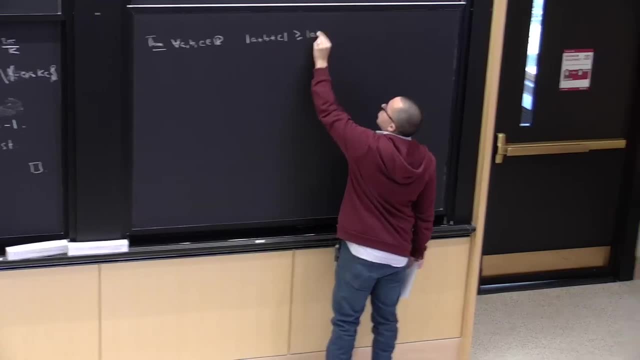 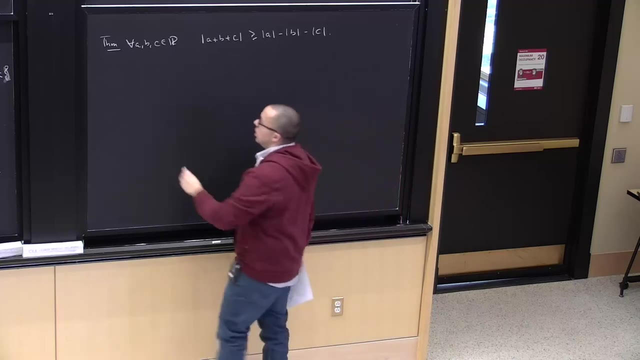 which is the following: for all a, b, c and r, the absolute value of a plus b plus c. This is bigger than, or equal to, the absolute value of a minus the absolute value of b minus the absolute value of c. okay, 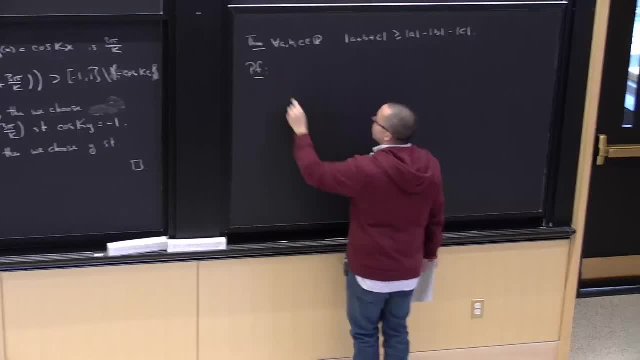 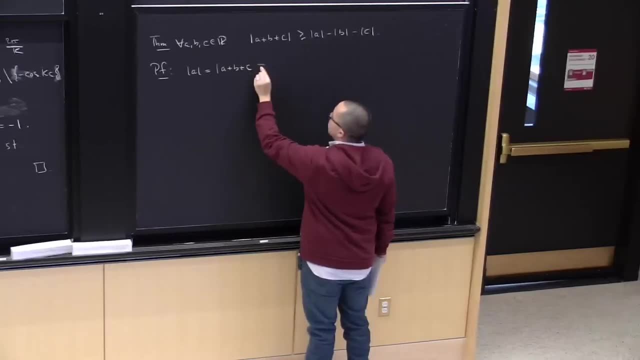 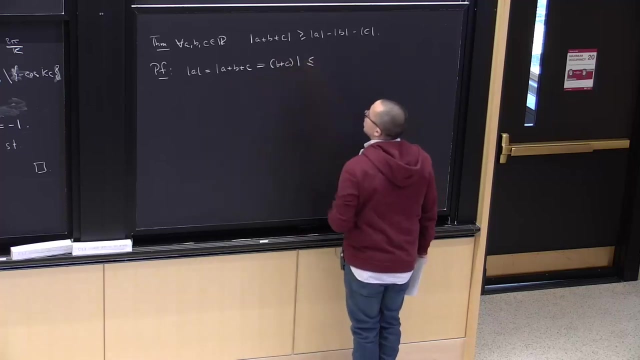 And the proof of this is just to use the triangle inequality tool. If we do that twice, we have the absolute value of a. this is equal to a plus b plus c, minus b plus c, and this is less than or equal to by the triangle inequality, the. 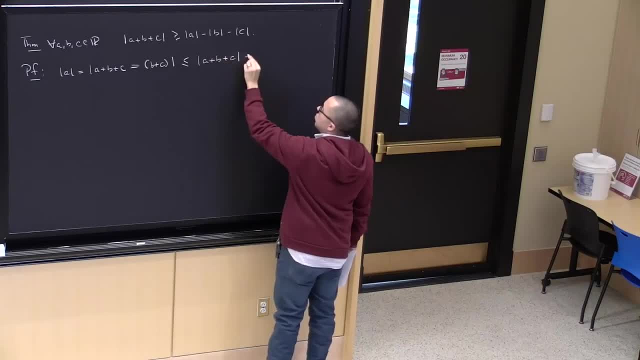 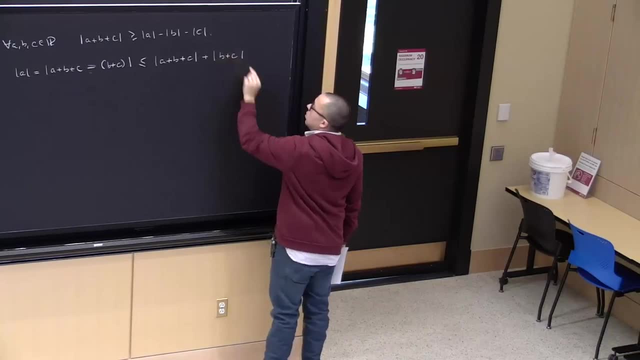 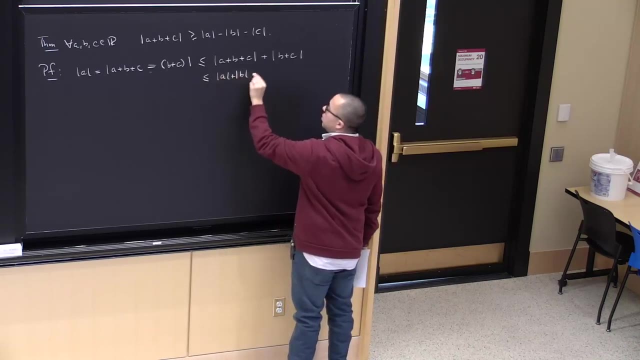 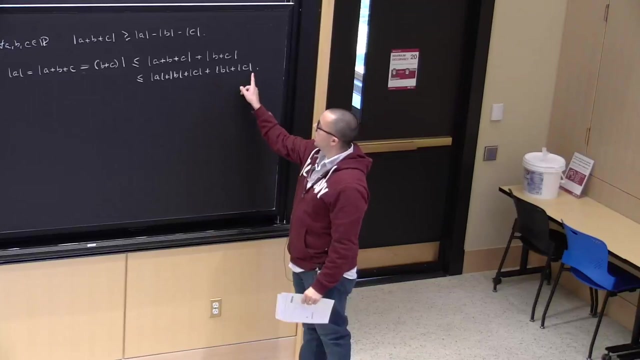 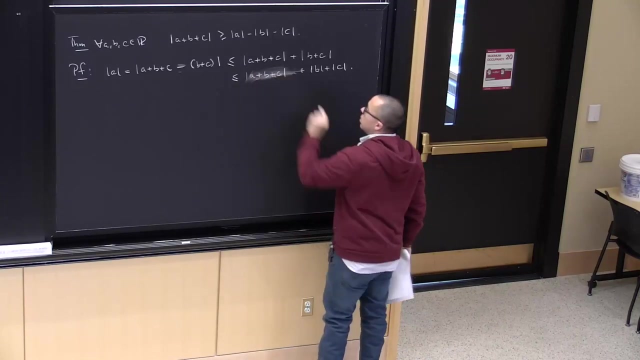 absolute value of a plus b plus c, plus the absolute value of minus times b plus c. but that minus goes away with the absolute value. And then I use the triangle inequality one more time here to get okay. And then if I subtract- oh, I didn't want to do that. 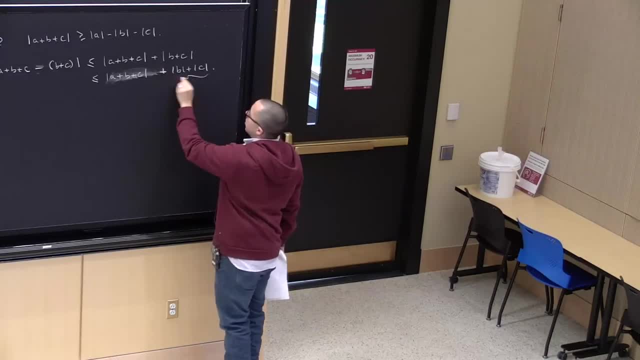 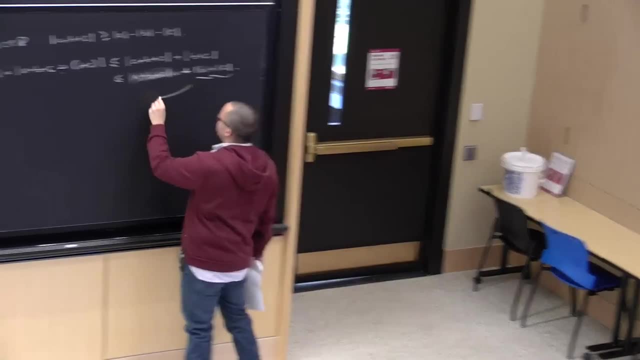 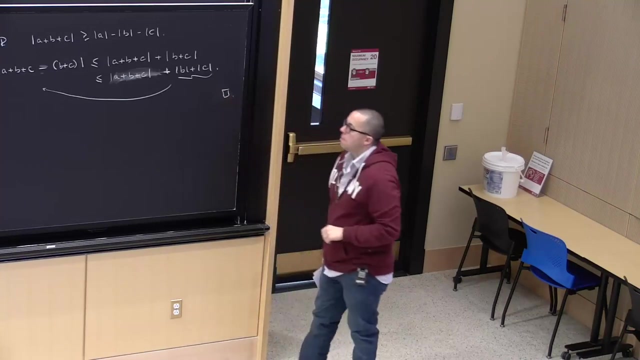 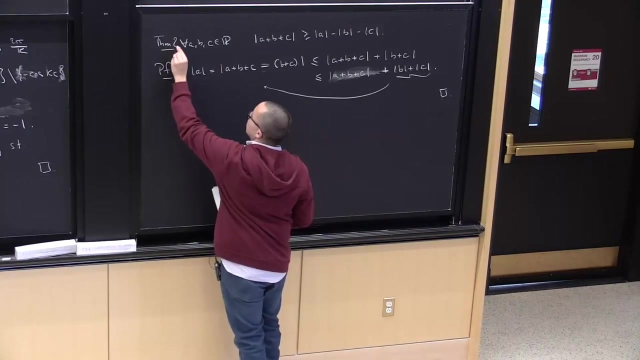 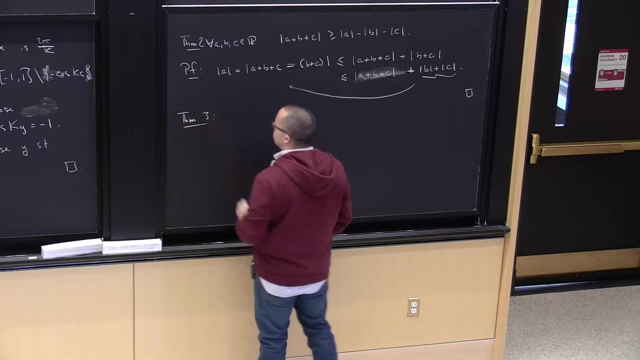 And so if I subtract this side over to the other side of this inequality, I get minus. okay, I get the statement of the theorem, All right. okay, so now we're gonna introduce: call this theorem two. Now let me introduce the guest of honor. 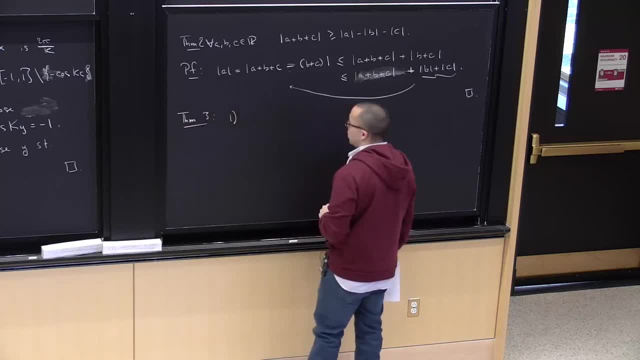 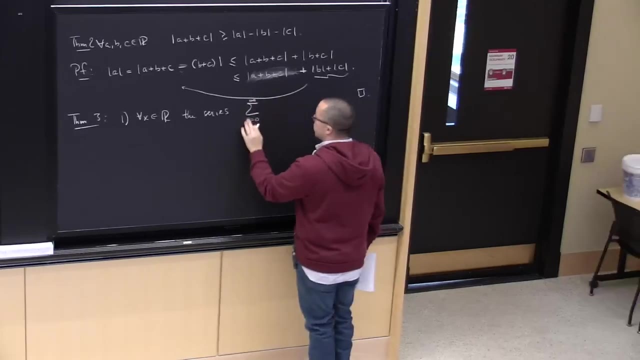 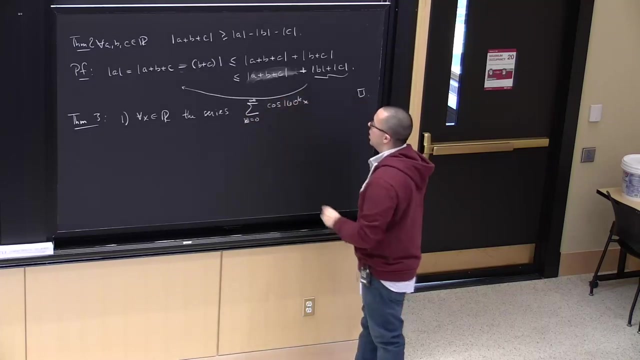 So first I have the following claim: for all x and r, The series given by sum from n equals 0 to infinity, And instead of n I'm gonna use k, cosine 160kx. So here's our very oscillatory guy over 4 to the k. 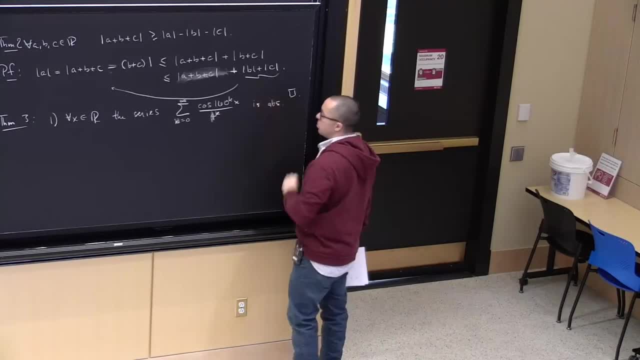 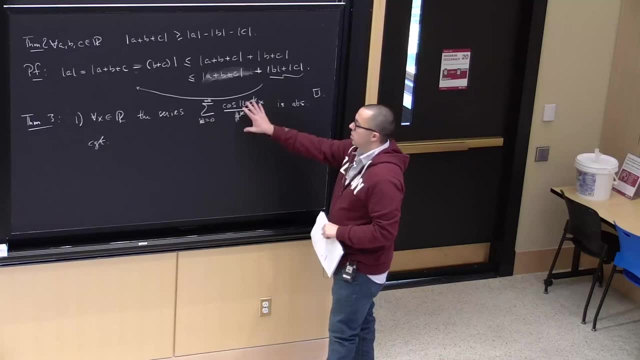 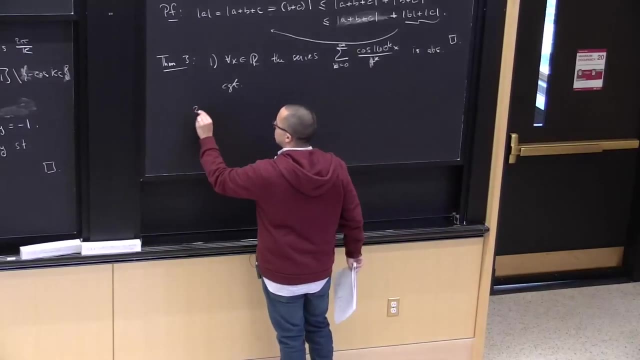 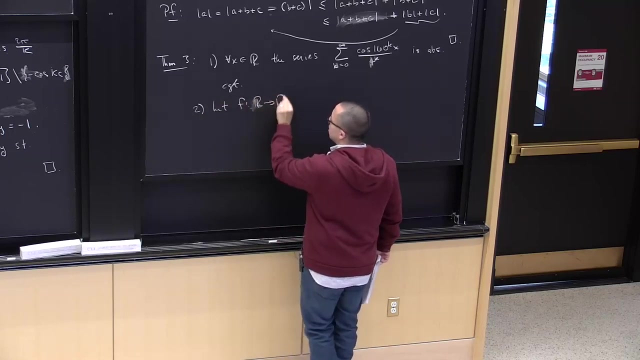 Is absolutely convergent, all right. So for each x and r, this series converges absolutely, so it spits out a real number. So I can define a function in terms of this series. Let f from r to r be defined by: 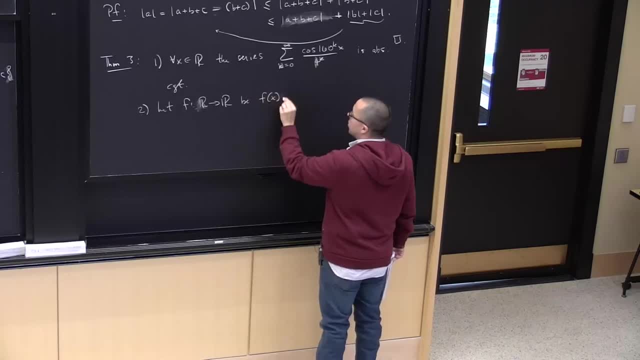 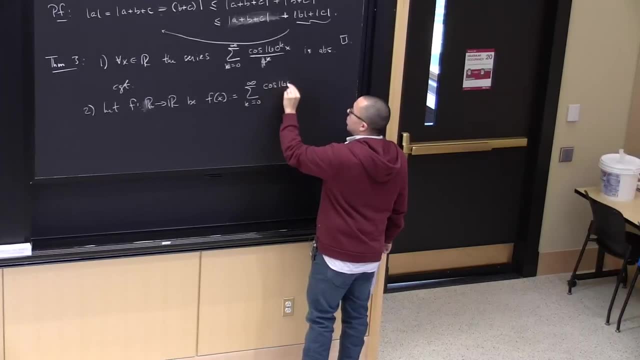 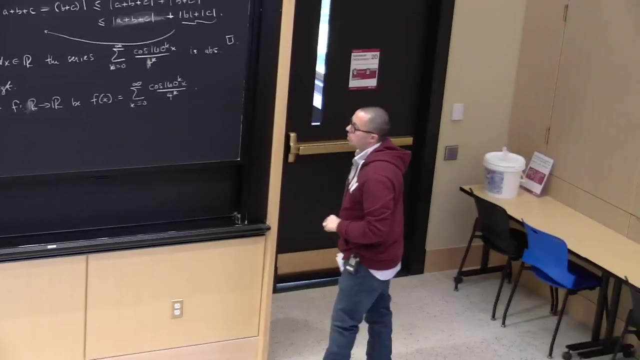 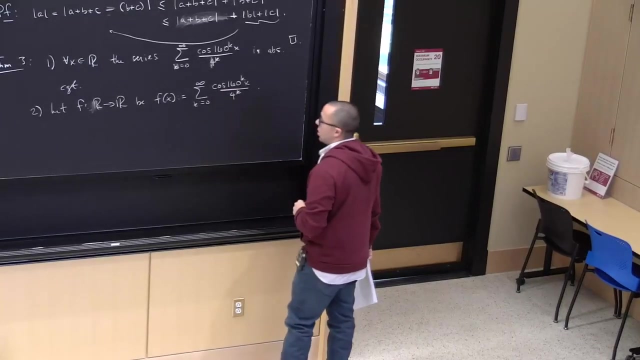 let f from r to r be defined by f prime. f of x is just the number that I get When I stick in x to the series Okay, Which is meaningful, because for all x this series converges absolutely. So this is just a function. 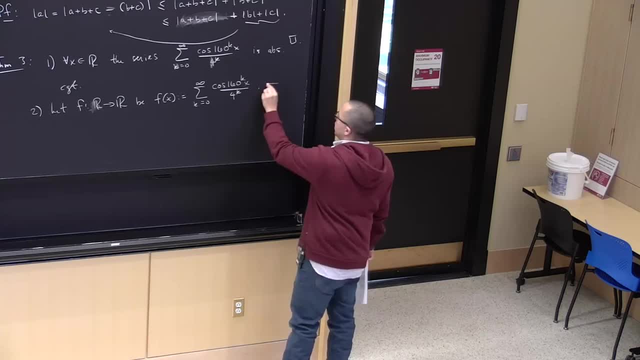 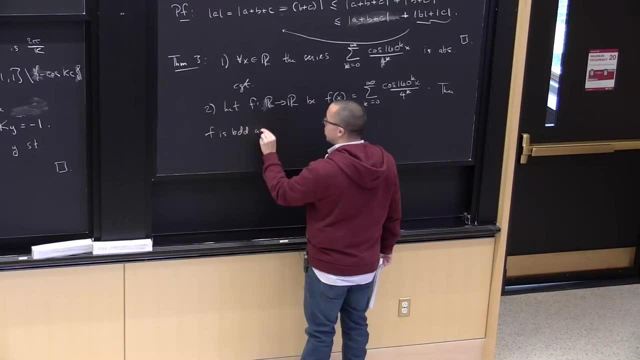 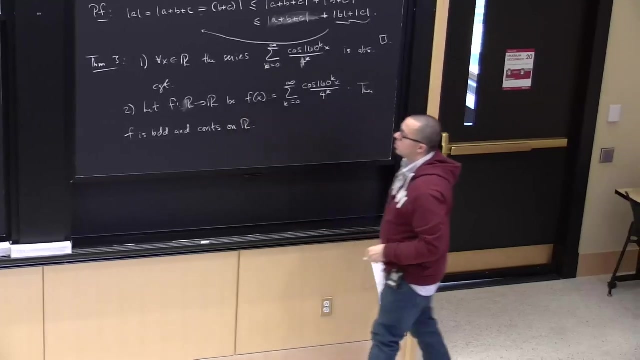 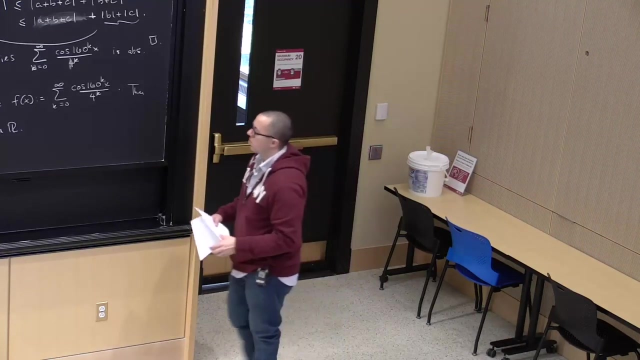 I just put in x, I get out a real number. Then the claim is: f is bounded and continuous. Okay, so this is gonna be our function, which is continuous but nowhere differentiable. all right, As you can see, it's built out of a bunch of very oscillatory functions. 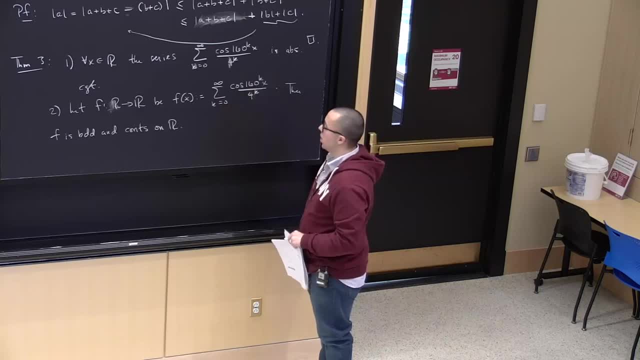 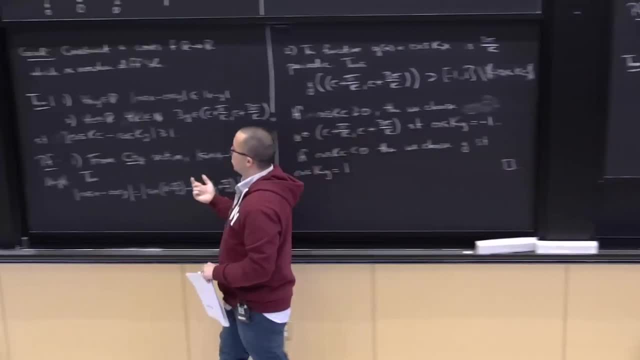 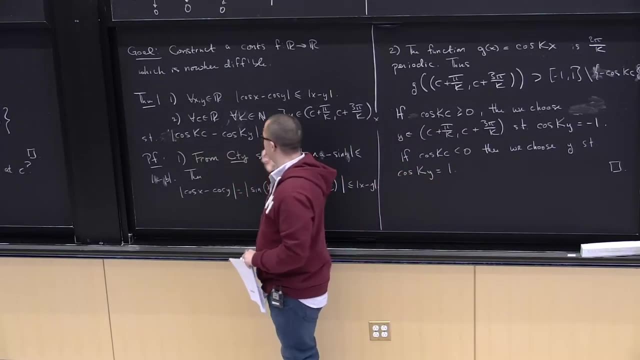 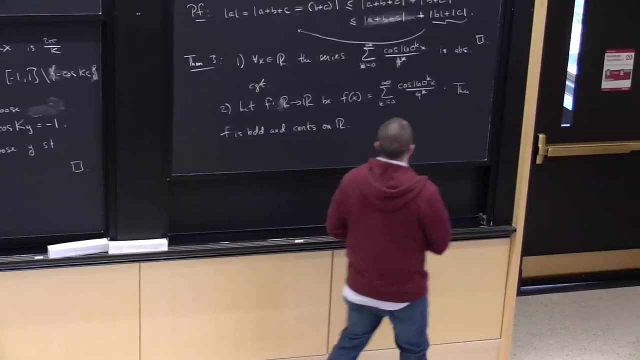 when we were talking about this theorem here. each one of those pieces is very oscillatory, on, you know, a very small interval that oscillates between two values that differ by at least one. Okay, And so all of these guys, all of these, 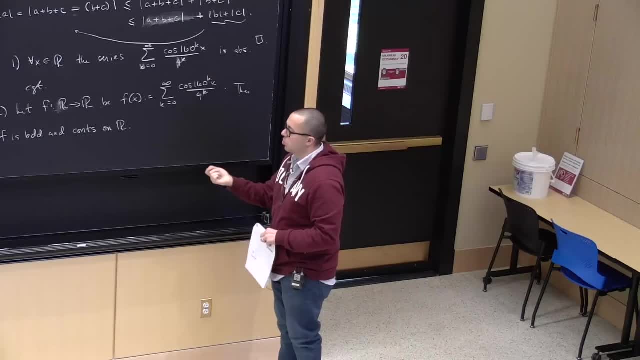 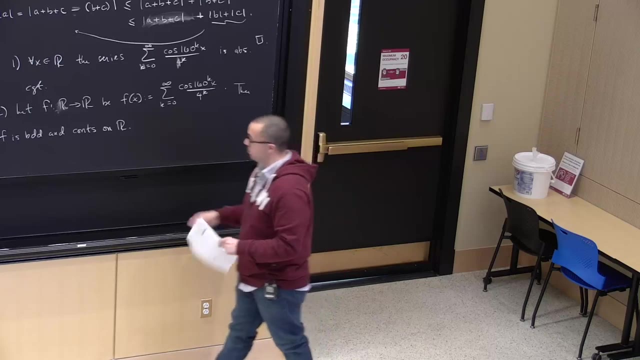 guys are oscillatory, and you know they're oscillatory on smaller and smaller intervals, and somehow we're adding them all up in a way to get a function that's oscillatory on arbitrarily small intervals and therefore it will not be differentiable. Okay So. 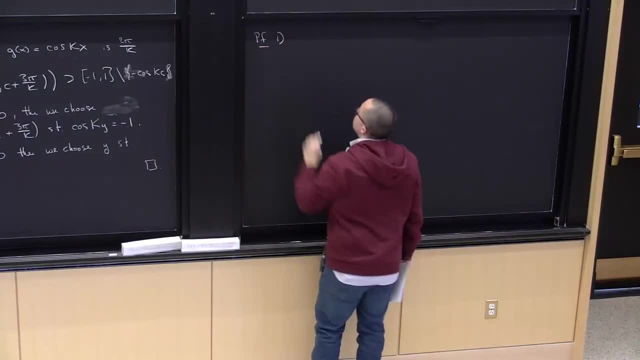 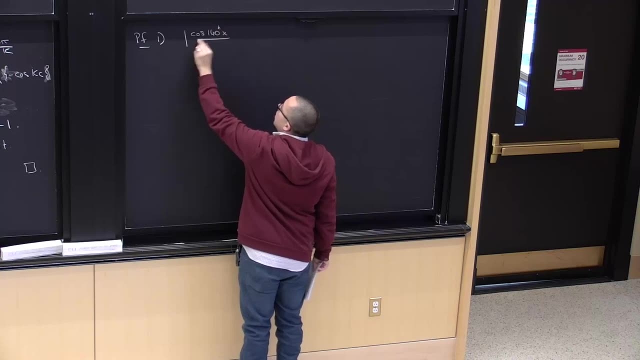 The proof of one is very easy. We just use a comparison principle. Cosine of 160k times x Over 4 to the k. This is less than or equal to, because cosine of no matter what you plug in, is bounded by 1.. This is always bounded by 1 over 4 to the k. 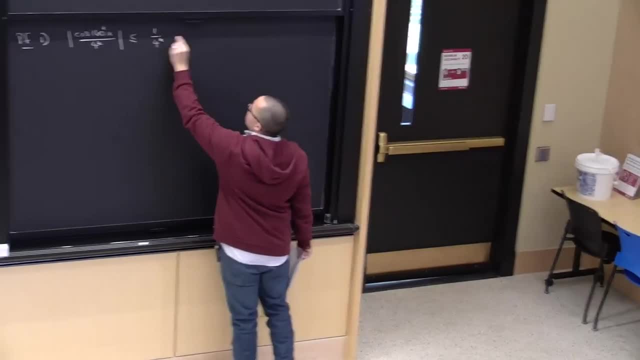 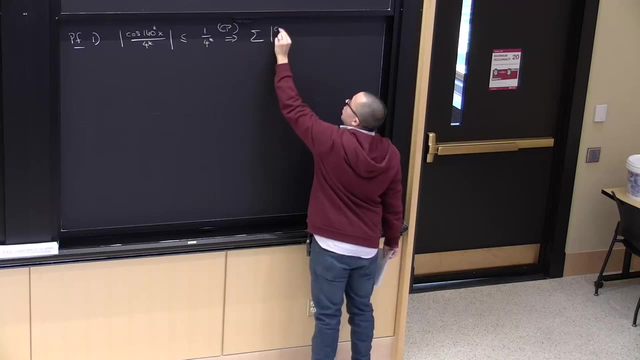 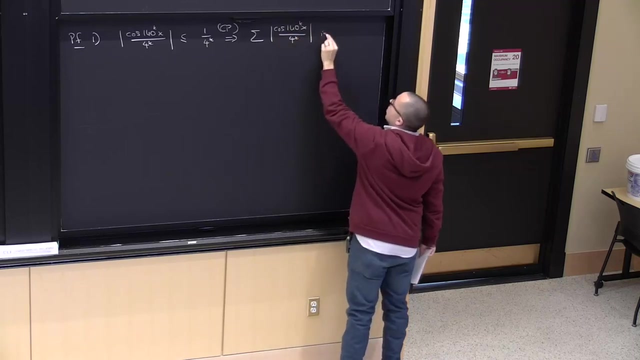 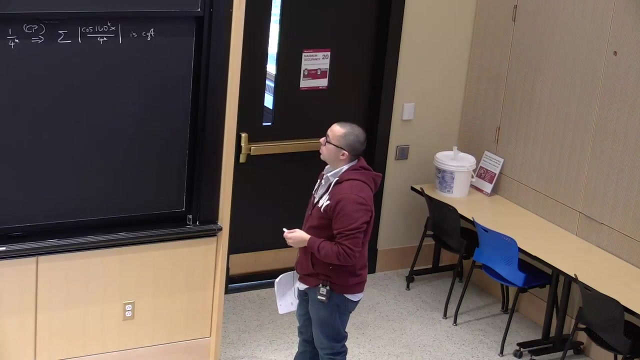 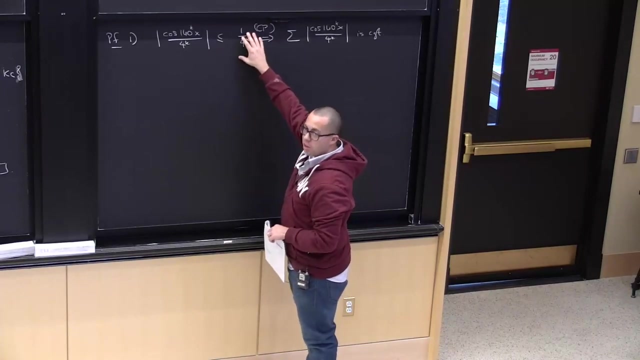 Right And therefore, by the comparison principle, we get that this series is convergent And therefore the original series is absolutely, absolutely convergent. Okay, So each of these is bounded by 1 over 4 to the k. This series converges. This is a. 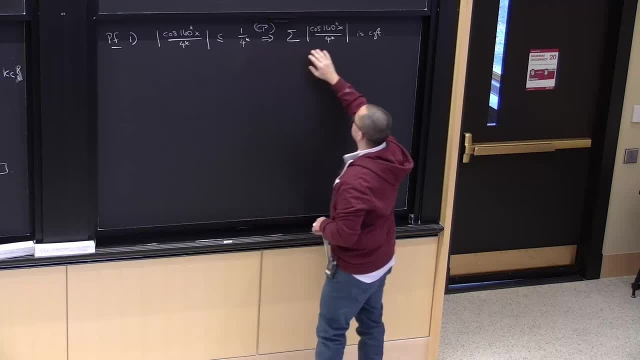 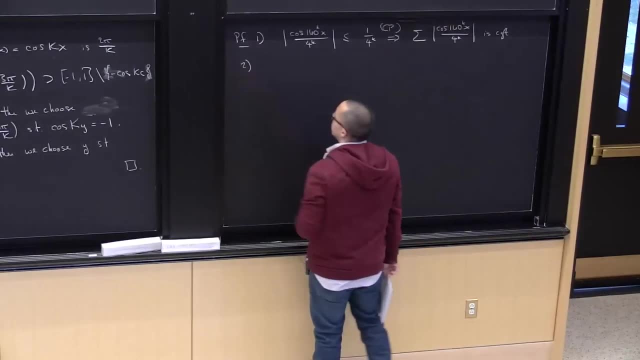 geometric series. Therefore, by the comparison principle, this series converges. Okay, So now we have this function defined by the series. Okay, No, this is not a power series, because the power series involves you know, you have to you. 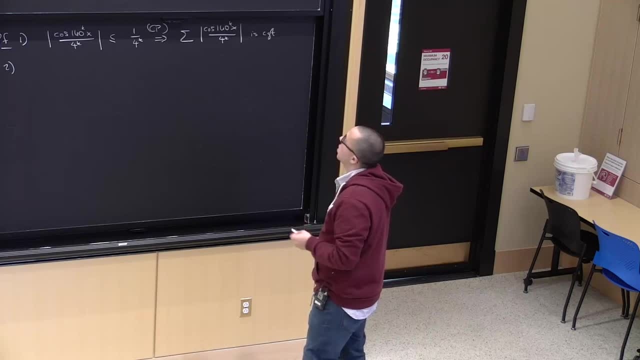 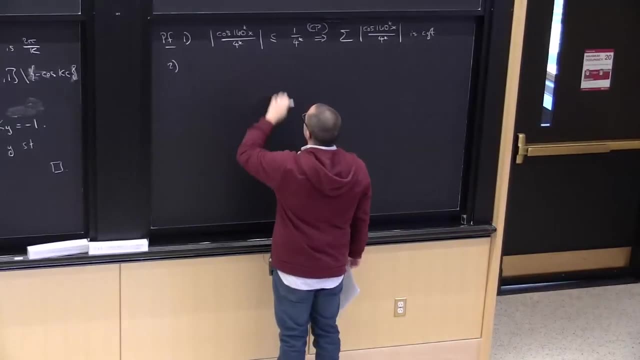 know really lay out the operating formula right, So you can't use it. you need to you polynomials in X. This is cosine of X, or number times X. So let's show it's bounded. The same proof, actually, that we gave here. 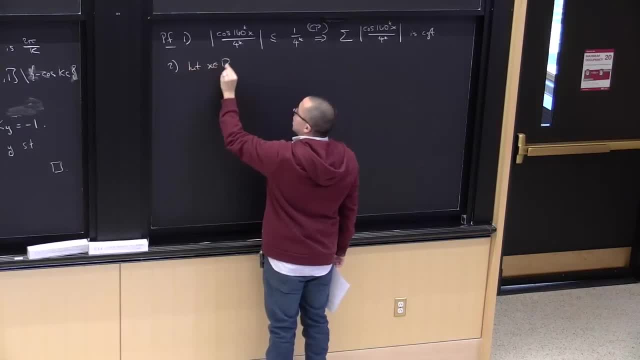 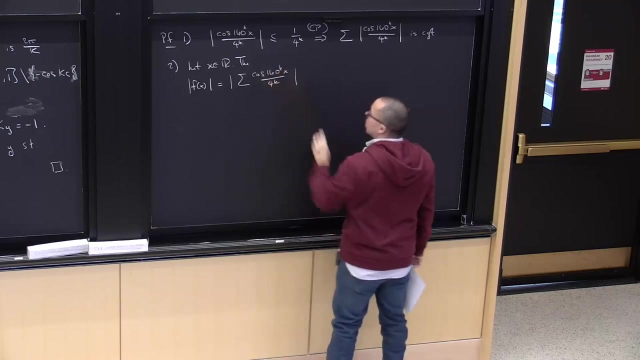 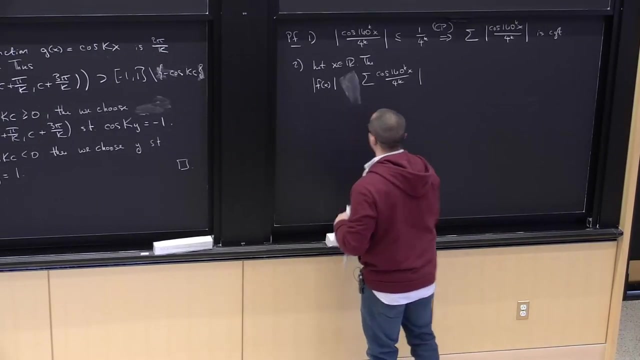 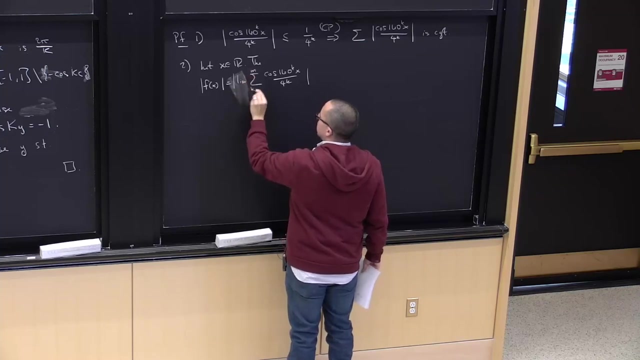 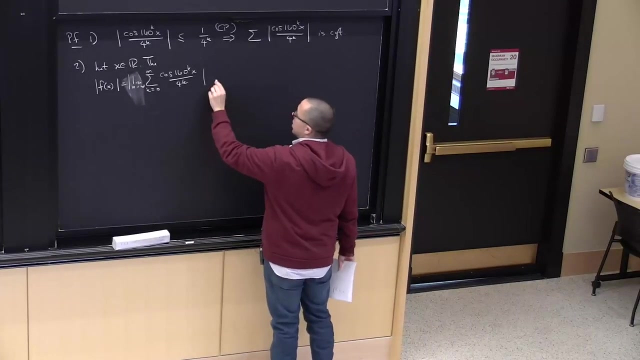 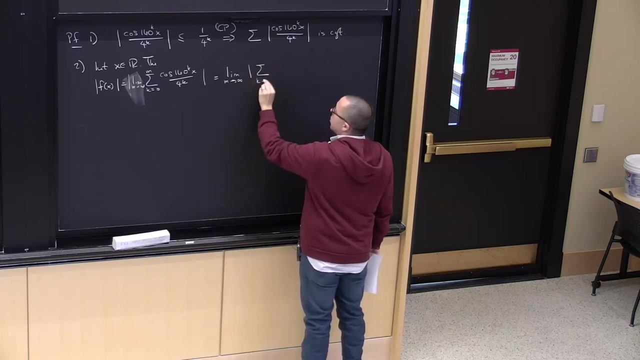 shows it's bounded with X being R, Then f of X equals. this is equal to the limit, as M goes to infinity of this. And now for absolute values. this limit pulls out Whenever the limit exists. the limit of the absolute value. 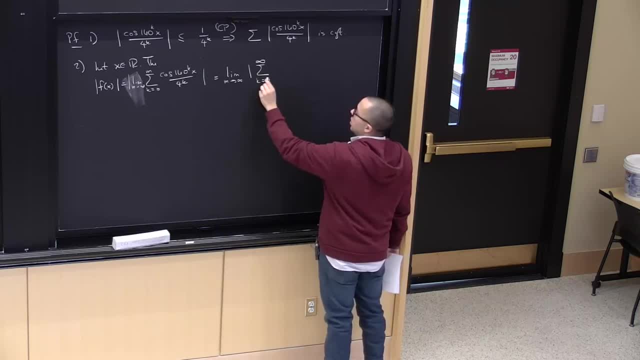 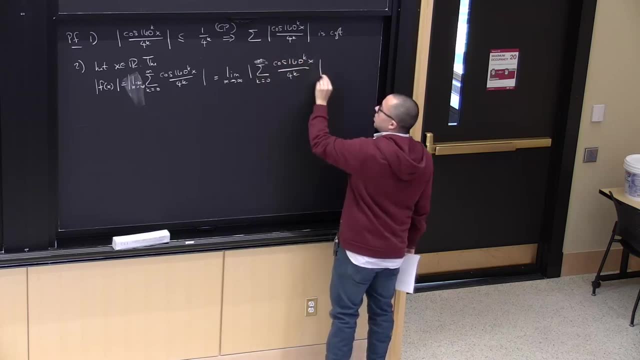 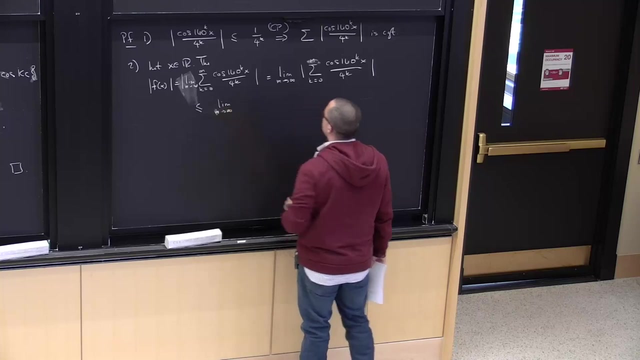 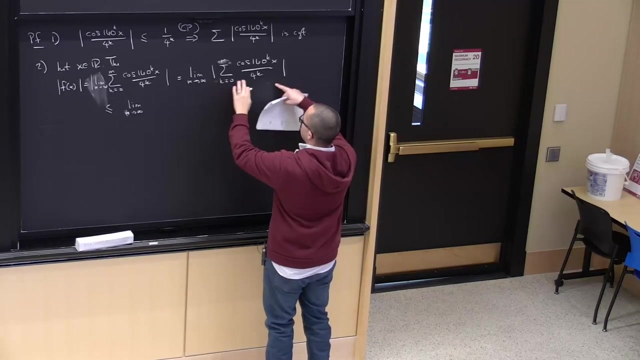 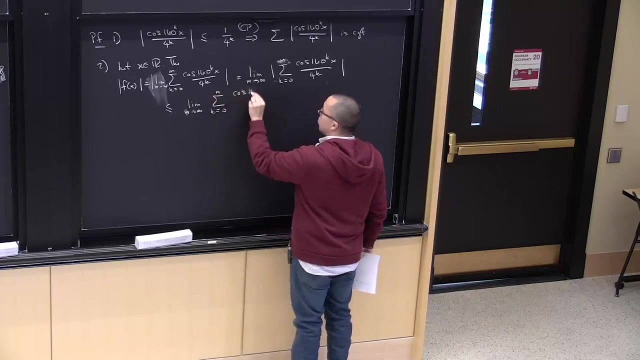 equals the absolute value of the limit And this is less than or equal to the limit, as M goes to infinity of bringing the absolute. So by the triangle inequality, this is just a finite sum. So I can bring the absolute values in and I get sum from K equals 0 to M. cosine 160K. 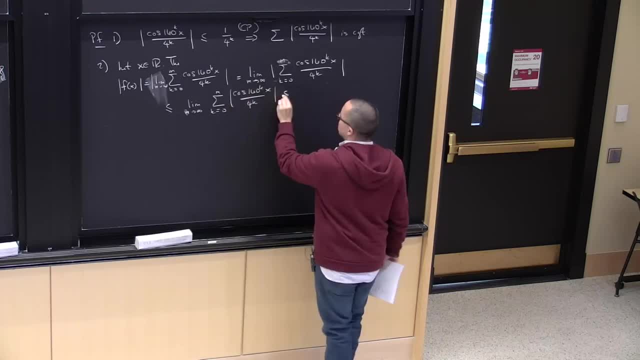 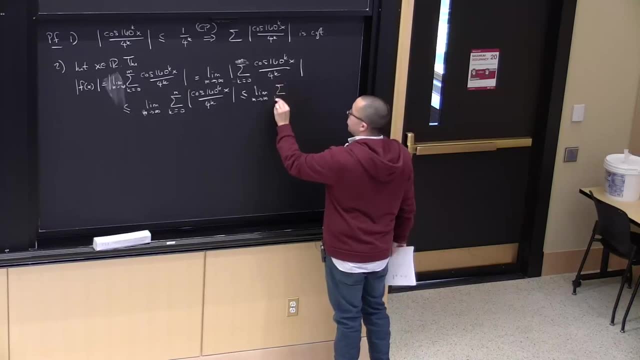 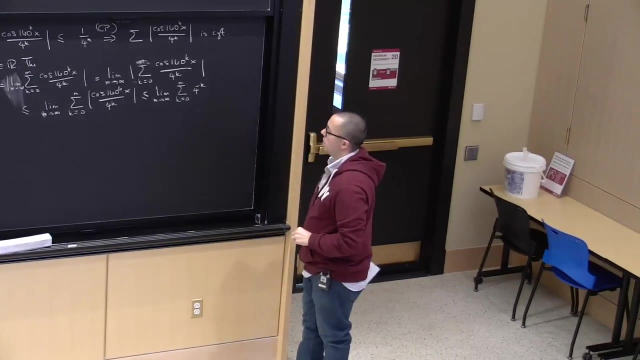 X over 4 to the K absolute value, And this is less than or equal to the limit- as M goes to infinity- of sum K equals 0 to M, of 4 to the minus K, again, because cosine of anything is bounded by 1.. 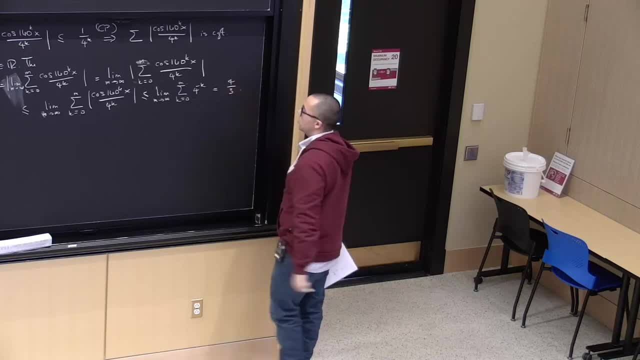 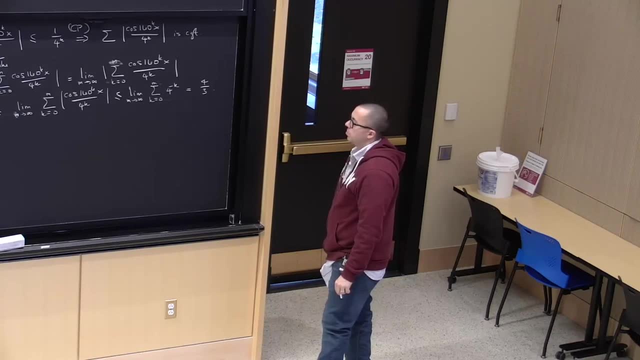 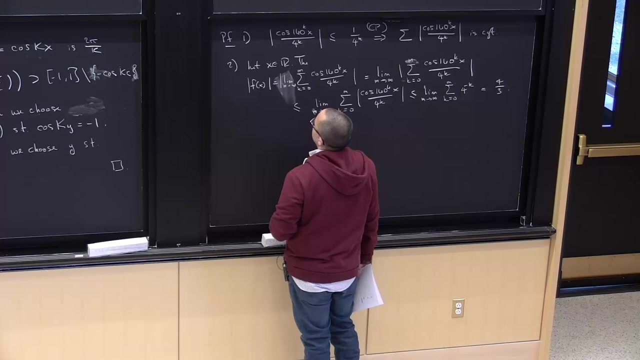 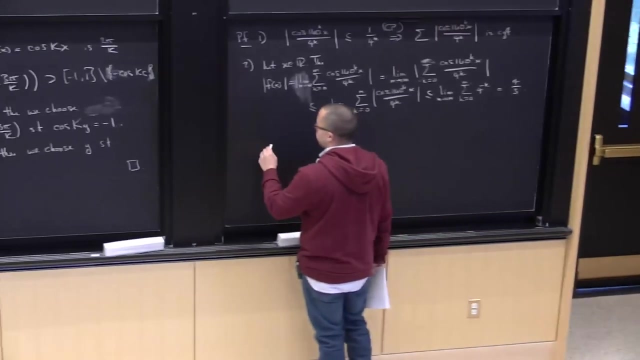 And this equals 4 thirds. This is just a sum from K equals 0 to infinity, of 4 to the minus K. So this function is always bounded by 4 thirds. So the function is bounded. Let's now show it's continuous. 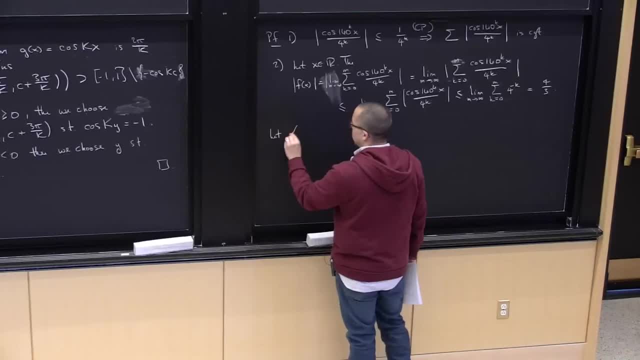 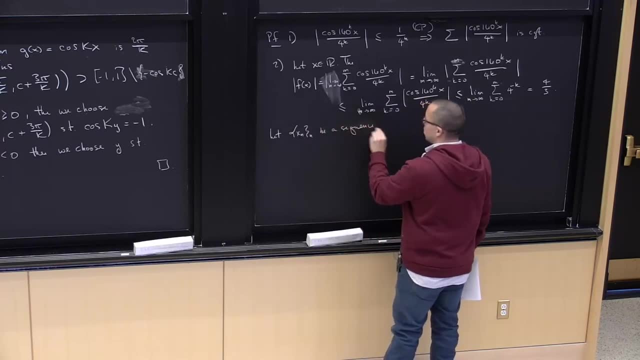 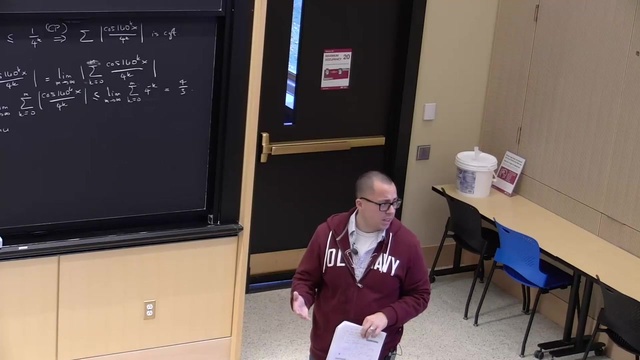 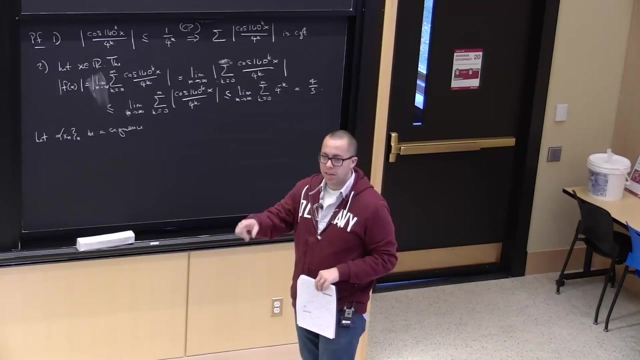 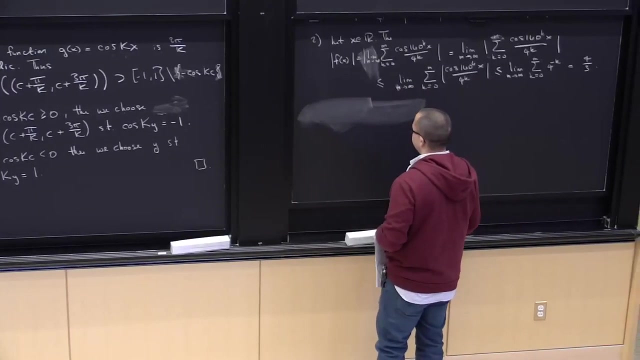 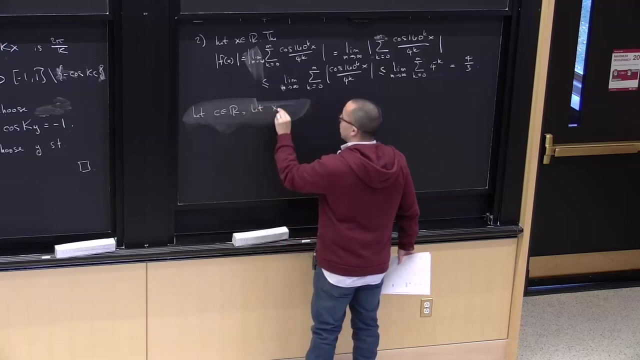 So to show a function that's continuous, remember we have that other characterization of continuity, that a function is continuous at a point, if, and only if, for every sequence converging to that point, f of xn converges to f of c. So before I start writing all this down, let c be an r. 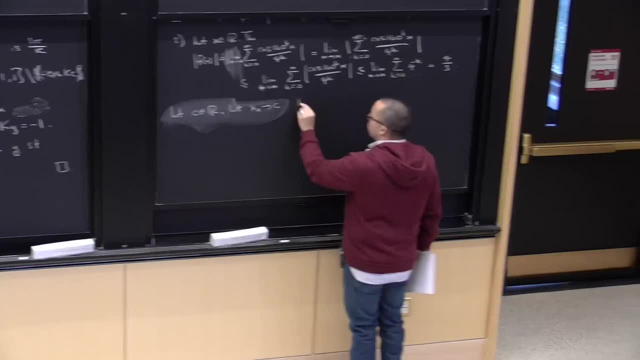 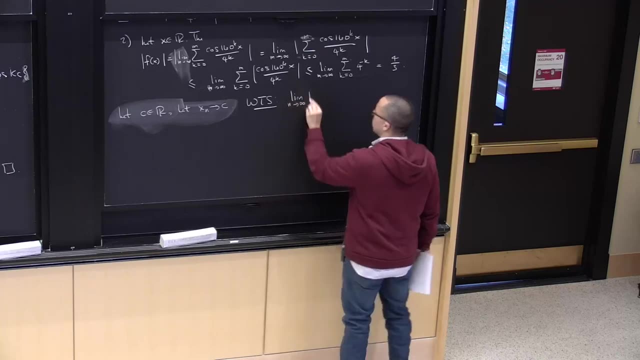 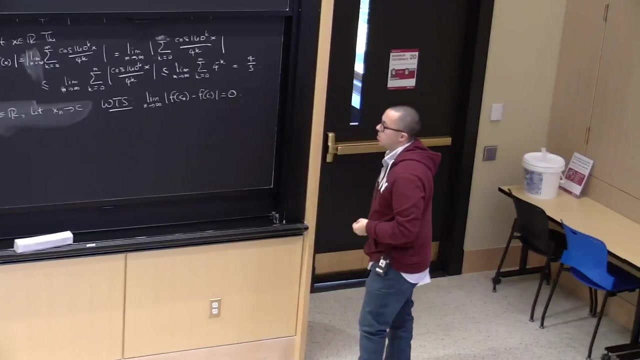 and let xn be a sequence converging to c. So what we want to show is that limit as n goes to infinity, of f of xn minus f of c in absolute value equals 0. That's the same as saying the limit as n goes to infinity. 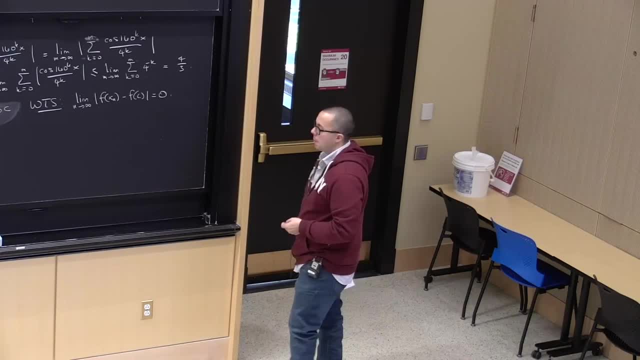 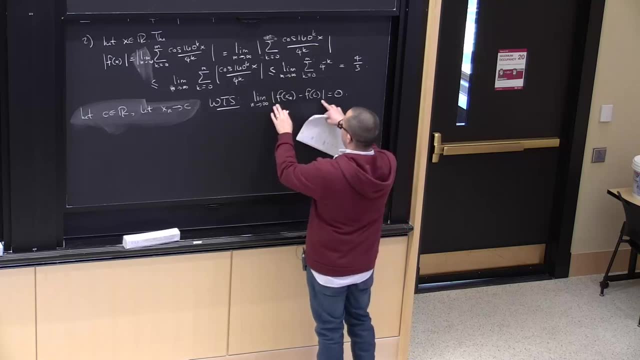 of f of xn equals f of c. Now f is a bounded function. so this sequence, f of xn minus f of c in absolute value is a bounded sequence. So it has a lim-soup And we did an exercise on the assignment. 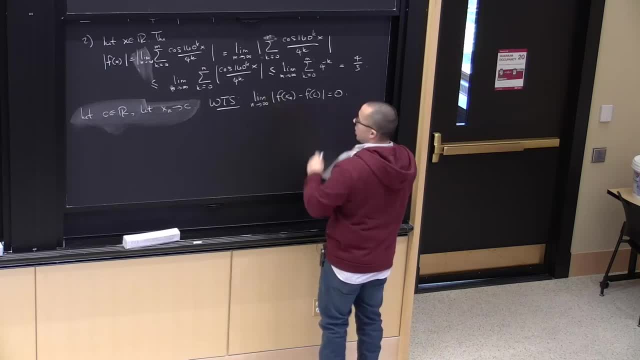 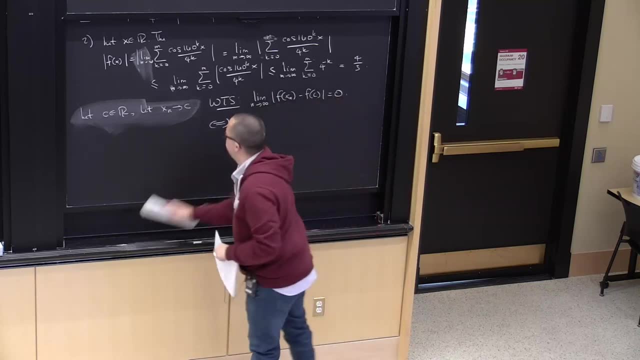 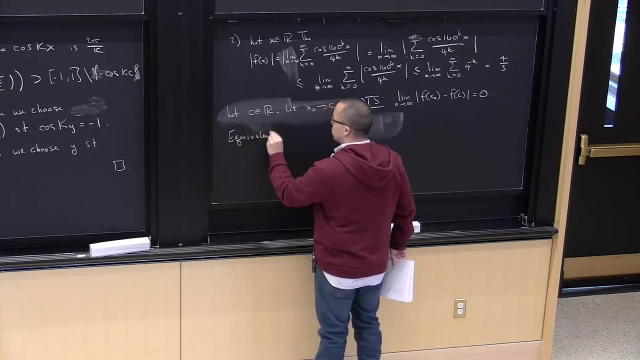 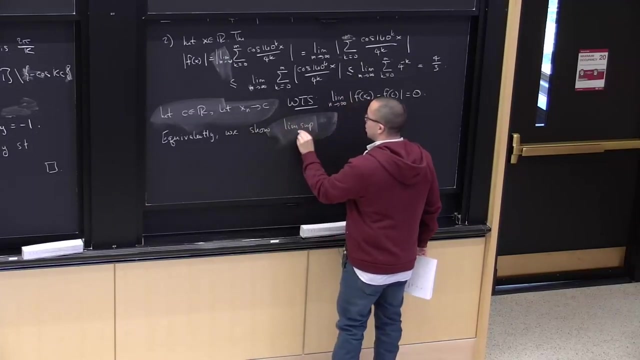 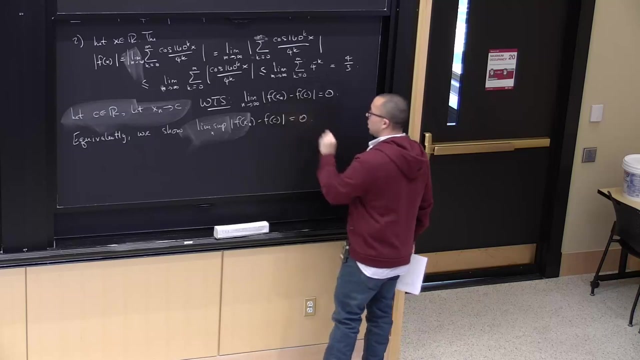 that the limit of a sequence equals 0 if, and only if, the lim-soup equals 0.. Equivalently, we'll show that the lim-soup of f of xn minus f of c equals 0.. This thing always exists for a bounded sequence. 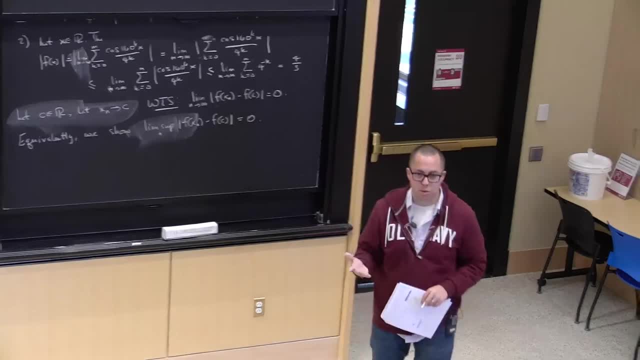 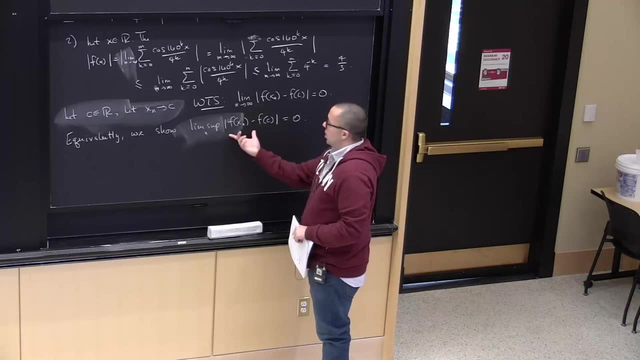 which is one of the reasons. what makes lim-soups so useful is that they do always exist. So if we show that this lim-soup equals 0, then this is equivalent to showing this limit equals 0.. Again, this was an exercise where you can take it as the lim-inf. 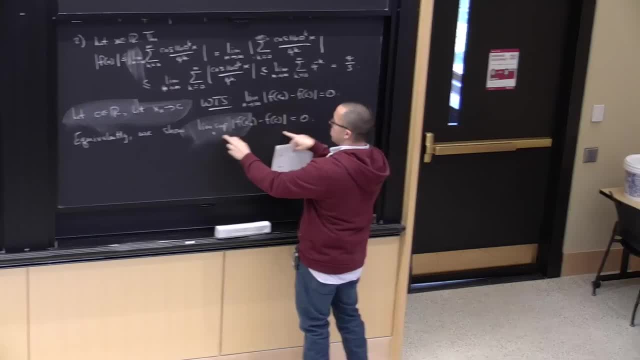 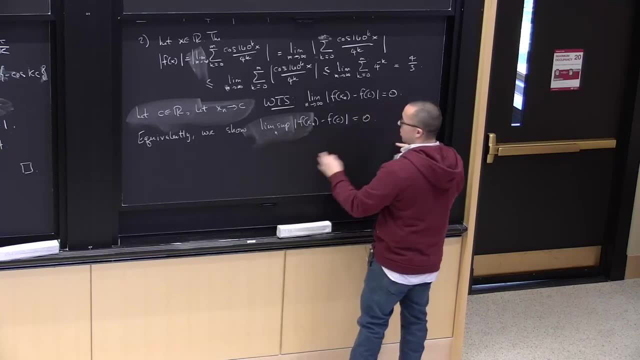 of something that's non-negative is always bigger than or equal to 0. So if we show this is equal to 0, we would have: 0 is less than or equal to the lim-inf of this thing is less than or equal to the lim-soup, which equals 0.. 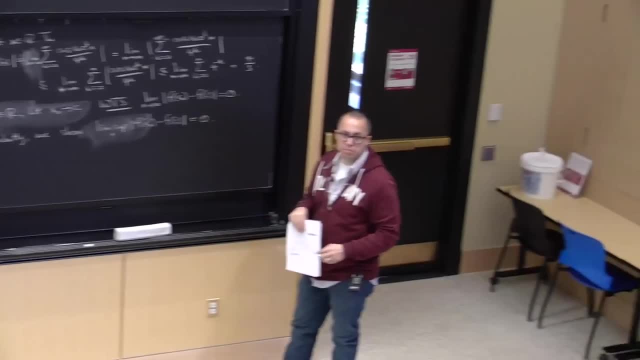 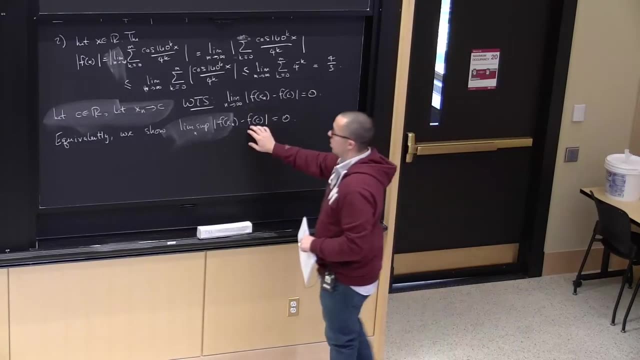 And therefore the lim-inf equals the lim-soup equals 0.. So that's another way of seeing that this is equivalent to this. All right, So we're going to show this, that the lim-soup of f, of xn minus f. 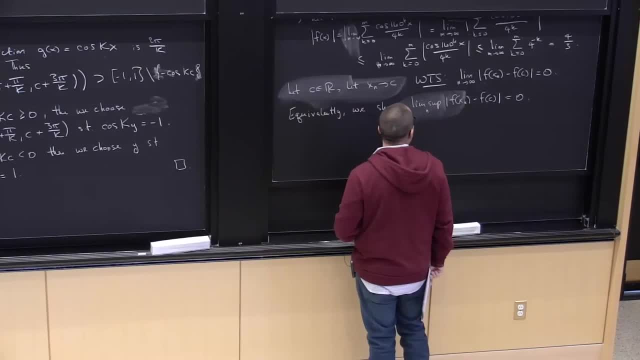 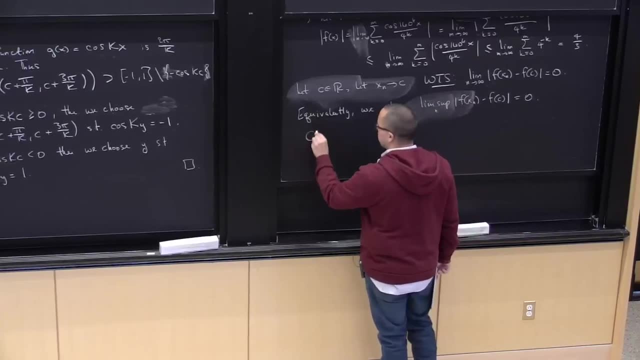 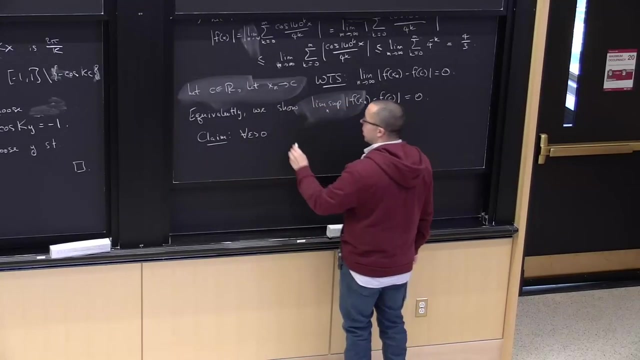 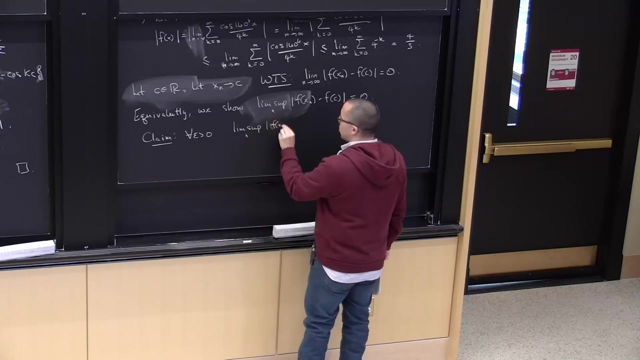 of c equals 0, but we don't, And so that might be a little tough. but what we can show, what we will show, is we'll give ourselves a little room, We'll show that, for all epsilon positive, the limb-soup of f, of xn. 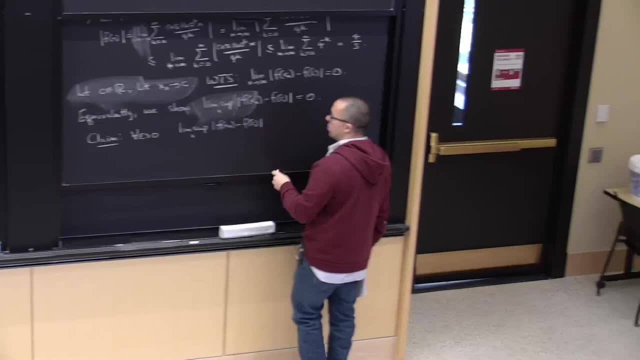 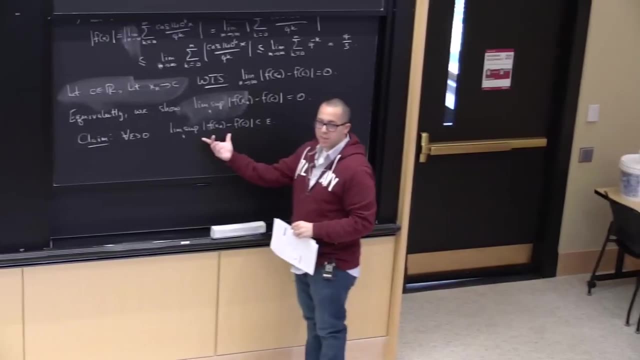 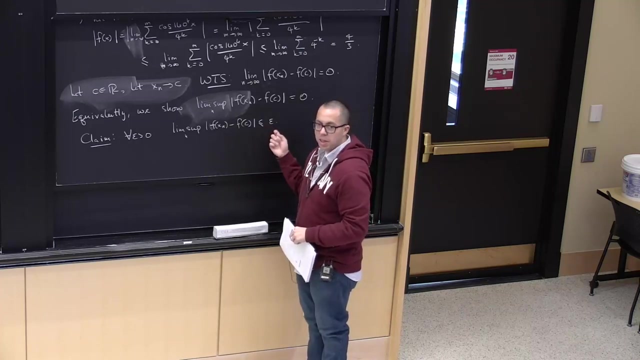 of n minus f of c, which is a non-negative number, is less than epsilon. So this is a fixed number, non-negative number, which is always smaller than put less than or equal to there, which is smaller than any number that I want. 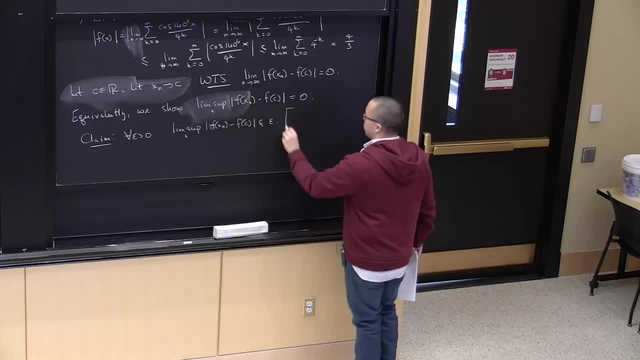 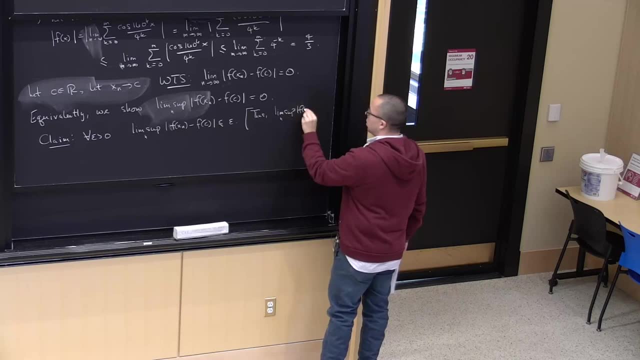 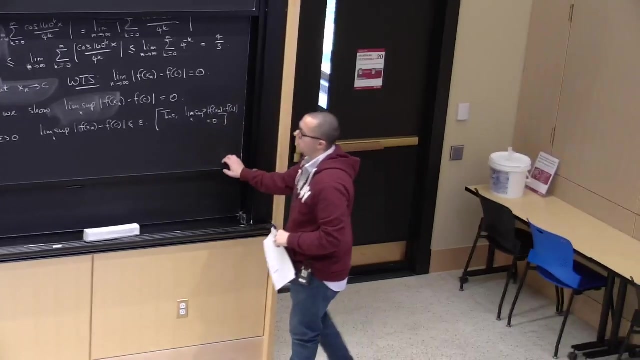 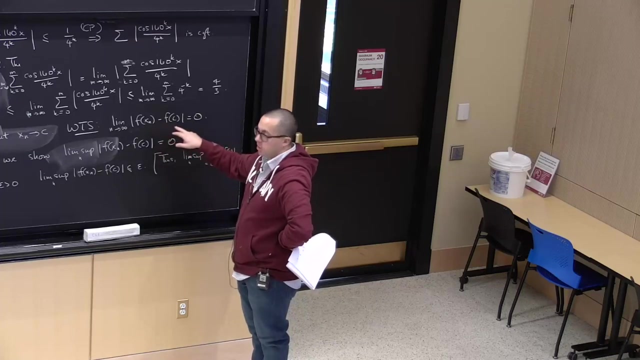 and therefore it has to be 0., Improving thus them soup. OK, So just to recap, we want to show we have a sequence converging to c. We want to show that f of xn converges to f of c. 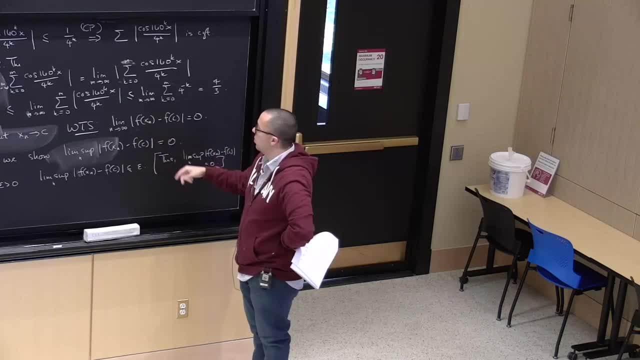 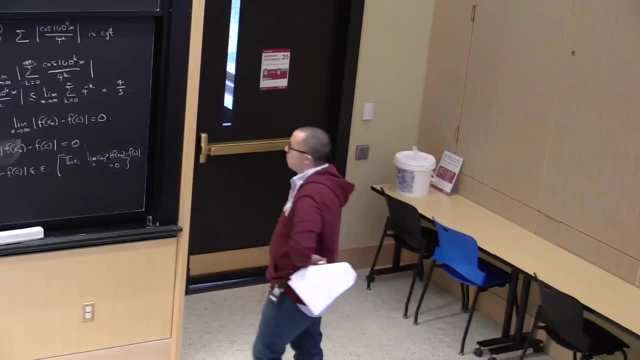 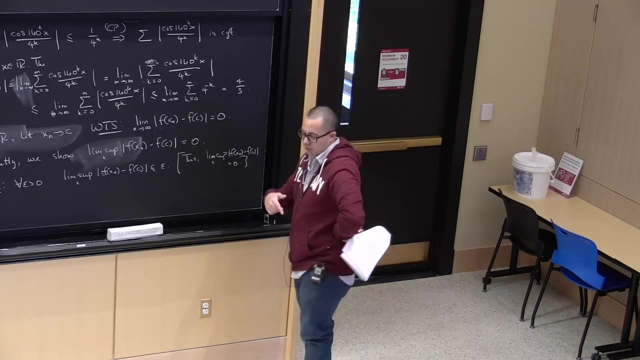 Another way of stating that is that this limit of the absolute value of the difference between these two, These two converges to 0. That's again a equivalent way of stating the limit, And in another assignment we proved that for a sequence of non-negative numbers. 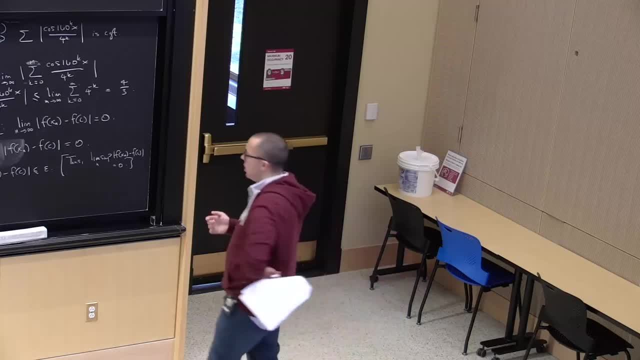 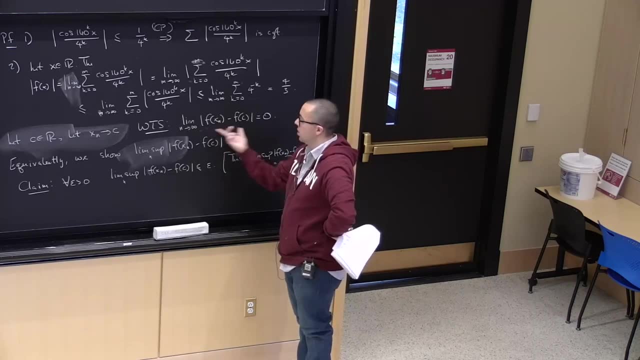 or, if you like, just for a sequence of numbers. it converges to 0 if, and only if, the limb soup of the absolute value converges to 0.. But this is a sequence of non-negative numbers. this absolute value, It's the value of f of xn minus f of c. 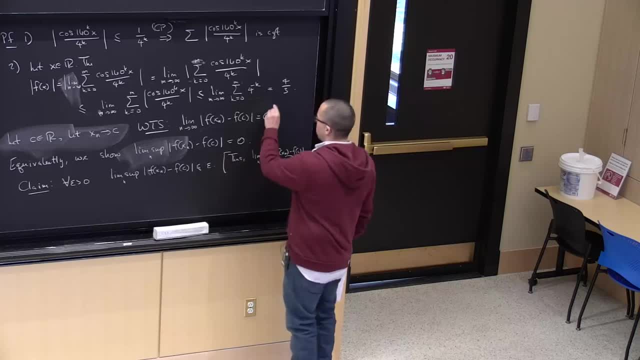 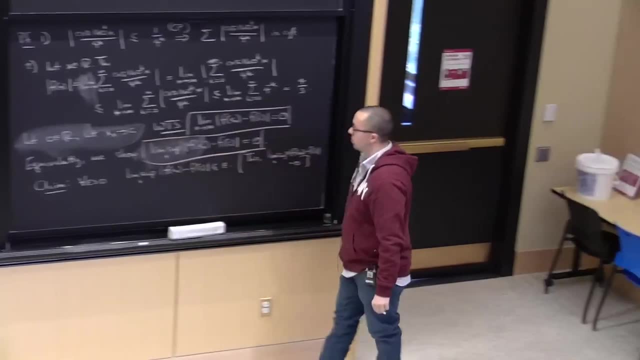 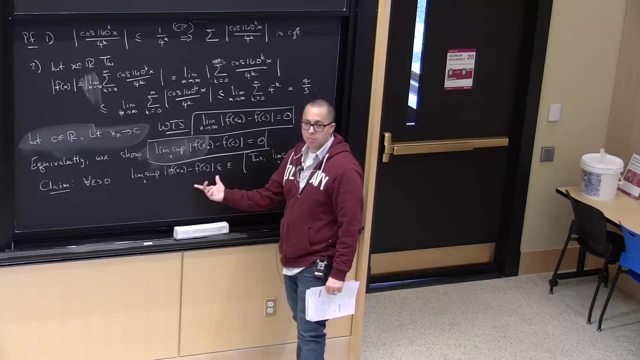 So this is equivalent to this. So this thing we want to show is equivalent to this thing right below it. Now, rather than show directly that this limit limb soup equals 0, we're going to show that, for all epsilon positive, it's less than or equal to that small number. 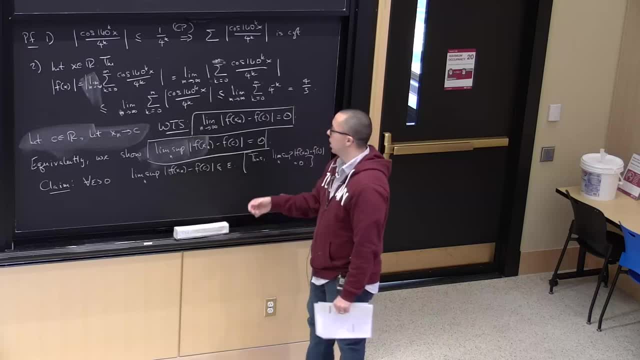 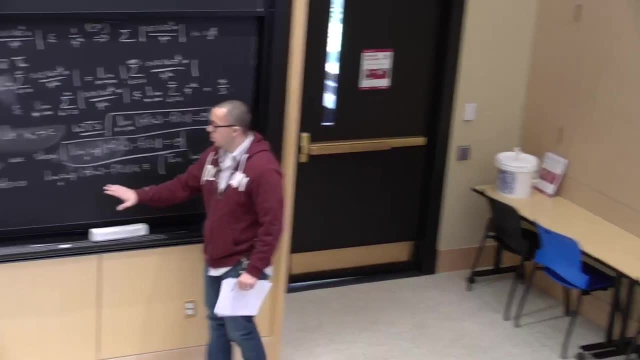 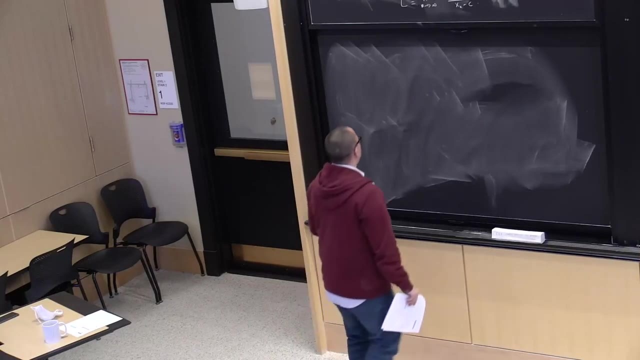 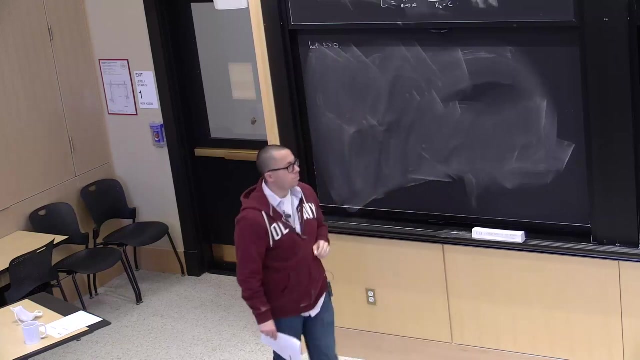 and therefore proving that it's 0 because it's a non-negative number smaller than every positive number. OK, So this is our goal: to show this. limb soup is less than epsilon. All right, So let epsilon be positive. We're now going to prove that that limb soup is less. 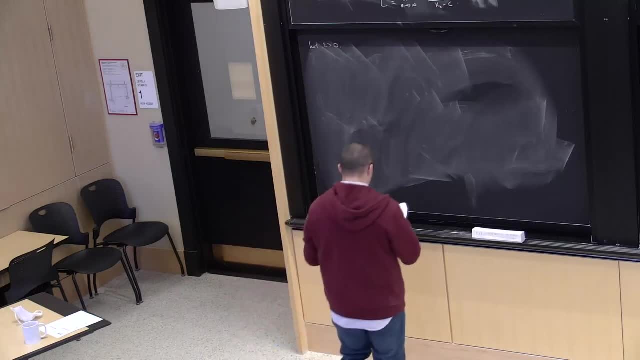 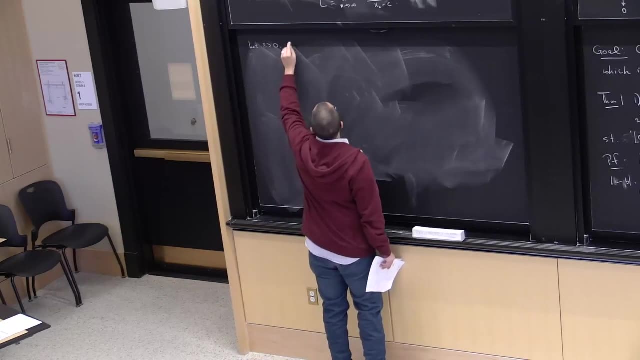 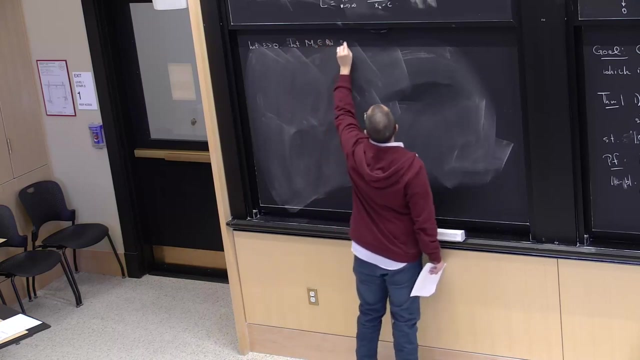 than epsilon. So, first off, that's our goal, And then we're going to show that that's less than epsilon, All right, So let's go ahead and fix that. OK off that m0 be a natural number, such that the sum from k 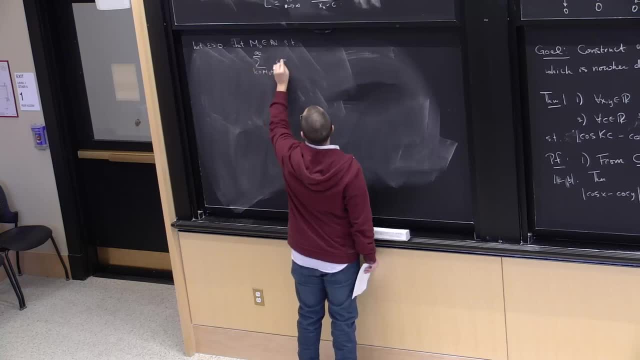 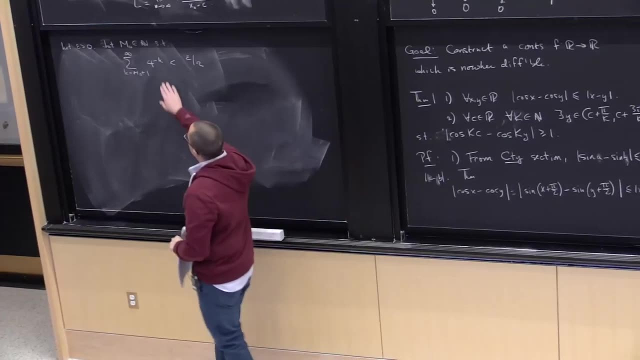 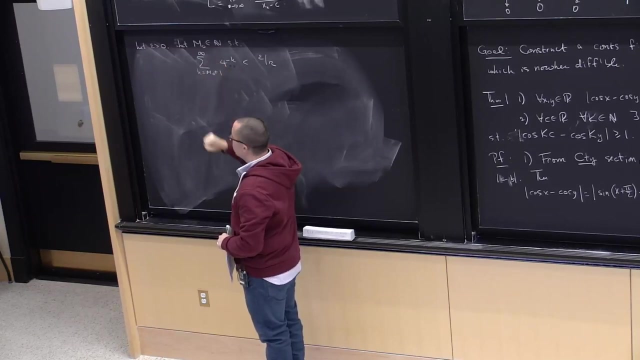 equals m0 plus 1 to infinity, of 4 to the minus k is less than epsilon over 2.. So this series here, this is a convergent series. if I go from k equals 0 to infinity, And we have this Cauchy criterion. 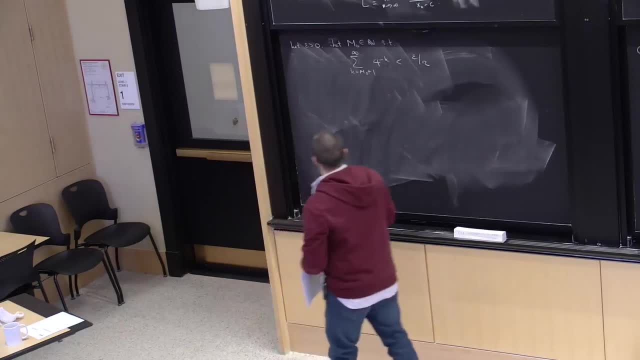 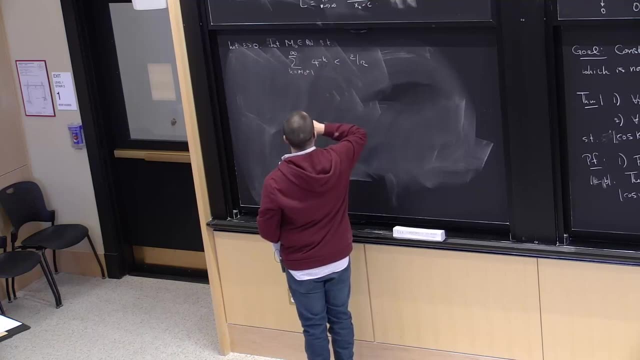 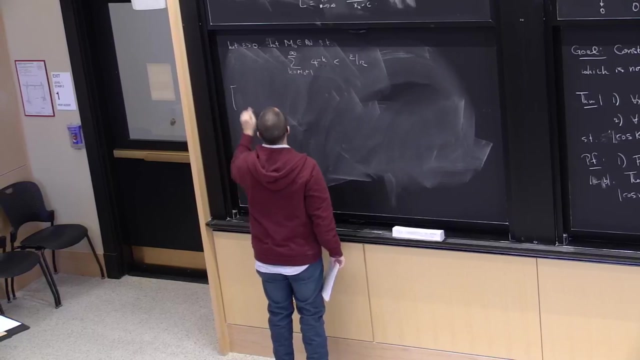 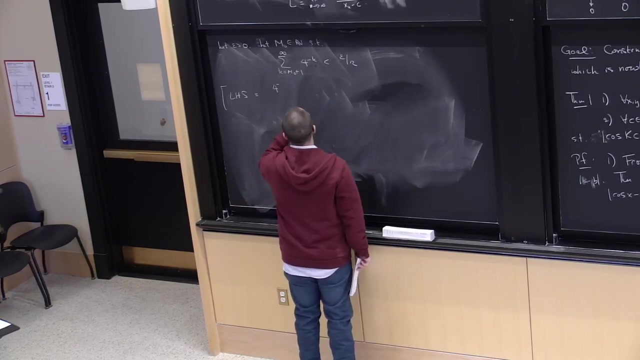 for convergent series, which can be equivalently stated as for all m0, a natural number, there exists. or for all epsilon, there exists. So first off, OK, rather than go through all that, we can actually just compute this that the left-hand side equals 4 to the 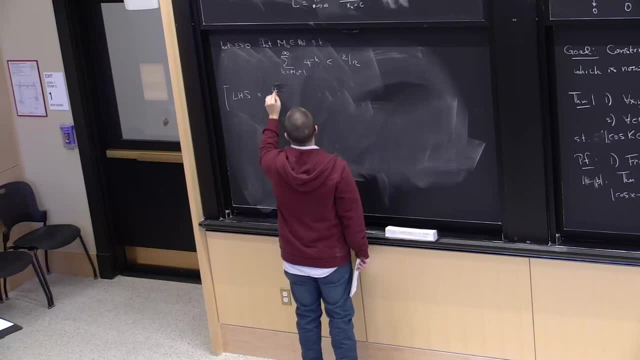 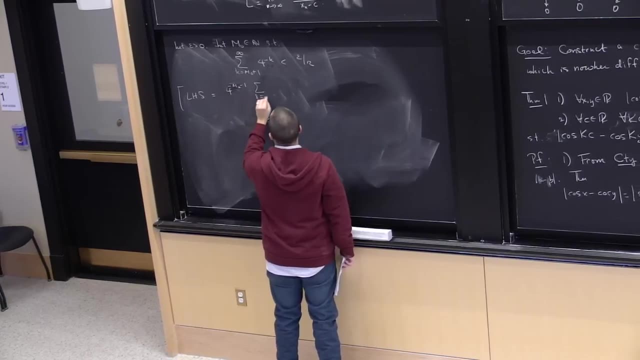 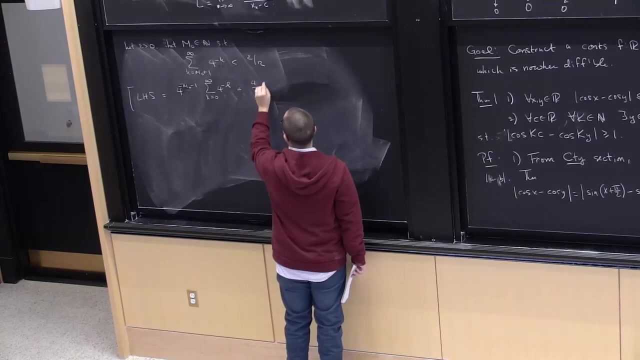 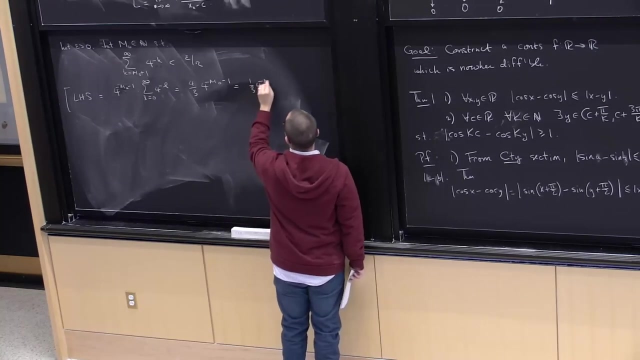 4 to the minus m0 minus 1 times sum from l equals 0 to infinity. 4 to the minus l, which equals 4 thirds 4 to the minus m0 minus 1,, which equals 1 third 4 to the minus m0, OK. 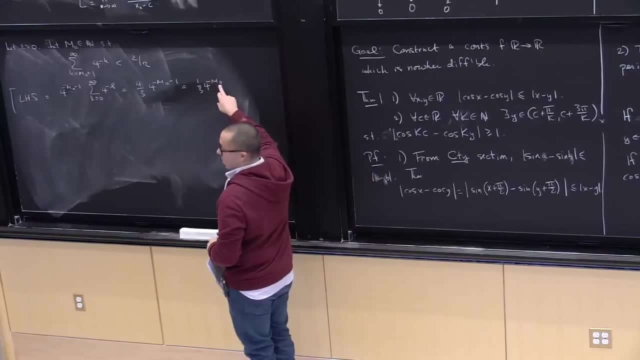 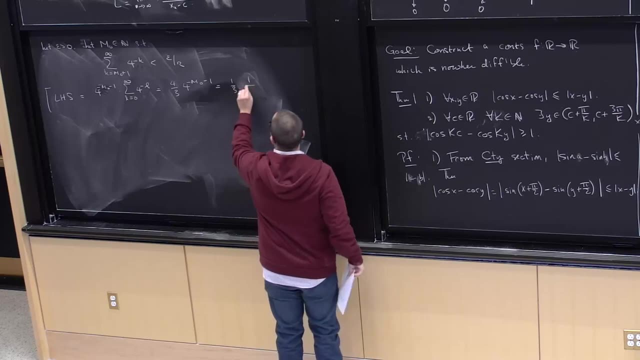 So if m0 is chosen very large, then it's going to be a natural number. So if m0 is chosen very large, this is 4 to the minus m0.. So this is like I can write this as 1 third over 1 fourth. 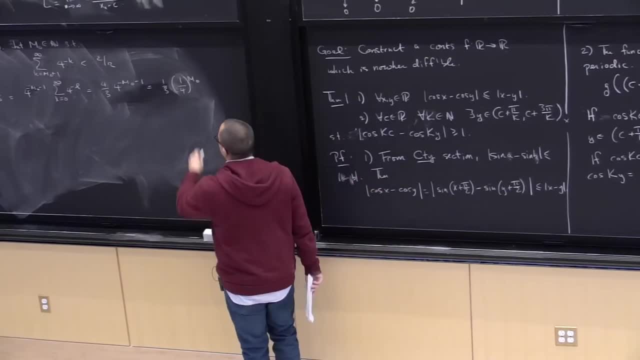 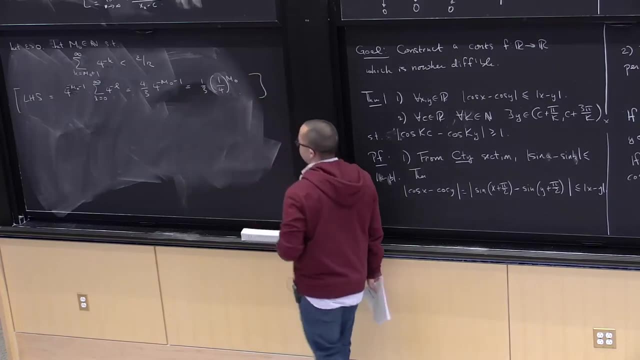 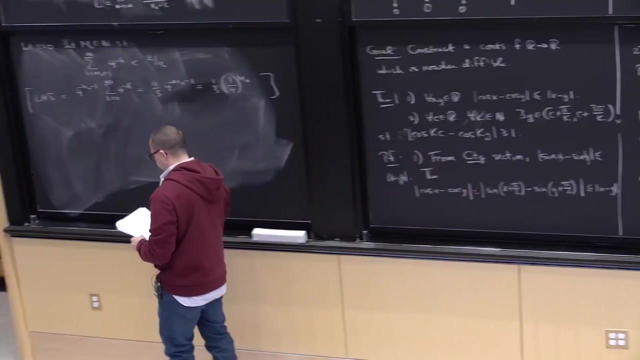 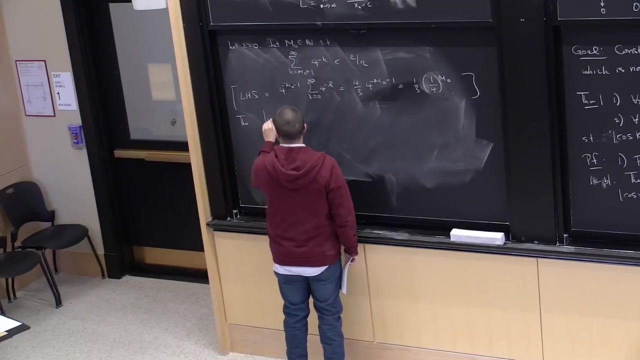 And as long as m0 is chosen very large, I can always make this very small. That's the left side over there, So I can always find an m0, so that this is the case. OK, And now we compute the Limb soup of f. 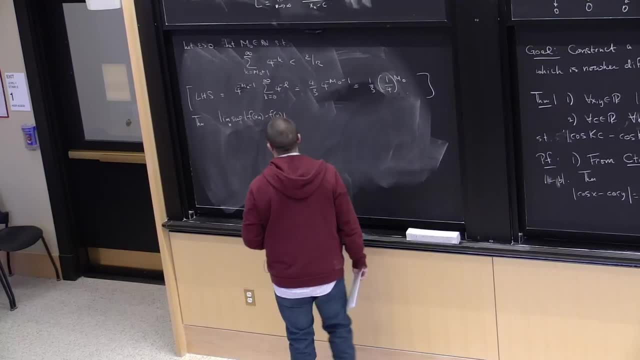 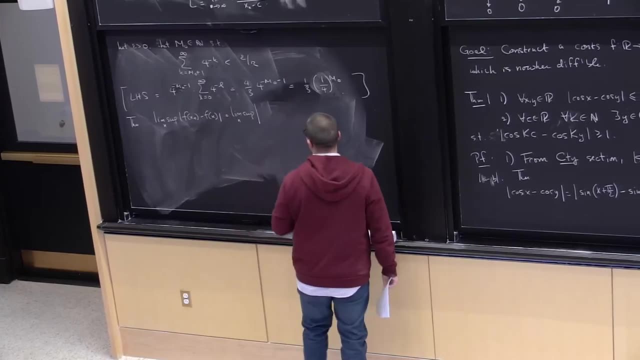 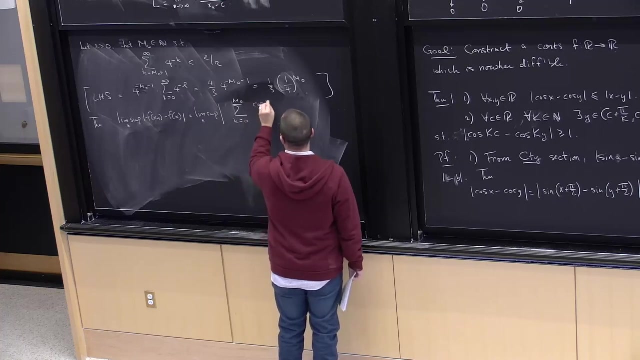 minus f. We split this up into two pieces. This is equal to Limb soup of n of two parts. sum from k equals 0 to m0 of cosine of 1 divided by 1. 2.9.0.. Kolb's enrolled' and so we had to get some arguments. 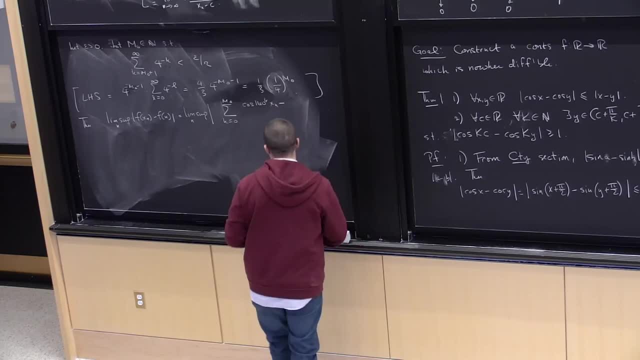 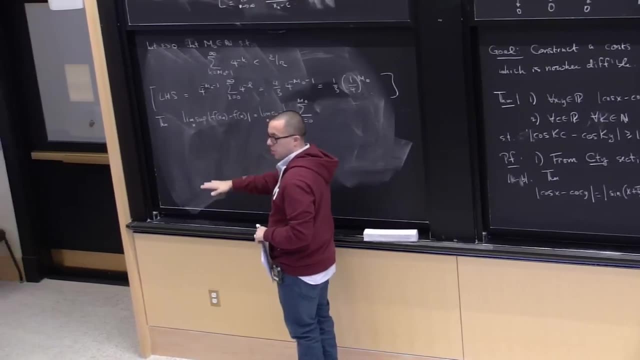 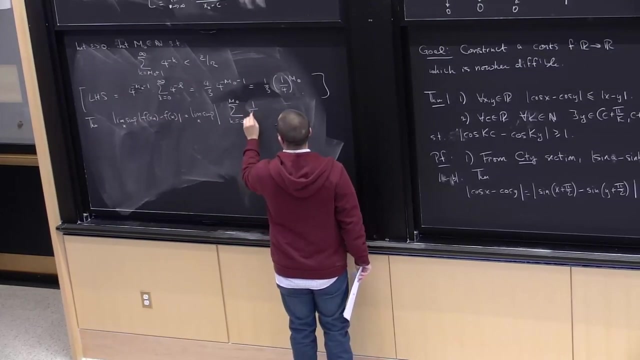 160k xn minus. so each of these is defined in terms of sum. so I'm going to break the sum up into up to m0 and then everything past m0.. This is equal to 1 over 4k times cosine. 160k xn. 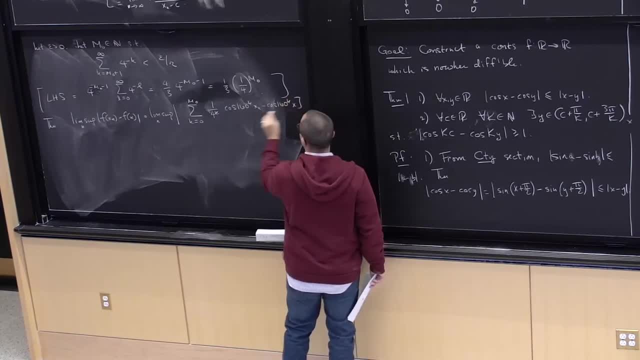 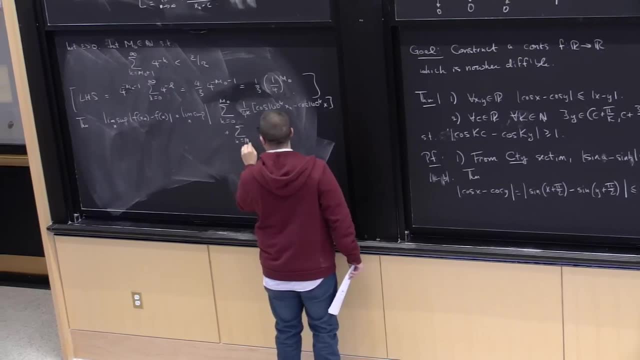 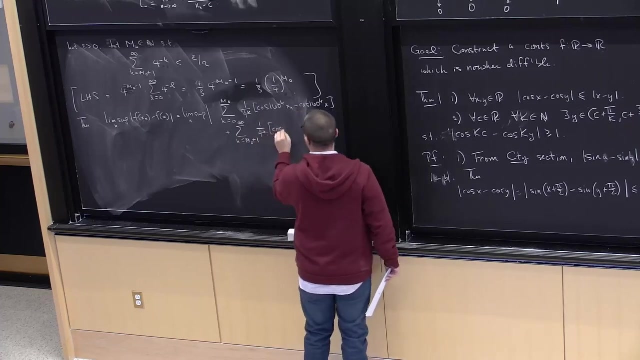 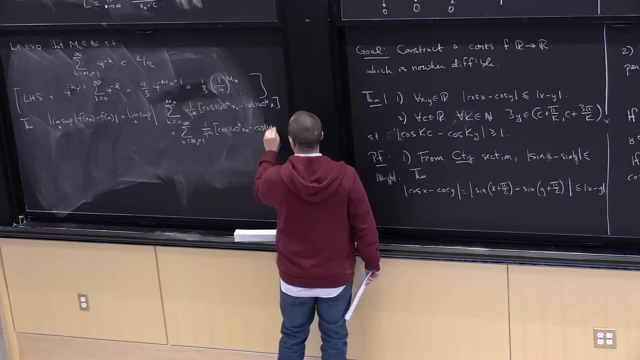 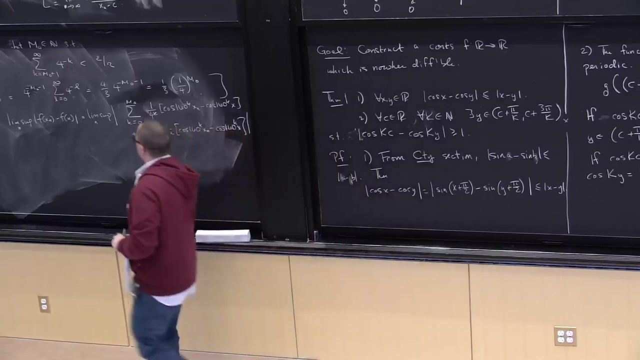 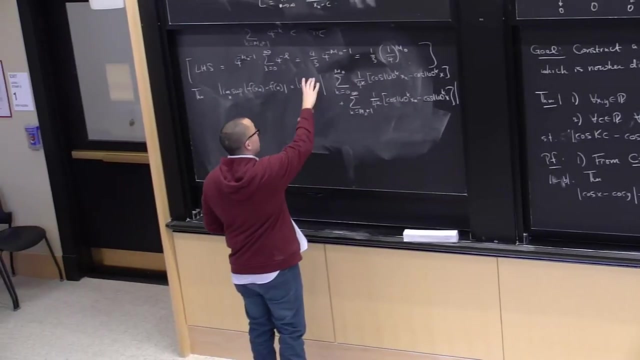 minus cosine, 160k. x plus sum from k equals 0 to m0, plus 1 to infinity, 1 over 4k, same thing Absolute value. And now we use the triangle inequality in the fact that limb soups preserve inequality. 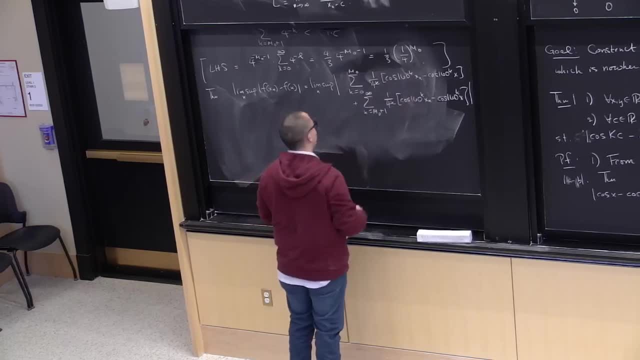 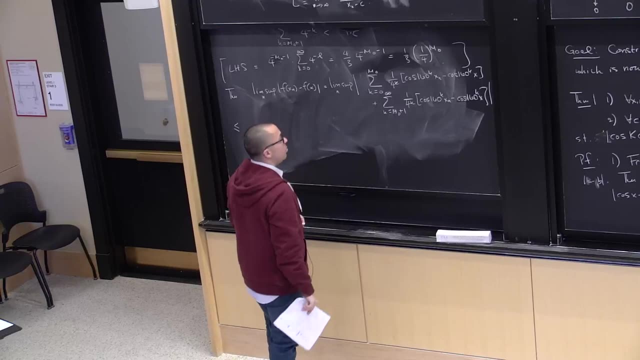 so the absolute value of this thing is less than or equal to the sum of the absolute values, and the limb soup of those sequences is less than or equal to the sum of the limb soups. That was another exercise from an assignment, or you did something similar with the limb imp. 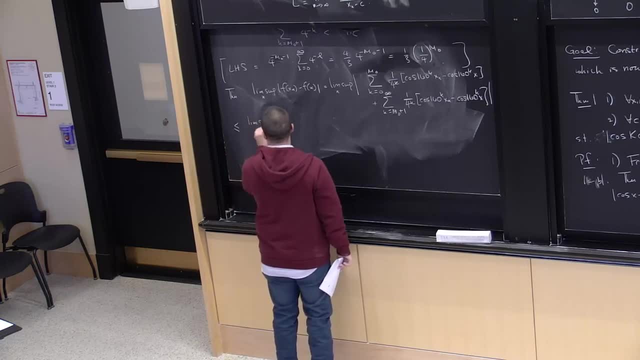 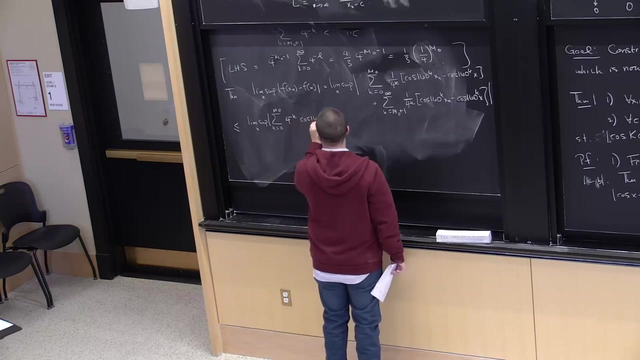 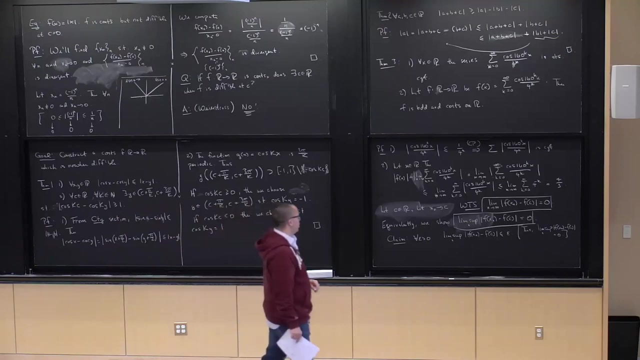 so this is less than or equal to limb soup. Now I use the triangle inequality. sum from k equals 0 to m0, 4 minus k cosine 160k. x of n minus cosine 160k. oh dear. So I've been writing x. I meant to write c. 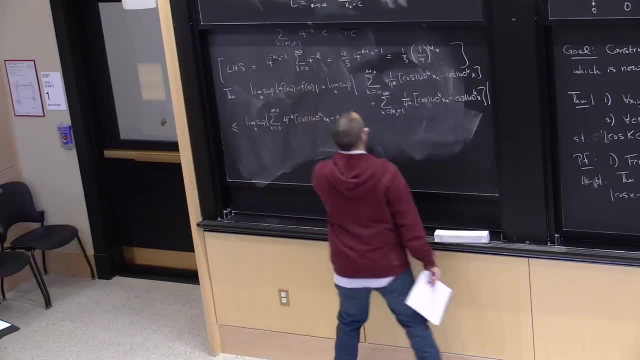 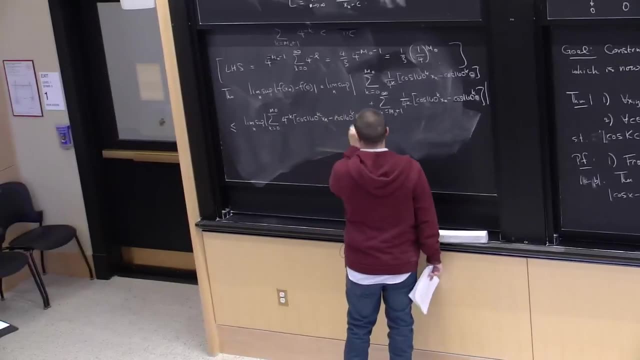 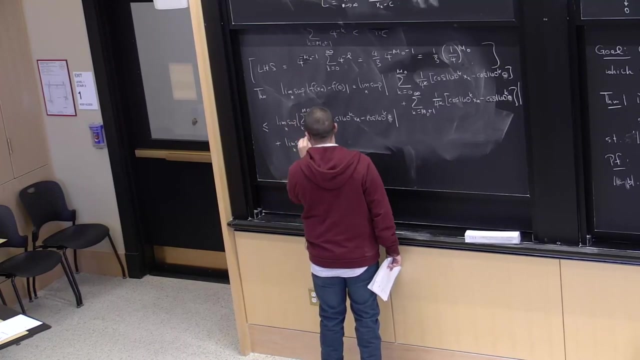 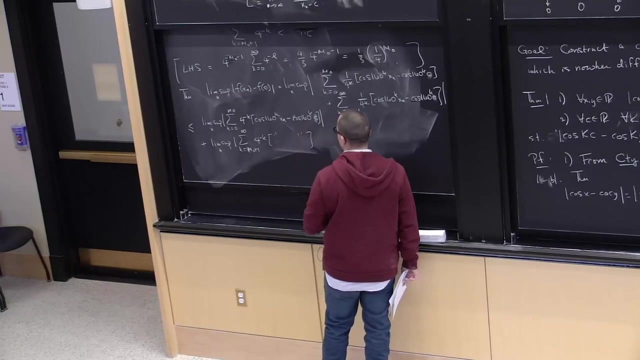 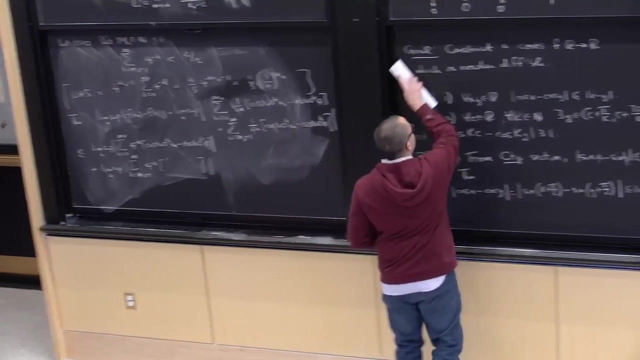 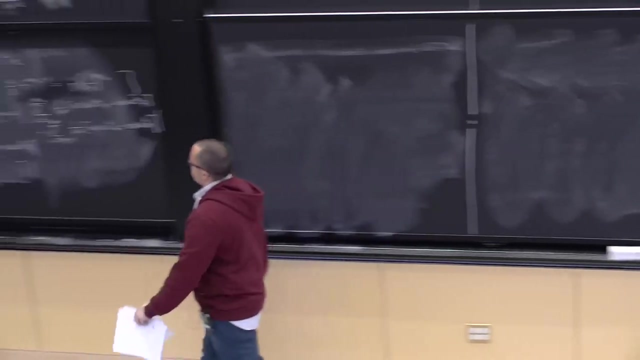 Sorry about that. c, c, c, c. Okay, And then same thing in these brackets here. okay, Now let's see I might keep that All right. so we have that, this limb soup of x of n minus f of c. 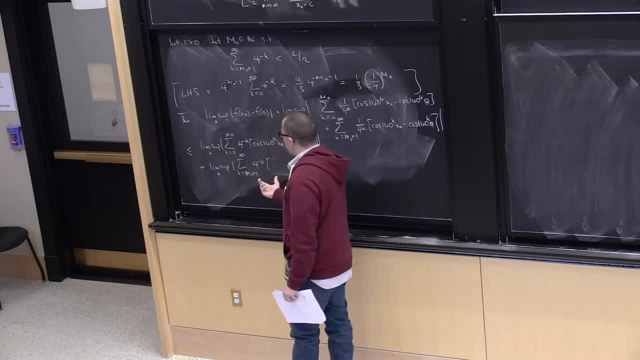 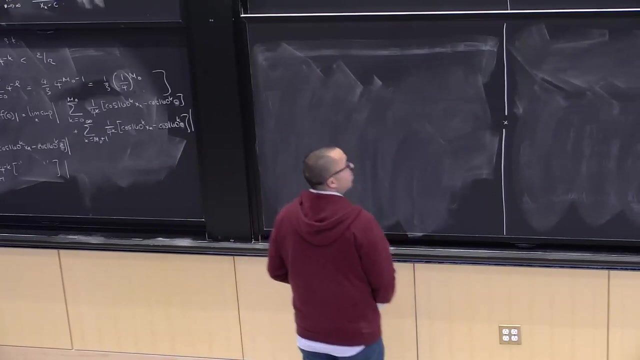 is less than or equal to the limb soup of this guy plus the limb soup of this guy. and now I'm going to use the triangle inequality again, bringing the absolute values inside of the sums, which is perfectly valid even for the infinite sum, by the same argument I used basically over there. 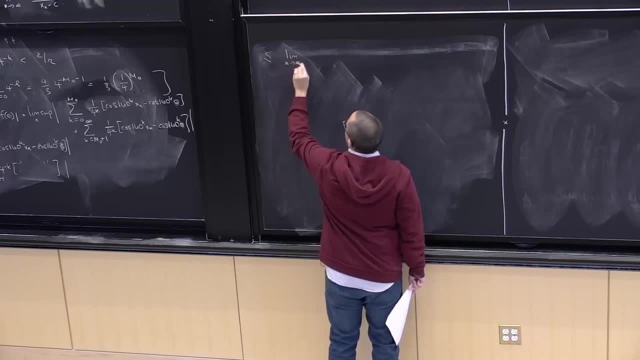 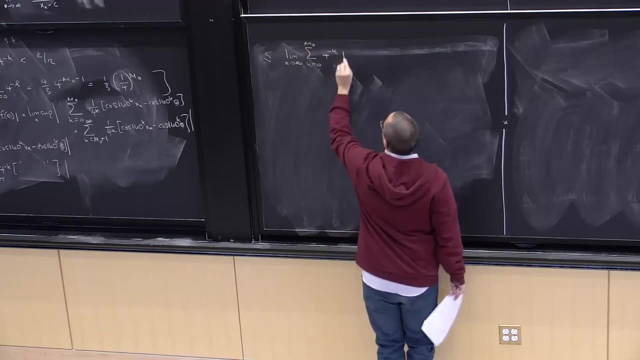 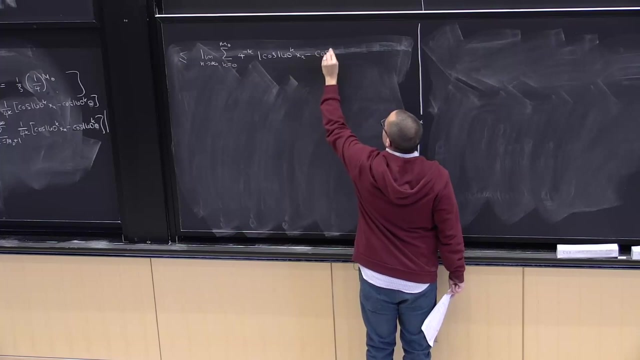 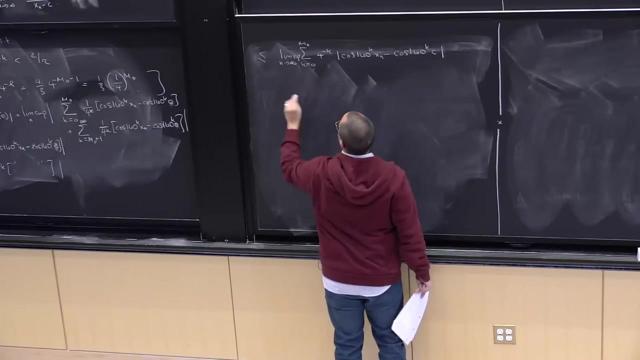 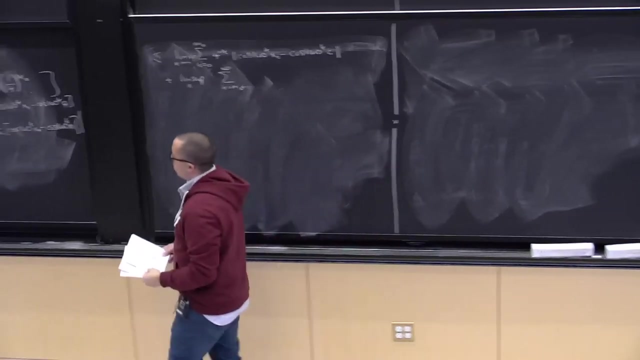 This is less than or equal to the limb soup, as n goes to infinity of Minus cosine of 160k c and soup plus limb soup of sum from k equals m0 plus 1 to infinity of now, the absolute value of the same thing. okay. 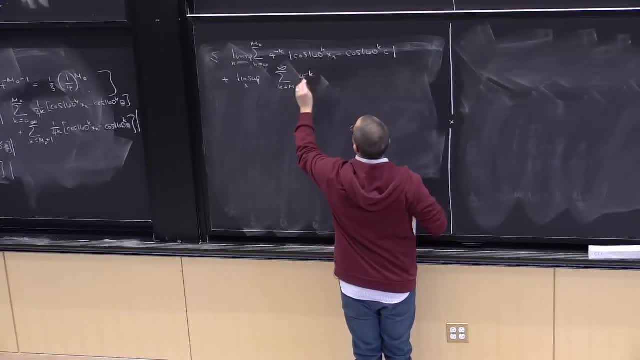 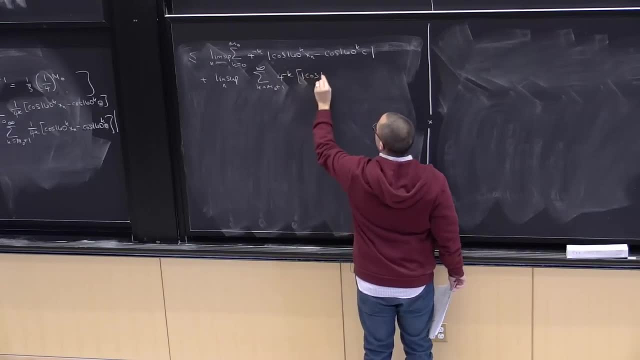 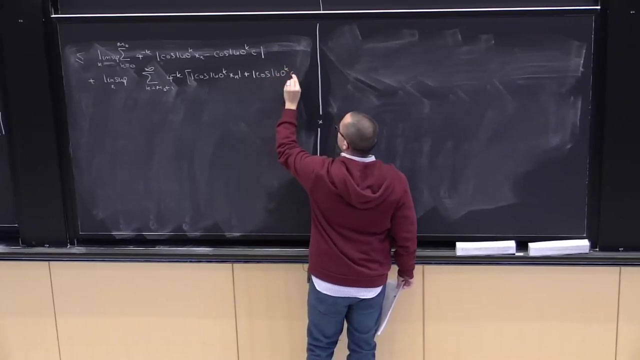 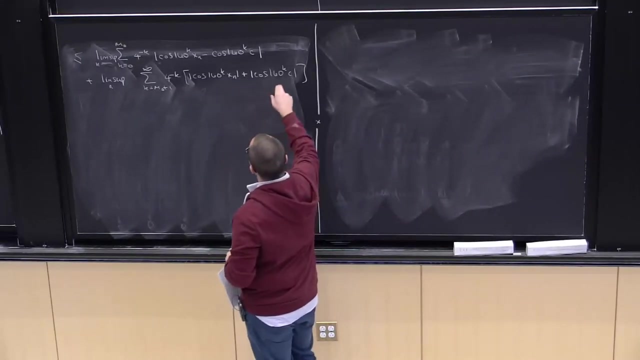 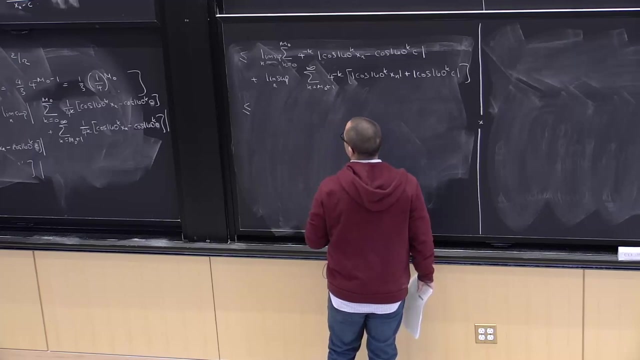 Okay Now I applied the triangle inequality to that. Okay Now, cosine of anything is always bounded by 1, so this is bounded by. first off, let me come back to this second one. m0 is fixed. Remember, this is not changing with n. 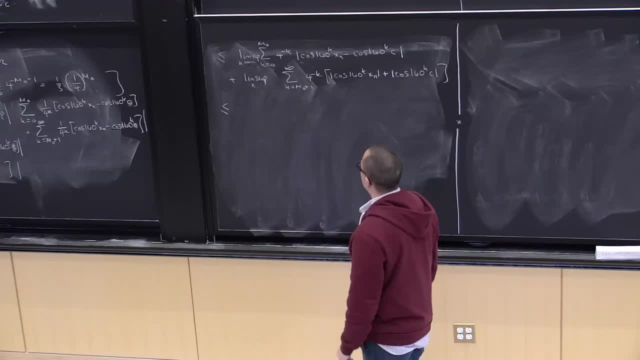 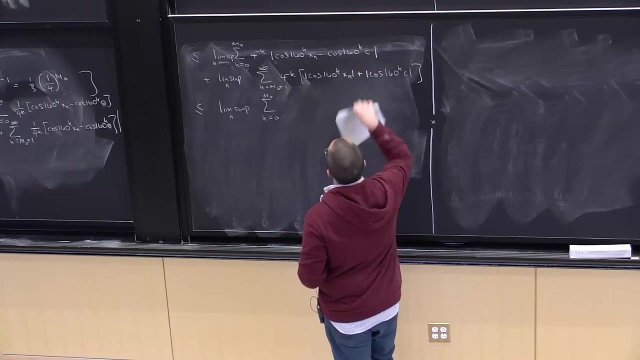 It's just fixed. It depended only on epsilon. okay, So m0 is fixed, and this is less than or equal to limb soup of n. Now we use what we know about cosine: that cosine of something minus cosine of something else. 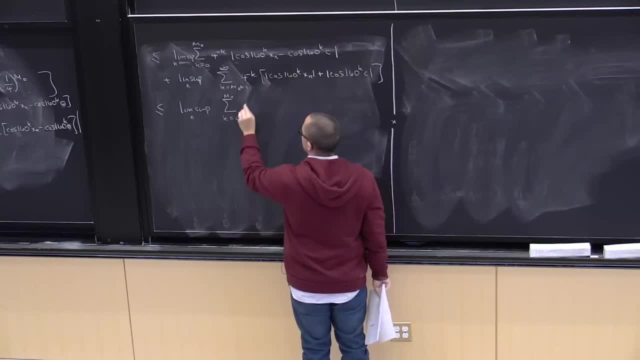 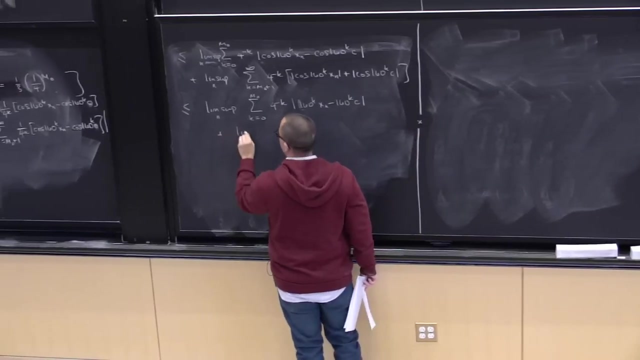 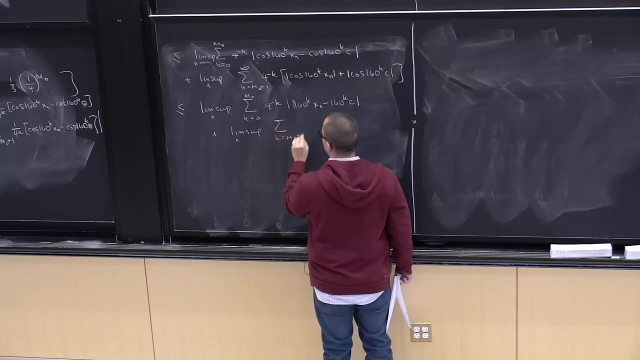 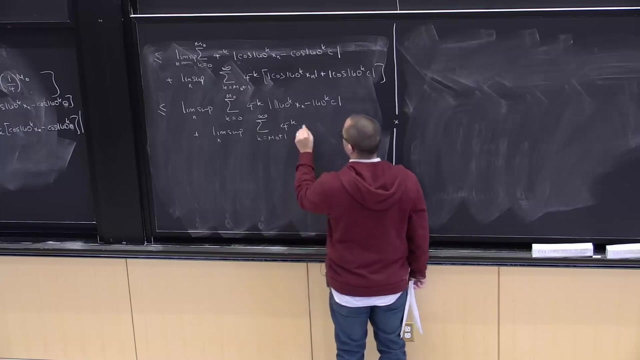 is bounded by the difference in the argument. so this is bounded by minus 4 to the minus k times 160k. xn minus 160k c plus limb soup of k equals m0 plus 1 to infinity 4 minus k times 2,. 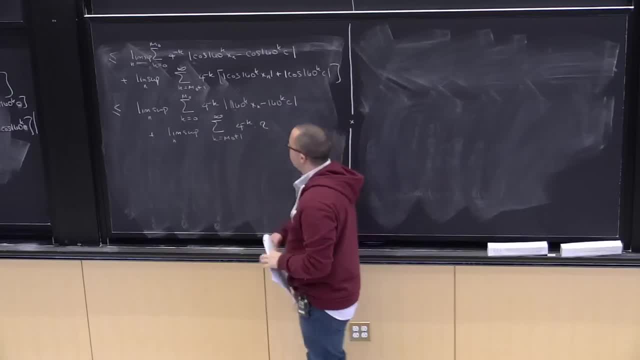 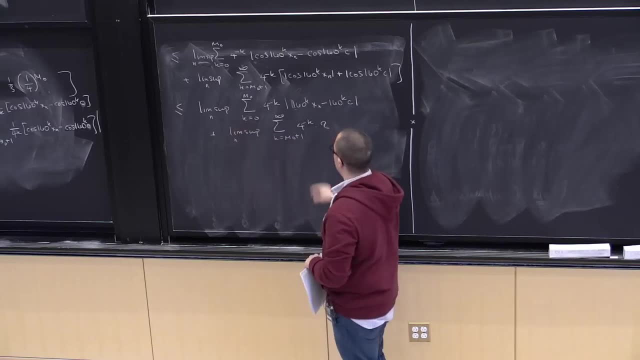 because this is bounded by 1, that's bounded by 1.. Now there's no n left here, so this is really just now equal to that, and we chose m0, so that this quantity here is less than epsilon over 2,. 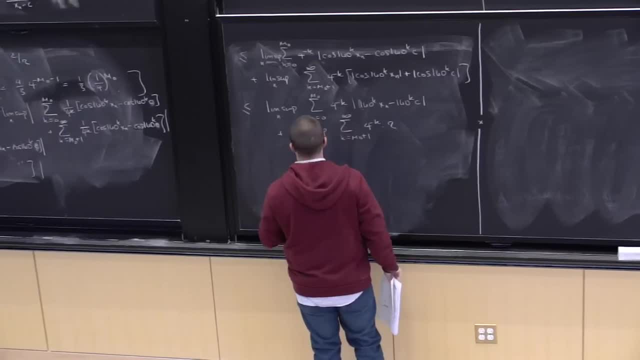 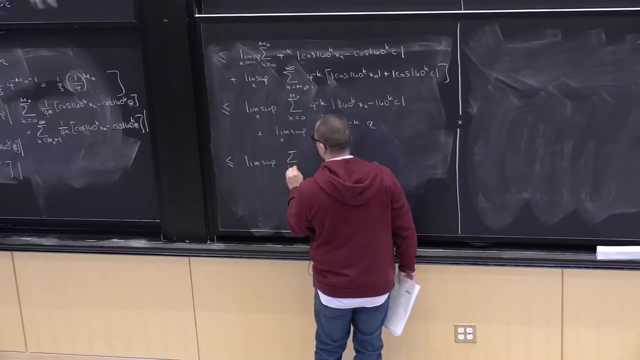 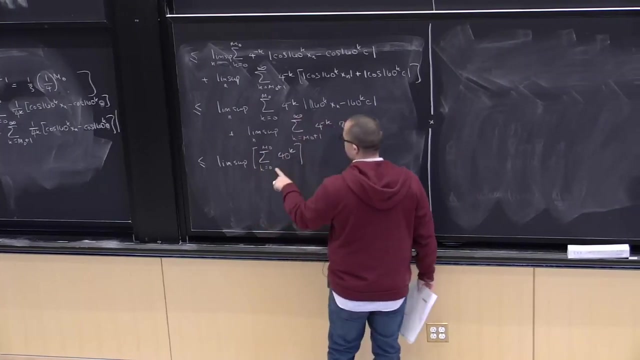 so times 2,. this is less than epsilon. so this is less than or equal to limb soup. sum from k equals 0 to m0 of 40k. Now again, this is just a fixed number, right? The limb soup is in n. yeah. 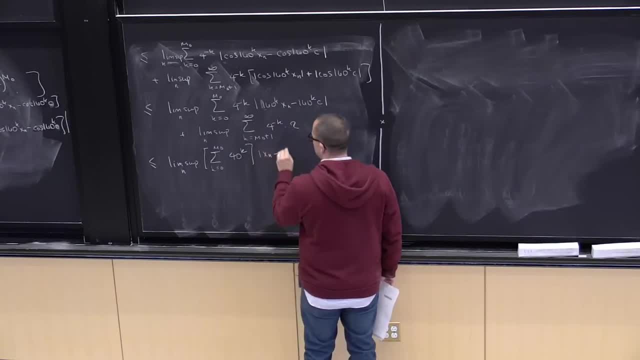 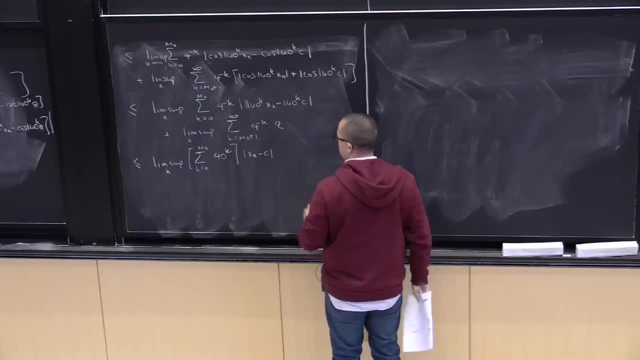 This is just a fixed number: times x of n minus c, right? The difference in this is just equal to 160k times 4 to the minus k, that's 40k. and then we chose m0, so that this quantity over here is less than epsilon. 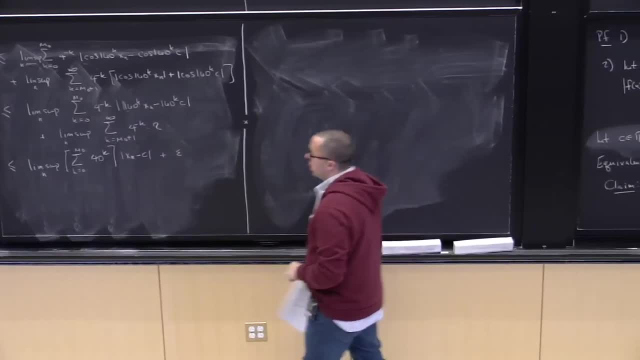 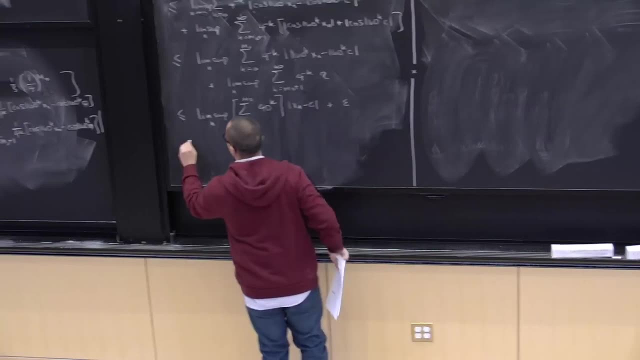 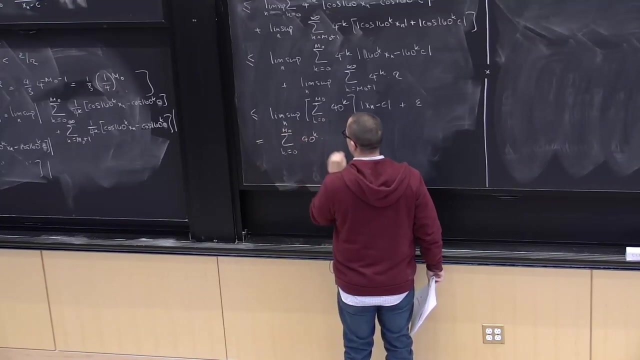 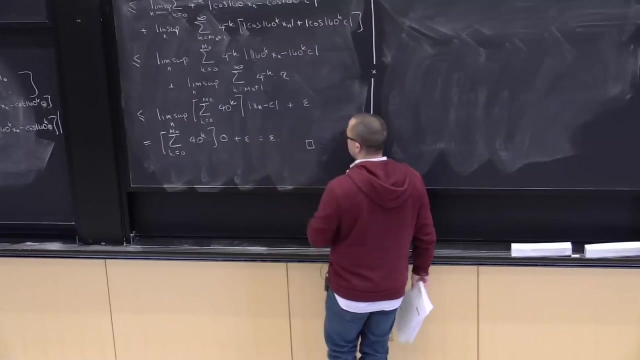 And now, as n goes to infinity, x of n is converted to m0, right, So the x of n is converging to c. So this thing here converges to 0 equals times 0, plus epsilon equals epsilon. 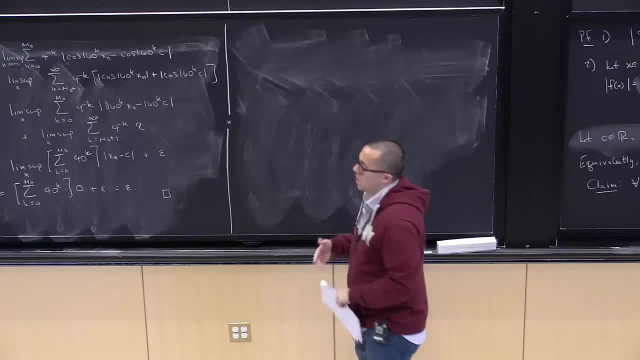 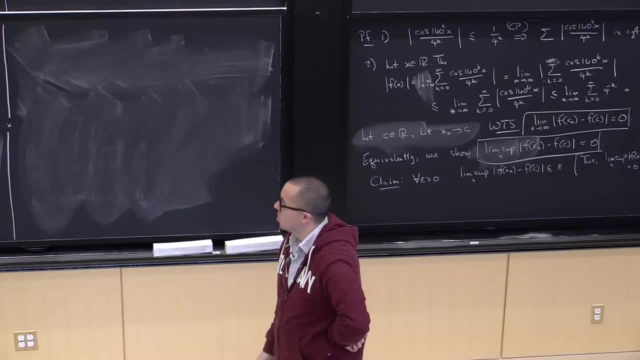 So you know, to me this is a real first proof of analysis where kind of you're using everything that you've been exposed to up to this point, right to this point, to prove a really deep theorem. So go through this slowly, but the estimates. 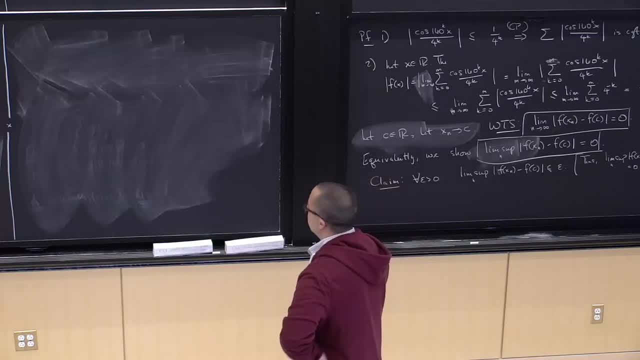 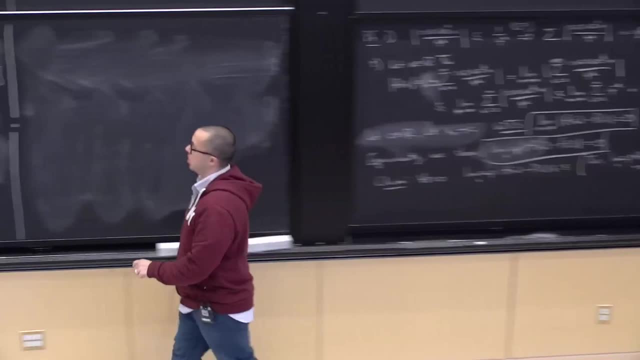 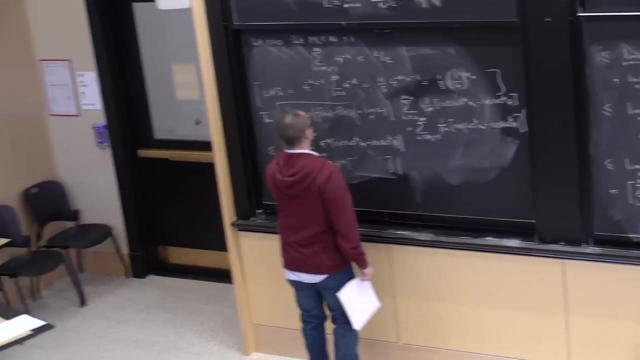 are not all that tricky once you have them in front of you. So we've shown that, for all epsilon, this Lemp's soup is less than or equal to epsilon, because, remember, we ended with epsilon here But we started off estimating this Lemp's soup here. 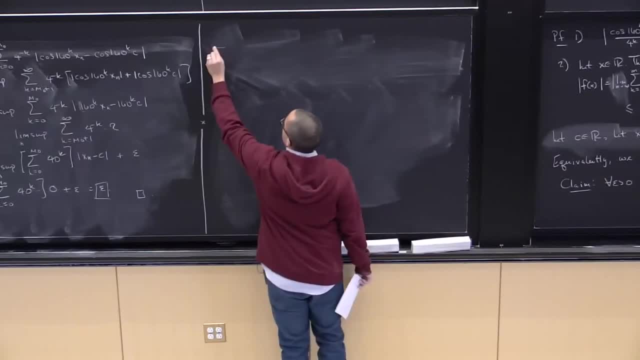 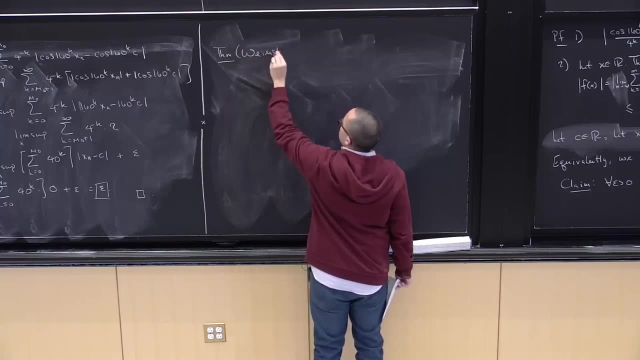 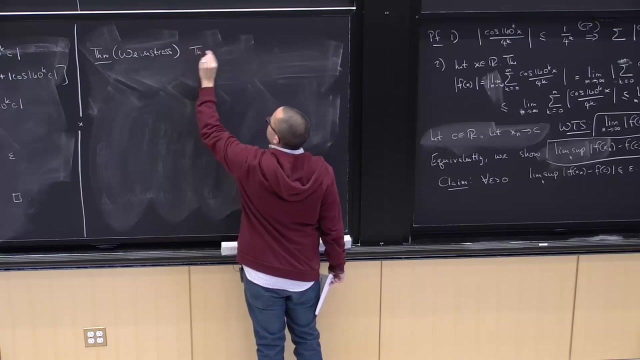 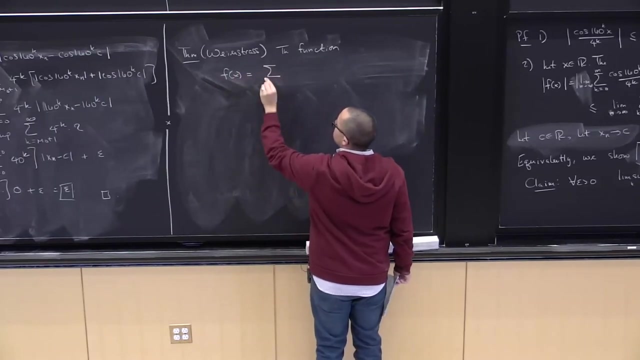 Now we're in a position to prove the final theorem that we want to prove, and this is due to Weierstrass. So it's a function which we've been studying: f of x equals sum from k equals 0 to infinity. cosine 160kx. 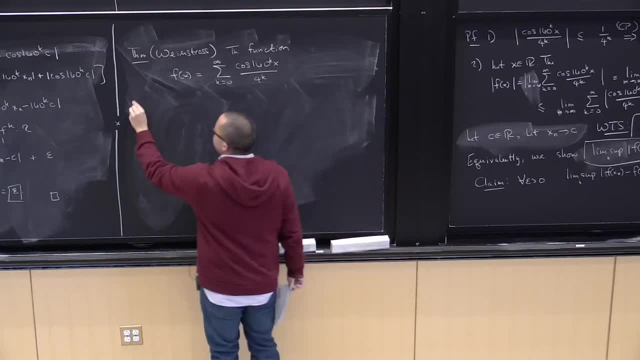 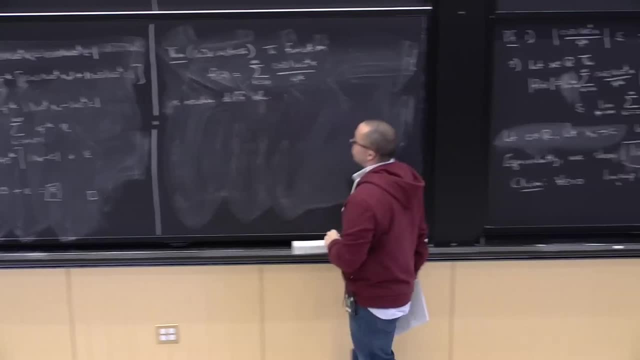 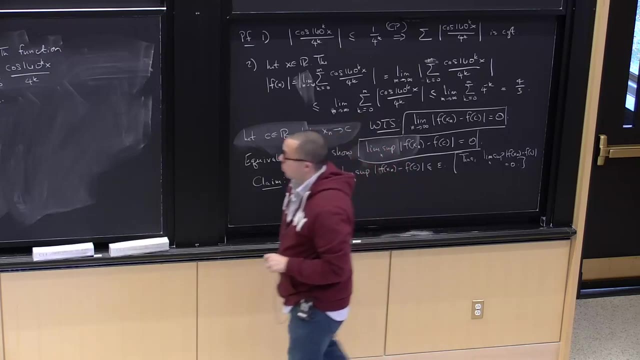 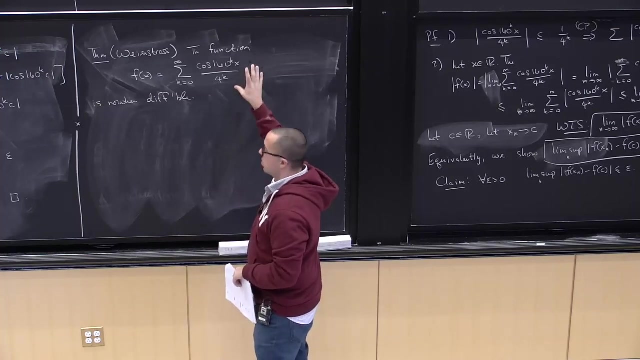 over 4 to the k is nowhere differentiable. OK, All right, So you know, with everything we've done so far, So we know this function is continuous, right, We've proven that. So this example, so this theorem, provides you. 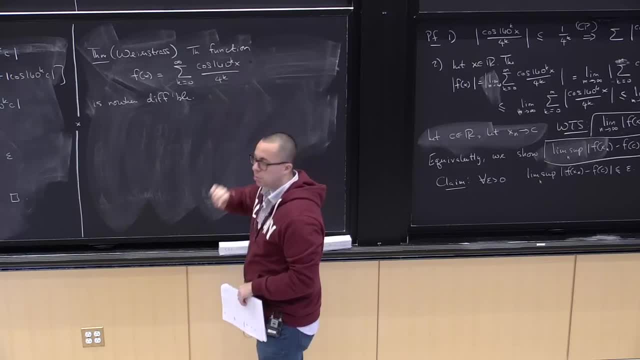 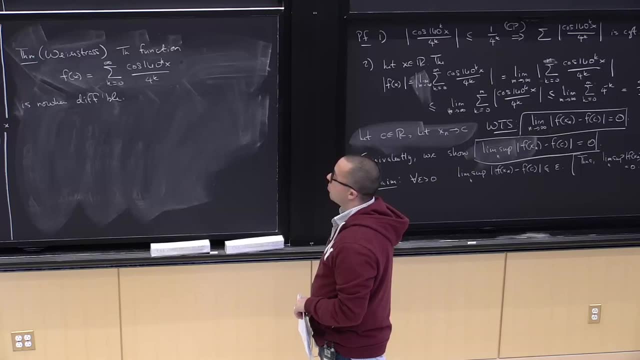 with an example of a function which is continuous but nowhere differentiable And with what we have on the board, namely, you know, the key parts are gonna be what's in that first theorem there, And this triangle inequality we have over here will be able to prove this. 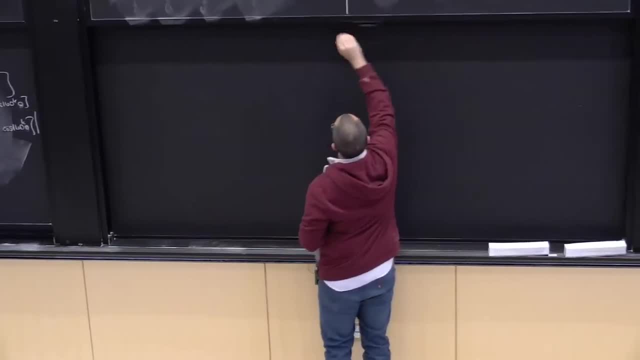 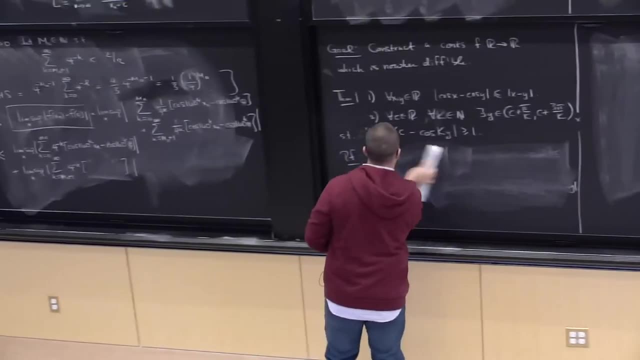 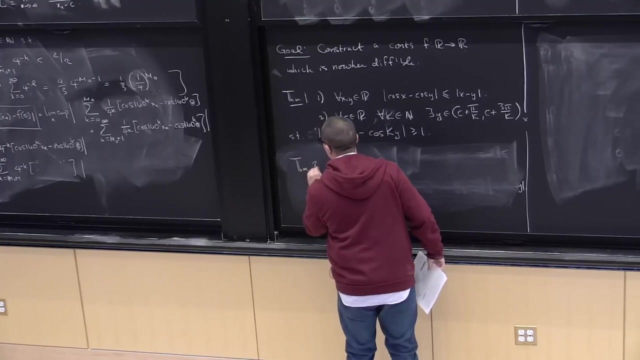 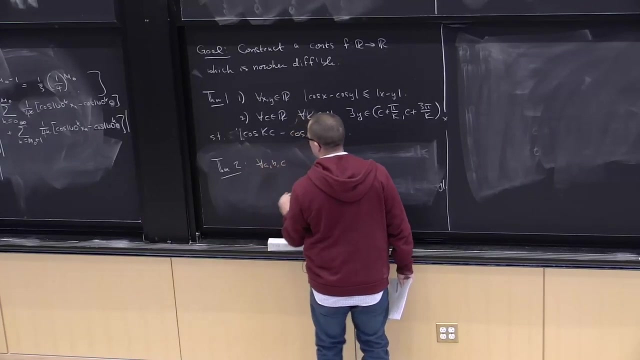 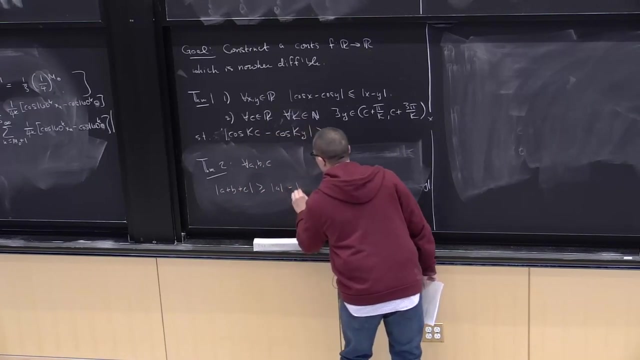 So, in fact, let me give myself a little space And I'm gonna state theorem two from over there, because I need some space to write in a minute For all. a, b, c. the absolute value of a plus b plus c is bigger than or equal to a minus the absolute value of b. 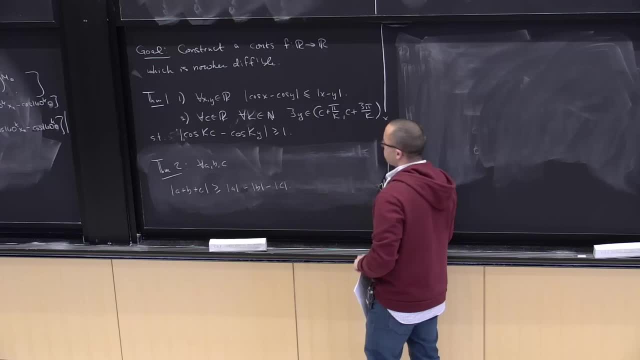 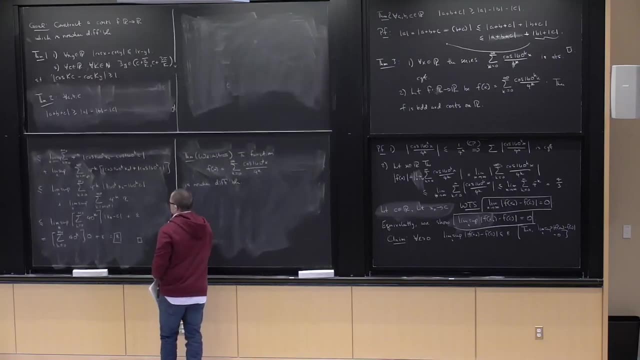 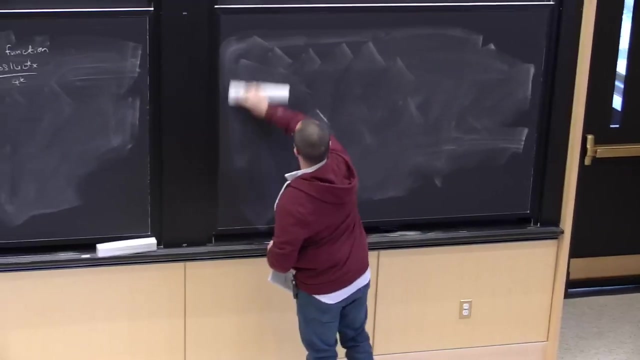 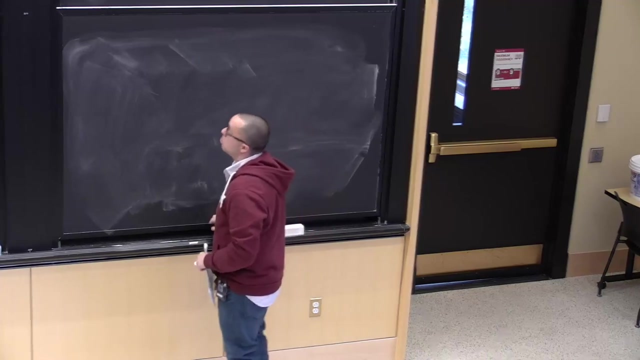 minus the absolute value of c. all right, All right. so let me re. let me re-summarize, since I've summarized it already, what we've done. We've gone from this point to this point. We've shown that this function here is well defined. 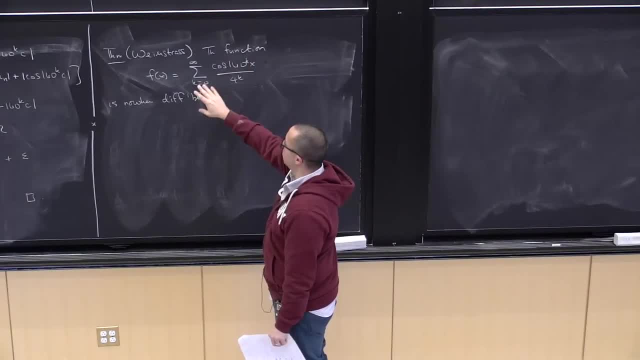 absolutely conver. this series is always absolutely convergent and therefore this function is bounded and or. we also proved that it's bounded and continuous. right, That was the previous theorem. So this function is bounded and continuous, and we're going to prove. it's nowhere differentiable. 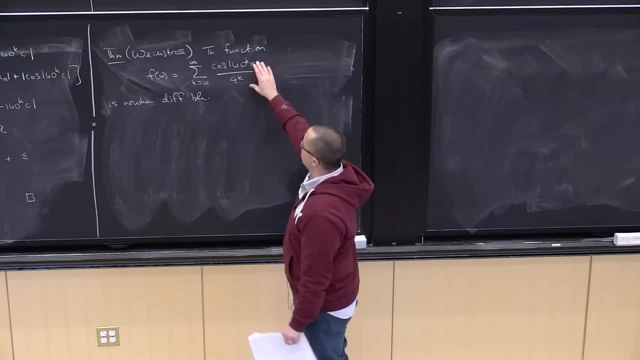 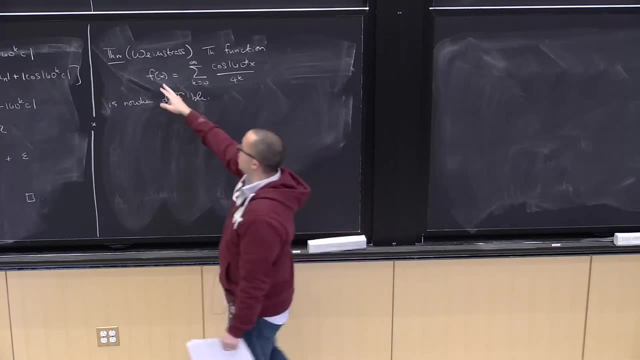 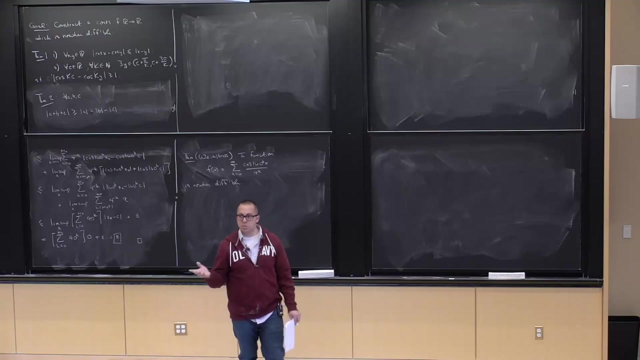 And again, what's the idea? The idea is that we built it out of functions which are highly oscillatory at smaller and smaller degrees, scales. So somehow this function is highly oscillatory at every scale. And if you have a function which is highly oscillatory of every scale, if some of you have heard of 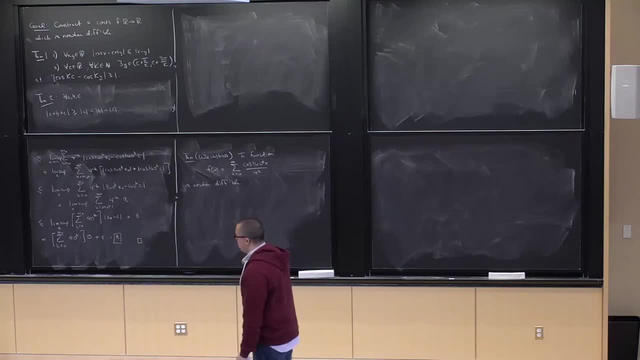 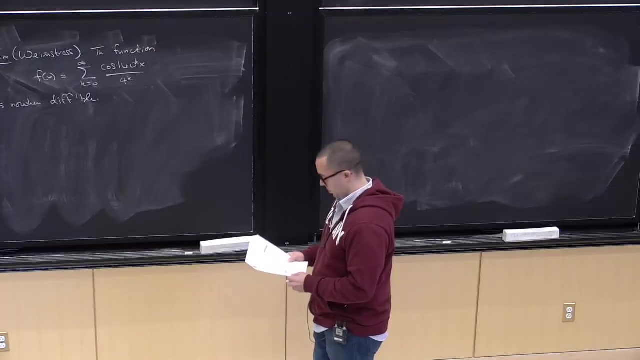 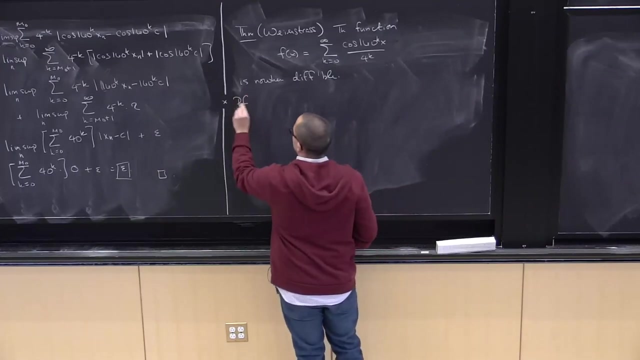 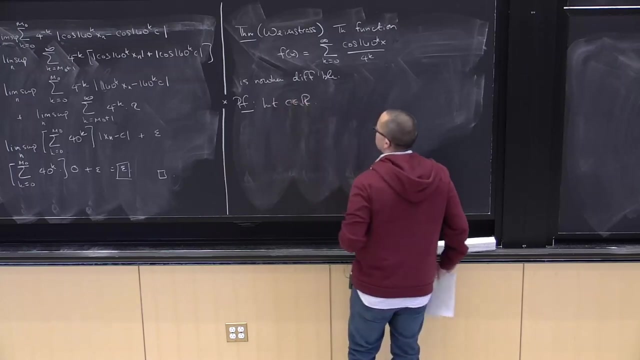 Brownian motion, which is a path which is highly oscillatory, then that function will not be differentiable anywhere. So proof, let's see be any real number And what we're going to do, just as in when we looked at f of x equals the absolute value of x. we're. 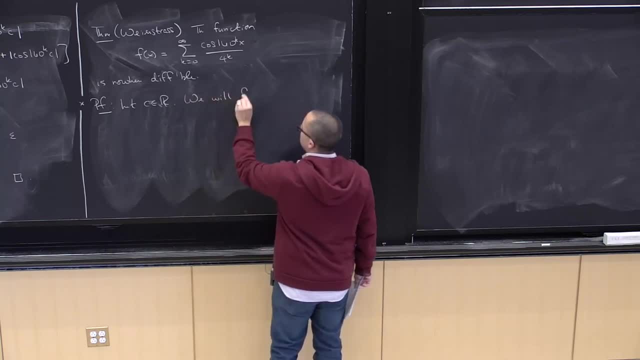 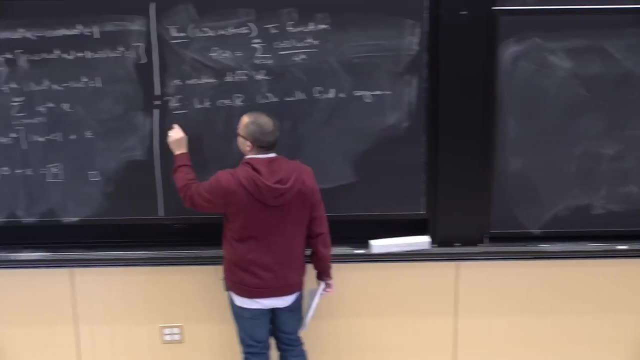 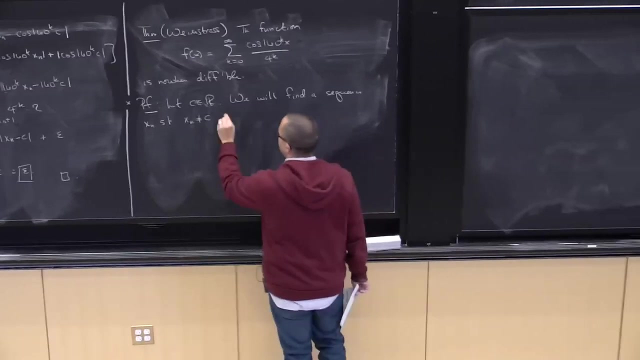 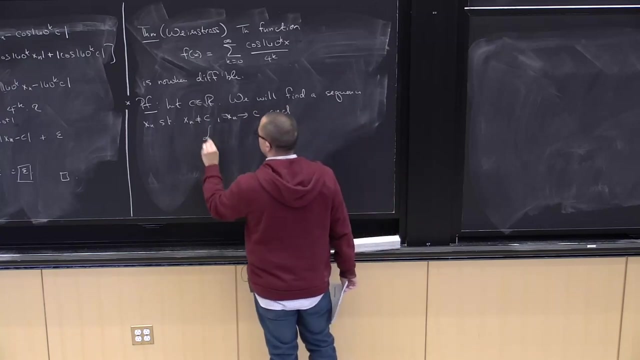 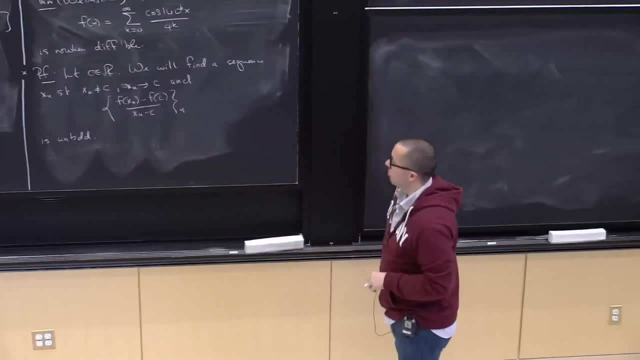 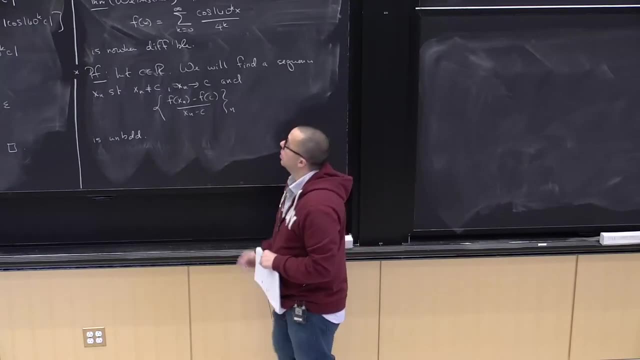 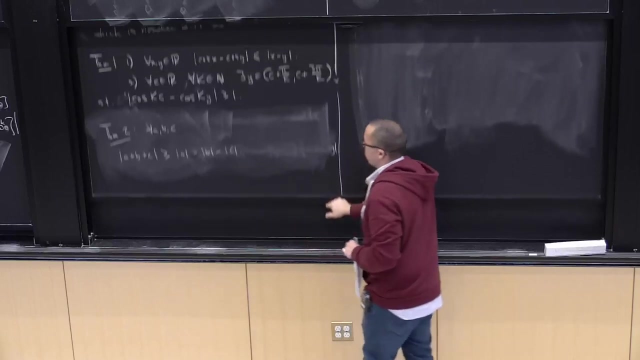 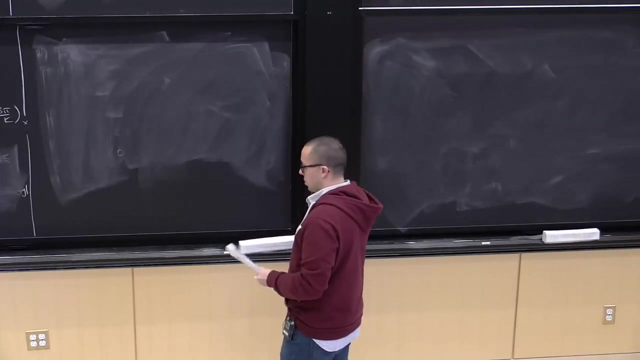 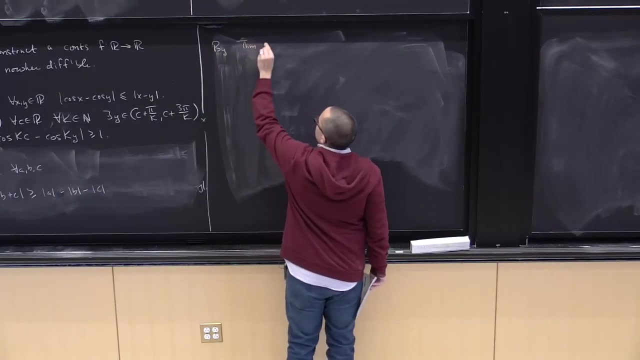 We'll go even further. So f of x is unbounded And therefore the sequence cannot converge And therefore the function is not differentiable at c. So we're going to use theorem one to find the sequence OK by theorem 1, namely part 2,. 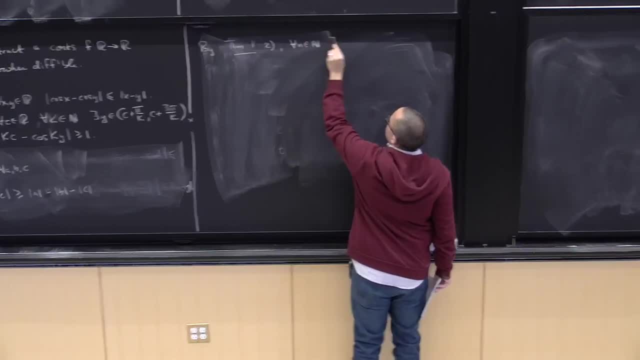 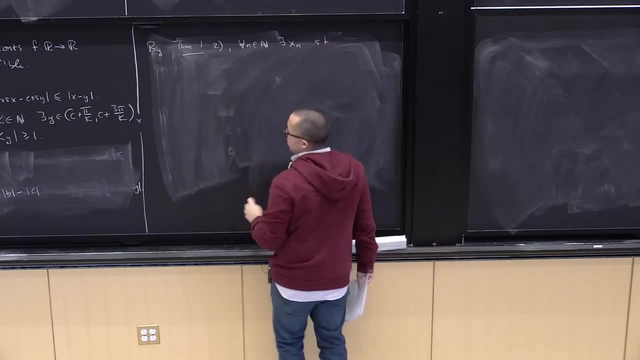 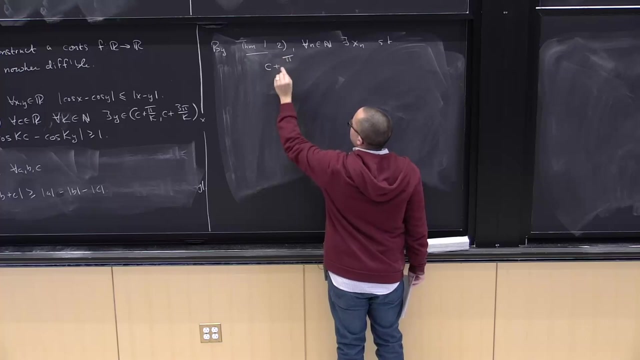 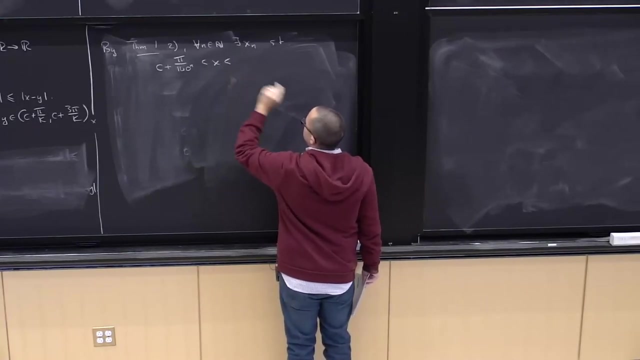 all in a natural number, There exists an x of n, such that what x of n is in this interval of the form? so c plus pi over 160n is less than x, is less than c plus 3 pi over 160n. 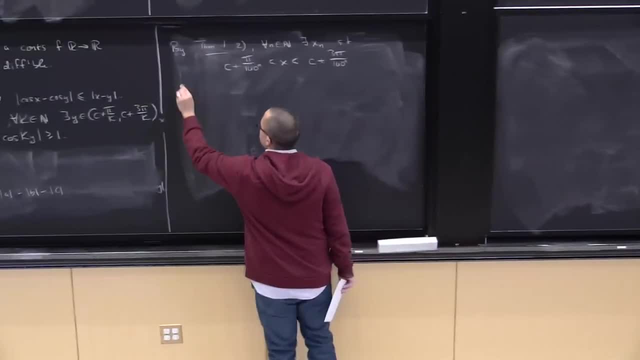 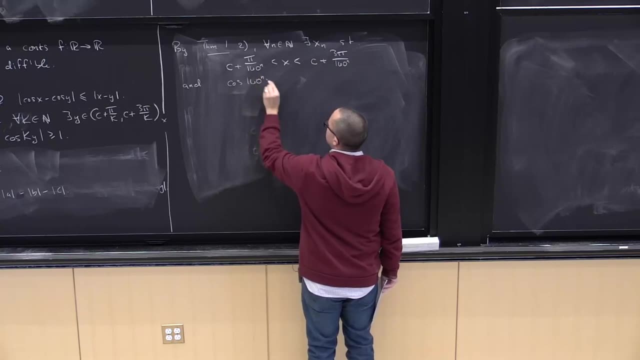 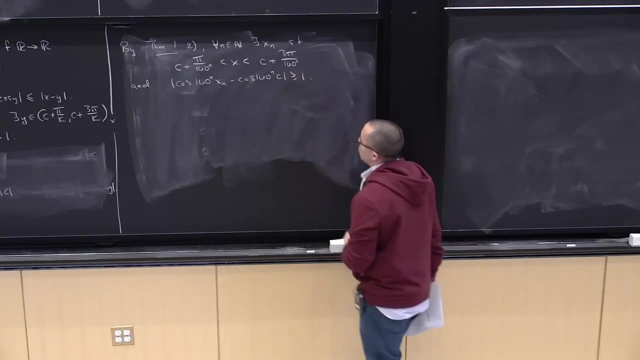 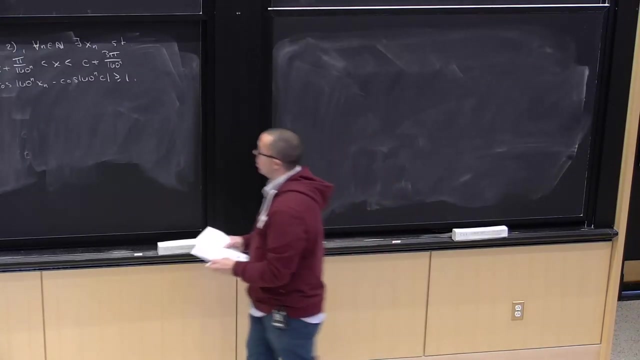 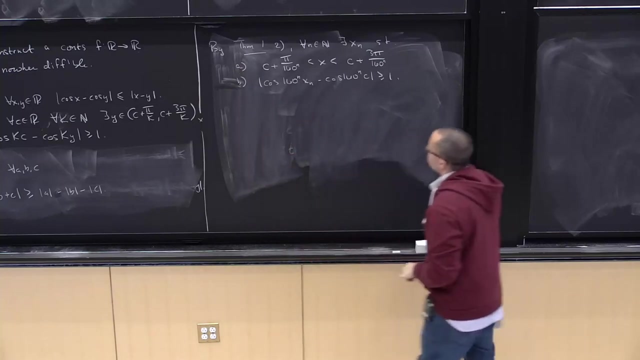 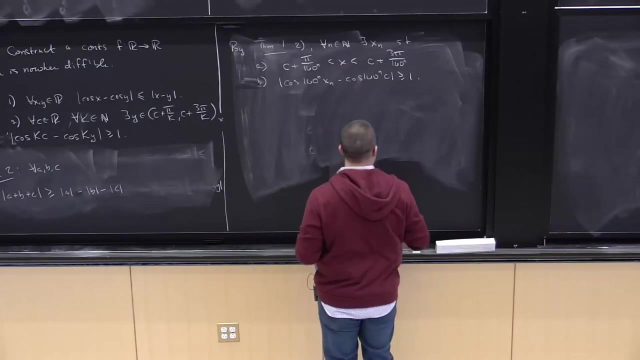 Okay, And cosine of 160n x of n minus cosine of 160n c is bigger than or equal to 1.. Okay, So let me call these two properties A and B. So another way of writing A is we could have instead written: 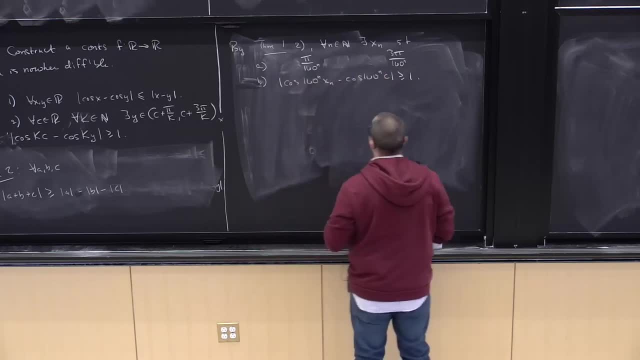 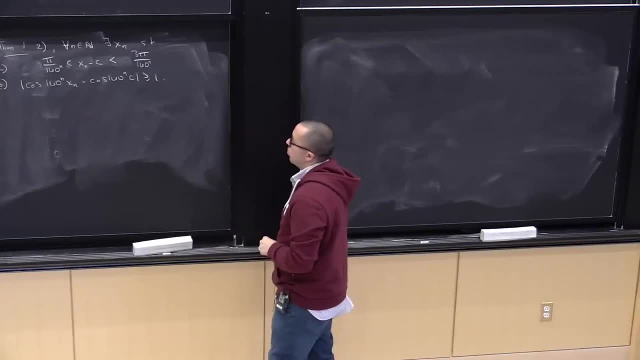 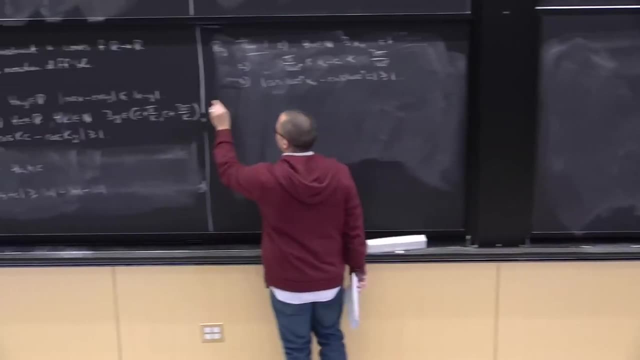 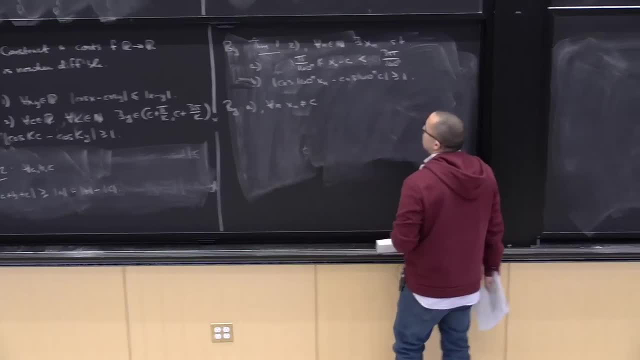 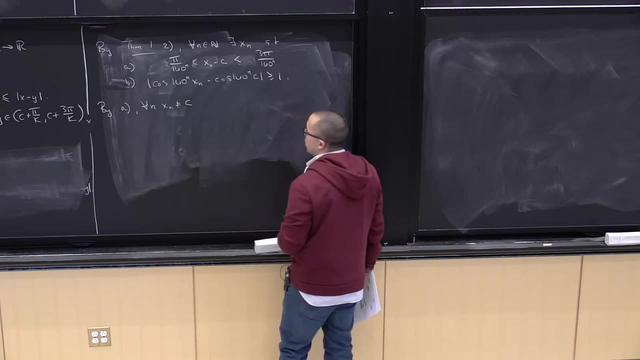 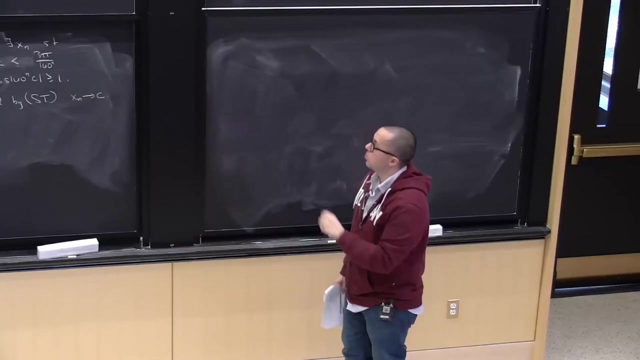 because their difference is bounded below by a positive number. I mean, their difference is actually positive and it's non-zero. so, And by the squeeze theorem, you know again, if you like, putting the C on both sides, we get that X sub n converges to C. So this will be our sequence, our bad sequence, for which? 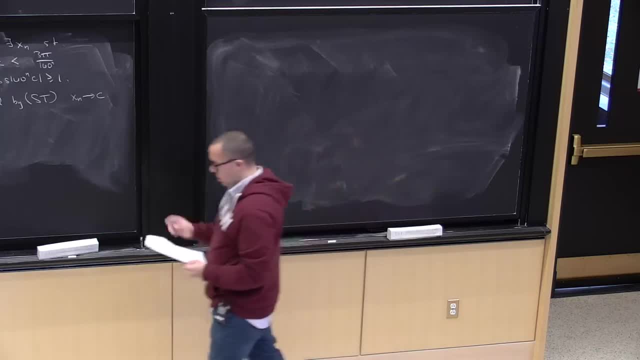 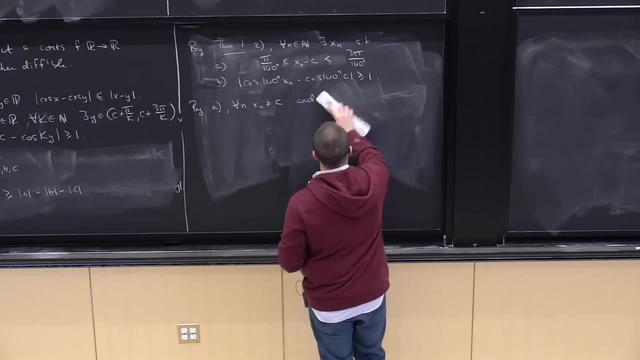 the difference quotient is unbounded. Okay, So in fact, let me write this out a little bit more. And X sub n minus C, which is equal to X sub n minus C, because this is positive, is less than 3 phi over 160 n. 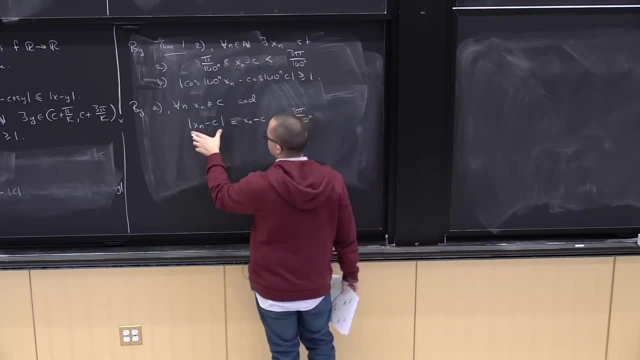 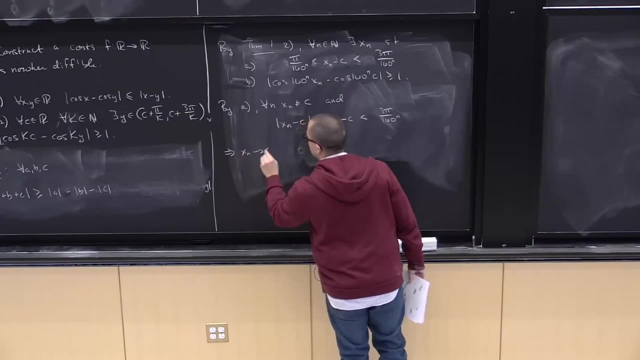 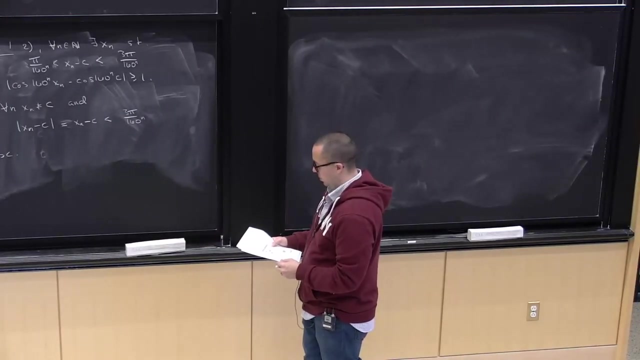 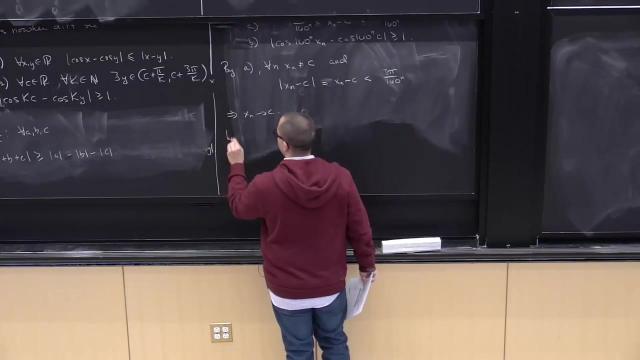 Okay, And this goes to zero. therefore, the absolute value of X sub n minus C converges to zero, and therefore X sub n converges to C. Okay, All right now, to lessen the number of times I have to write cosine 160k, let fk of X be. 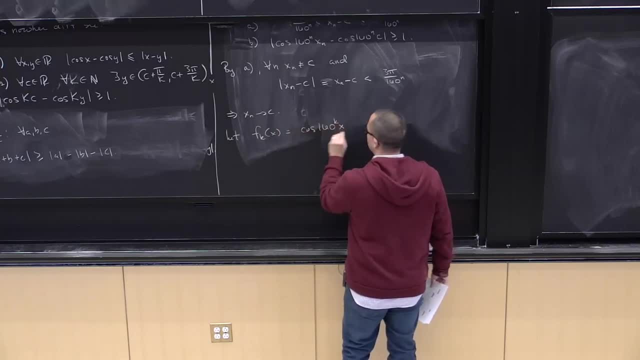 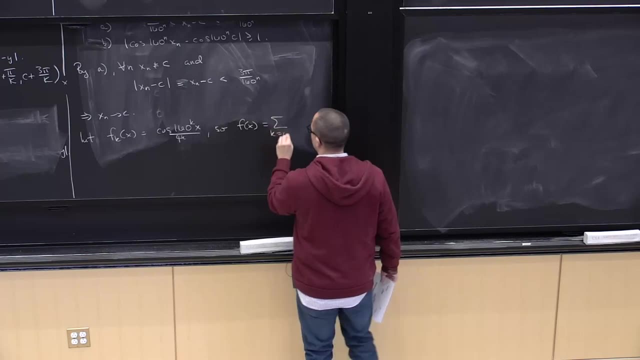 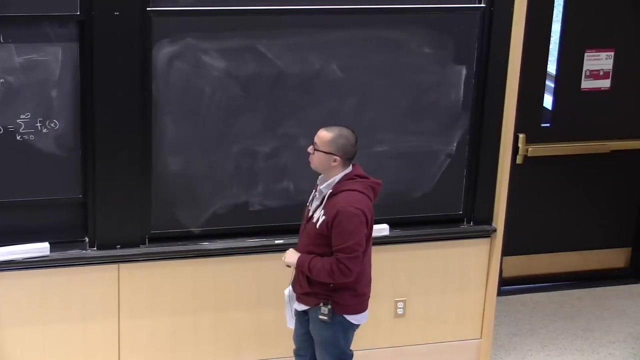 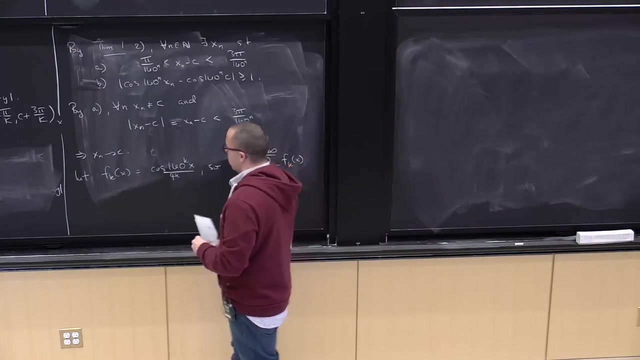 cosine 160k. Okay, X over 4 to the k. So f of X is equal to the sum of k, equal to zero of fk of X. all right, And now? what we're going to do is we're going to find a lower bound on the absolute value. 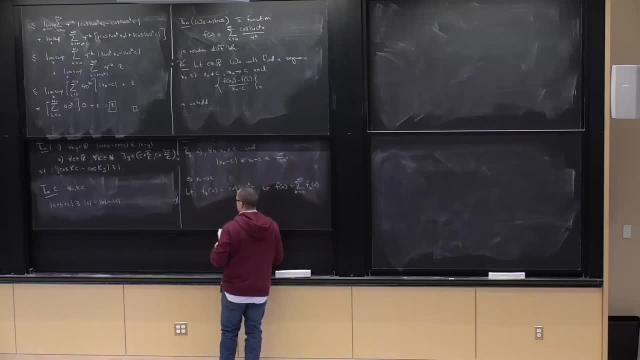 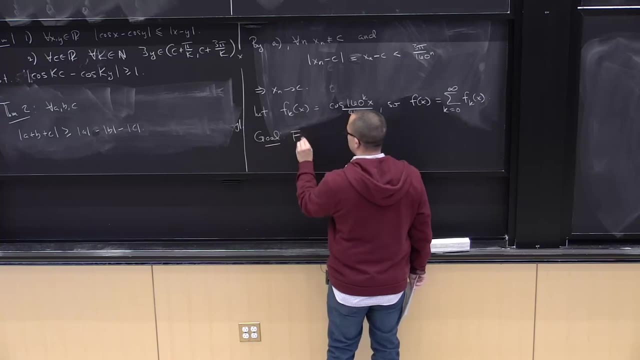 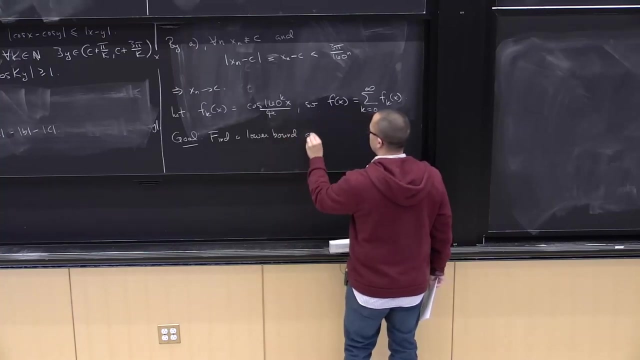 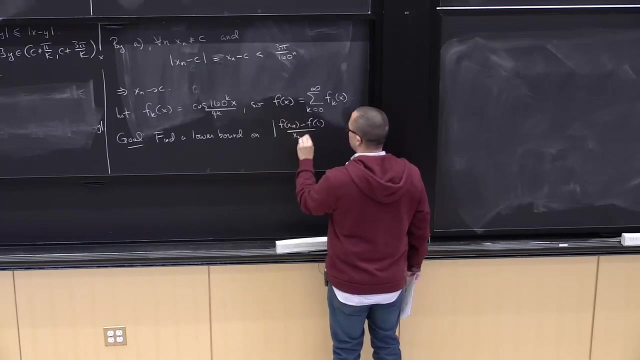 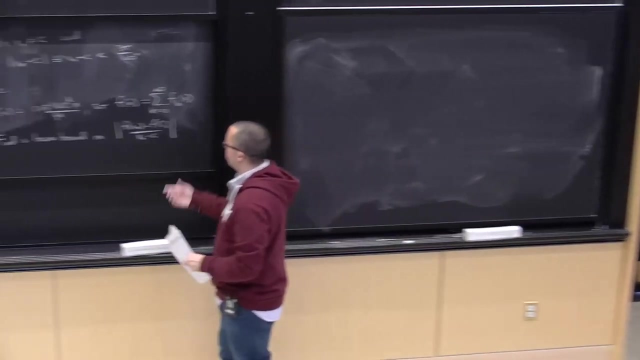 of f of X, n minus f of C over X sub n minus C converges to zero. Okay, So that's going to be phi over X of n minus C. So now Find a lower bound on. Okay. Okay, If I can find a lower bound on this absolute value which? 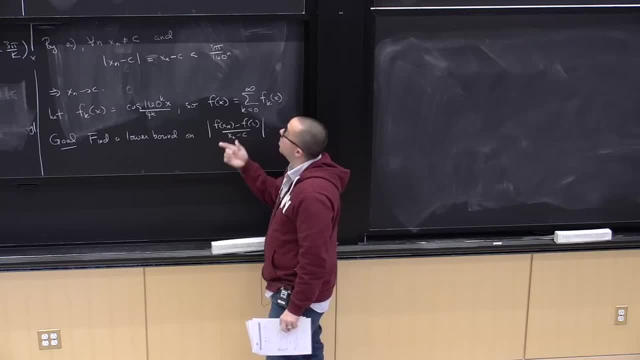 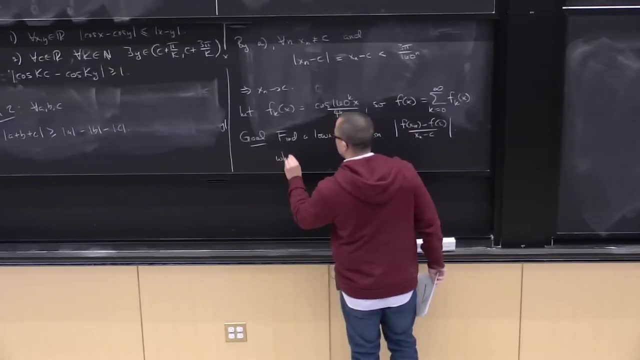 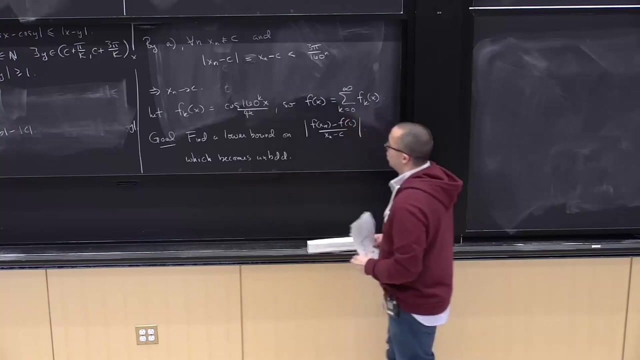 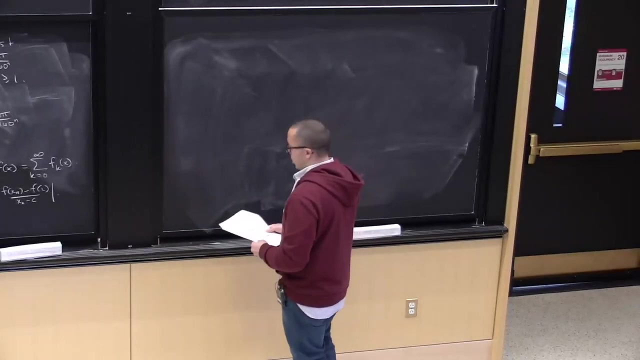 is getting large, as large as I wish, then that proves that this sequence is unbounded and I'm done, OK, OK, So let's look at the absolute value of f of xn minus f of c. Let's just write this: 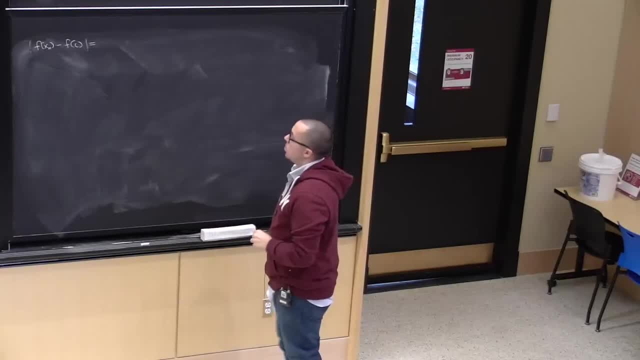 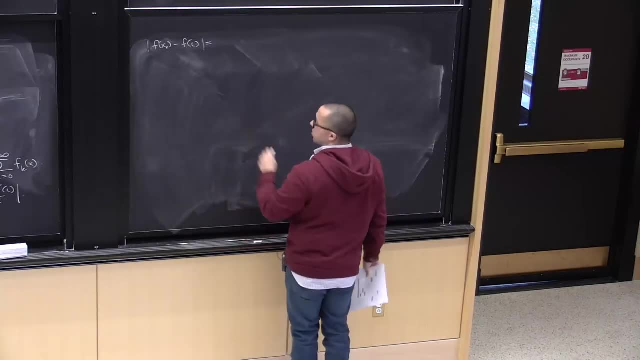 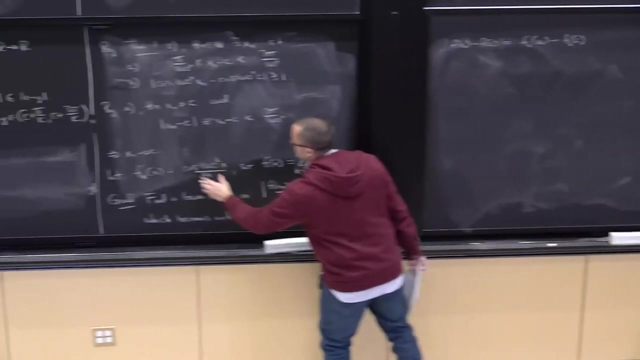 And In a few different ways, or not a few different ways, but let's split it up as a sum. So all of these guys are equal to sum of f sub k. So I have the nth one. So remember f sub k. this is just one of these building. 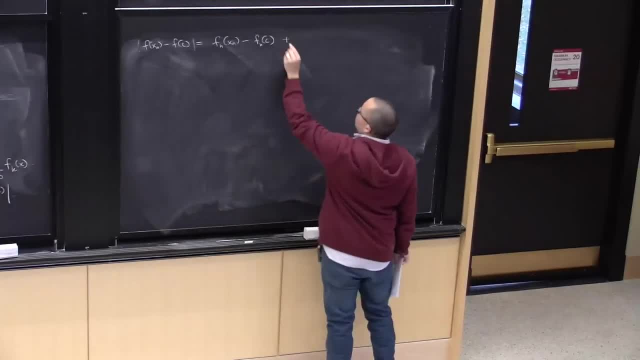 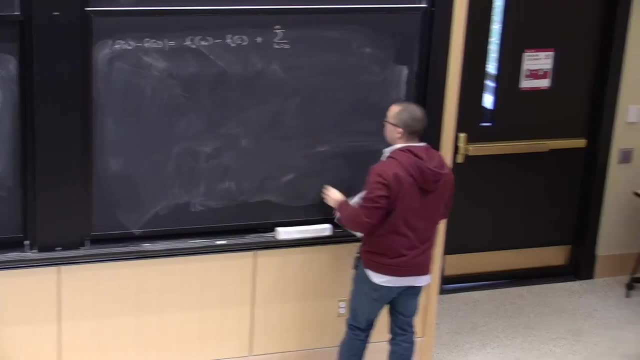 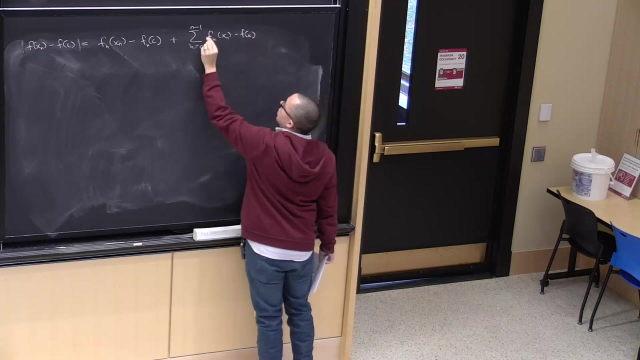 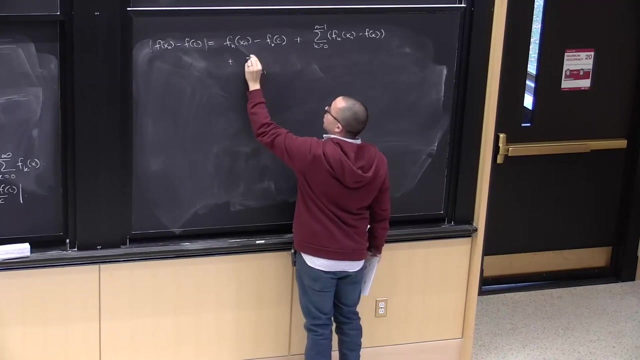 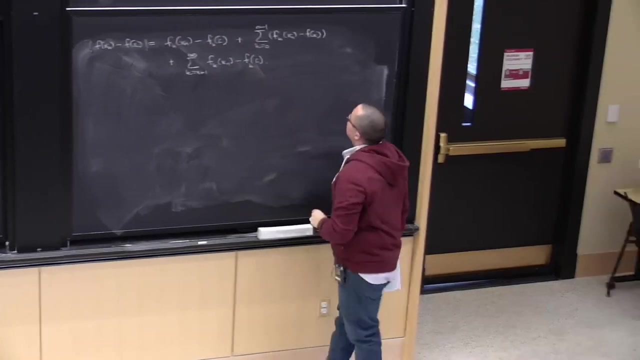 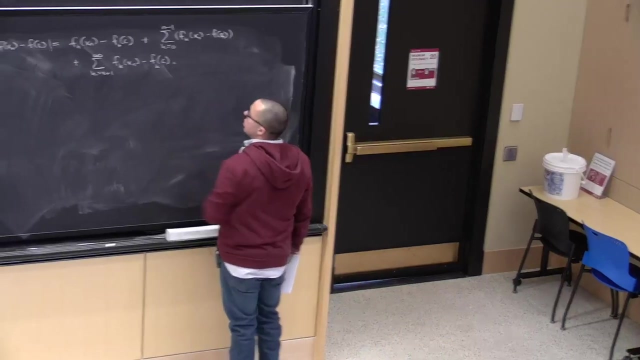 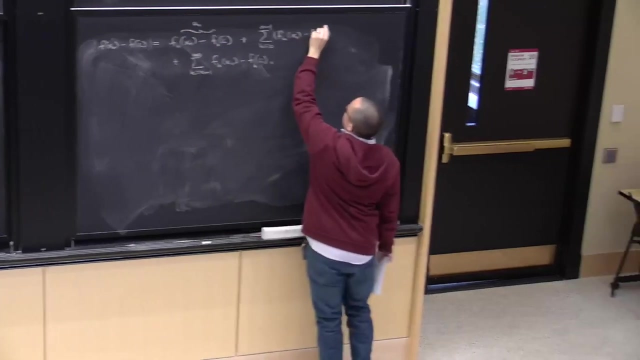 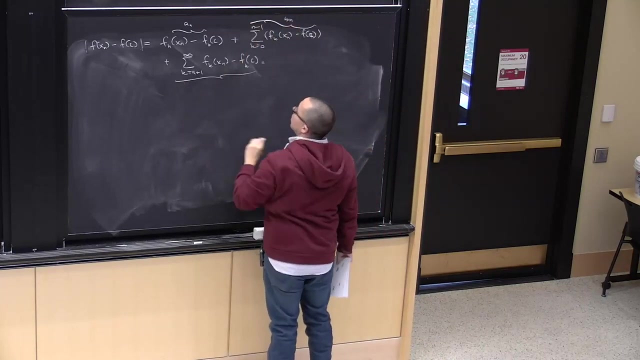 blocks plus sum from. So k equals 0 to n minus 1, plus put an x here. I meant to write c, And so I'm going to let a sub n be this first number, b sub n be the second number, including the sum. 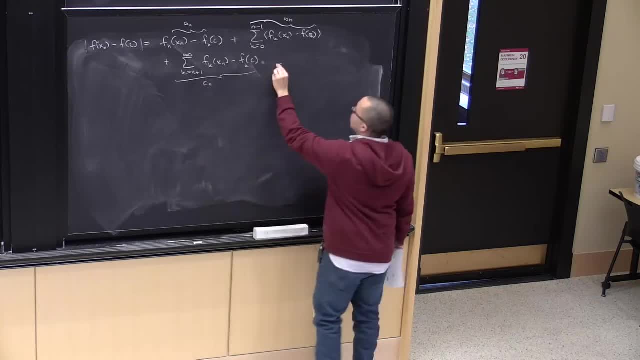 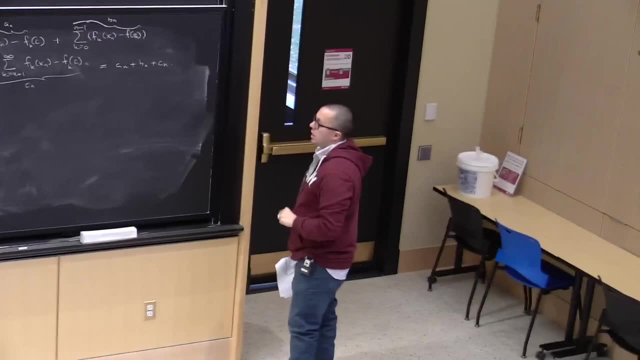 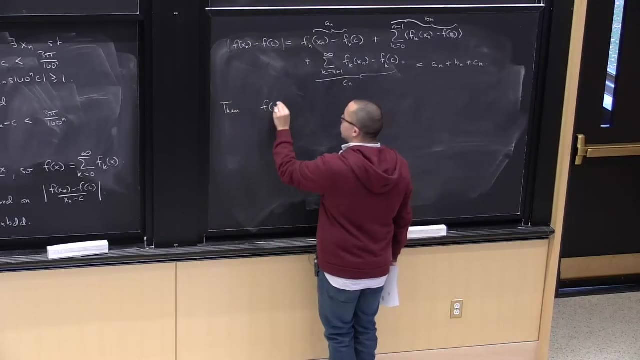 And this will be c sub n. So this is equal to a sub n plus b sub n plus c sub n. And now I'm going to use that triangle inequality I've proved Then f of x sub n minus f of c is greater than. 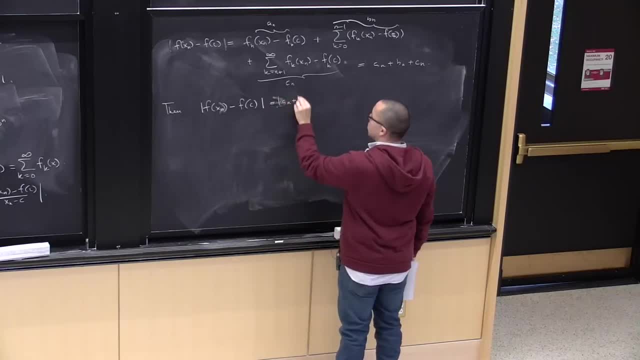 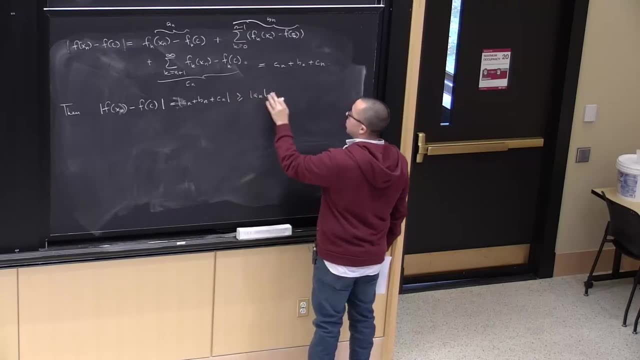 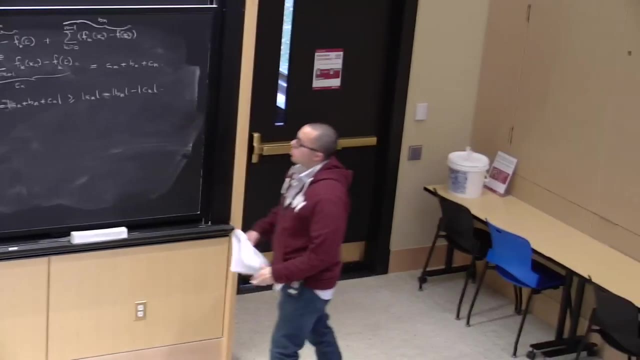 which is equal to a sub n plus b. sub n plus c. sub n is bigger than or equal to a sub n minus b. sub n minus c sub n. OK, Now, a sub n. This is going to be. This is just the difference between these guys. 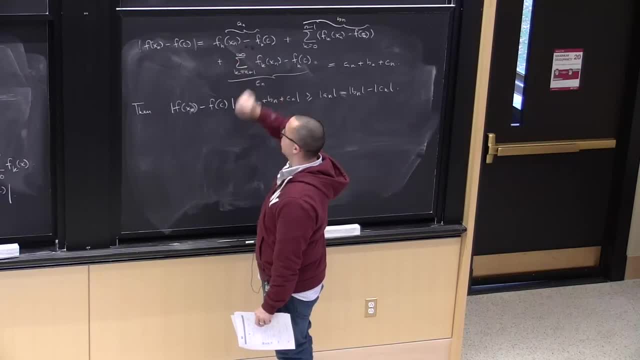 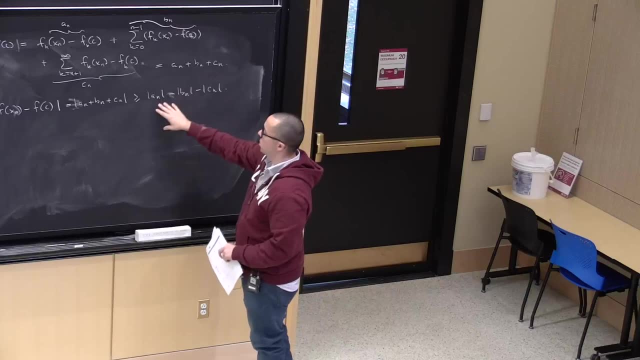 This is bounded below by 1.. So it's kind of large, Not 1, but 1 over 4 to the n. These other guys we'll prove are very small compared to the a sub n. And then this lower bound, this upper bound we have on x sub n. 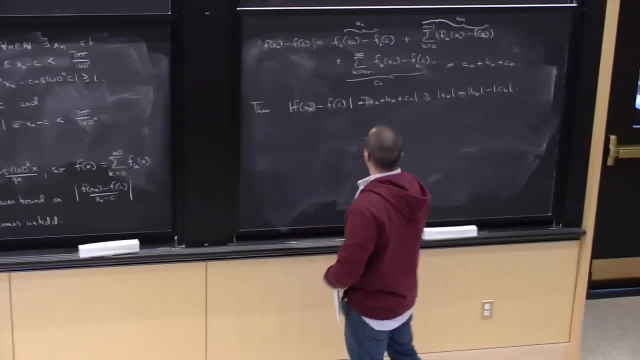 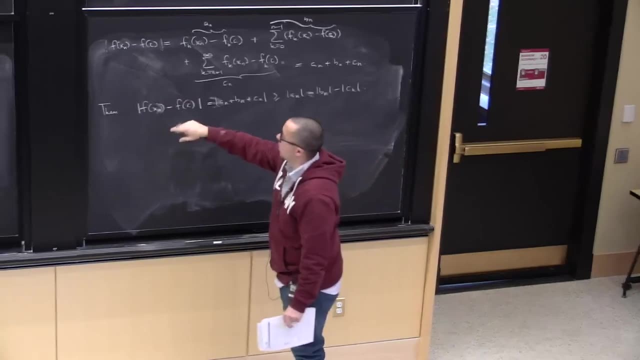 minus c will be the nail in the coffin, as we see. So our goal is now to estimate from below a sub n. Remember we're trying to find a lower bound for this quantity over x sub n minus c, So we need to estimate these things from below. 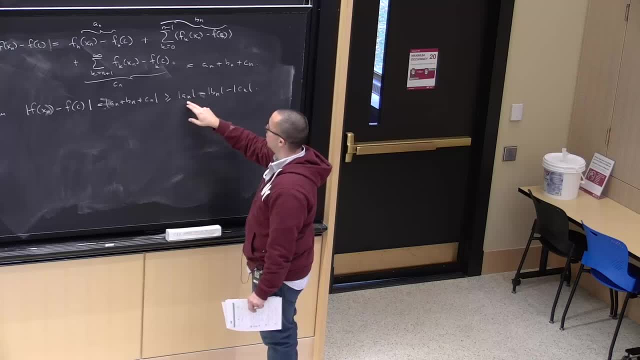 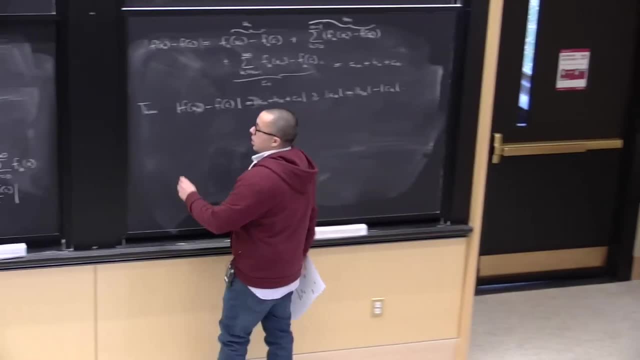 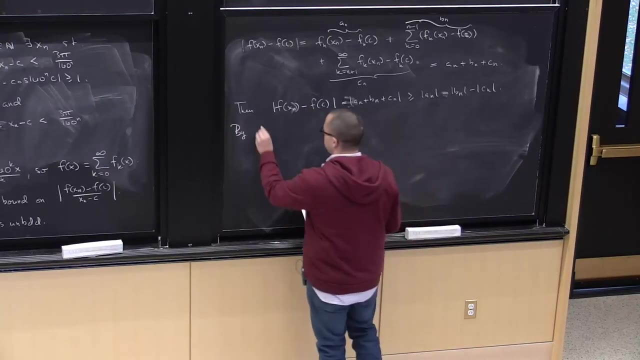 or this sum from below. That means we need to estimate this from below. and then b sub n and c sub n, since they have minus signs from above. OK, Now, by b, a sub n, which is equal to 4, to the minus n. 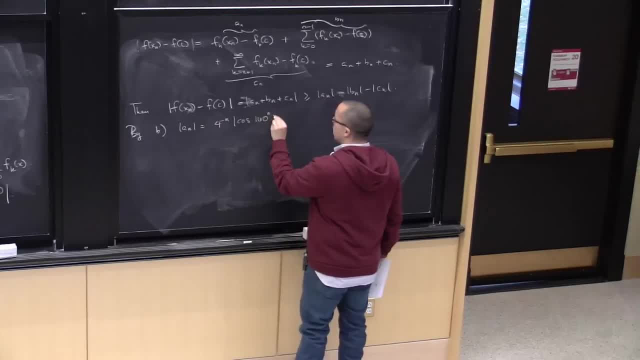 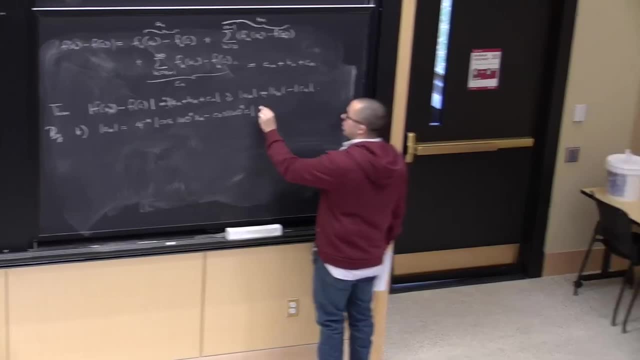 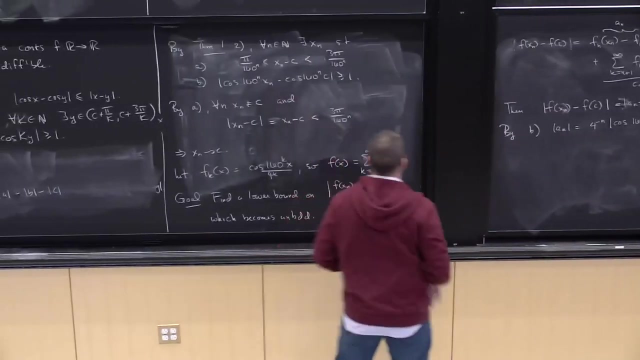 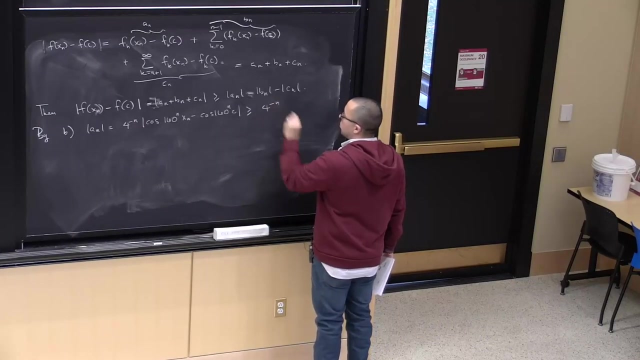 cosine 160 in x sub n, minus cosine 160 to the n c. This is remember how we chose these x sub n's. This is bounded above by 1, or bounded below by 1.. So this is bigger than or equal to 4.. 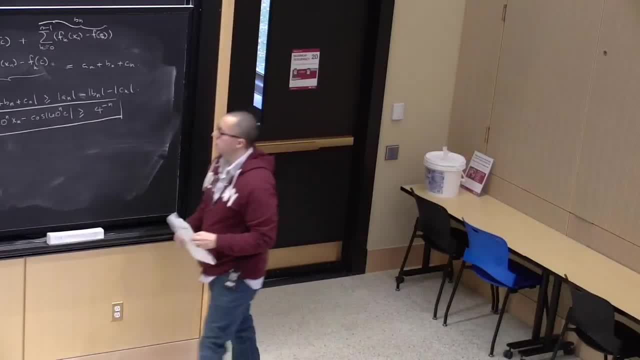 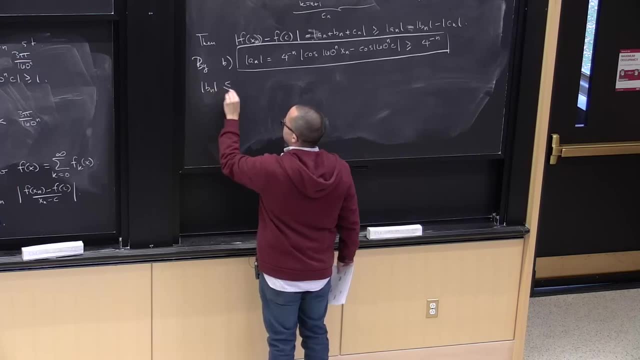 4 to the minus n. All right, So that's a sub n. Now let's look at how big b sub n is. Now we want to bound this from above, because when it hits the minus sign, this will flip the inequality and we'll. 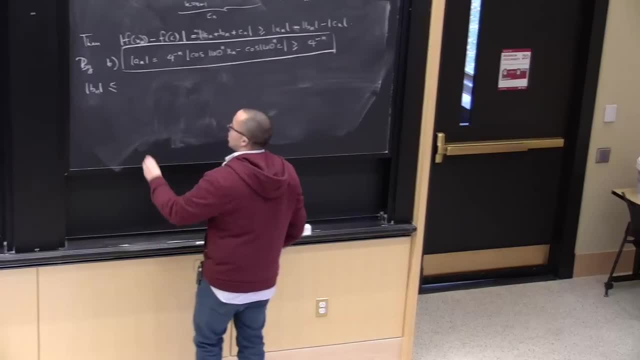 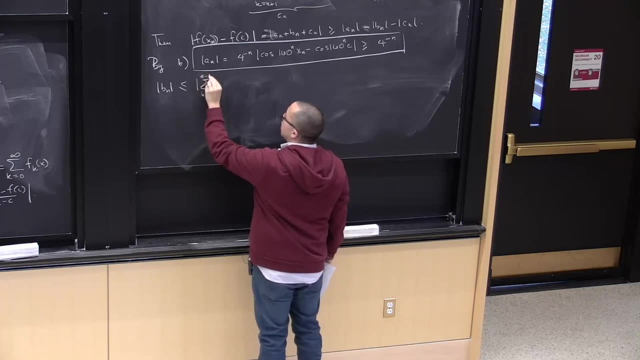 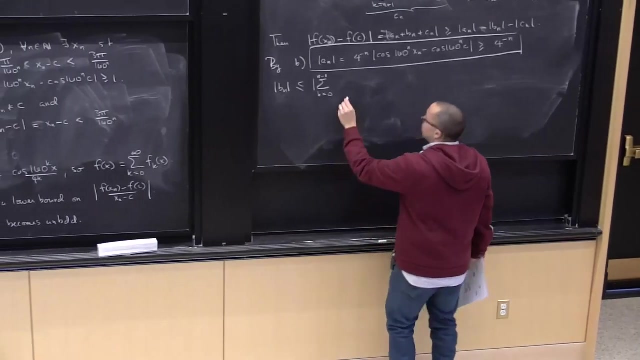 have that this will be bounded from below by something. So the absolute value of b sub n- OK, that's equal to sum- from k- equals 0 to n minus 1, of f, k of x, of n minus f, of c, k of c. 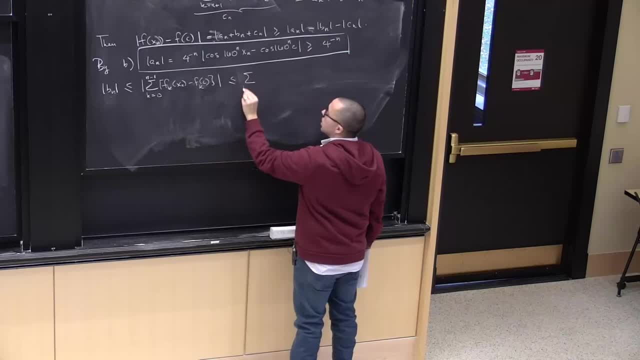 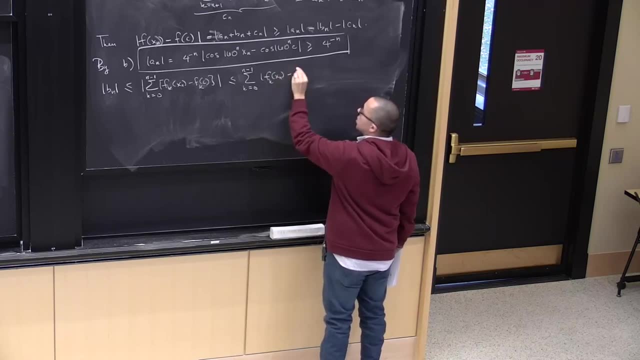 And bringing the absolute values inside by the triangle inequality, this is less than or equal to sum from: k equals n minus 1, of f of f, k, x, of n minus f, k of c. And now, Nice enough, Very good, All right. 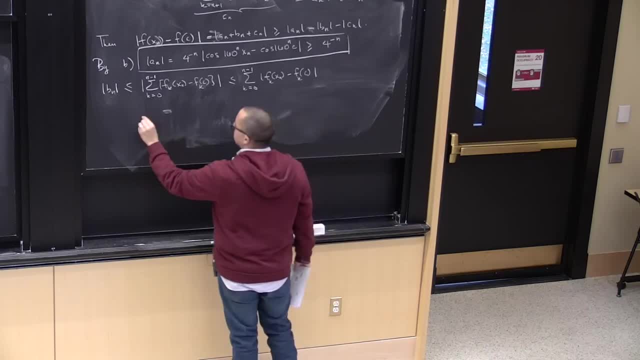 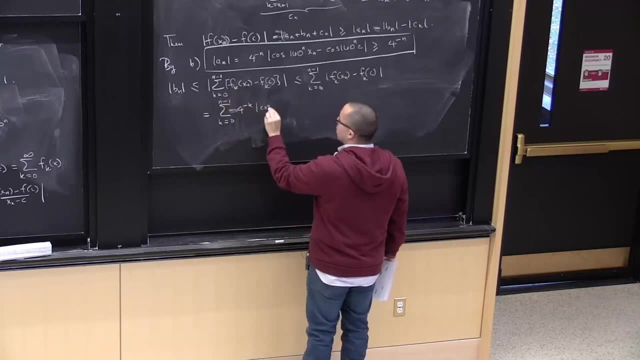 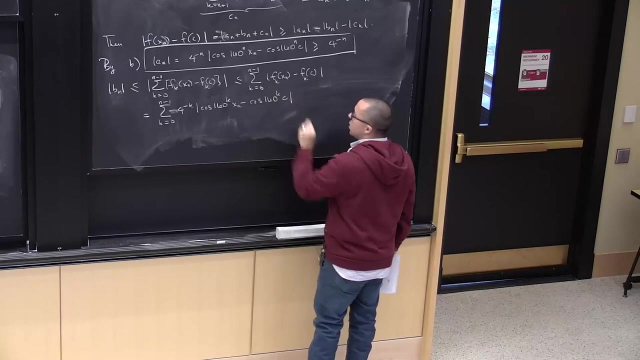 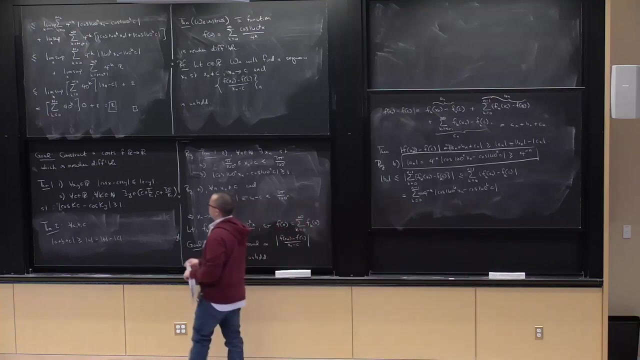 OK, And here Gosh. So this is equal to sum from k equals 0 to n minus 1, 4 to the minus k cosine 160 k x of n minus cosine of 160 k c. And now we use theorem 1, number 2, or number 1, I'm sorry. 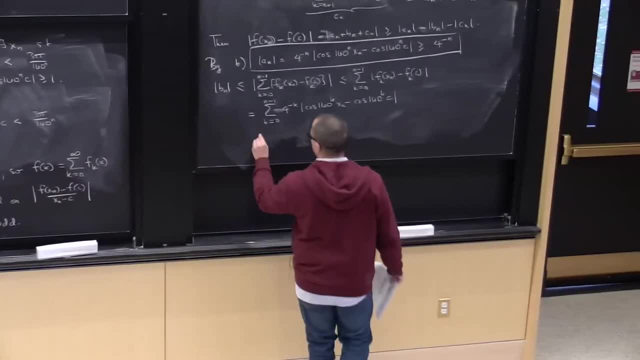 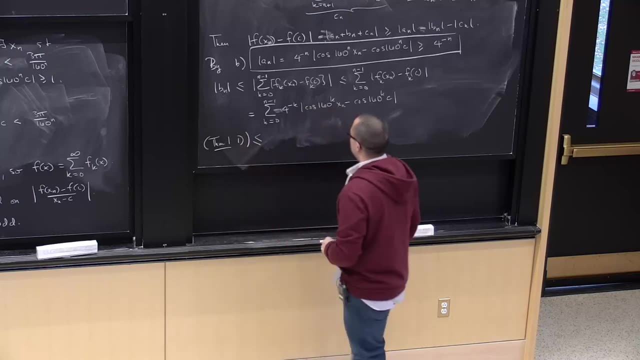 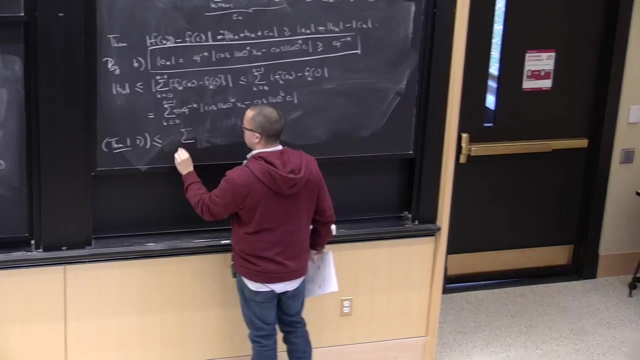 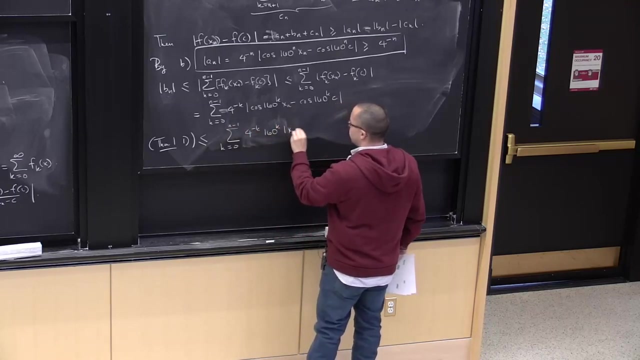 Theorem 1, part 1.. So this is theorem 1, 1.. The difference in these is bounded by 160 k times the difference in those two. so that's, And now these things we can sum up in closed form. 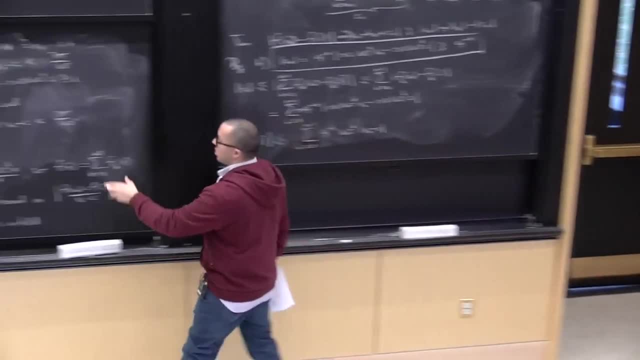 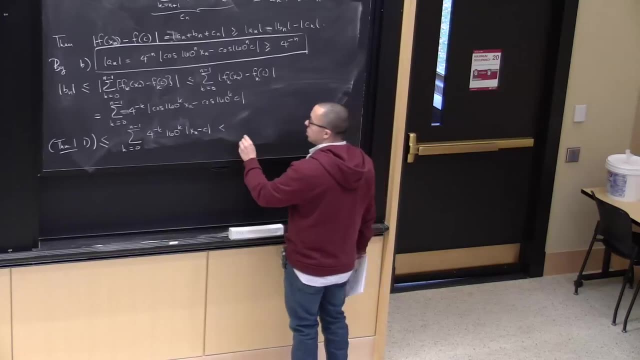 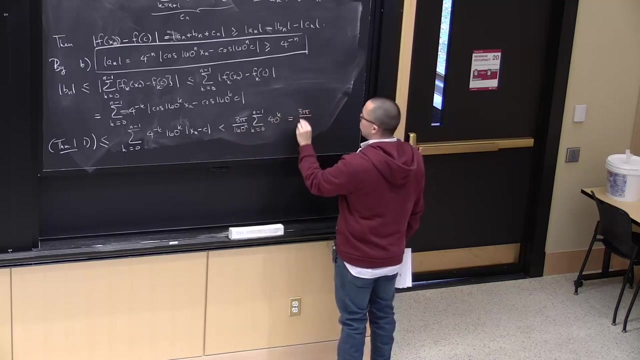 Well, actually, x of n minus c- We proved, We proved- is less than 3 pi over 160 n. So this is less than sum from: k equals 0, n minus 1, 40 k, And this equals 3 pi over 160 n. 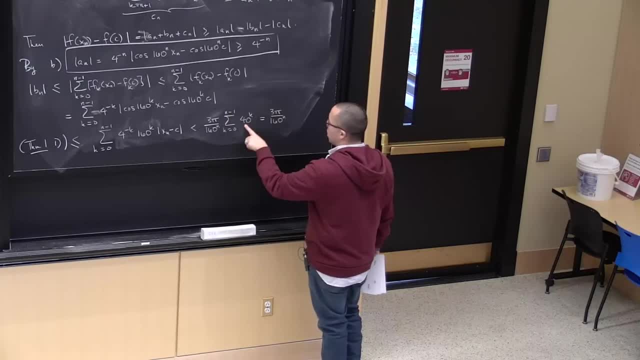 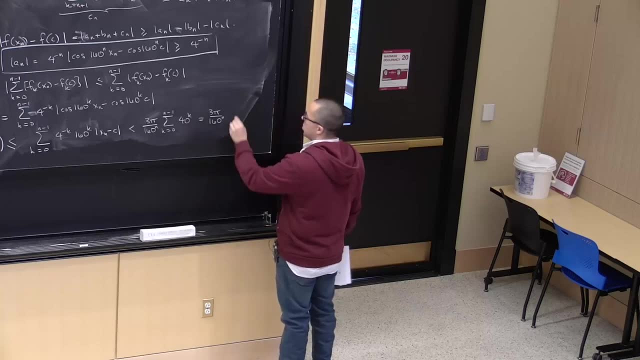 Now, sum from k equals 0 to n minus 1, 40 k. We use this formula for summing a geometric, Geometric sum. This is equal to what? is this? equal to 40 to the n minus 1 over 39.. 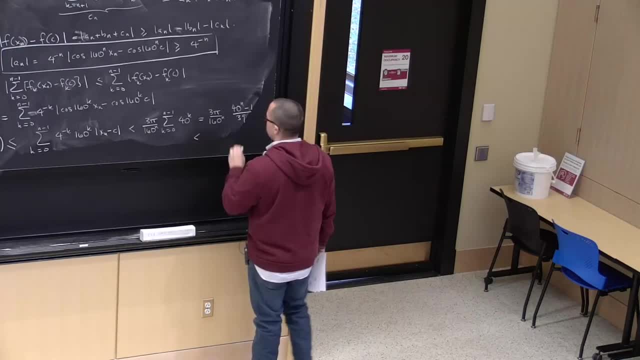 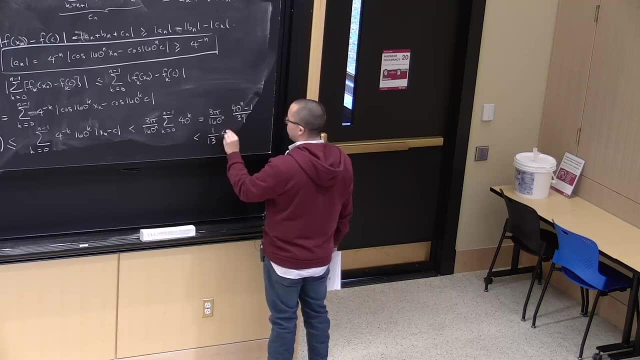 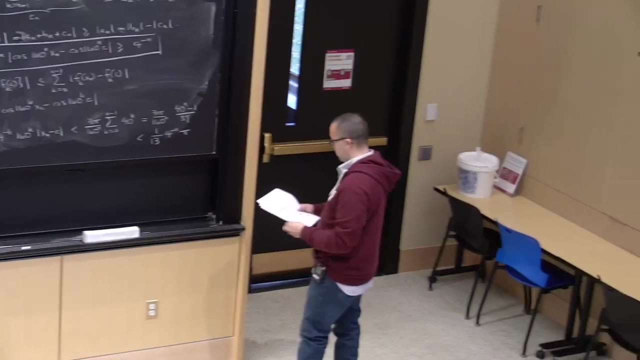 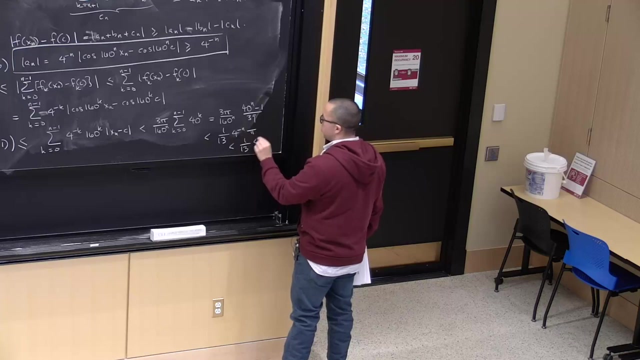 And which is less than okay. so take away the 1.. This is 1 over 13.. 4 to the minus n times pi. All right, And that's less than pi is less than 4, so plus 1.. 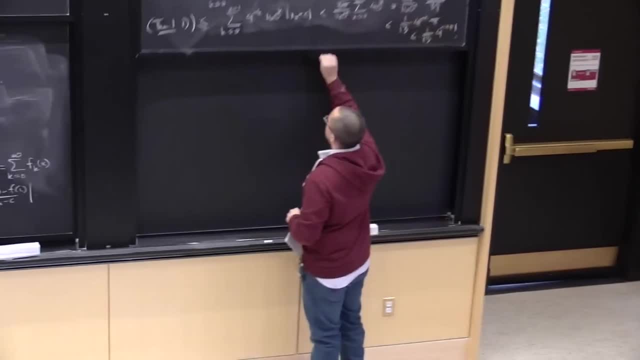 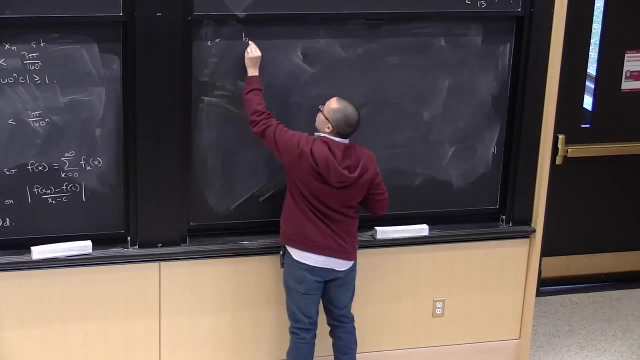 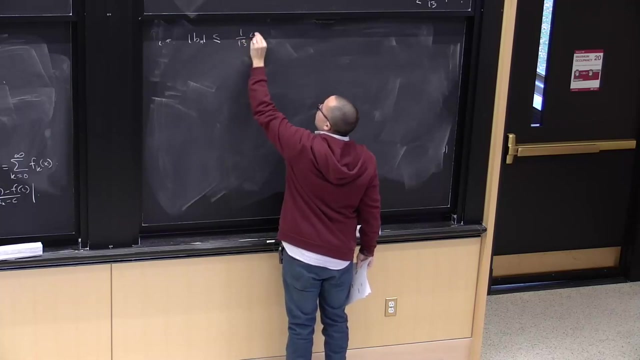 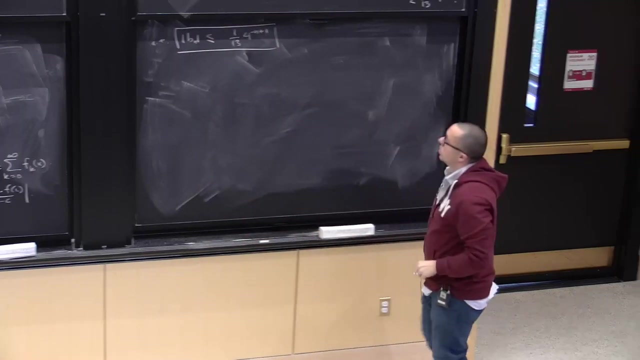 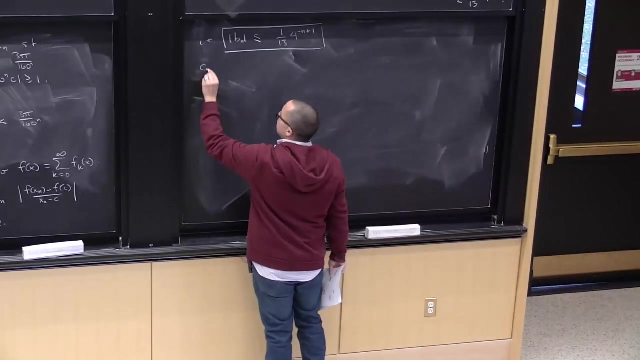 Okay, So let me summarize this. This is less than or equal to 1 over 13,, 4 to the minus n plus 1.. Okay, Okay, Now for the last box. this is less than the absolute value of c. 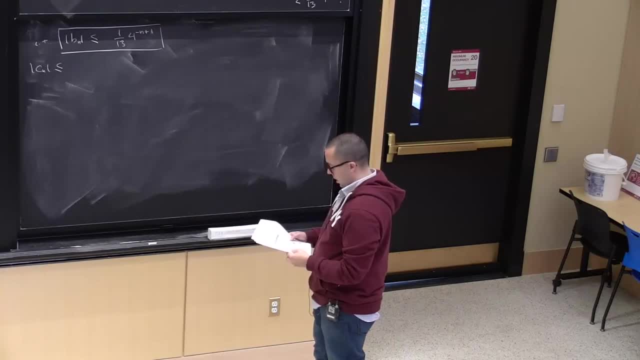 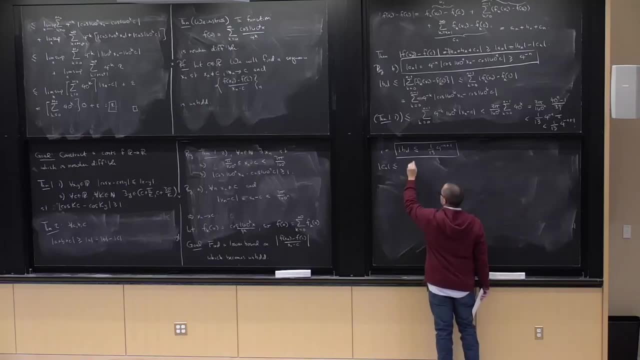 b sub n. an absolute value is less than or equal to. now we just kind of do a brutal estimate. We bring the absolute values inside. Okay, so this is equal. so just as we had before with the b sub n's. 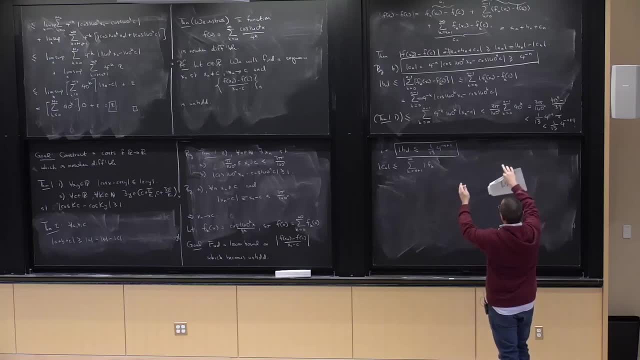 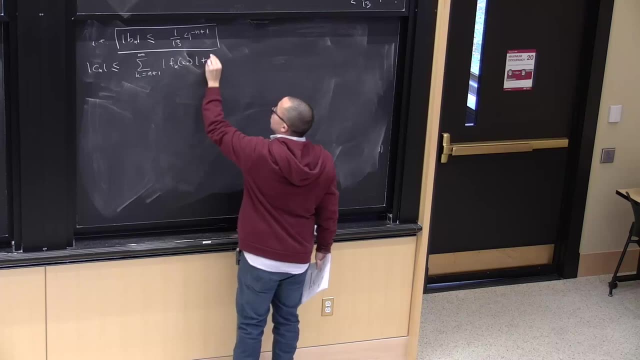 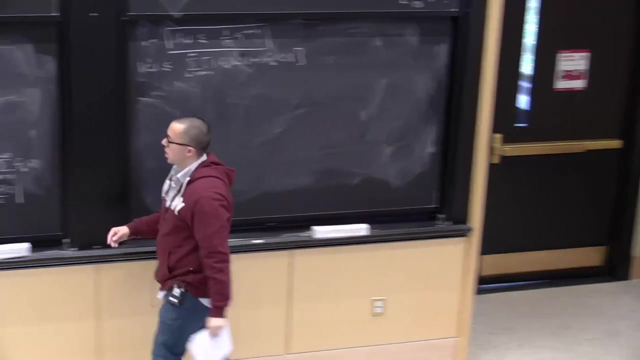 except now we're summing from: k equals n plus 1 to infinity, brought the absolute values inside, And then let's use the triangle inequality on that. This is Remember: fk is equal to cosine of 160k times x over 4 to the k. 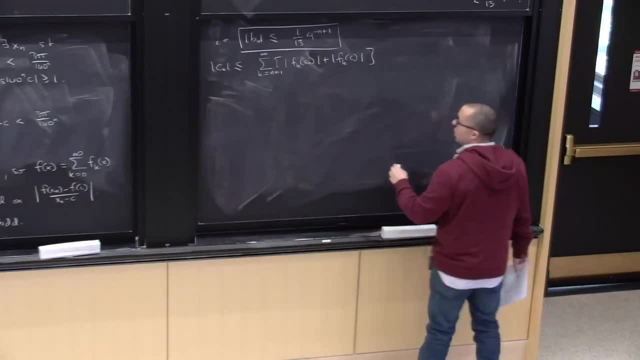 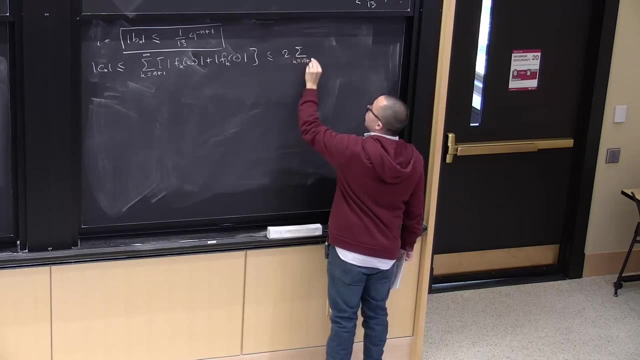 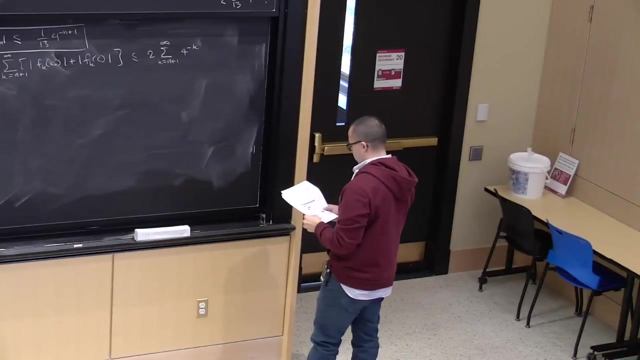 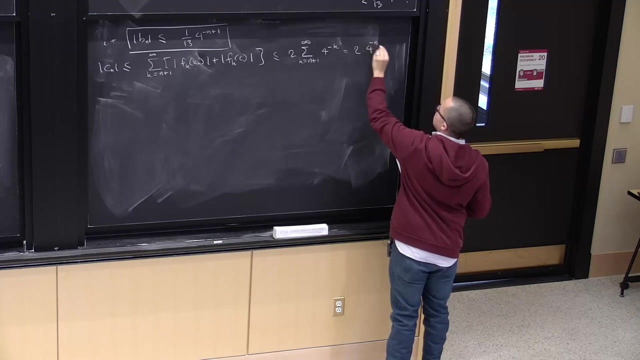 So that's no matter what you plug in, that's bounded by 4, 1 over 4 to the k. Okay, and now this we can actually sum: This is equal to 4 to the minus n minus 1 times sum from. 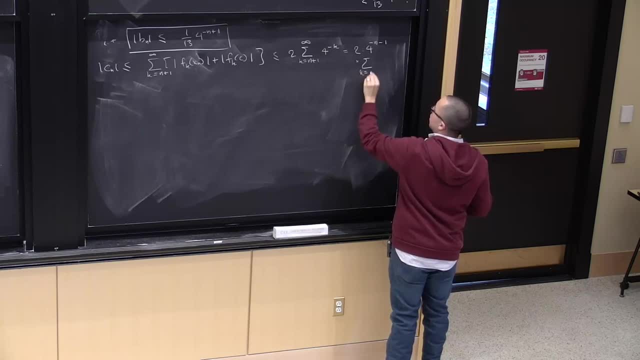 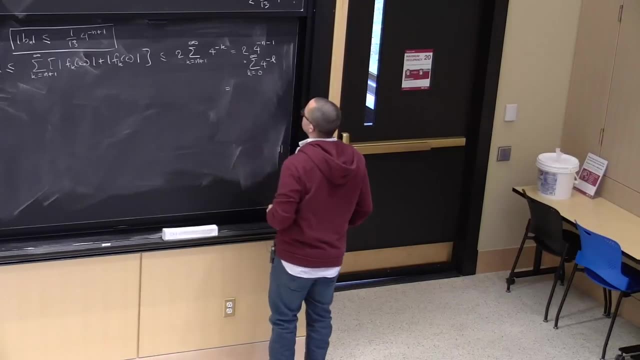 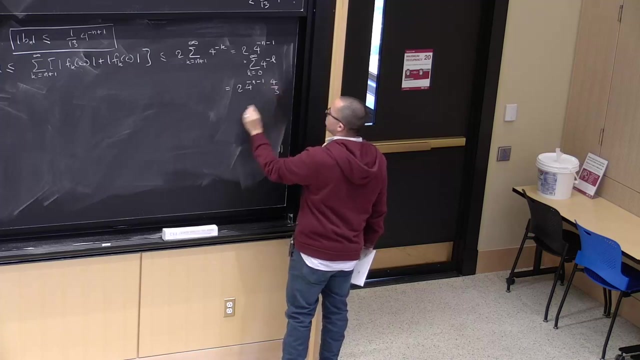 l equals 0 to infinity, of 4 to the minus l. And what does this equal? This equals 2.. Okay, 2 times 4 to the minus n minus 1 times 4 3rds equals 2 3rds 4 to the minus n. 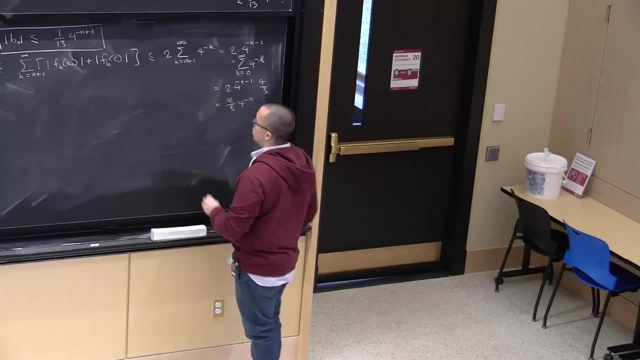 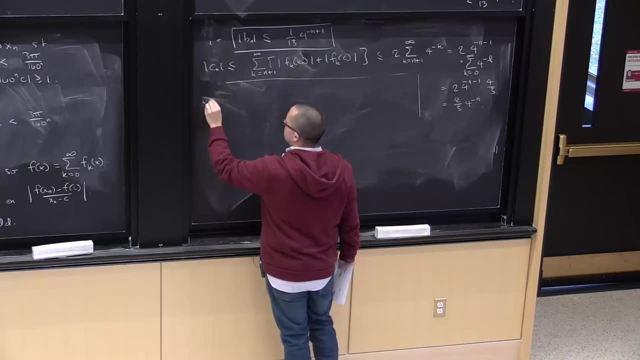 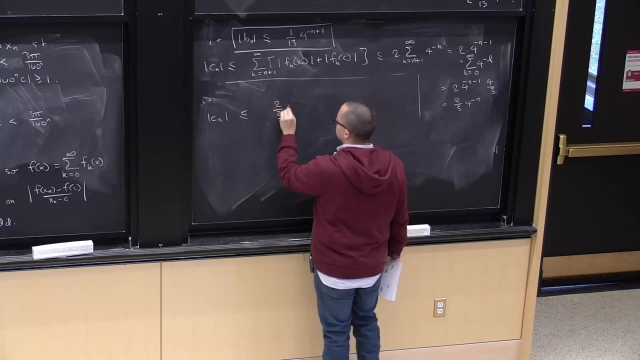 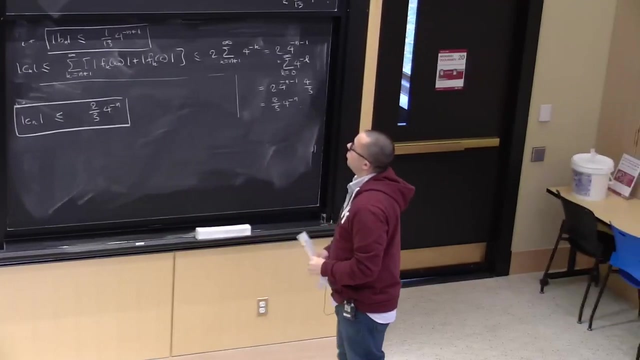 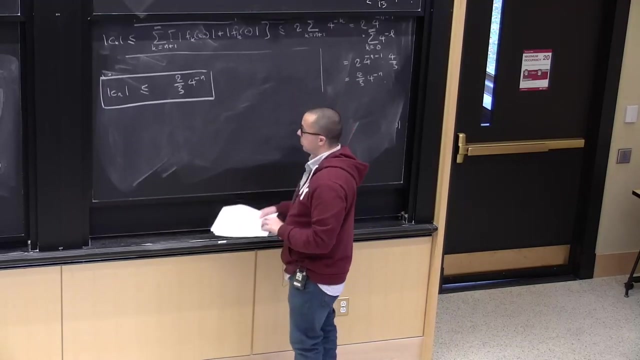 Okay, So my board work's getting a little shoddy, but it'll be okay. Ie, we've proven that the absolute value of c sub n is bounded by 2 3rds minus n. All right, so combining everything that we've done, 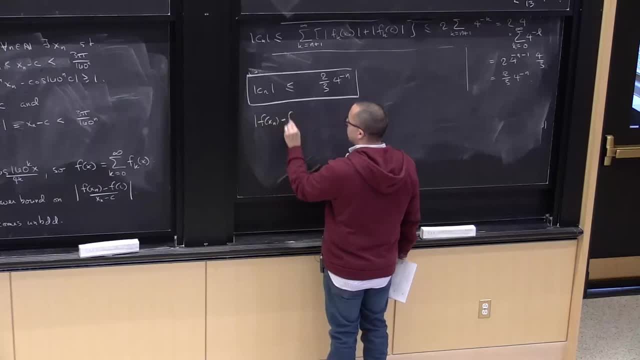 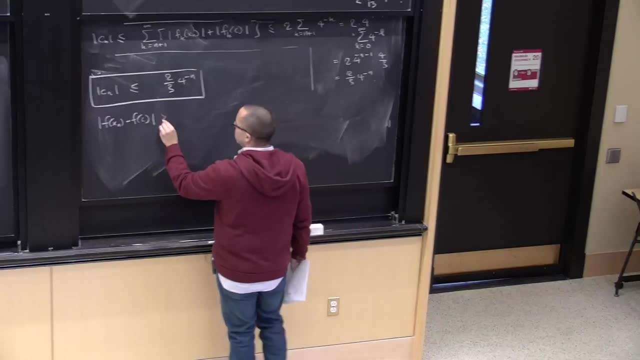 we've shown that f of x sub n minus f of c, which remember is equal, is bounded below by: 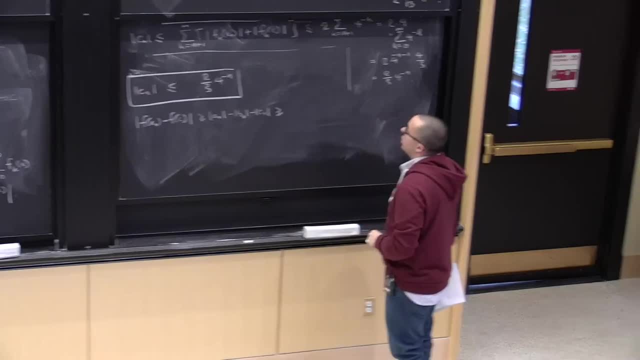 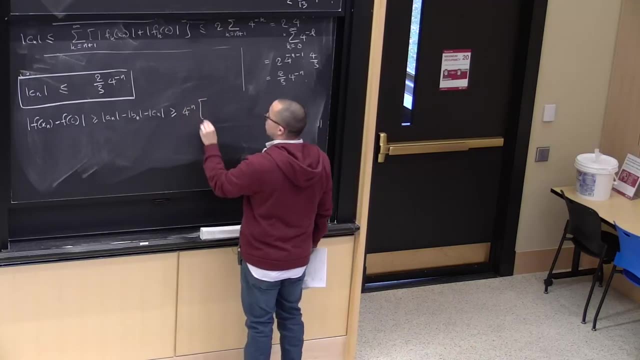 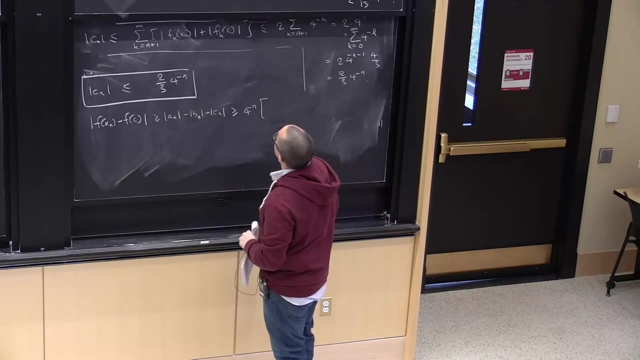 This is bounded below by a sub n, remember. so the first box is bounded by 4 to the minus n. So first off everything, the a sub n, b sub n, c, sub n, they all have some 4 to the minus n involved. 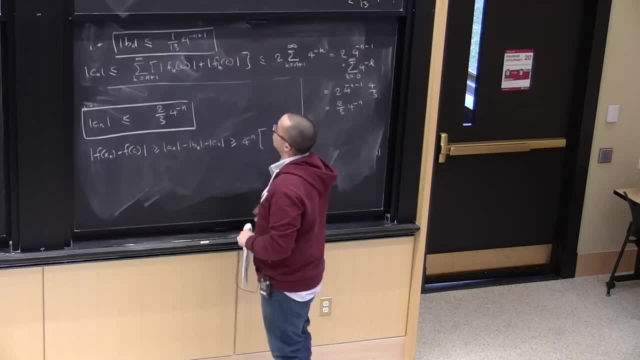 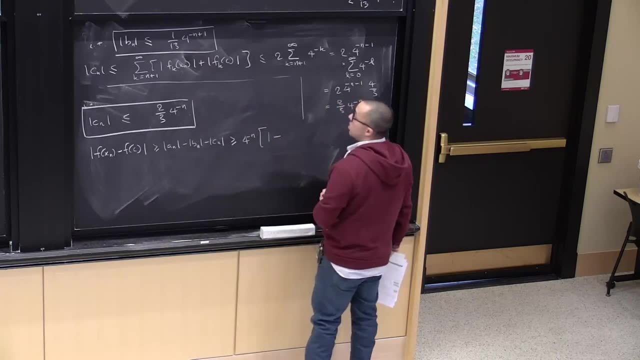 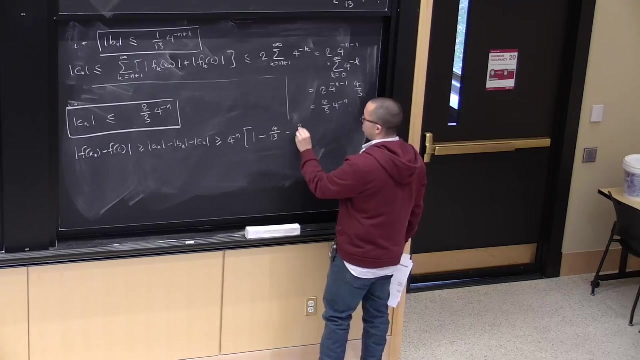 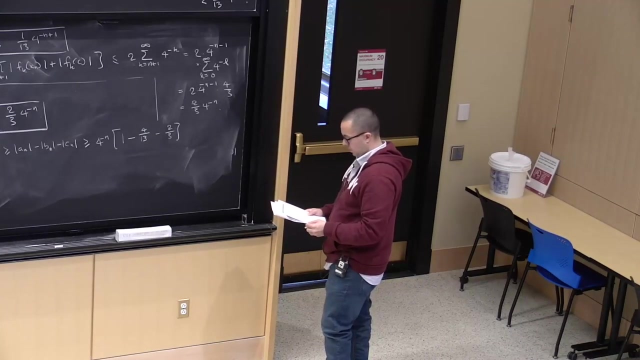 What happened to my estimate for b? Oh, covering it up, 4 to the minus n. this is 1 coming from the a sub n's and minus 4 over 13 coming from the b sub n's, minus 2 thirds coming from the c sub n's And if you do the arithmetic, this is 4 to the minus. 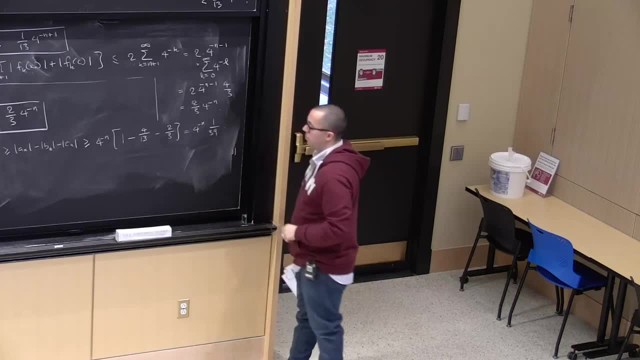 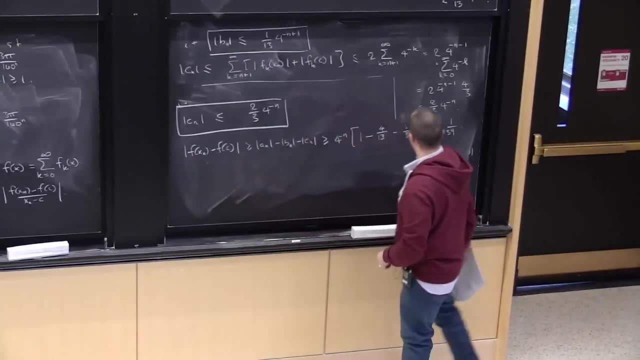 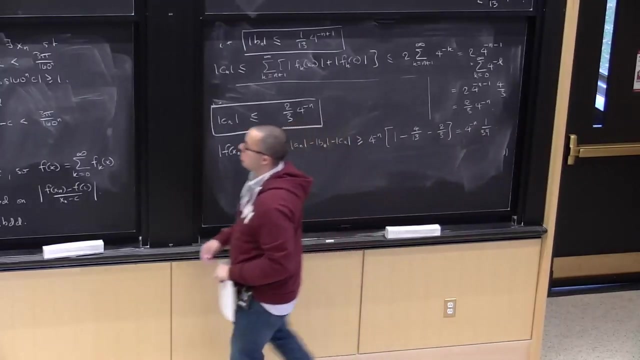 n 1 over 39. So f of x sub n minus f of c is bounded from below by 4 to the minus n times 1 over 39. Now I just divide by x sub n minus c, which is bounded above by 3 pi. 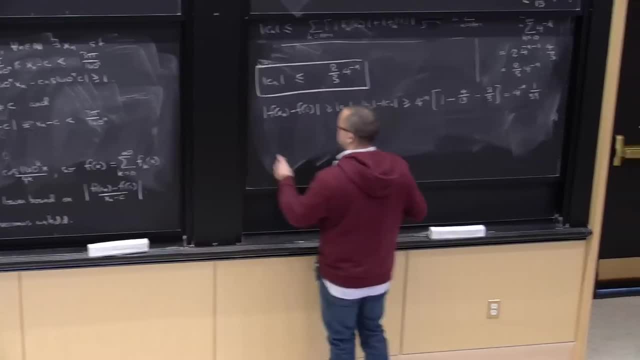 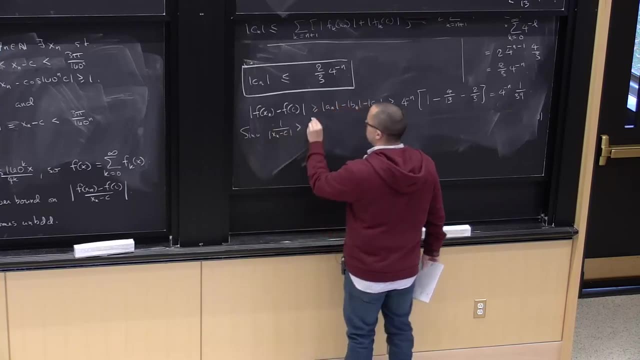 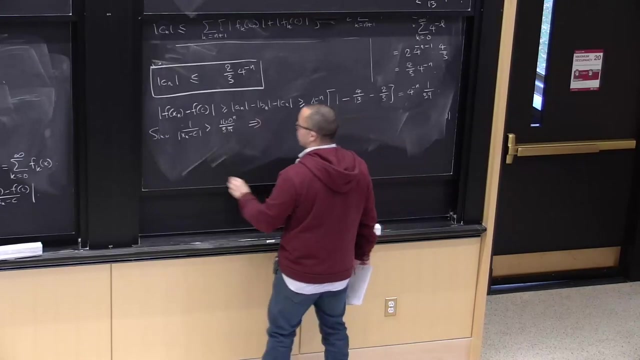 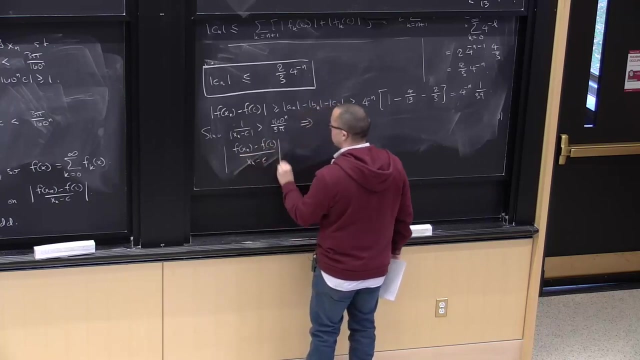 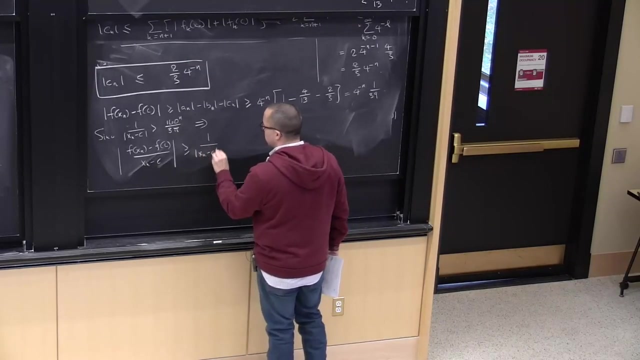 over 160 n And therefore when I Take reciprocals I get that. I get that the absolute value of f of x sub n minus f of c over x sub n minus c is bounded from above by 1 over x sub n minus c times 4 to. 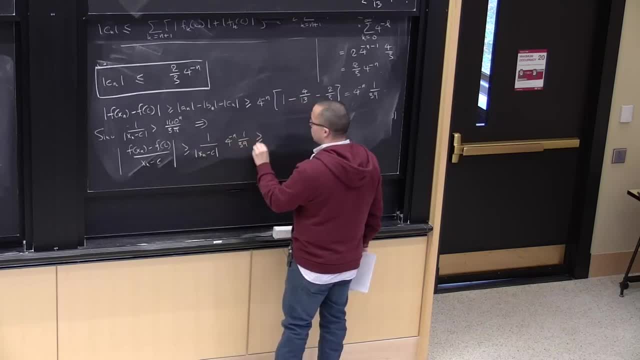 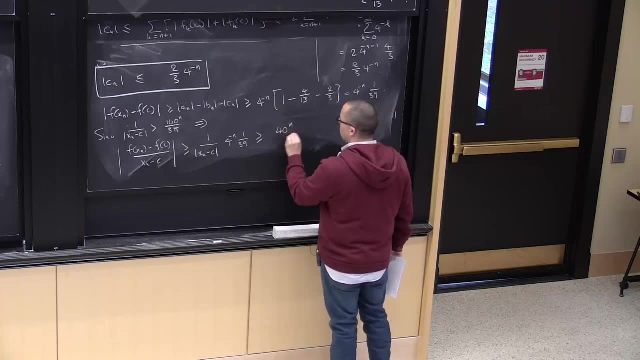 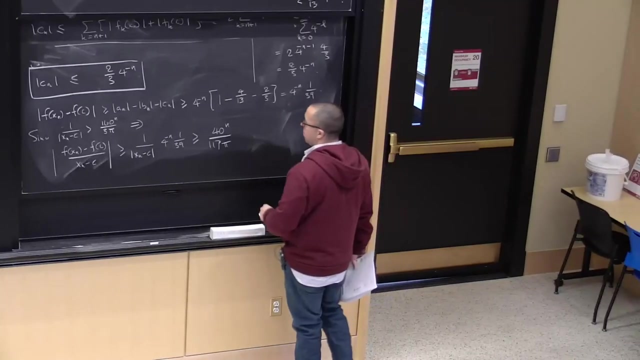 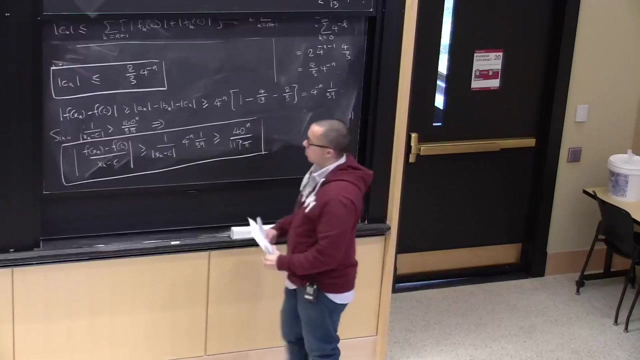 the minus n 1 over 39, which is bounded below. by Now inserting This estimate here, I get 40 n over. I think that's 117 pi. Is that it? Yes, And therefore the absolute value of the difference quotient is bounded below by 40 to the n over some. 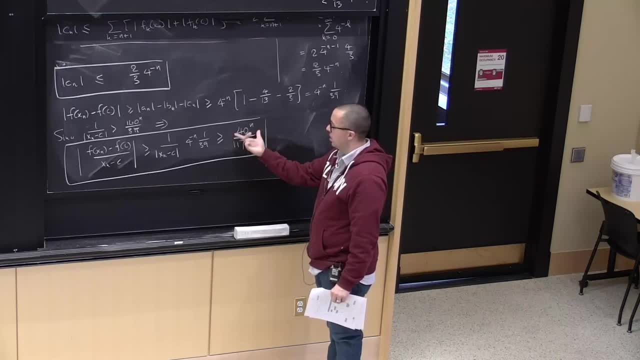 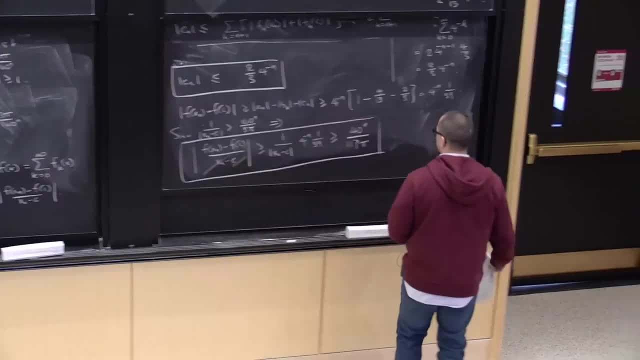 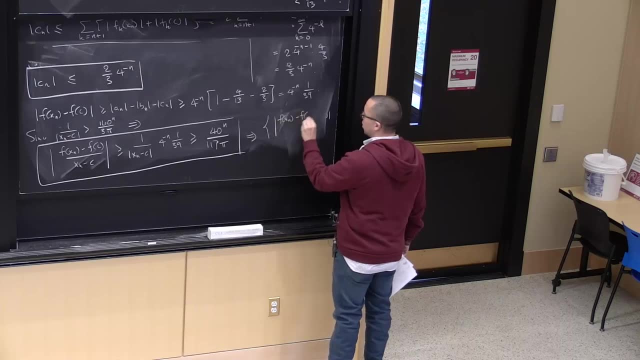 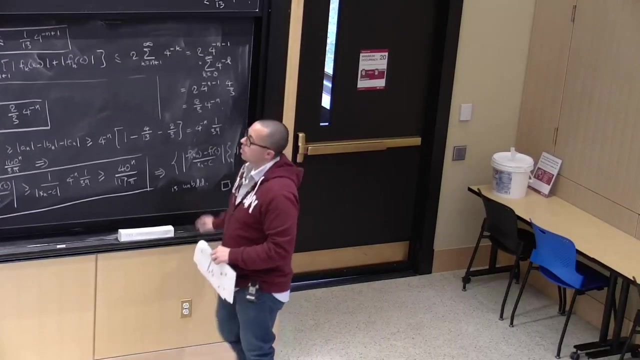 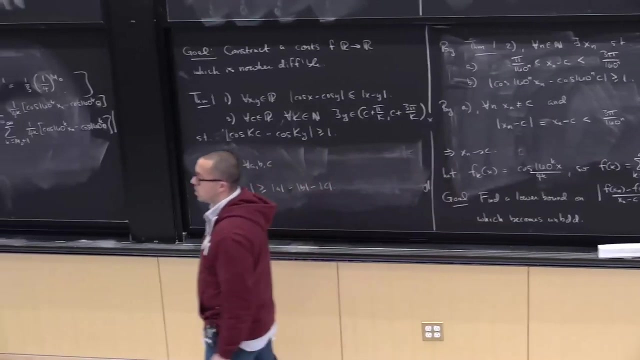 And therefore the absolute value of this difference quotient is unbounded. which finishes the proof. All right, So we've done some things. If things, maybe a few things- that you haven't seen in calculus course, definitely haven't seen, this most likely, and really this is the first result that 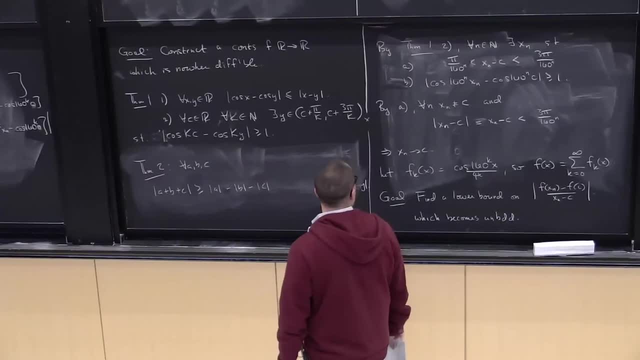 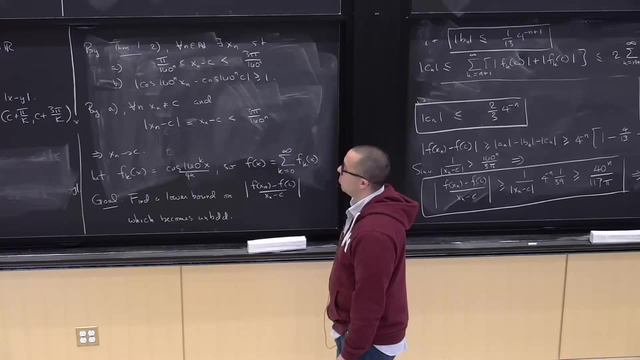 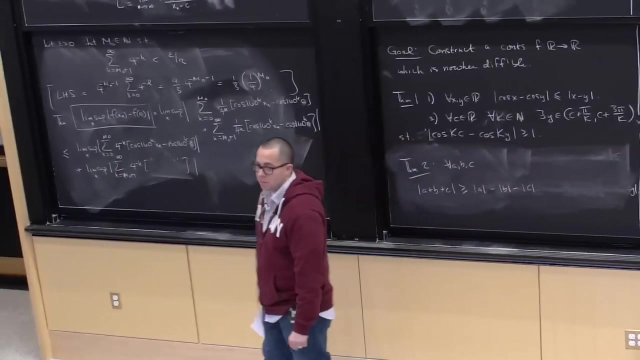 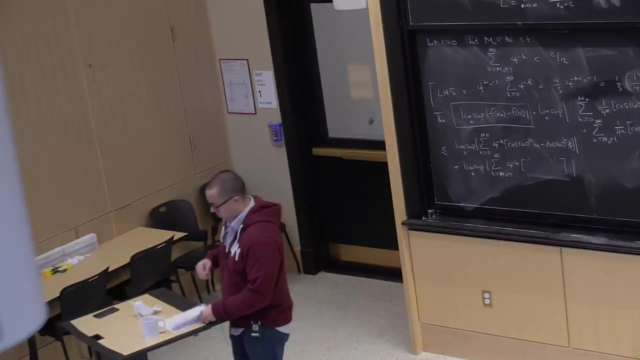 involves, you know, a lot of math that we've covered up to this point to prove a very, you know, non-trivial and deep theorem: that that differentiability is is a bit of a miracle. okay, it's a miracle when it happens. okay, we'll stop there.